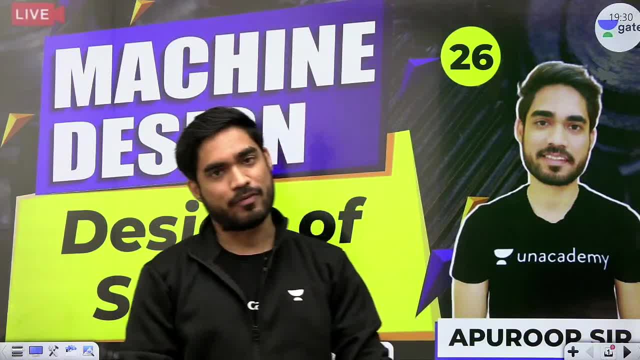 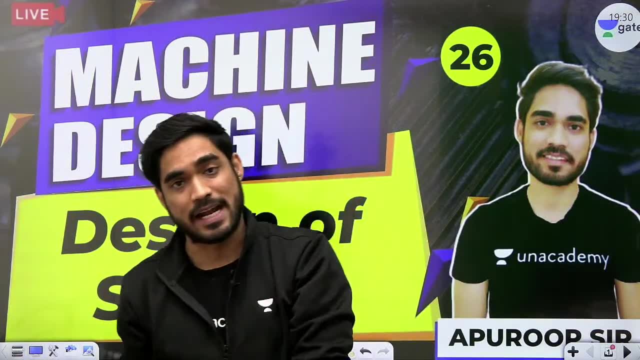 Today we are going to complete the entire syllabus of machine design, Whatever is in the syllabus of GATE. I have taken each and every topic. Each and every topic is explained in detail. I have covered all the theory part, all the numerical parts, all the PYQs. 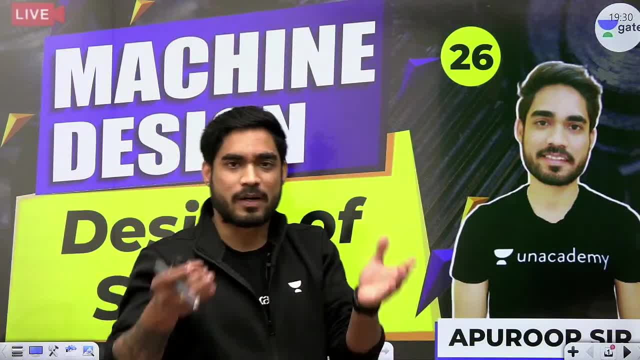 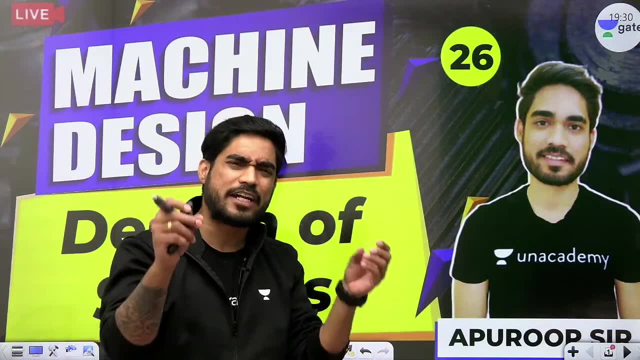 So this is one comprehensive course, Although it's a crash course, but it is more than a comprehensive course of machine design If you are preparing for GATE 21,, GATE 22,, GATE 23,, whatever year you are preparing for. 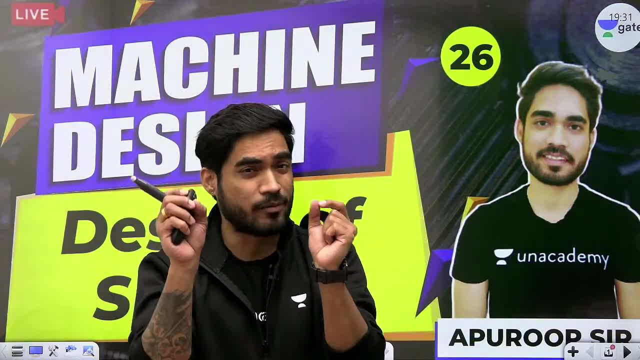 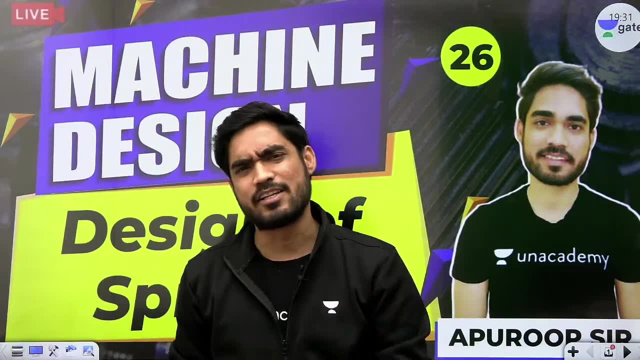 You can watch this entire lecture series because this will be a single source of preparation for machine design. This will be a single lecture series of machine design. If you watch this lecture series, then after this you don't need any other source of machine design. 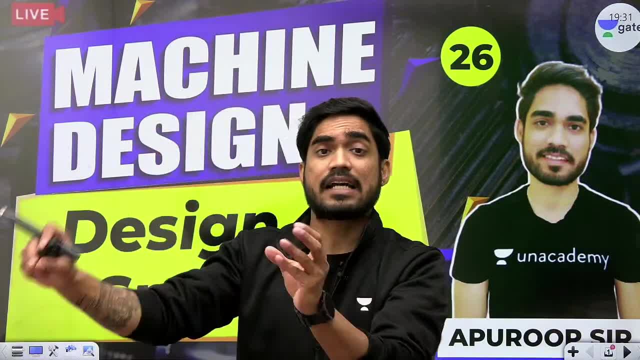 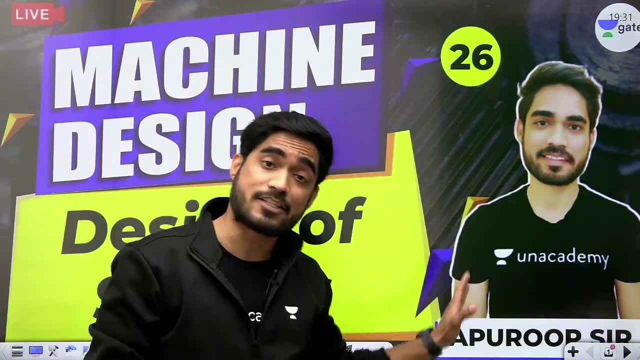 You don't need any book. you don't need any lecture. This is my guarantee, Even previous year questions. I have solved all the topics in the class. In this lecture series. you get everything: Theory, numericals, PYQs, everything. 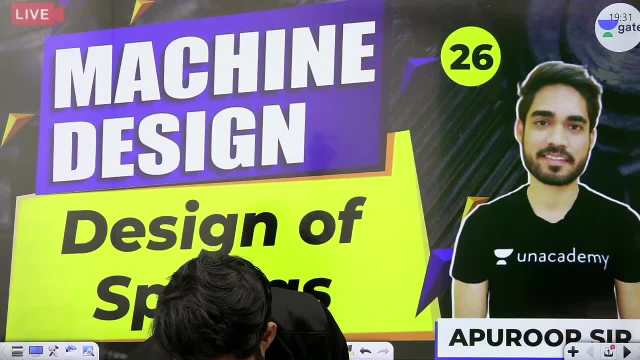 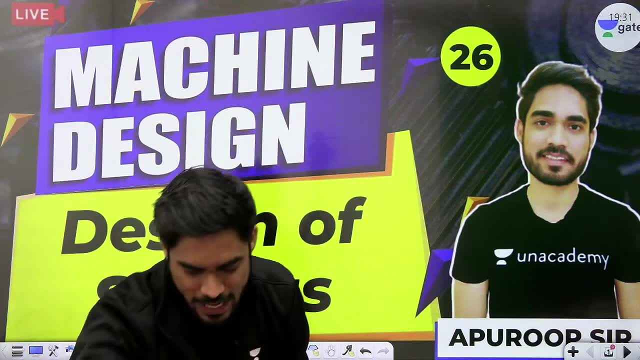 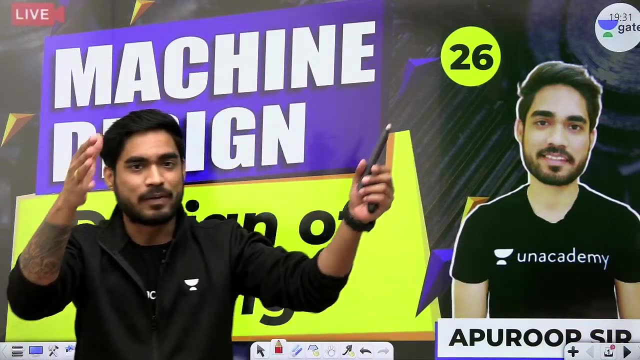 So this will be the last class of machine design and we will complete the entire syllabus of machine design with this lecture. Good evening Ankita, Good evening Kalpesh. So don't forget to hit the like button and don't forget to share the link with your friends and tell them that this is a complete lecture series of machine design. 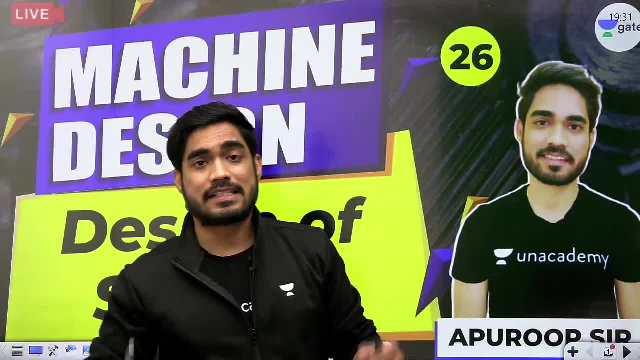 You can share the link of the playlist with all your friends and tell them that this is a complete lecture series of machine design, If you are preparing for GATE 21,, GATE 22,, GATE 23,, whatever year you are preparing for. 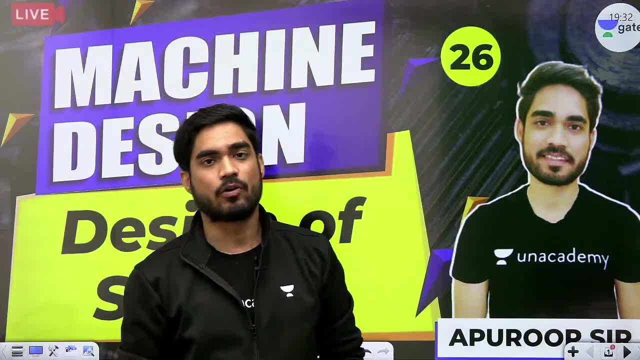 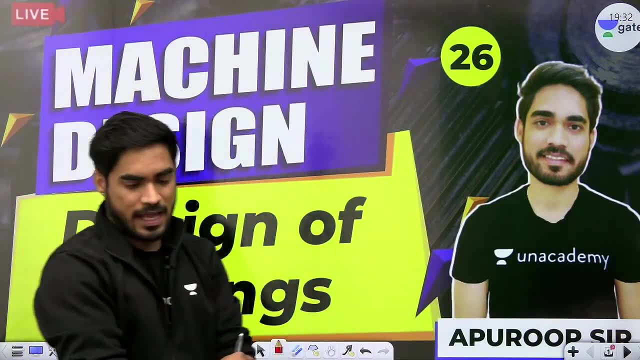 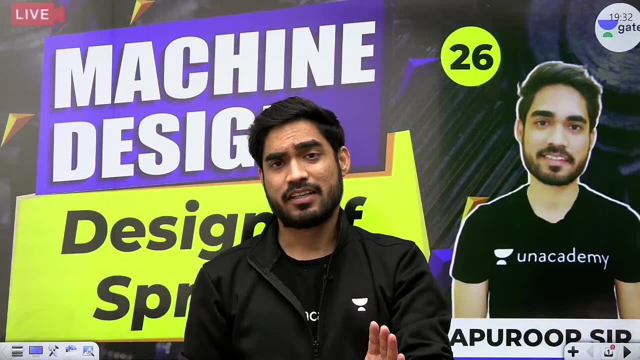 If you are preparing machine design on your own, if you are studying machine design by yourself, then you don't need to worry. You just watch this lecture series and your entire machine design will be prepared. So this is design of spring. Today, we are going to learn about the design of spring, which is the most, the most, not the most. 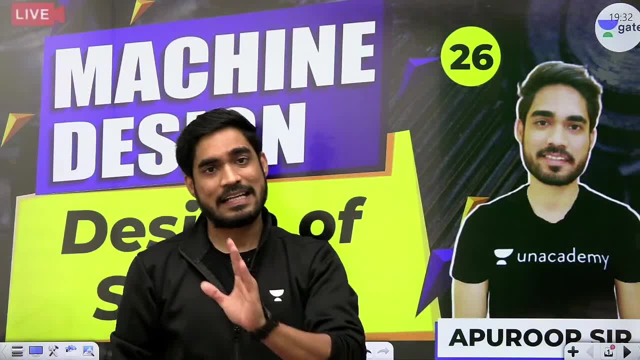 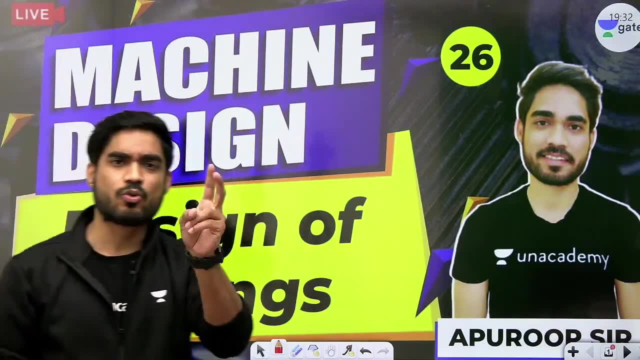 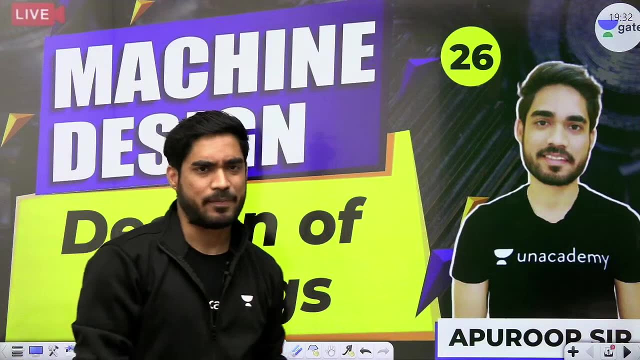 It is the easiest chapter of machine design and you can easily solve any question of machine design, any question of springs, With just two equations. Two equations and all the questions are made. It is a very simple chapter, Very, very easy chapter. 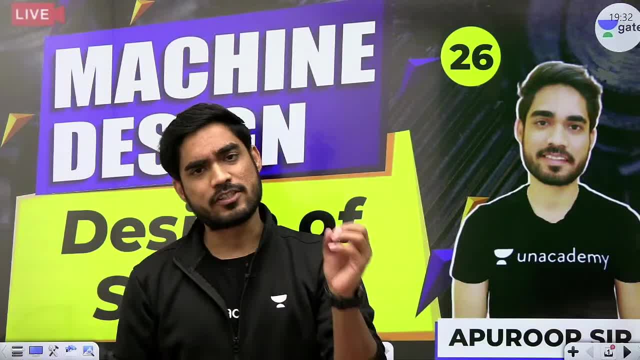 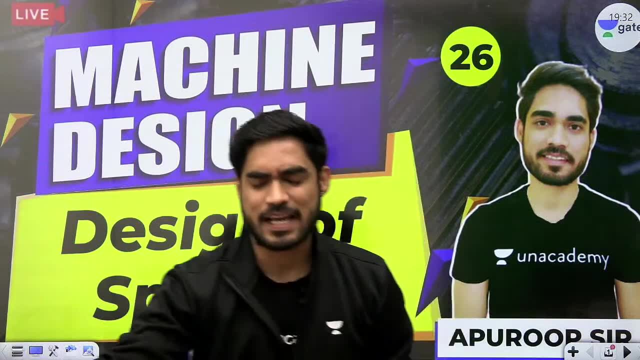 If you get a question from design of spring means son, you will score definitely 100 out of 100 in machine design. If the question of spring is stuck with machine design, son, it will be made easily. It will be made very easily. 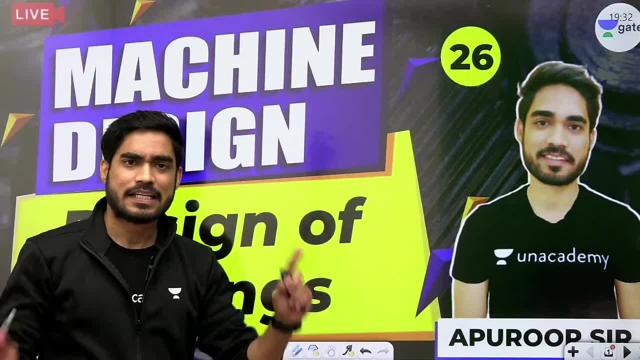 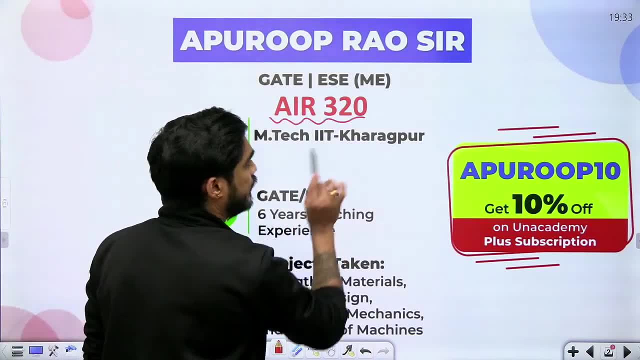 Okay. So today we are going to complete design of spring. We are going to complete the entire machine design. Okay, If you are watching me for the first time, let me introduce myself. My name is Apruv Rao, All India rank 320 in gate mechanical. I have done my MTech from IIT Kharagpur. My specialization was design. 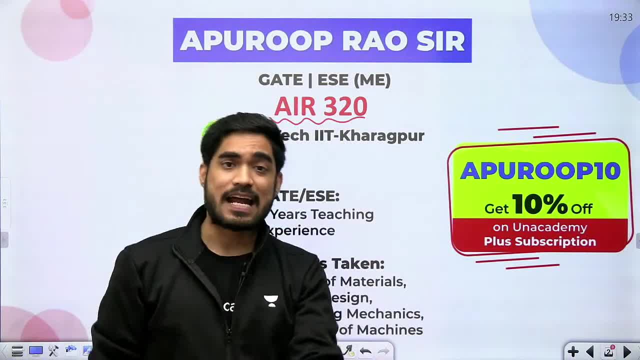 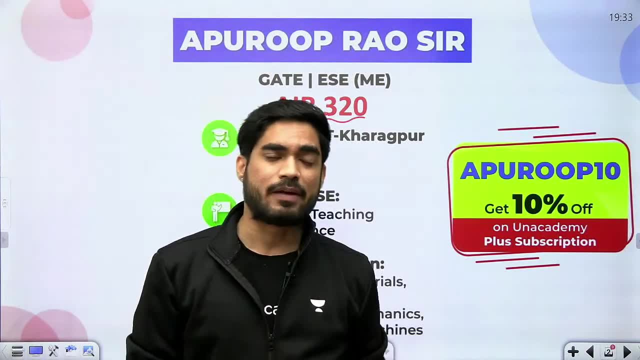 In my final year I was recruited by Mahindra and Mahindra and I was placed at Mahindra Research Valley, which is the R&D of Mahindra, where the cars and tractors of Mahindra are designed. So I worked there as deputy manager for two years in the field of design. 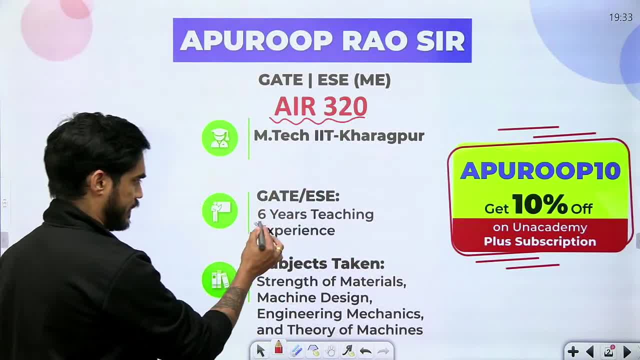 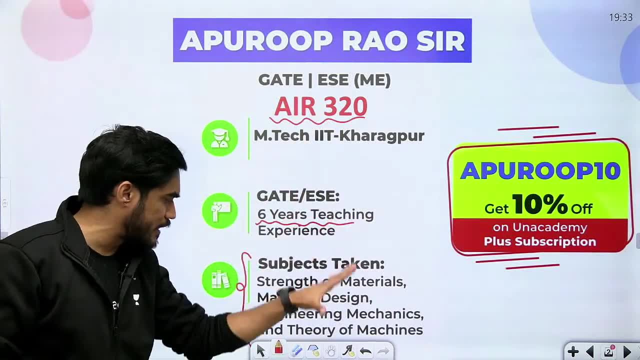 Then I decided to quit my job and I started teaching. So I have been teaching for more than six years now And I teach all the subjects of design, SOM, MD, EM, TOM, And you can watch the lecture series of all these subjects. 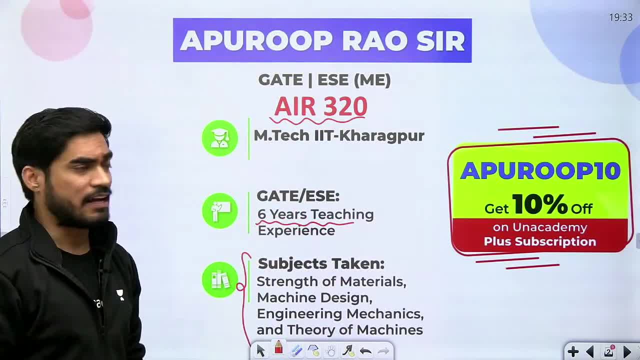 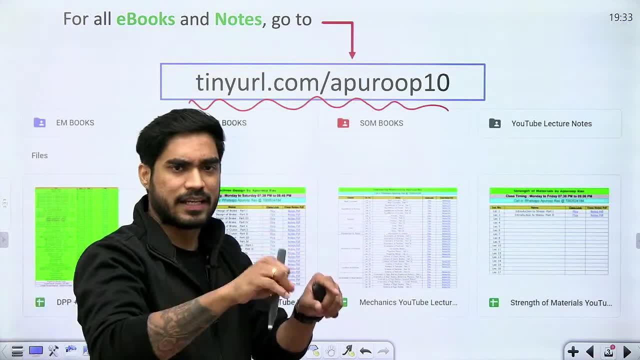 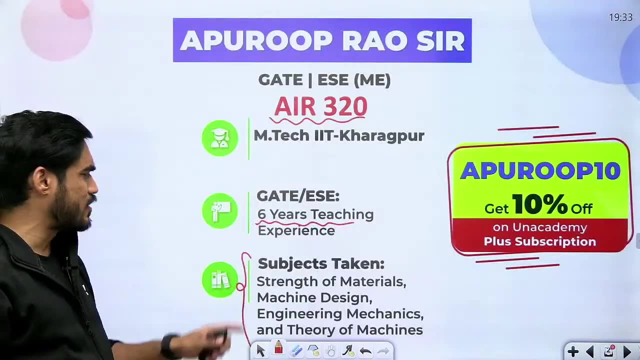 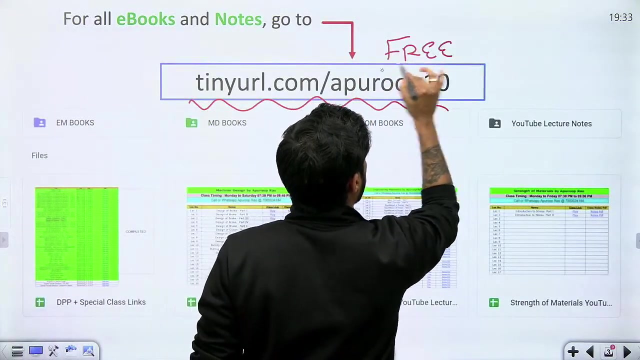 The complete lecture series of all the subjects is available here in this link: tinyurlcom- slash- approve10.. Open this link, son. Type this link in your web browser. Enter this address in your web browser. Enter And you will get the entire lecture series of strength of material, machine design, engineering, mechanics and theory of machine completely free of cost. 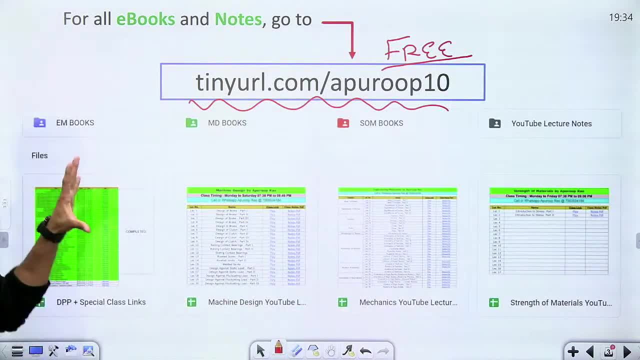 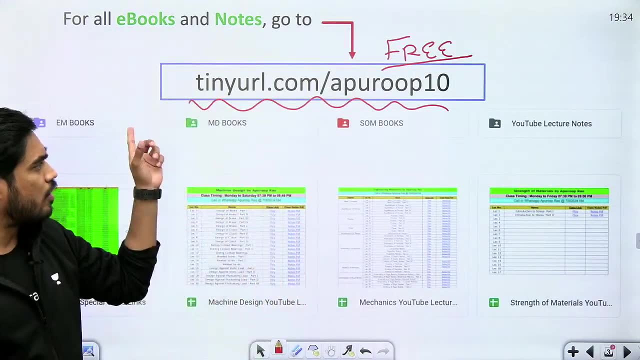 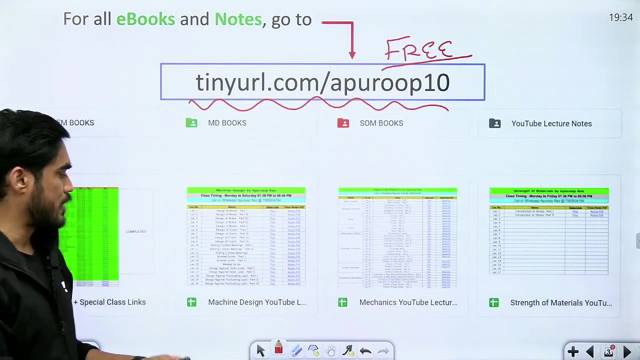 The entire lecture is completely free, my brother. Anyone can watch it. You can watch it anytime, You don't have to pay anything. You don't have to pay anyone. The entire content on this link is completely free. You will get the video. You will get the PDF of every class. 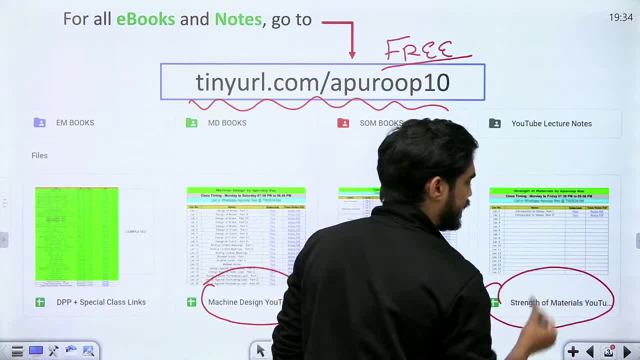 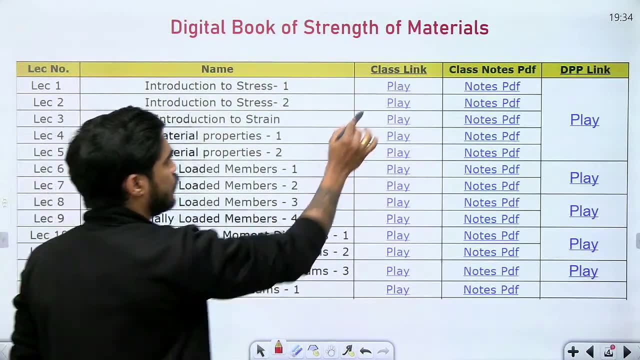 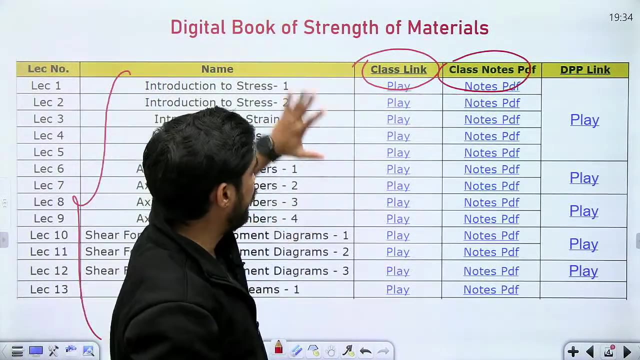 So I have prepared subject-wise Excel sheets. in this link I have made subject-wise Excel sheets And in these Excel sheets you will find the YouTube class link, the PDF, Everything you need about that subject. Everything is here, son. 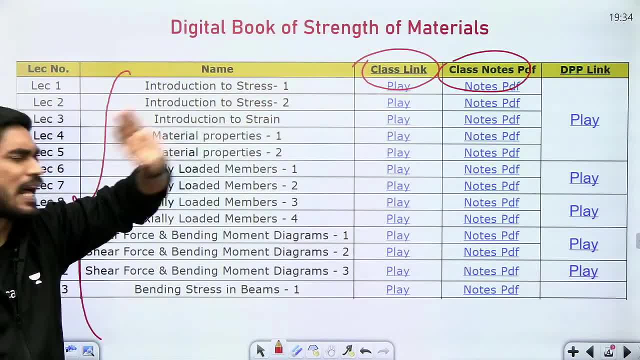 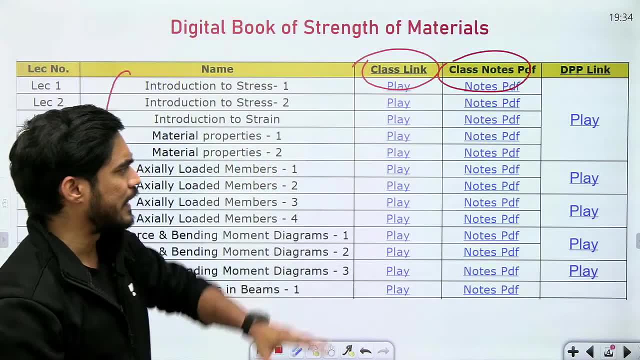 All the things: YouTube class, PDF, everything, Special class. Everything is updated, son, So you don't have to go here and there, You don't have to search anything. Everything is well organized, well structured in these Excel sheets. 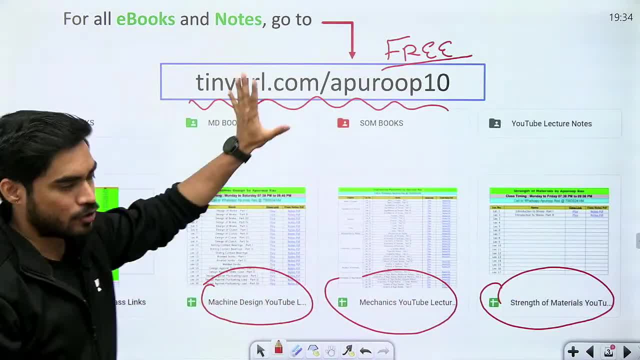 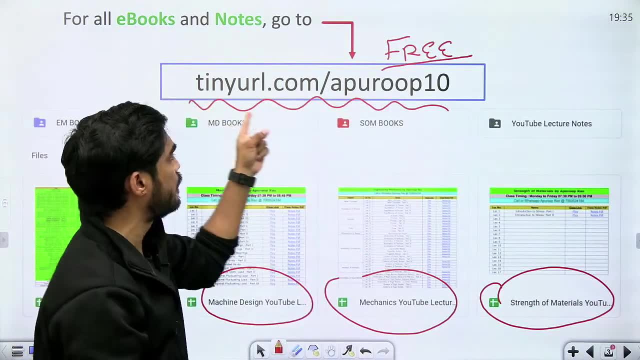 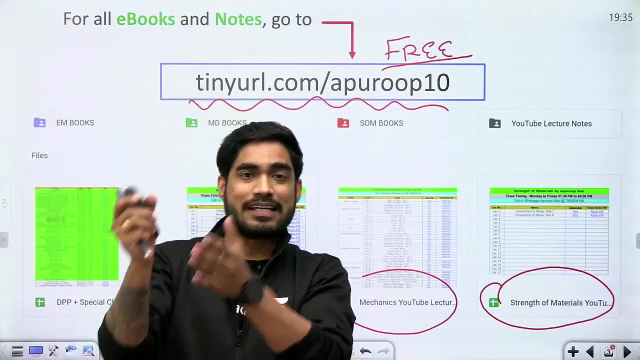 Subject-wise Excel sheets. For every subject there is an Excel sheet. So, son, all you need is open this link, And don't forget to share this link with your friends also. Tell your friends about this link as well. Let them know that there are entire free lecture series of strength of materials, machine design, engineering, mechanics and theory of machines. 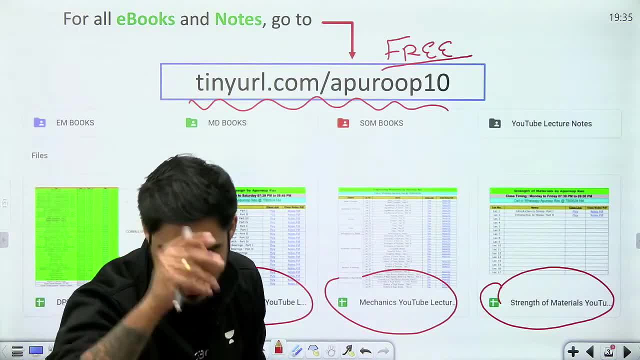 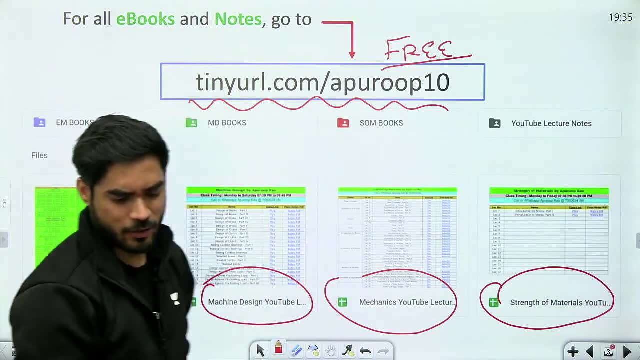 Okay, Good evening Shivam. Good evening Sonali. Good evening Prem. Welcome everyone. Good evening Amrend. Good evening Pravalika. Good evening. good evening. good evening Welcome, son Welcome. 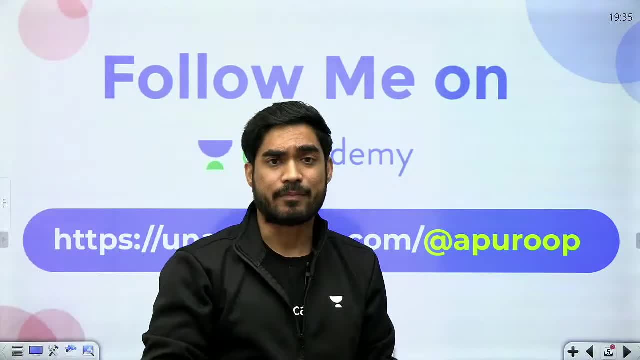 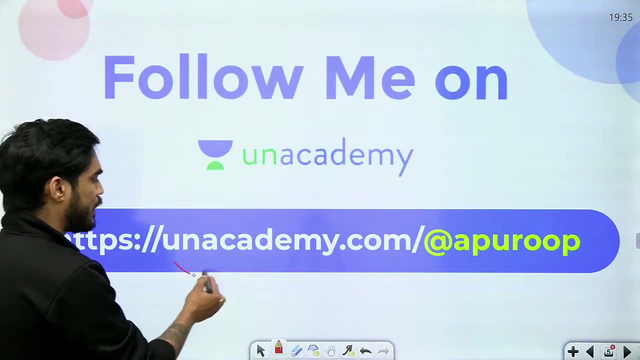 And you can also follow me on Unacademy. You can also follow me on my Unacademy profile. My Unacademy profile link is this: Unacademycom- Slash At the rate approved. You open this link and you will go to my profile. 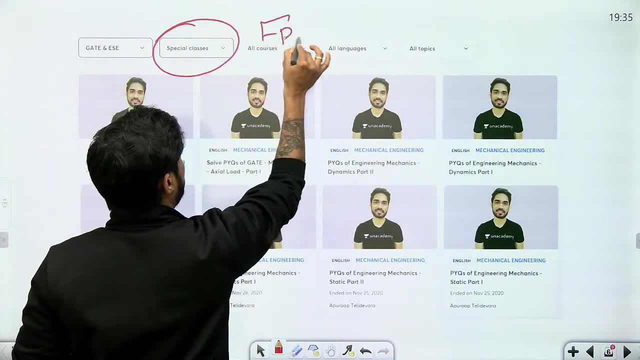 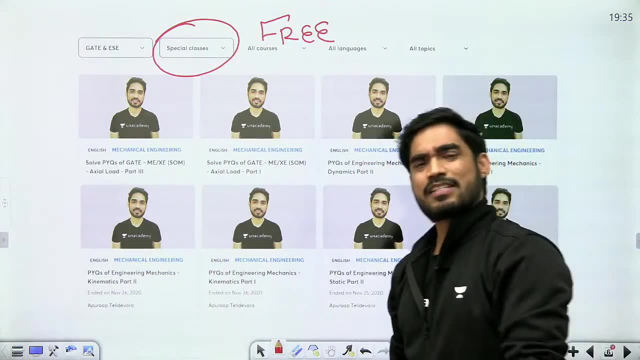 And there you can watch all my free special classes in one place. You will see all my special classes in one place. I have taken special classes on some very important topics of design. I have taken special classes on all the PYQs of design. 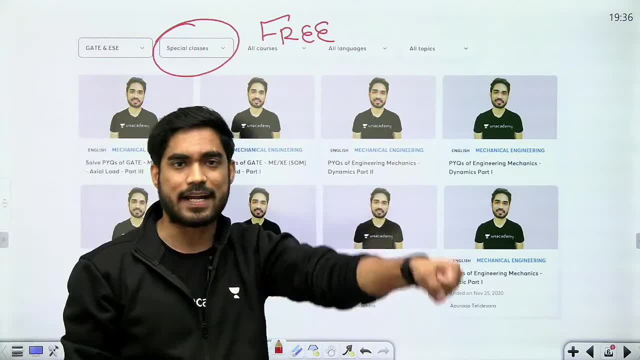 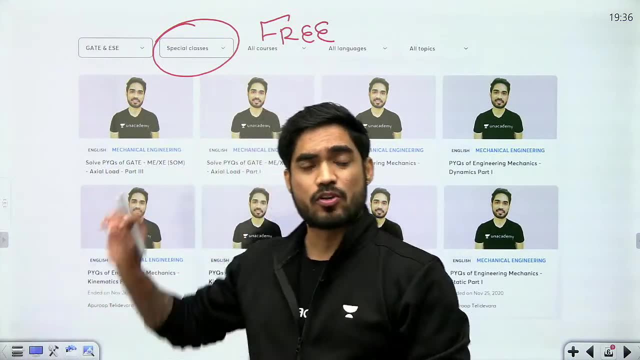 EM, SOM, EMD, All the PYQs Previous year questions of GATE. We have solved them in special classes. Okay, So if you want lecture by like topic by topic. PYQs of the subjects of design son. 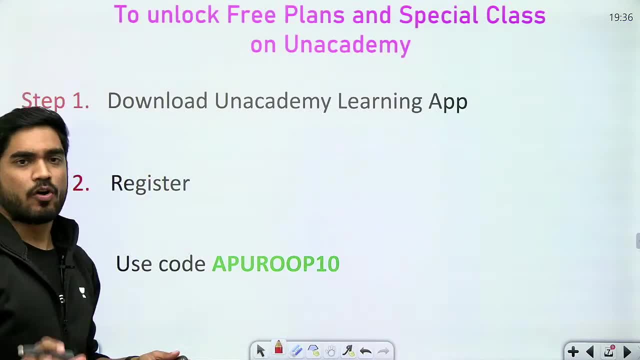 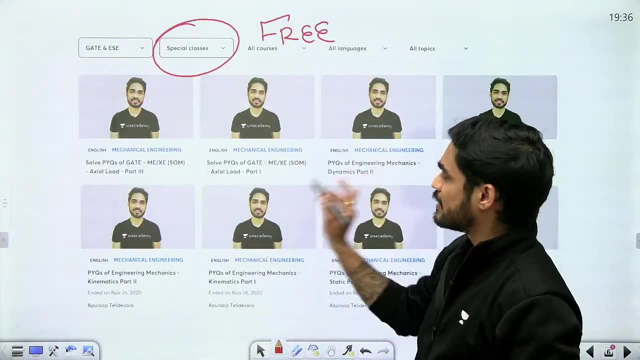 Don't forget to go to this. Okay, And if you want to watch these classes, what you need to do is you need to download Unacademy learning app, Because these special classes are taken on Unacademy, So you need to download the Unacademy learning app. 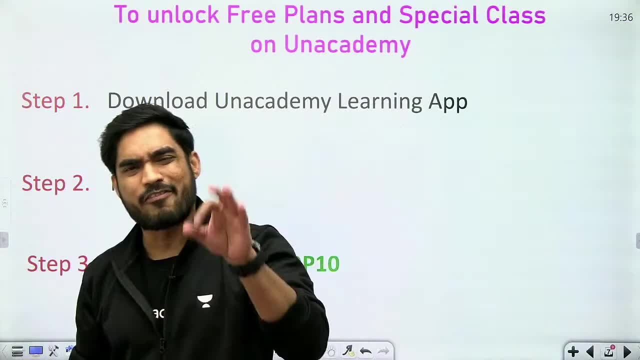 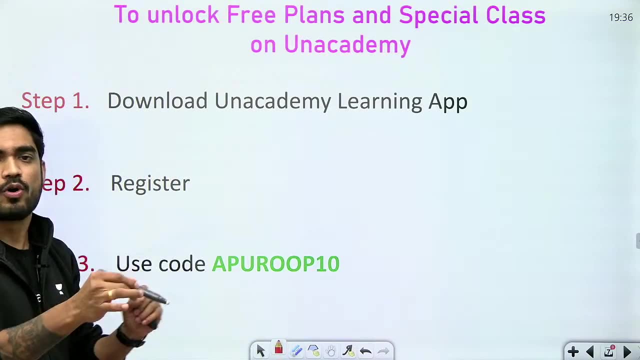 You need to register. And then, son, If you are trying to open your first special class, Okay, If you open your first special class of your life, then they will ask you to put a code. So what is your code? 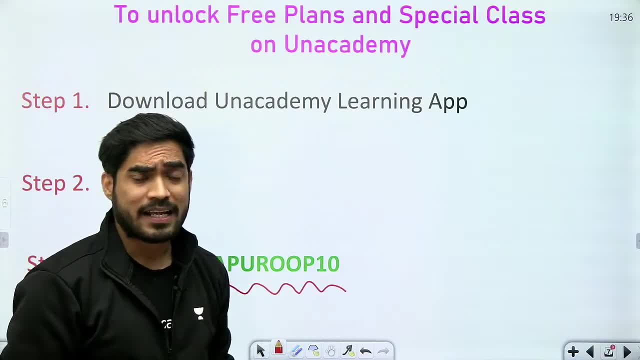 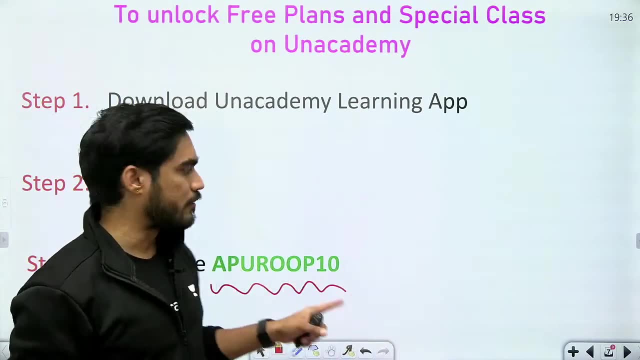 Your code is APPROVE10.. Use APPROVE10 invite code and all the special classes will be open. Not only mine, but every special class on Unacademy will be open for you, son, using this code: APPROVE10.. Okay. 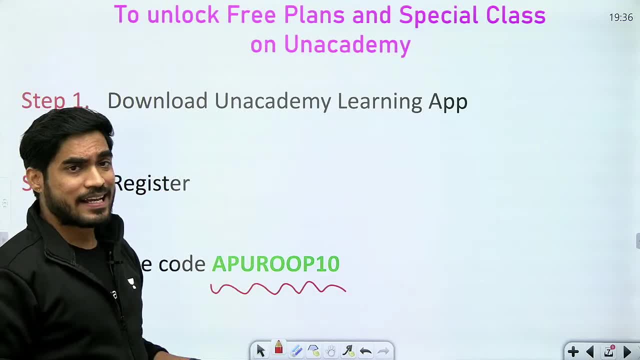 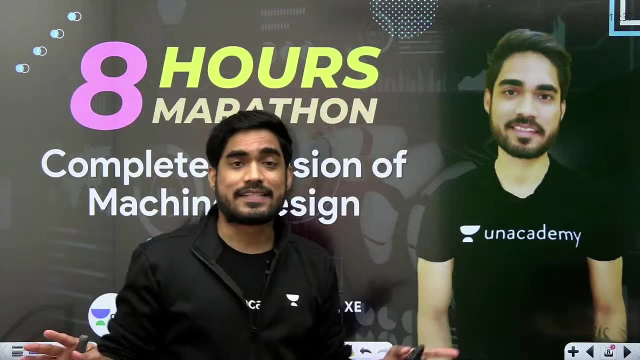 So don't forget to download the Unacademy learning app and use APPROVE10 in order to open all the special classes. Okay, And a very important news: Today we are completing the lecture series of machine design. We are completing the syllabus of machine design. 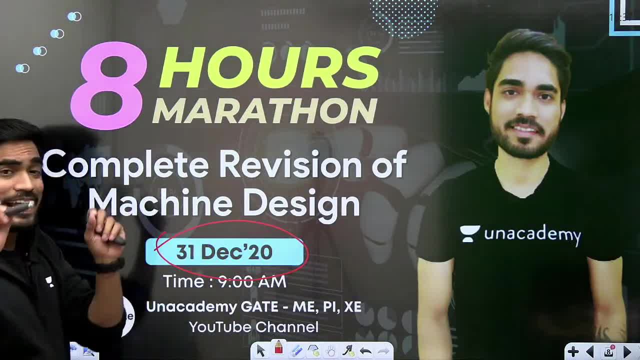 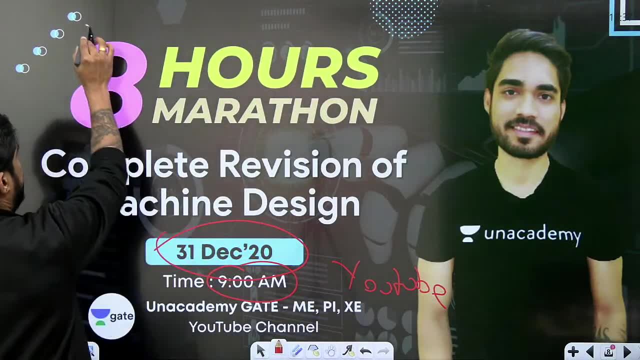 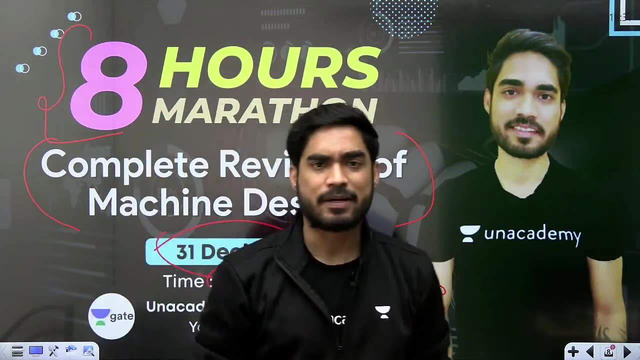 And tomorrow, 31st of December, the last day of the year, at 9 am on YouTube I will be taking 8 hours marathon class on the complete revision of machine design. So all the students who have watched my machine design lectures, all of you are invited to join me tomorrow. 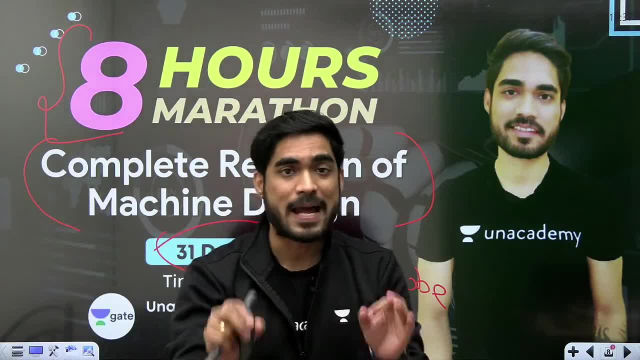 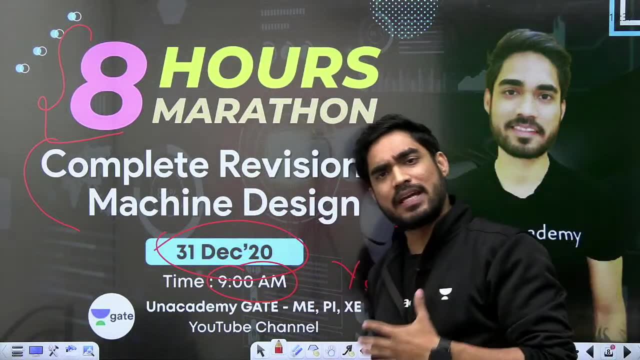 Okay, At 9 am Tomorrow morning, after taking a bath at 9 am, sit down, open your laptop, your phone and watch this marathon class with me. We will completely revise the entire machine design in one single class. 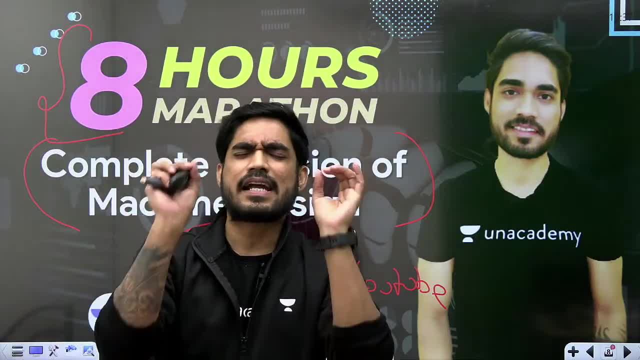 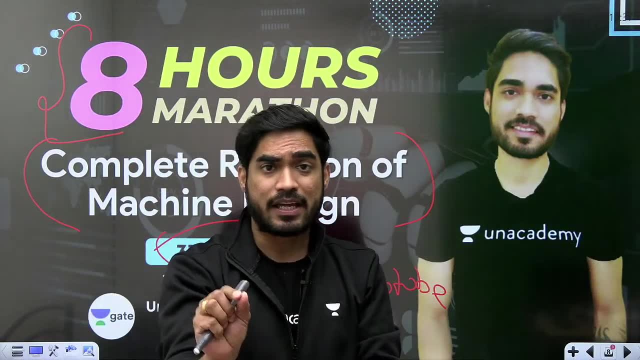 So dedicate one day of tomorrow and your machine design will be prepared in such a way that you won't need to open it again till the exam. I can guarantee that if you give me half of the day tomorrow, Half of your day, Half of your day tomorrow. 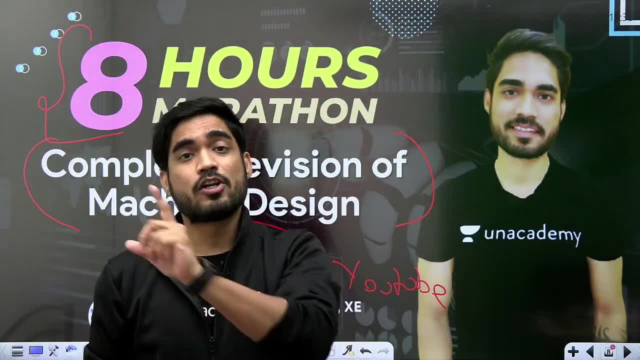 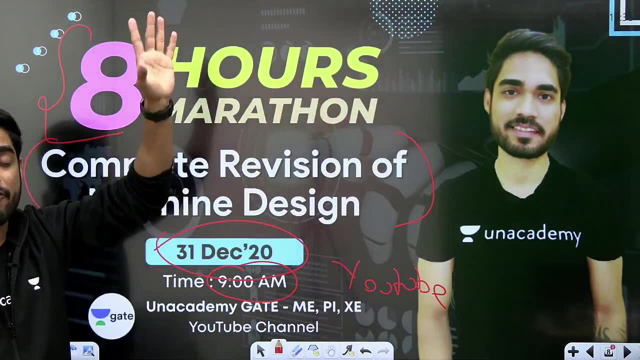 Then my son, your machine design will be completed in such a way that you will not even have to revise it until the last day of exam. Open the last day of machine design lecture and machine design notes And just go by looking at the formula once from there. 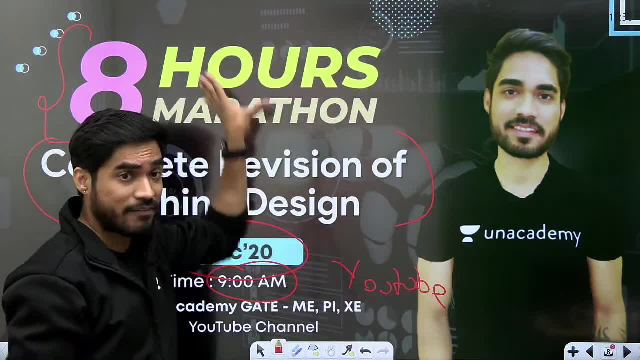 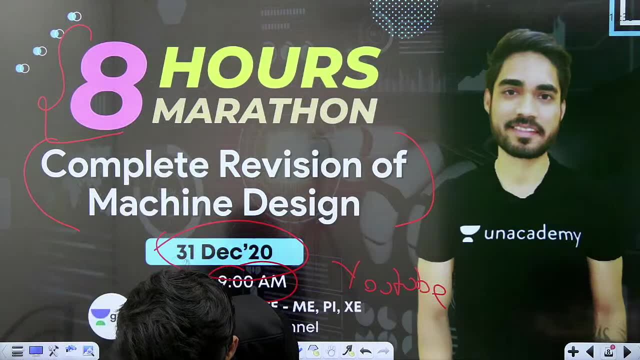 Before that, you won't need to look at machine design again. We will revise machine design in such a way. Okay, We are going to revise machine design in this way. We are going to make it. Yes. Thank you so much, Rishay. 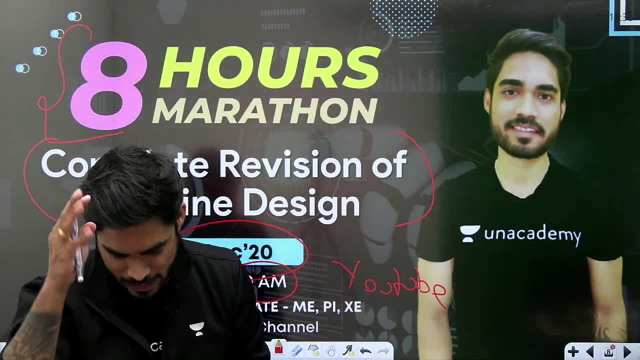 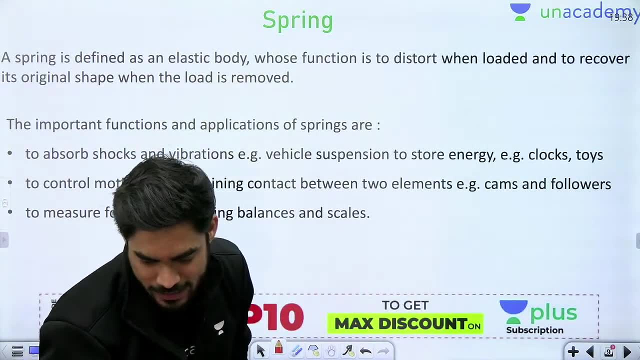 Good evening Akshay. Good evening, Good evening Adil. Good evening Jitendra. Good evening Vikas. Welcome everyone, Welcome. Welcome Welcome, My brother. it is spring lecture. It is spring lecture. 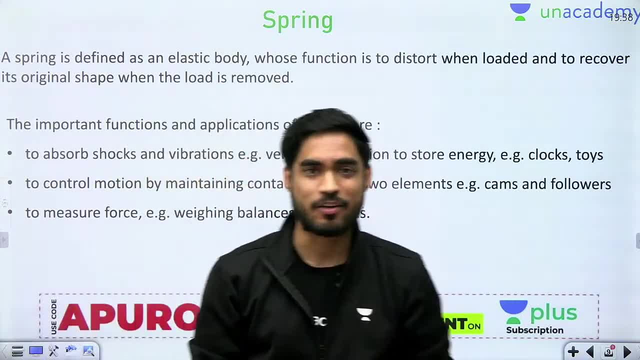 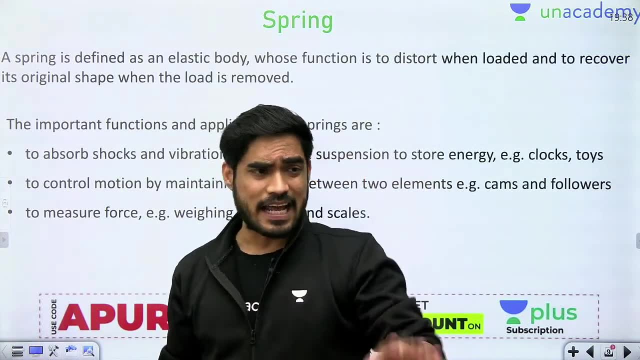 Okay, So let's start the lecture series. Okay, Let's start the lecture of spring. So this is the last class. Okay, And I have already told you so many times, If you are worried that I have not taken this topic, I have not taken this topic, then that is not in the syllabus of GATE. 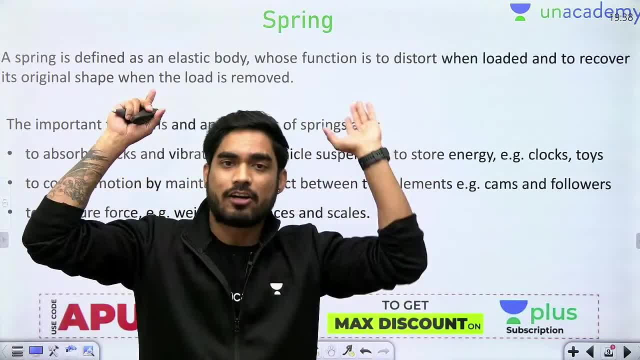 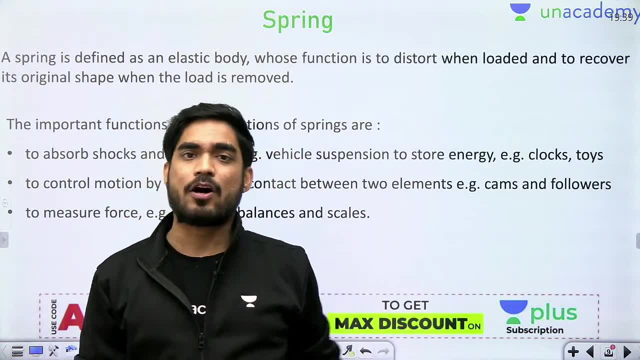 In the syllabus of GATE, Whatever it is. I have already taught all those things. Whatever was in the syllabus of GATE 2021, I have completed all those topics. So don't worry about the syllabus. Let me worry about the syllabus. 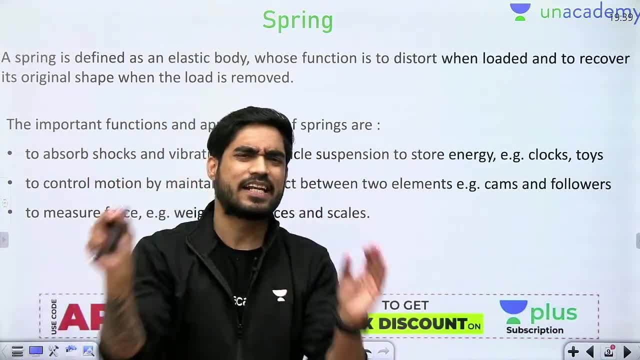 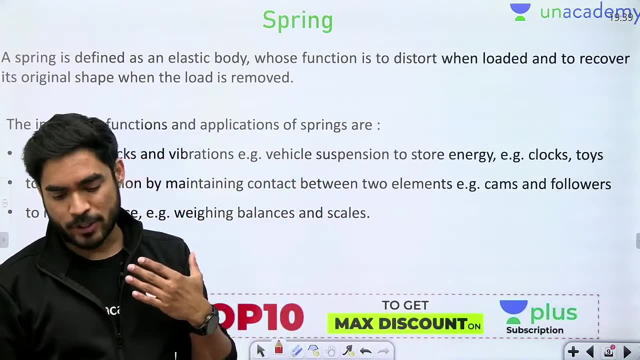 Let me worry about the syllabus. my brother, You just enjoy the lecture of BAT. You just read the lecture of BAT. Give your time, Work hard. That's it. Leave the worry of syllabus on me. Okay, Good evening, Ayush. 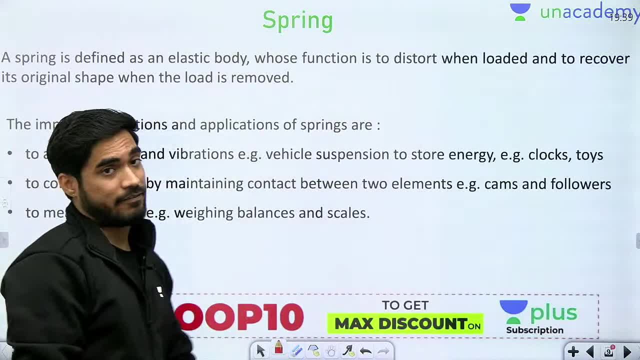 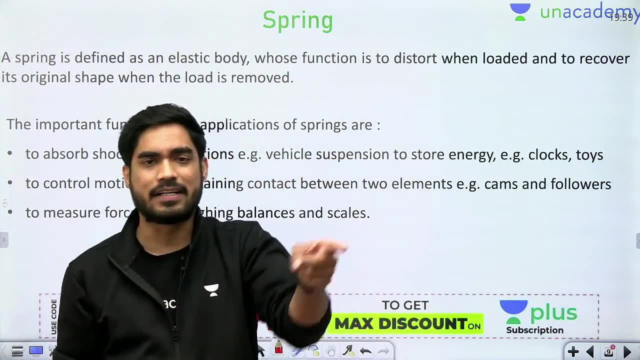 Good evening, Brijesh, Welcome, Welcome. So, my brother, let's start with the lecture of spring. So what is spring? Exactly what is spring? If I ask you what is spring, my brother, you can easily point it out. 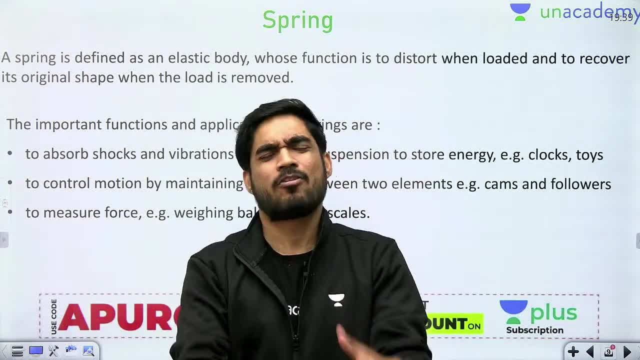 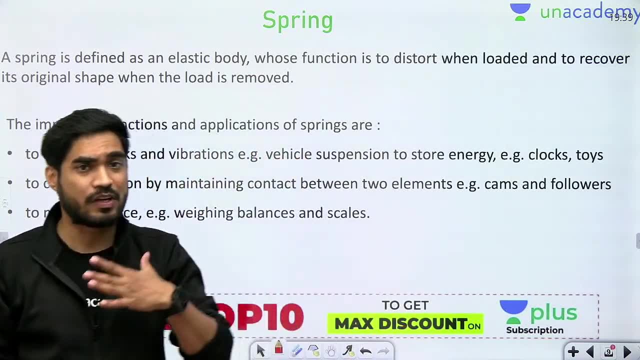 This is spring, This is spring. But, my brother, what exactly is the definition of spring? Not definition of spring, But what is so special about spring? What is so special about spring? So, my brother, there is one characteristic which we need, which we expect from spring: 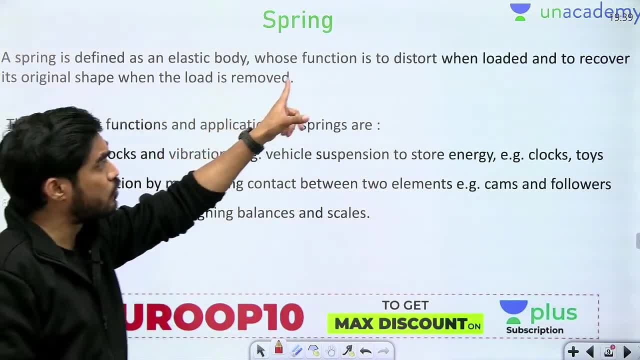 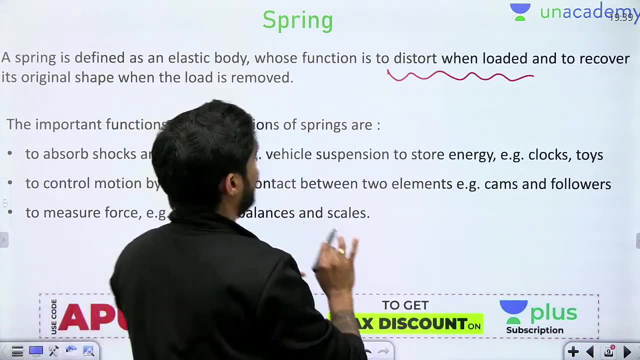 Okay, And what is that? Spring is defined as an elastic body whose function, the main function, is to distort when loaded and to recover its original shape when load is removed. So basically, we use spring so that it is distorted, deflected. okay. 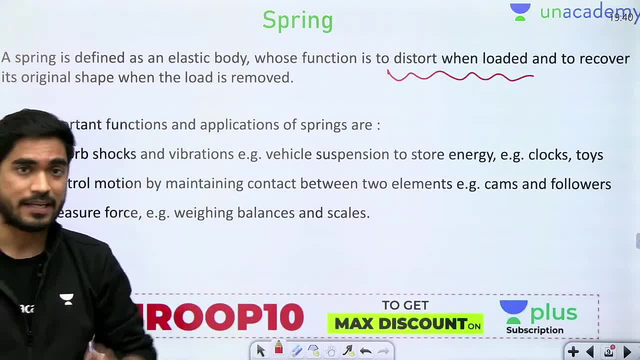 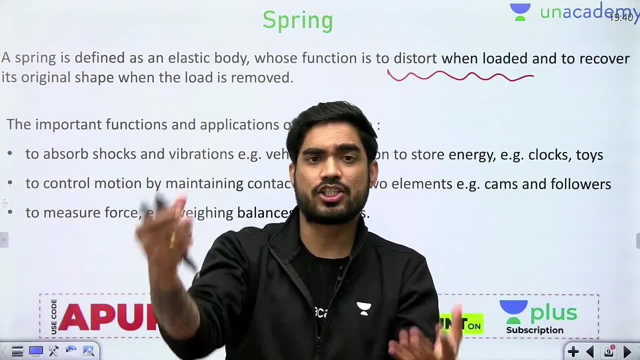 This is the special characteristic of spring which makes it so special. okay, Why is spring special? Why is spring important? Because it can deflect when loaded and it will regain its original shape and size when unloaded. That's why the spring is so important. 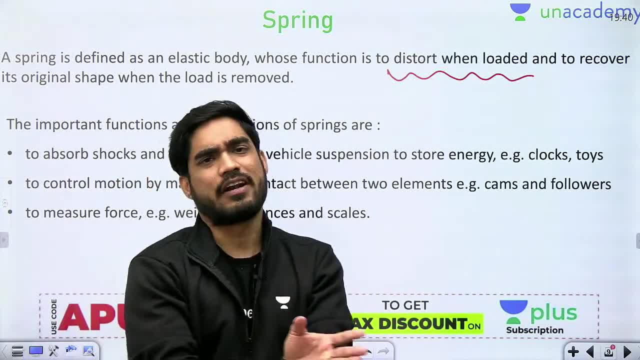 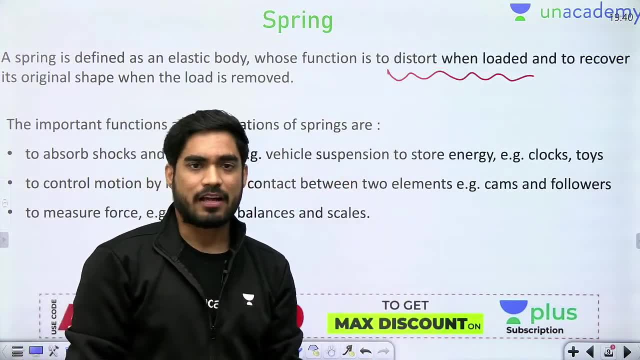 Now my son. in different applications we use this characteristic differently. In different applications we use this characteristic in different ways. Okay, In some applications we use it to store energy. In some applications, we use it as a support system. 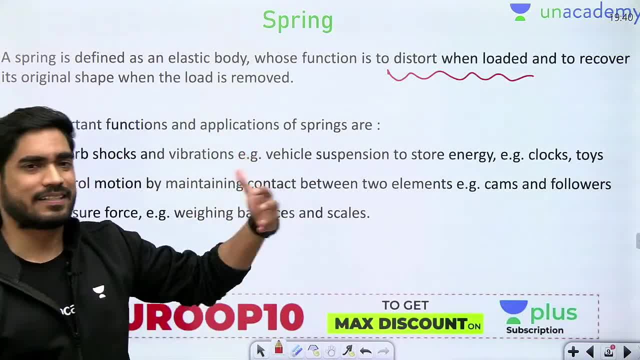 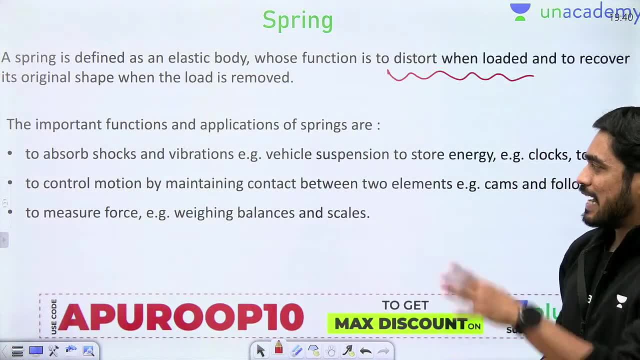 So my son, in different applications the use of this characteristic of spring is different. Okay, In different applications the use of this characteristic is different. Okay, So my son understand how it can be used in different applications, Okay. 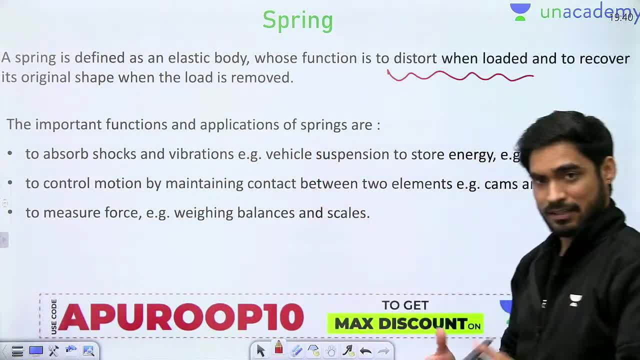 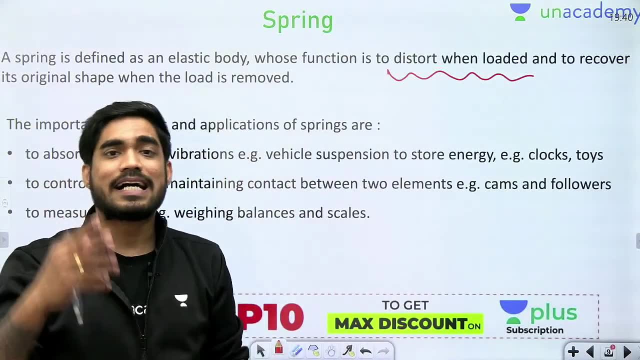 The first application is to absorb shocks and vibration Means. it is like a support system. It is absorbing the shock and vibration So that it is not transferred to other machine elements. This spring absorbs the shock and vibration in such a way that it is not transferred to other elements. 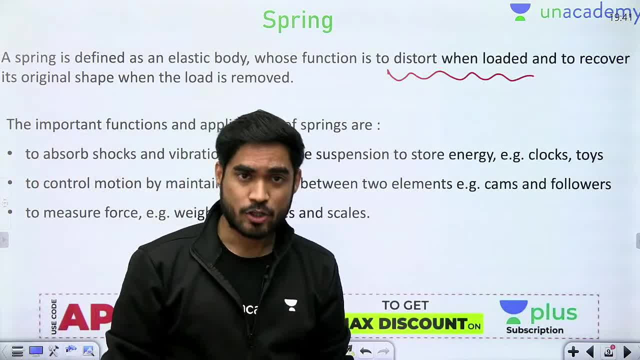 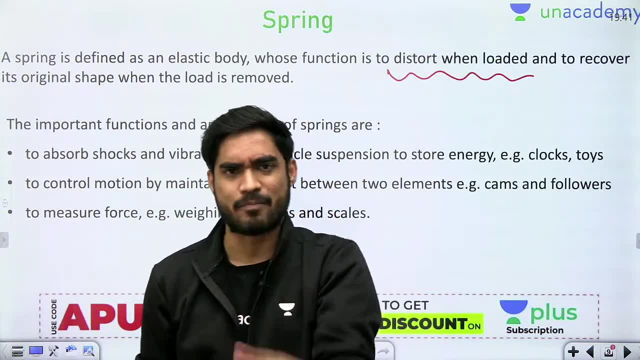 Okay, For example, your suspension system of vehicle. You might have seen a mono spring in your bikes. Nowadays there is a mono spring in bike. Mono spring means a single helical spring in bike, So that is used to absorb the shock and vibration. 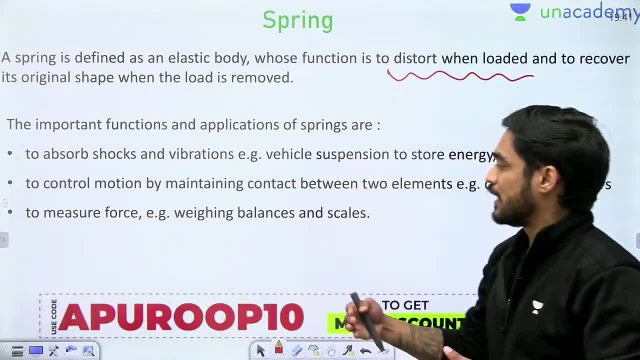 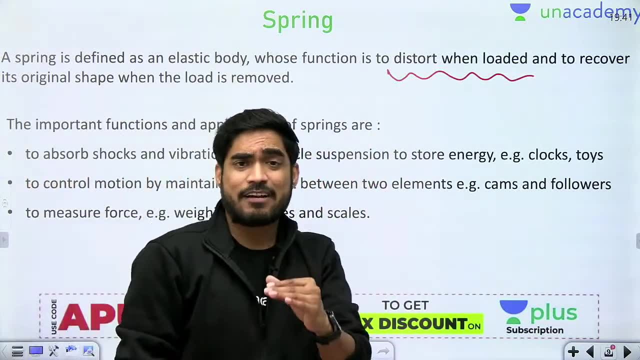 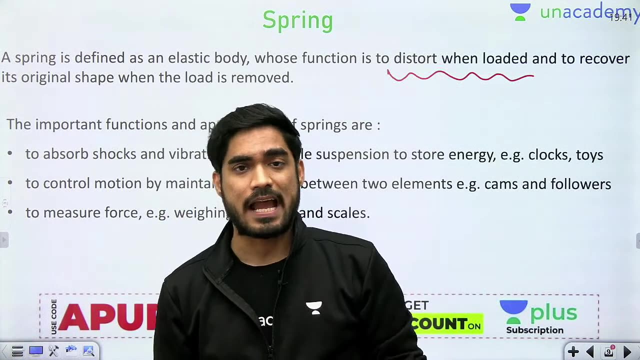 The second application is to control. Control the motion by maintaining the contact between two elements, such as cams and follower. Okay, So cam and follower may, if you want the follower to always. sorry, if you want a follower to always be in contact with the cam. 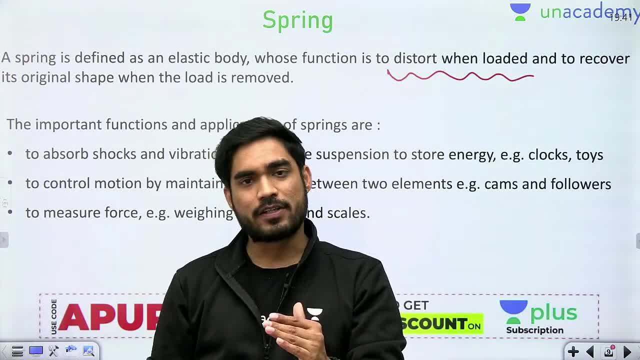 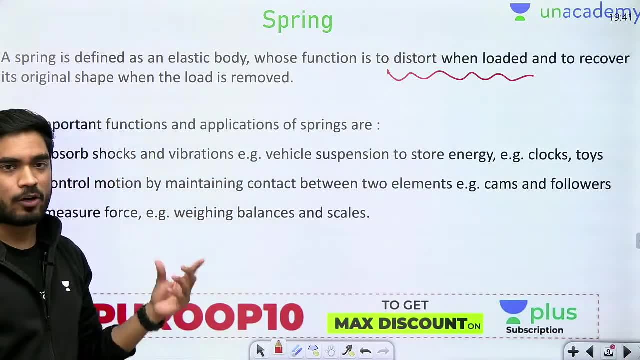 then, my son, you support it with a spring, Due to the spring force, the cam is always in contact with the follower. Okay, So, my son, it is used in cam and follower in order to keep them in contact with each other throughout. 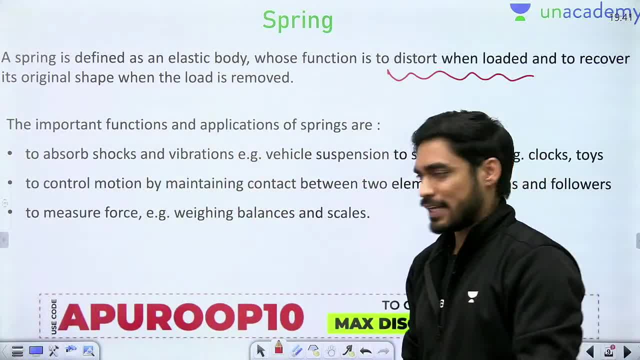 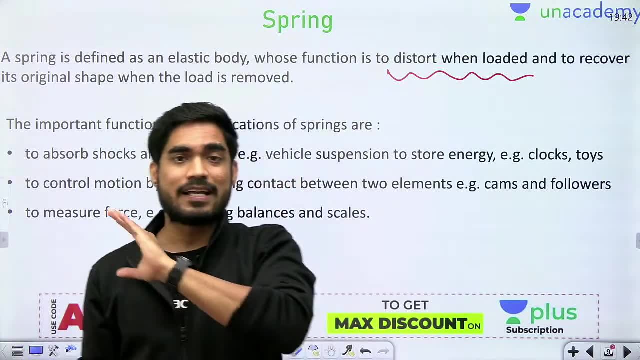 Okay, Okay, Okay, Okay. So the third application is to measure the force, For example, weighing, balances and scales. You have seen the scale, Okay, In that also, we use spring, Okay, So, my son, spring has different applications. 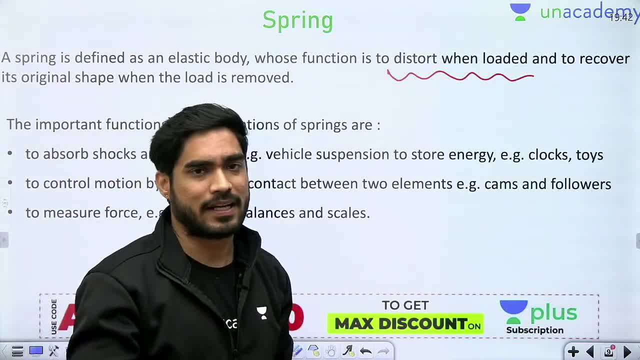 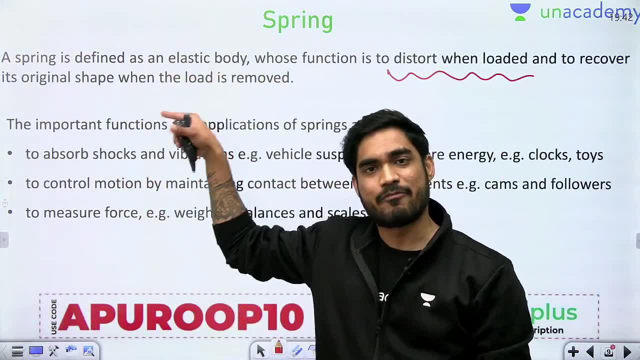 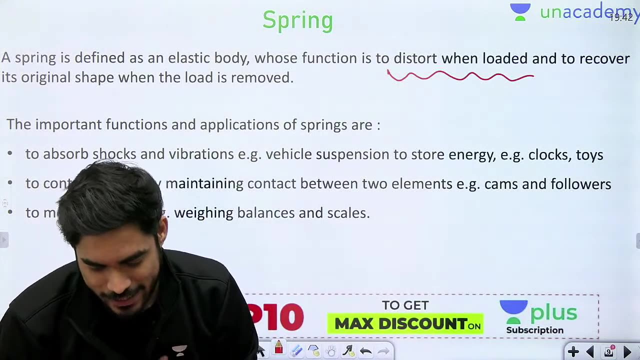 But in every application the important feature of spring is the function of spring is to distort when loaded and to regain its shape when unloaded. That is the important characteristic of spring, which makes it so special. Okay, Thank you so much, Adil, thank you so much. 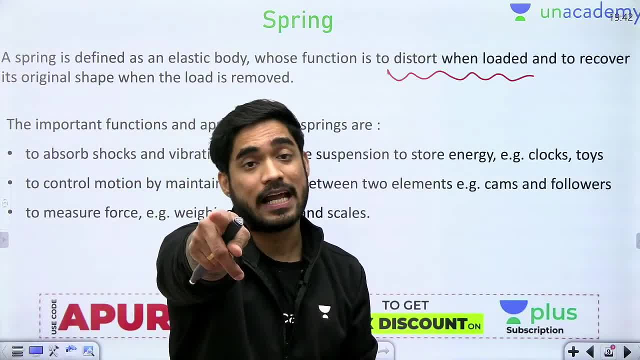 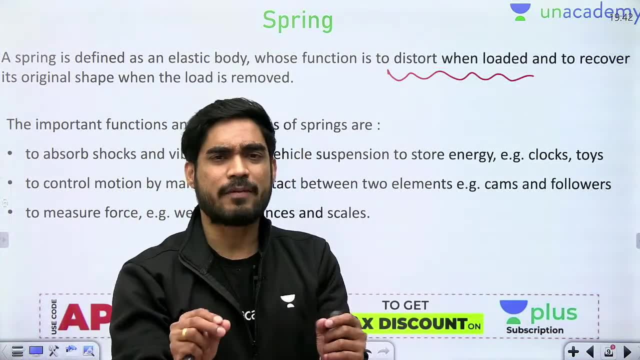 Adil for such a compliment. Son, please don't forget to hit the like button. Everyone press the like button and then watch the lecture. my brother, If you like my lecture, then hit the like button. And, son, this is the last class. 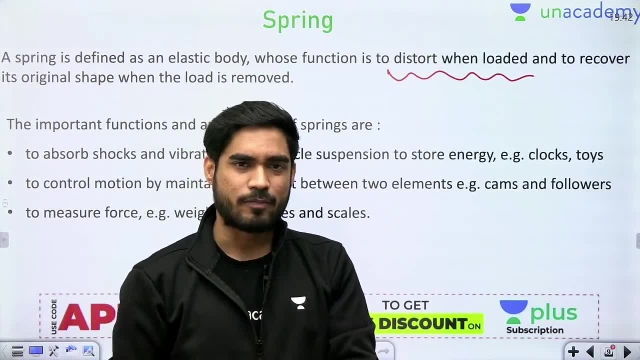 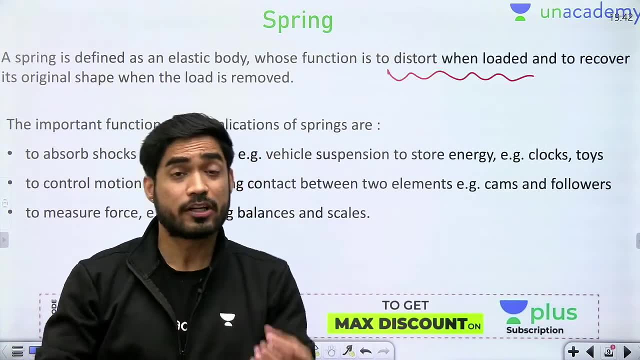 So what I expect from all of you is: if you like something about my lecture, please write it down in the comments. If you don't like something about it, something about the lectures, then also please write it down. Whatever you want to say, whatever you want to tell me, you can write that down in the comment box. 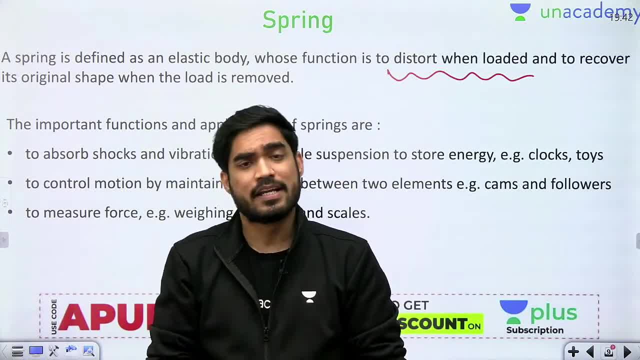 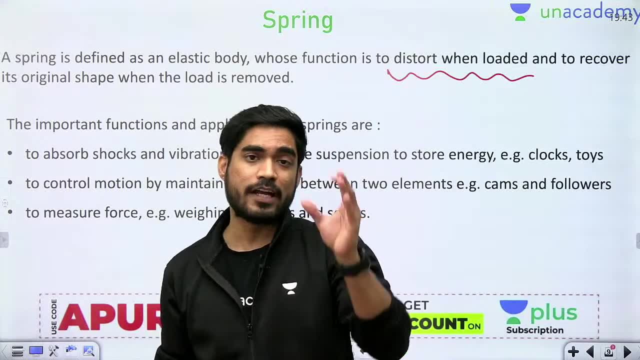 Okay, What you like, what you dislike, what improvements you want, all of that you can write in the comment box. Son, I really love reading the comments. I really love following whatever you are saying. Okay, I follow all things. I read all things. 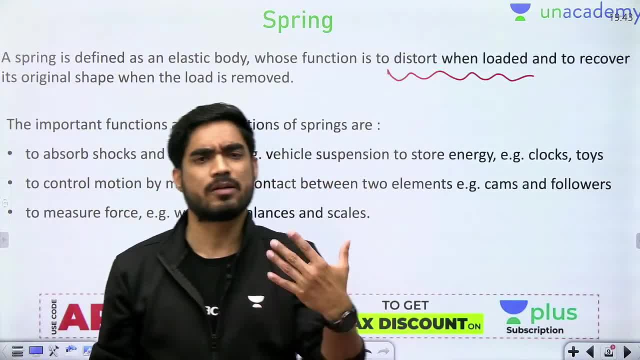 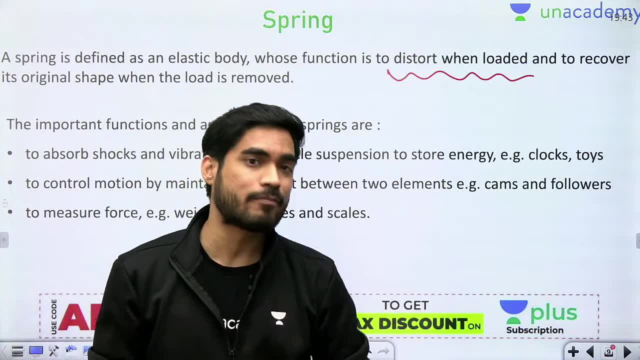 What you are writing in the comments. you are writing good, you are writing bad. something is bad, something can be improved, So I also try to improve on that. So I will keep on updating myself. I will keep on improving myself in order to do better and better here. 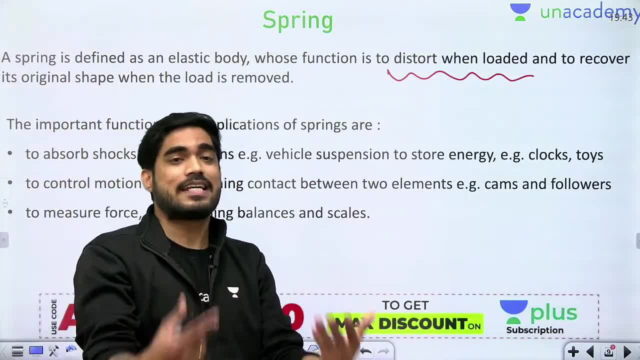 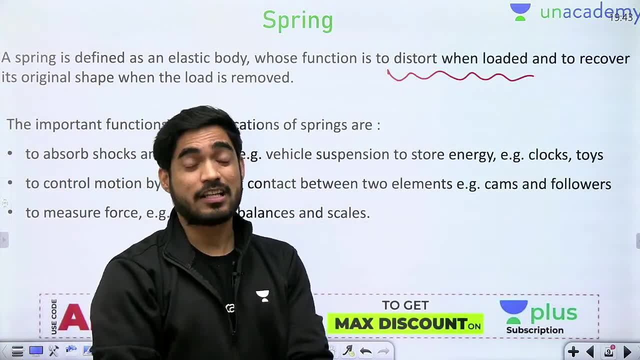 Whenever I come in front of you, I will improve myself. So I will study well, I will deliver good content, I will deliver it in a good way. that's all I want, Okay. So, son, whatever you like, please write it down in the comments, not only in the live chat, because, son, sometimes I skip the live chat. 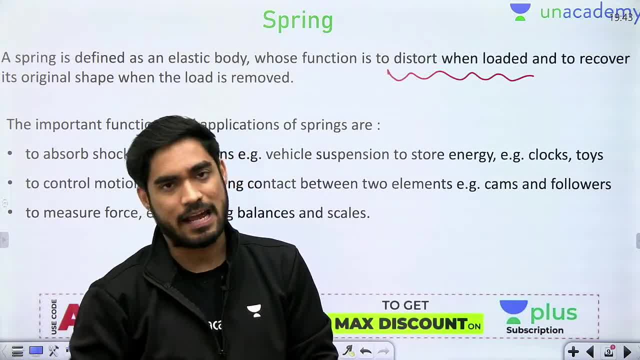 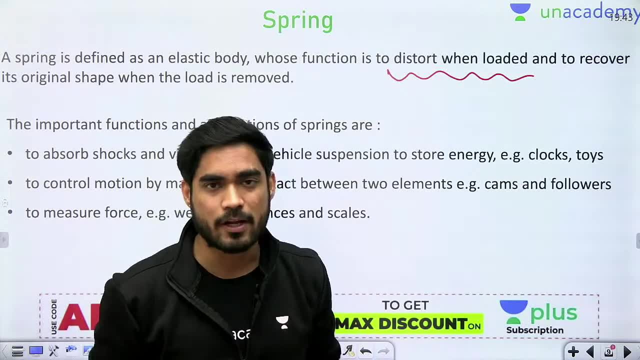 Sometimes I am not able to read each and everything you write in the live chat. but, son, in the comments box, whatever you write, that will stay permanently. After the lecture ends, the live chat will be gone, but the comments will always stay there. 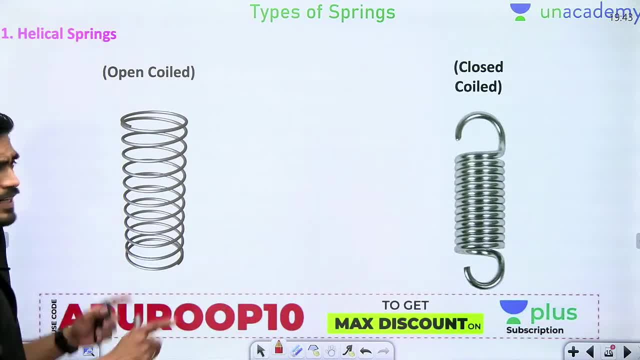 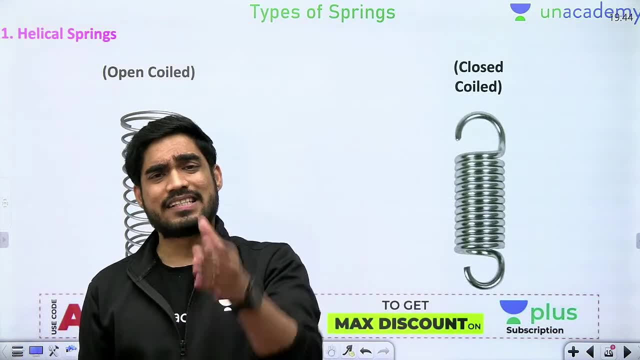 Okay, Thank you so much. Thank you so much. Okay Now, son, there are different types of spring used under different application, and what is the difference? exactly? The difference is the type of load. Okay, There is a difference in load in every spring. 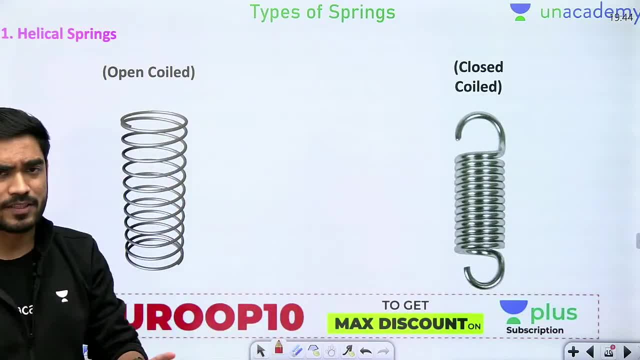 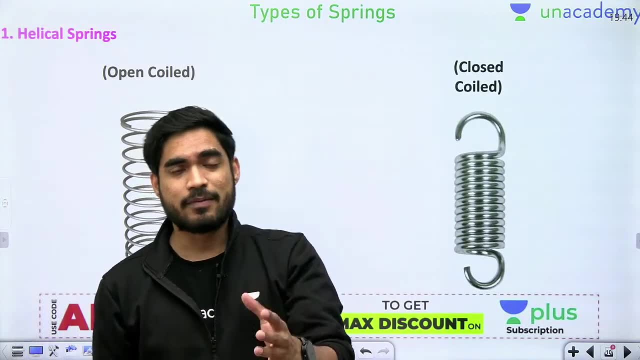 Okay, The difference is in the load, Son, according to the load, if you compare, if you categorize- sorry, if you categorize the spring, then, son, the first category is helical spring. Now, what do we mean by helical spring? 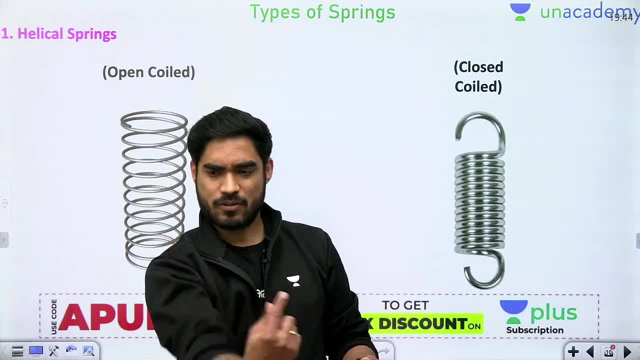 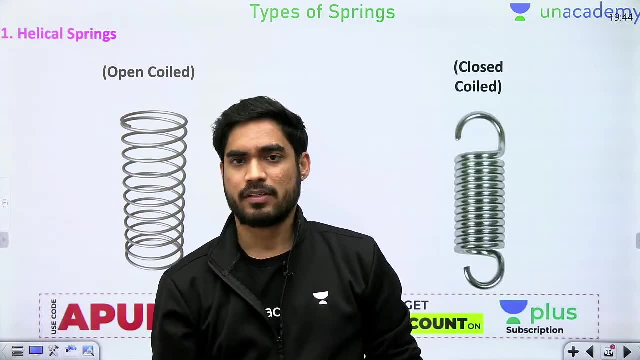 What does helical mean? What does helix mean? This is helical. okay, This is helical. So let's say, you have a metal wire, long metal wire, and you have turned it into helical form, so then you get a helical spring. okay. 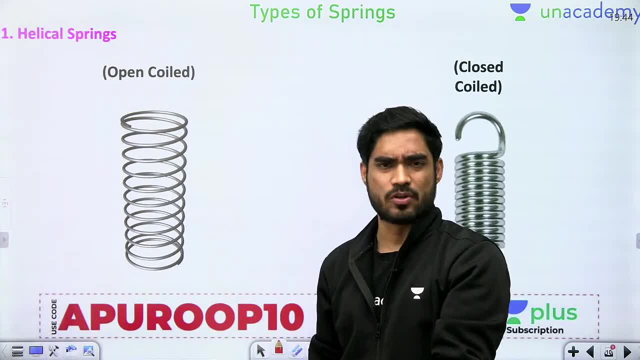 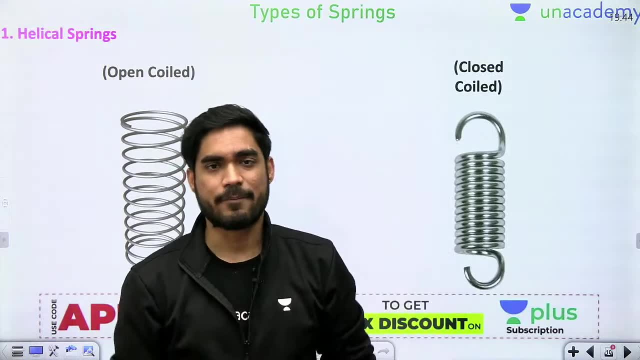 Practically lot of times. you see helical springs only In suspensions. you see helical spring in pen. you see helical spring in weighing machine. you see helical spring okay, So son, in helical spring also there are two types: open coiled and closed coiled. 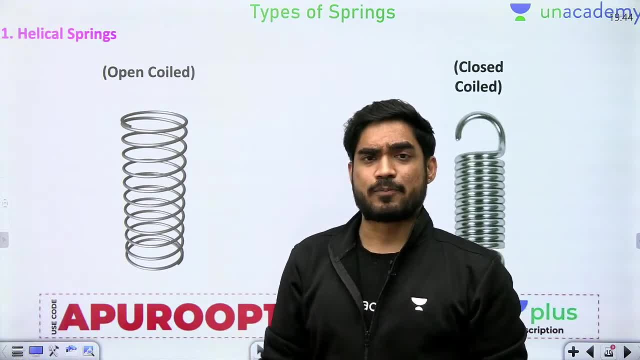 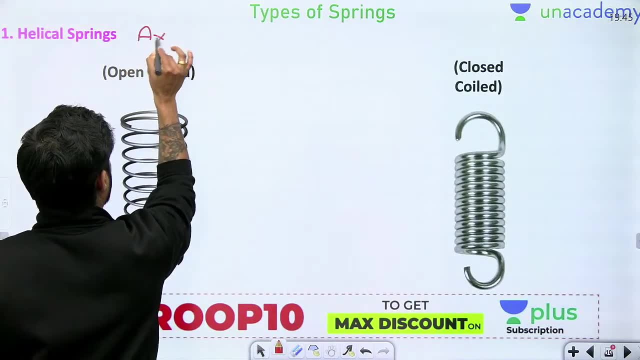 So understand the difference between them. Helical springs are used to sustain axial load. Helical springs who are? they used to sustain, my brother, Axial loads. Okay, How does load look in helical spring? Axial load. 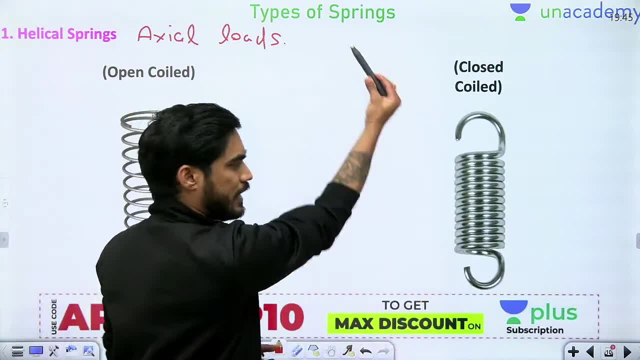 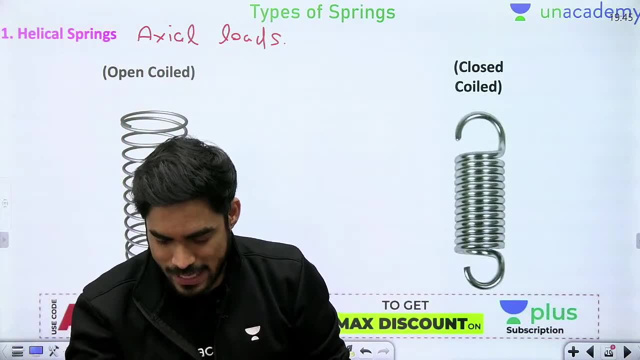 What do we mean by axial load? This is the axis of the spring: right Vertical axis. This is the axle of the spring. So if the load is applied in the direction of the axis, if the load is applied in the direction of the axis, 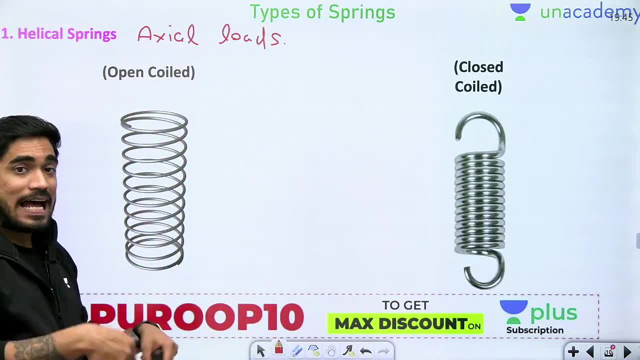 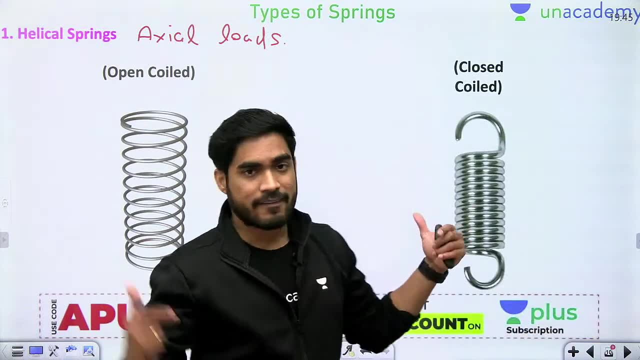 then it is known as Axial load. Now, axial loads are of two types: tensile and compressive. So can you tell me, just by looking at the springs, which one will be able to sustain tensile load and which one will be able to sustain compressive load? 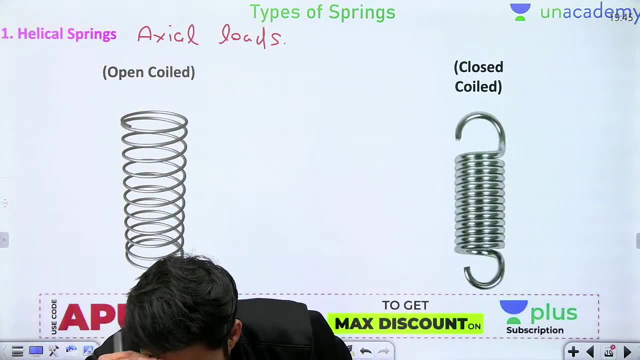 Can you tell me? Thank you so much, Gopalakrishna. Thank you so much, son. Thank you so much. That is such a great compliment. Thank you so much. Thank you so much, Ayush. Thank you so much, Vikas. 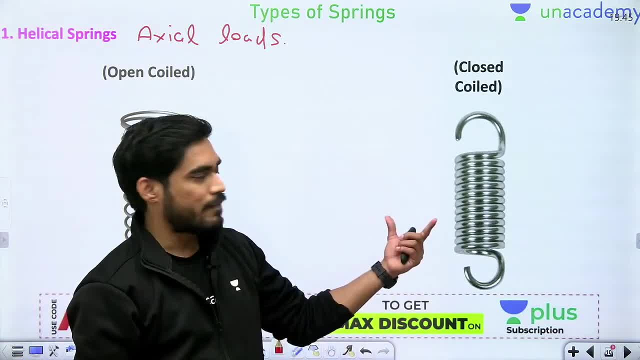 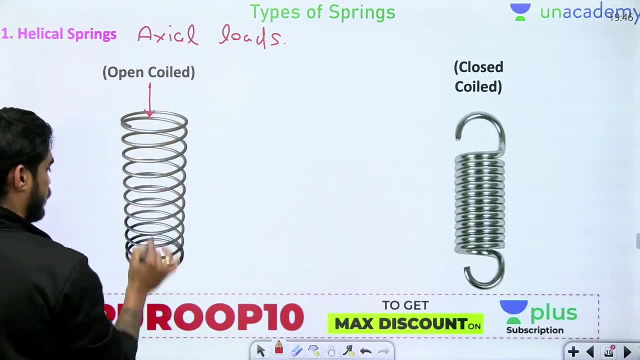 Thank you so much, son. Thank you so much. Thank you so much. Okay. So, my brother, by looking at it, you must be able to understand that this will be able to sustain compressive loads, because there is a scope of compression here. 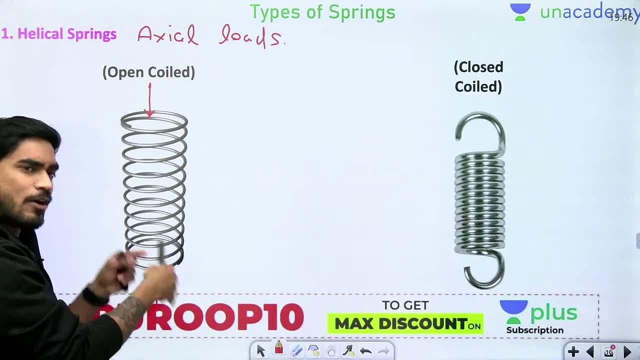 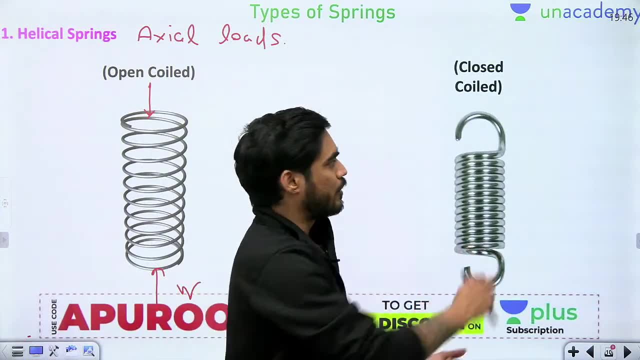 It can also sustain tensile load, Not only compressive load, it can also sustain tensile load. But especially, it is used in compressive load. Okay, But this cannot be compressed because there is no gap. Can you see? 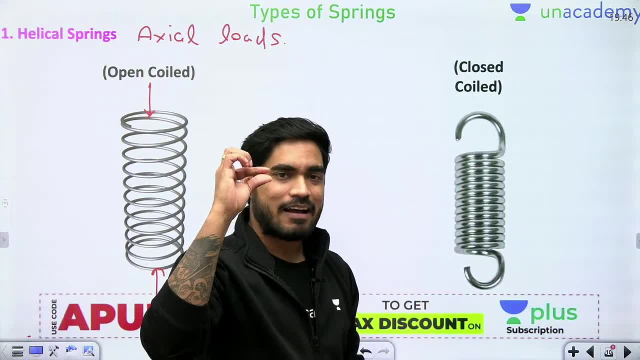 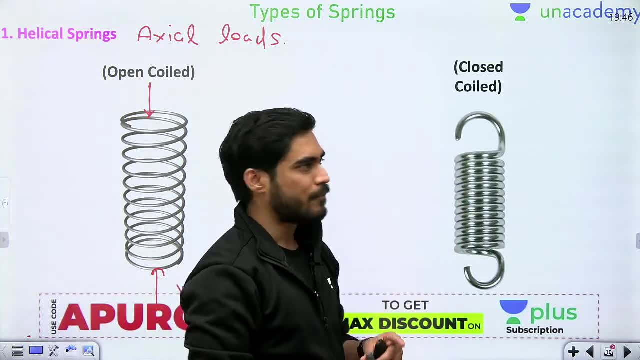 There is no gap. The coils are at very negligible. The coils are at very negligible distance from each other. The coils are not separated, They are very close to each other. So this will be able to sustain only tensile load Okay. 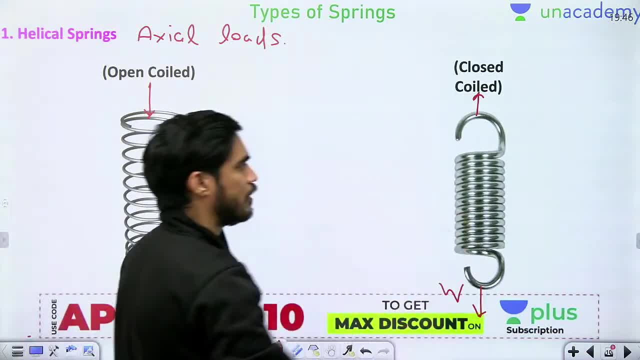 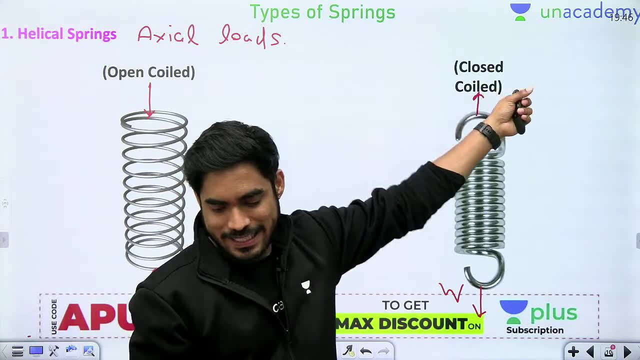 This will be able to sustain compressive load and this will be able to sustain tensile load. That's why this is also known as compression spring and this is also known as tension spring. This is called compression spring and this is called tension spring. 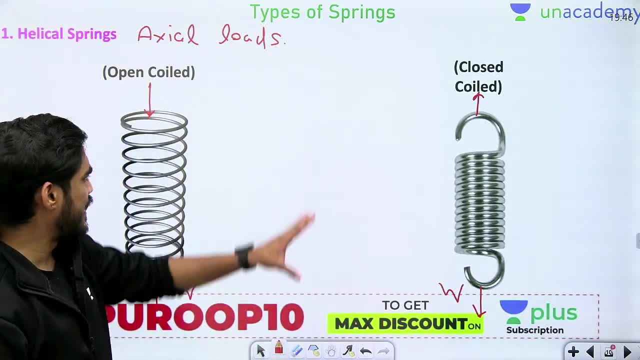 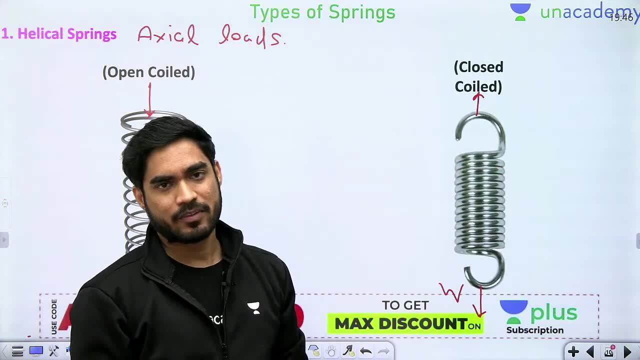 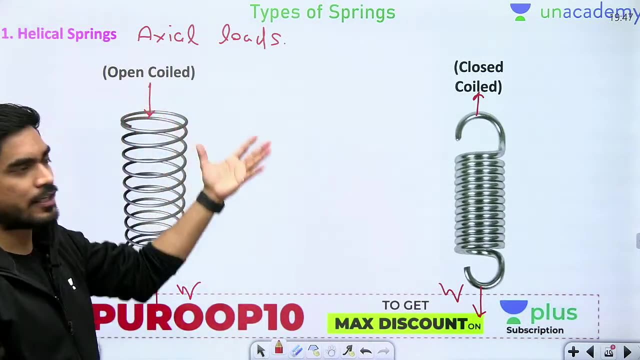 Now, my brother, you must be thinking: okay, this is a compression spring, this is a tension spring, But why do we need to use these two springs separately? Why can't we just call them coil spring? Why don't you just call them coil spring or helical spring? 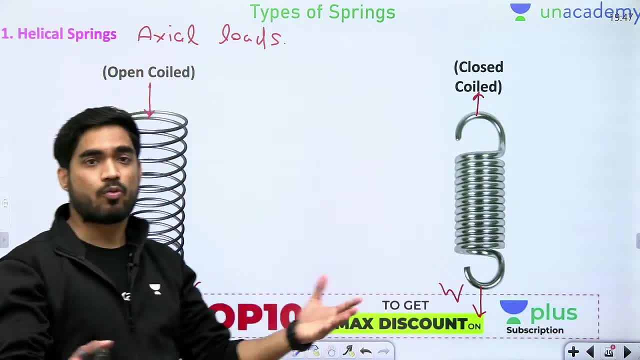 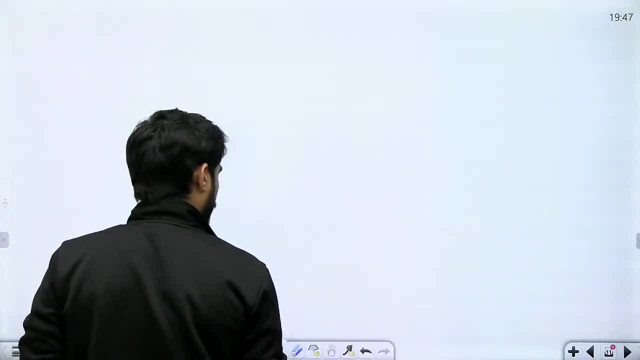 Why closed coil helical spring, open coil helical spring? Why? What is the difference in their analysis? What is the difference in their design? So understand my brother, Understand the difference in their design. Okay, Okay, First of all, 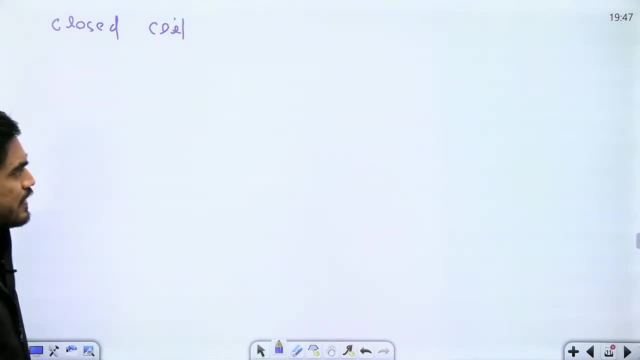 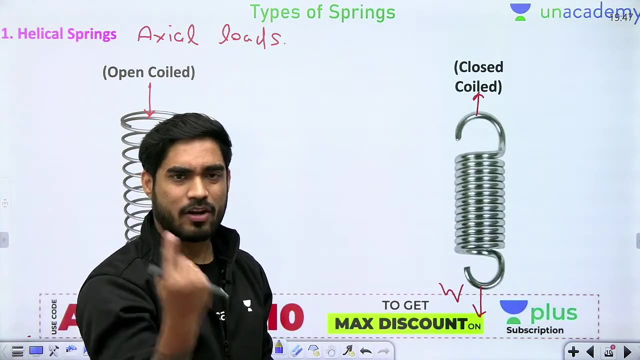 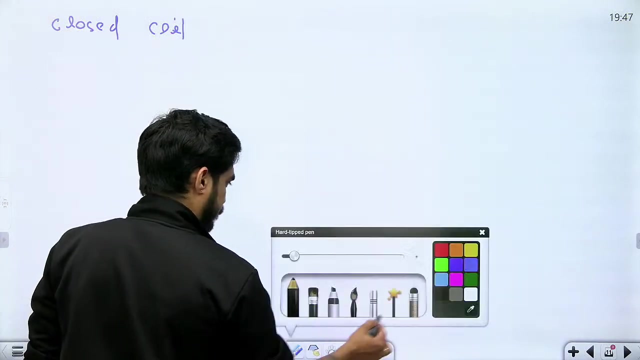 I will talk about closed coil helical spring. Okay, So in case of closed coil helical spring, the coils are at negligible distance from each other. Okay, The number of turns: different turns of coil are at very close distance. So, my brother here, I can say that the turns are almost horizontal. 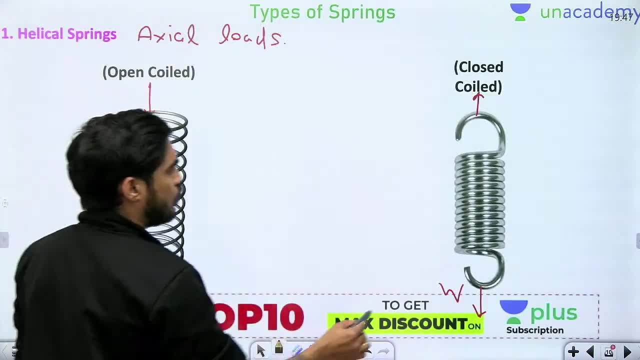 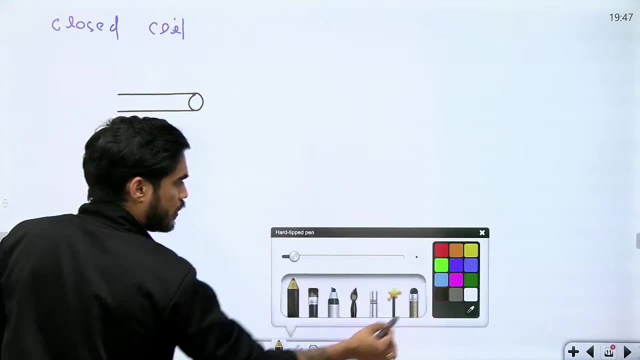 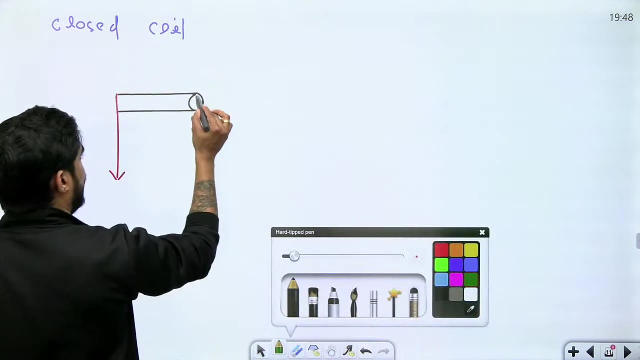 Okay, These turns are almost horizontal. Now the load is passing through the center. So let's say this is half of the half of the turn. So the load is passing like this. Okay, Now can you see, this load is exactly parallel to this cross section, almost almost parallel. 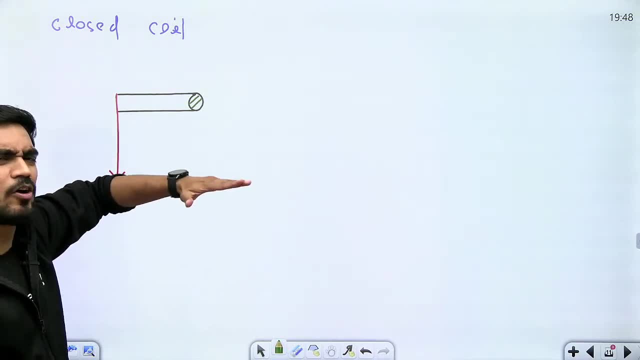 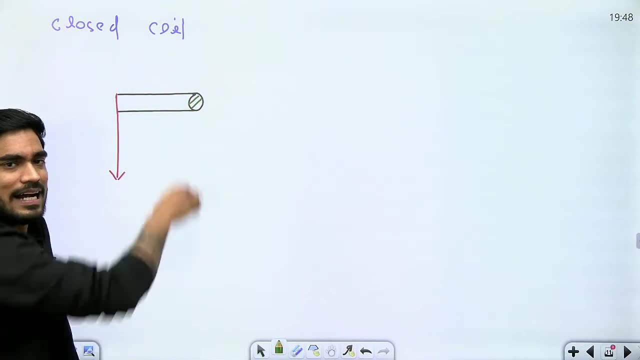 Okay, Because, my brother, it will not be exactly horizontal, it will be almost horizontal. So this load is almost parallel to the cross section. So, due to this load, there will be a direct parallel force on the cross section. 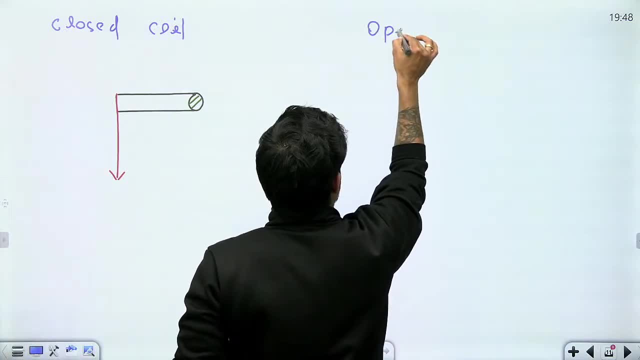 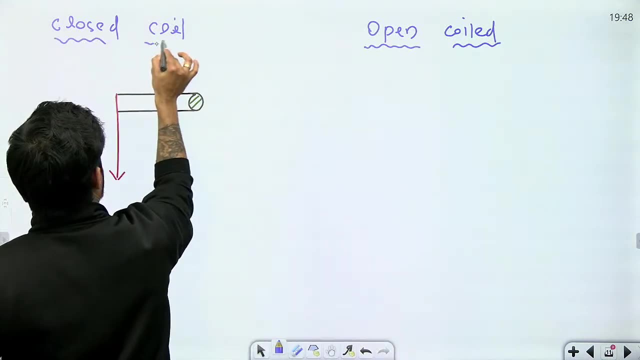 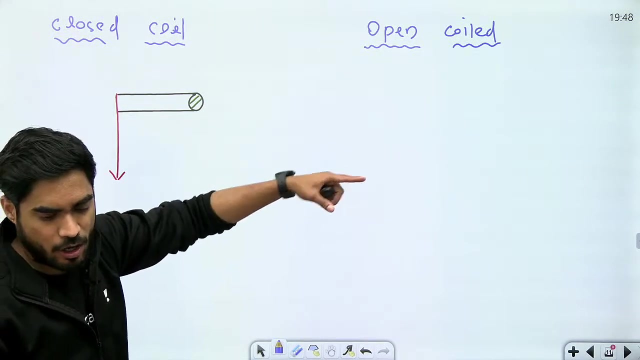 But, my brother, if you see open coil helical spring in open coil helical spring, you cannot assume that. you cannot assume that the turns are almost horizontal, You cannot assume that the spring is almost horizontal. The spring will be like this at some angle. 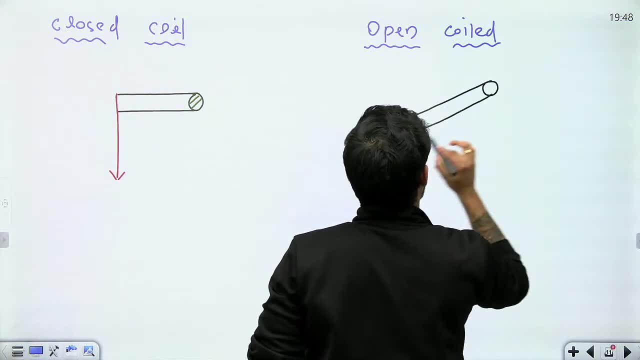 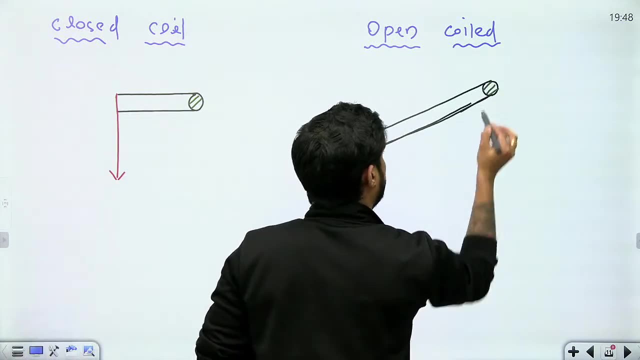 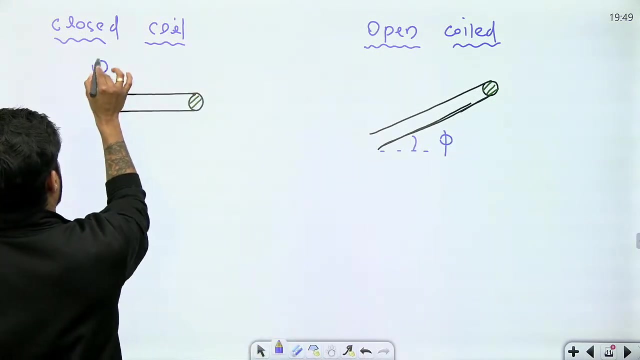 It also stays at an angle, But the angle in this is very small. Okay, Now, I will tell you, Now, I will tell you, Now, I will tell you how much angle is there exactly. Okay, So, my brother, the angle, this angle, this angle, which can be known as phi, it is less or equal to 10 degree in closed coil. 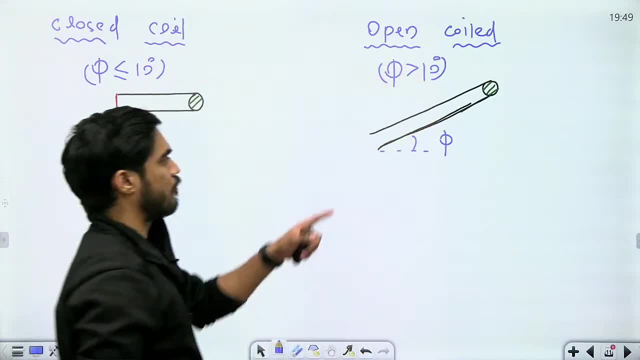 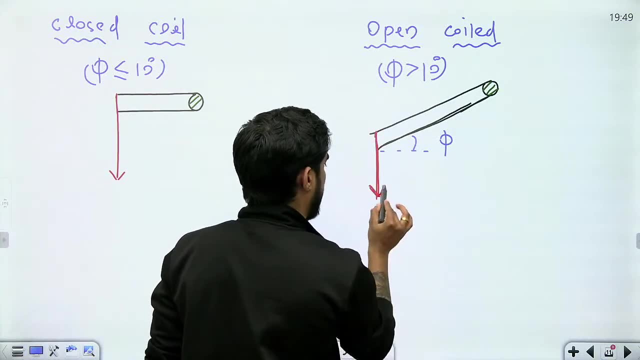 But phi is greater than 10 degree. in open coil, Phi is known as helix angle. Now, my brother, the load is acting like this. Let's say the load is acting like this. Okay, So can you see that? 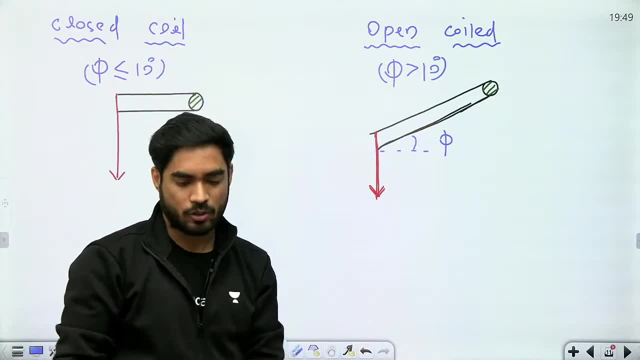 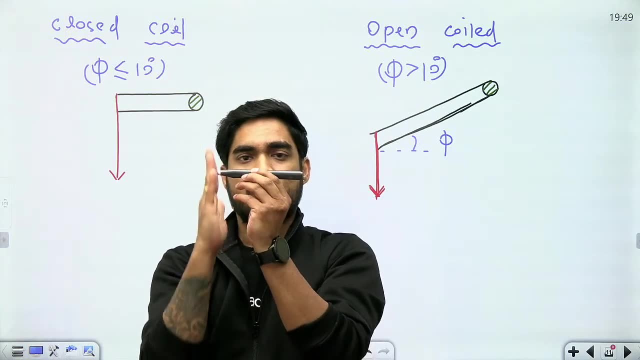 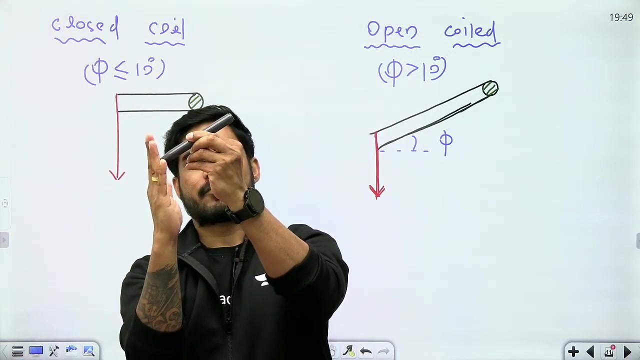 But the cross section is not exactly parallel to the load. The load is so sorry. the load is acting like this. In case of closed coil, your cross section is like this: Okay, Can you see. But if I turn this, then the load is acting like this, but my cross section is inclined. 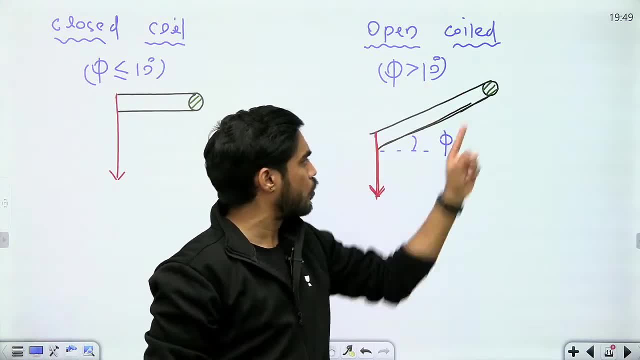 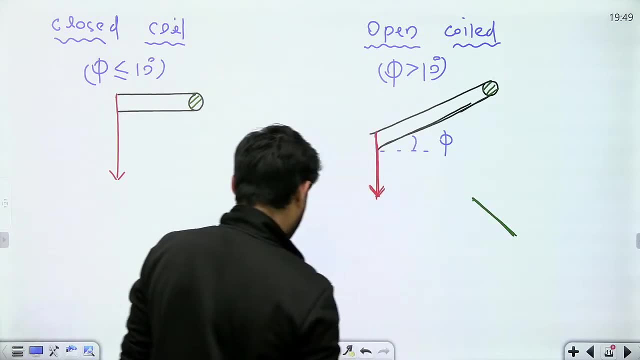 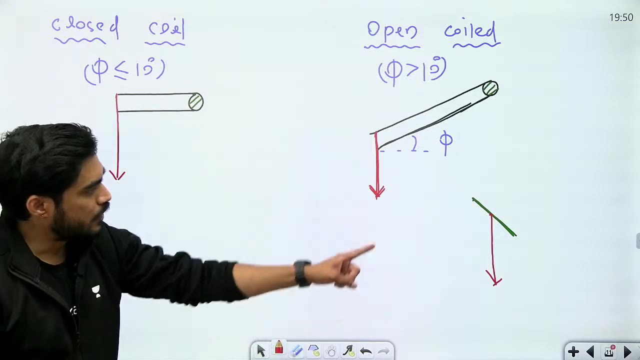 Okay, If I transfer the load exactly on this cross section, then you will get to see something like this: Okay, This is the cross section, This is the cross section, And if I transfer this force here, then this will be the force which will neither be parallel nor be sorry- which will neither be parallel nor be perpendicular. 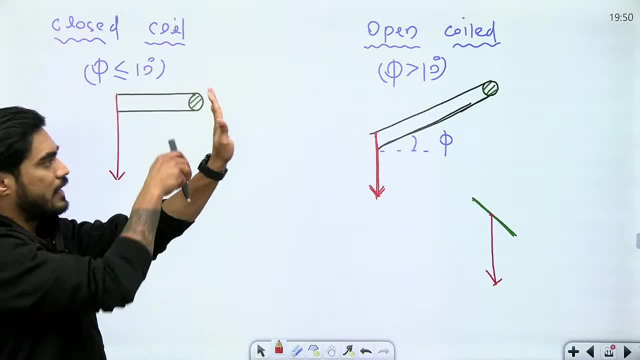 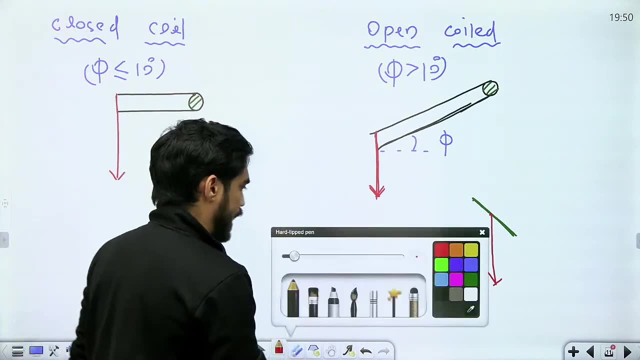 This is neither parallel nor perpendicular. Here it is exactly parallel. The load is like this, cross section is like this, But here it is like this. Okay, So, my brother, if you calculate the stresses here, then you will get to see something like this: You will have to resolve this force like this. Okay, You will have to resolve it like this. So that is the difference between closed coil and open coil. In closed coil helical spring, the force can be assumed parallel to the cross section. 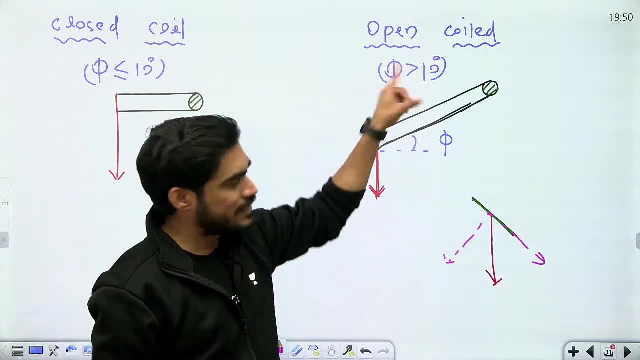 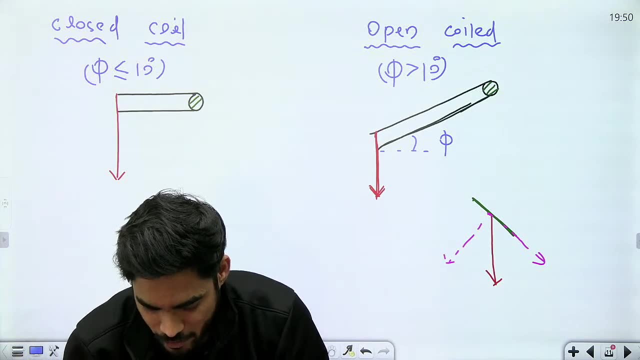 But in open coil. you can't assume that because this angle is greater than 10 degree. Okay, This angle is greater than 10 degree. Okay, Is it clear? Good evening, Parth. Good evening. Good evening. Good evening, Dibyanshu. 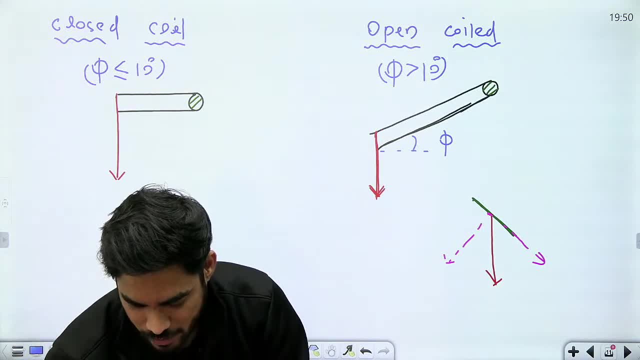 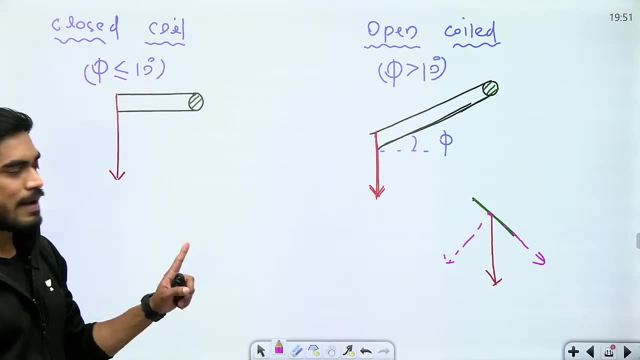 Good evening. Thank you so much. Thank you so much, Prem. Thank you so much, Ankur. Thank you so much. Love you all. Love you all. Thank you so much, Kalpesh. Thank you so much. So, my brother, is this thing clear? 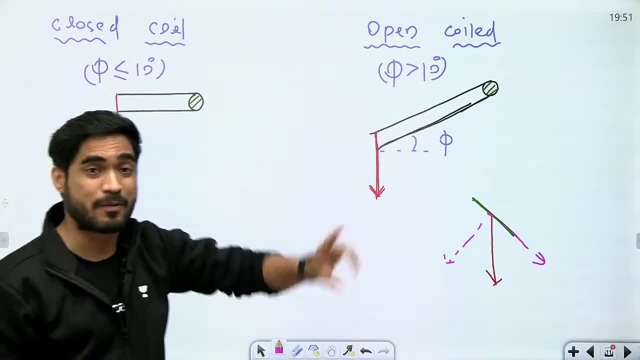 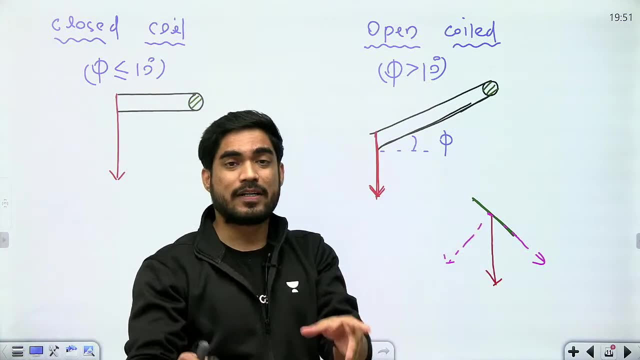 Is this thing clear? What is the difference between closed coil helical spring and open coil helical spring from the point of view of design? Now you don't have to worry about open coil helical spring, Because in our syllabus we don't need to deal with open coil helical spring. 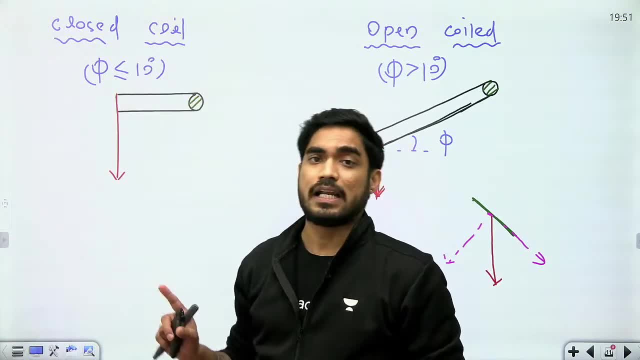 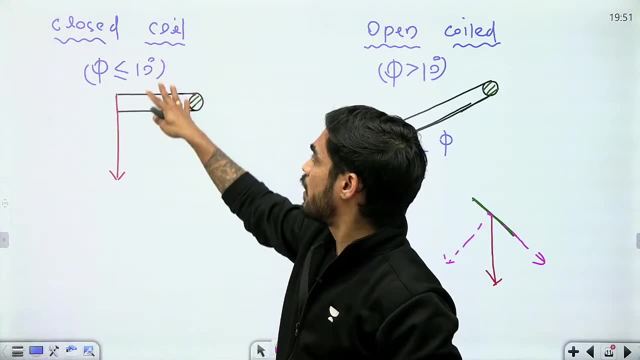 Okay, In our syllabus we only need to deal with closed coil helical spring. You don't have to deal with open coil helical spring at all. Okay, Don't worry about open coil helical spring, Only focus on closed coil helical spring. 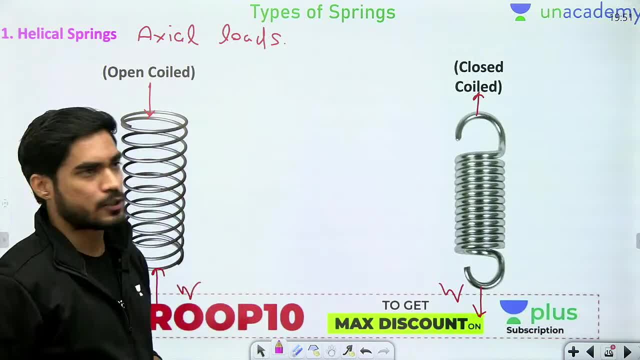 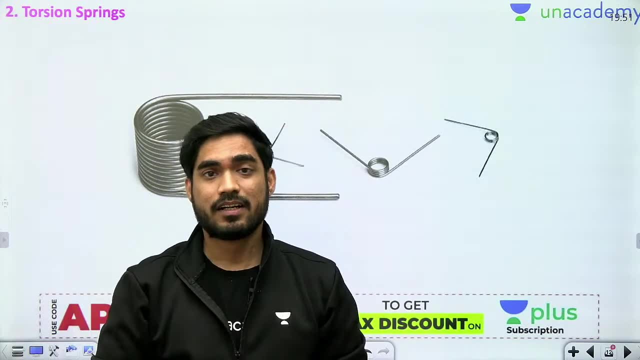 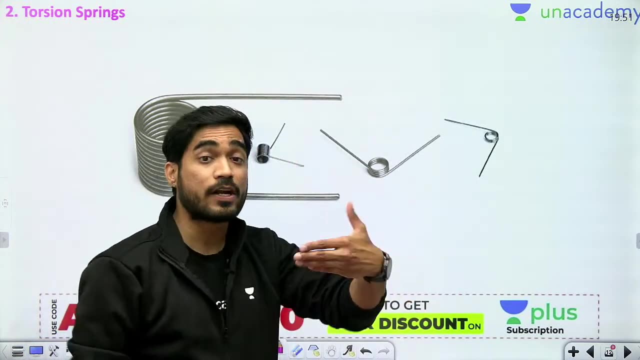 Okay. So my dear is this clear: The first type of spring, helical spring. Next is torsional spring. Now, my dear torsional spring, you might have seen in clips. Okay, In clips you keep your paper board in its clip, or in the clip with hairs. you might have seen door hinge. 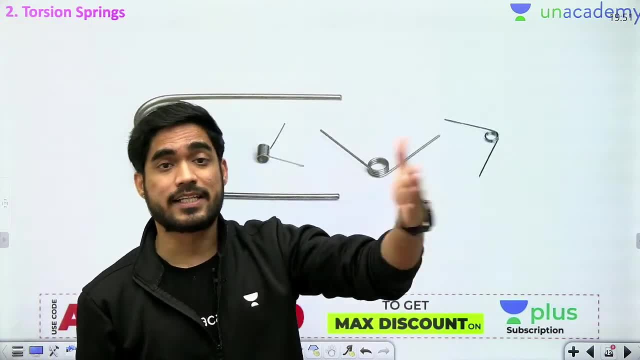 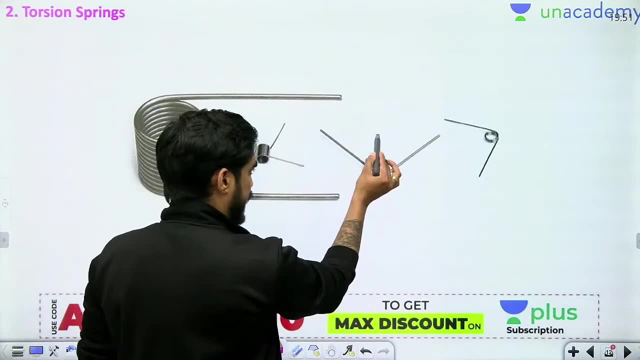 Door hinge, The hinges which are used to automate. They automatically shut the door. So, my dear, those door hinges also use this type of spring. Okay, So now in this spring, my dear, this is the axis of the spring. 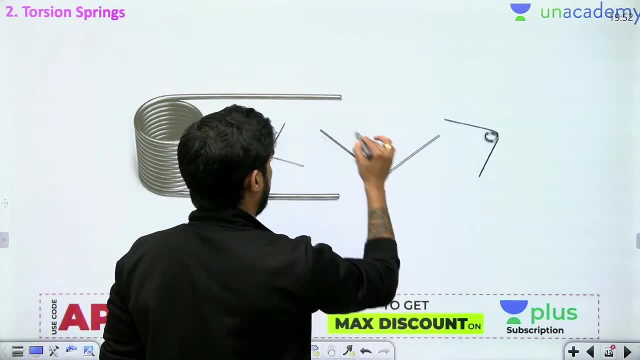 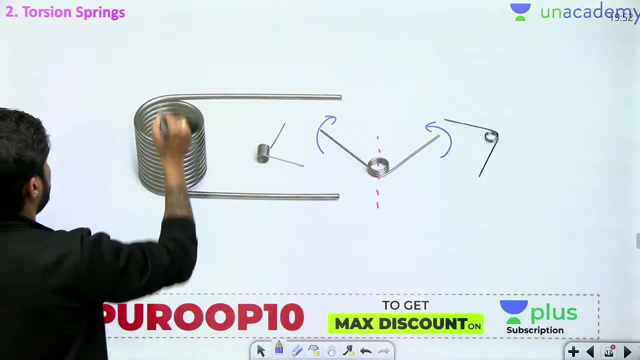 Okay, Now, if I am applying this kind of movement, if I am applying movement like this, So, my dear, which kind of movement will this be? This will be torsional movement. right, This will be torsional movement, Torsional movement or twisting movement. 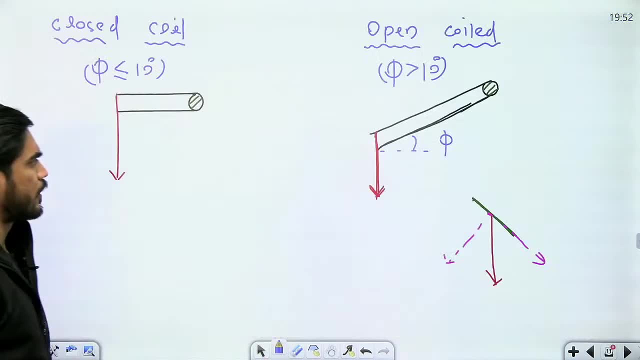 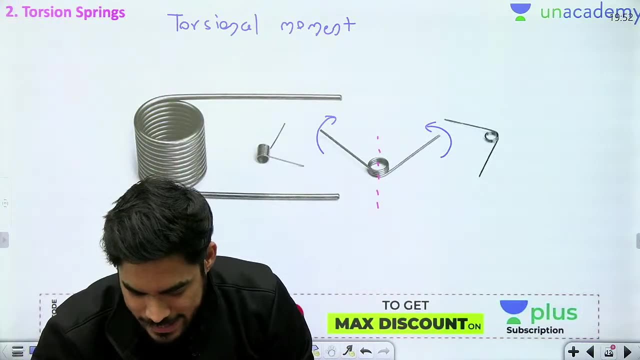 So, my dear, these are used to support torsional movement. Okay, Just like these are used to sustain axial loads, these are used to sustain torsional movement. Thank you so much, Vikas. Thank you so much, Jiahul Haq. 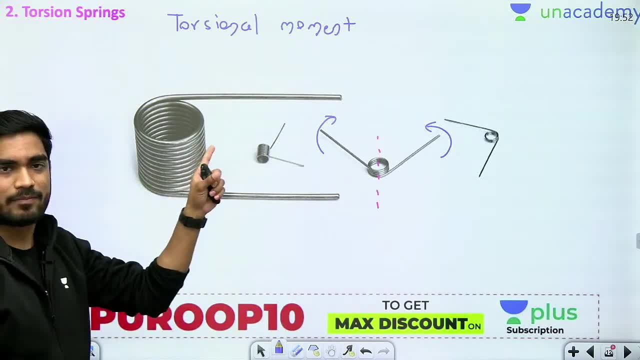 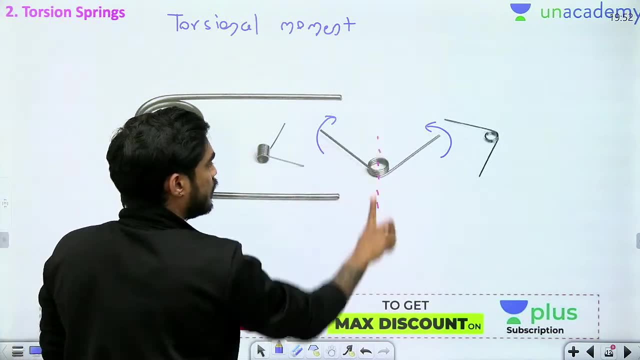 Thank you so much. Thank you so much, my dear, Thank you so much. So, my dear, this type of spring that is used to support twisting movement. Okay, When you will apply load on this, you will apply load like this: 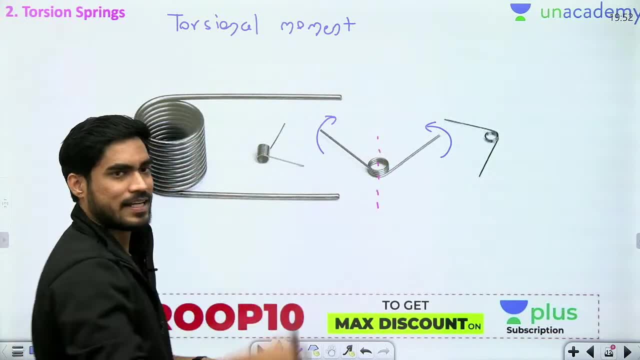 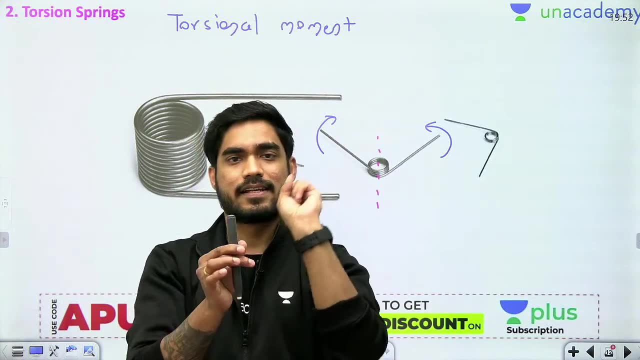 So what will this be for? This will be for axis. this will be a twisting movement. Right, This is the axis of my spring. I am applying movement like this, So my movement is acting about this axis. So if the movement is acting about this longitudinal axis, it is known as twisting movement. 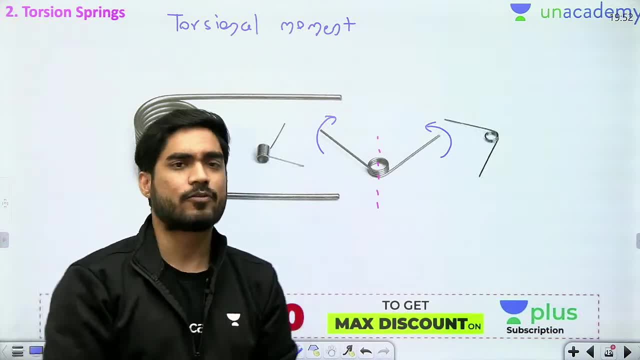 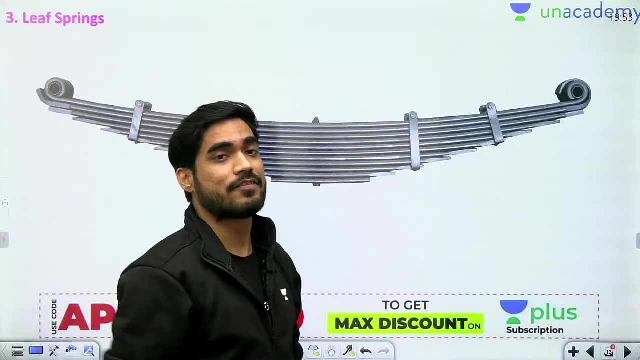 Right, If it is looking like a movement of longitudinal axis, that is a twisting movement. So this is a twisting movement. Okay, Then my dear leaf spring. Now, where have you seen leaf spring? Where you might have seen leaf spring? 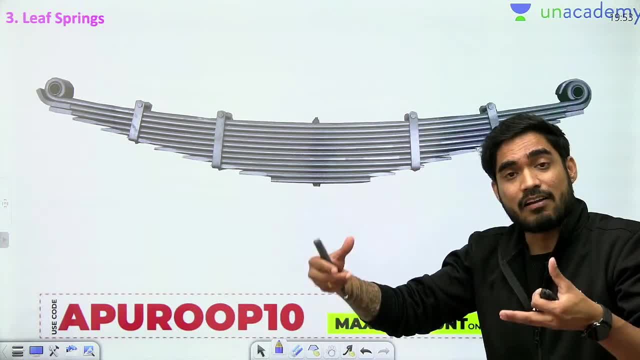 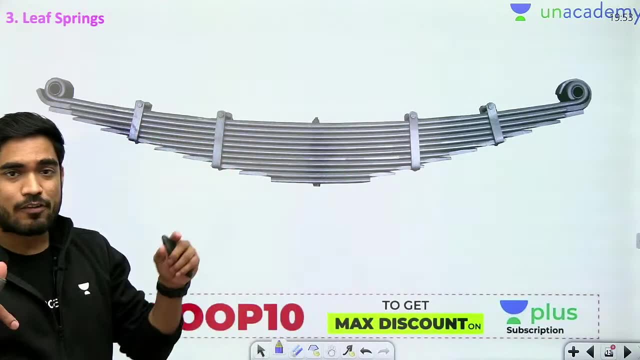 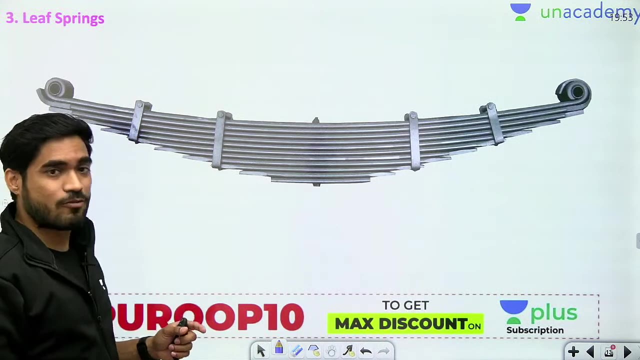 My dear. you might have seen leaf spring in very heavy duty vehicles like trucks, lorries, Right In those. you might have seen leaf springs. Now, leaf springs are used in suspension Suspensions. In suspension, they are used in order to sustain what 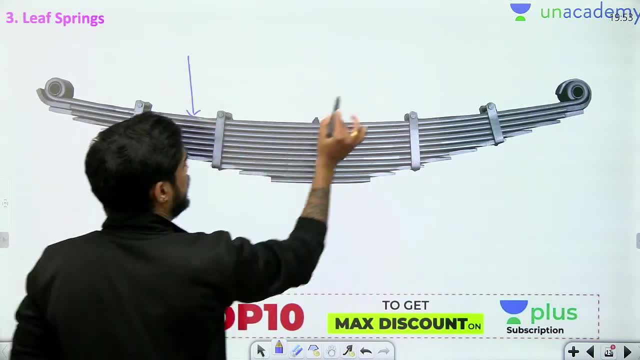 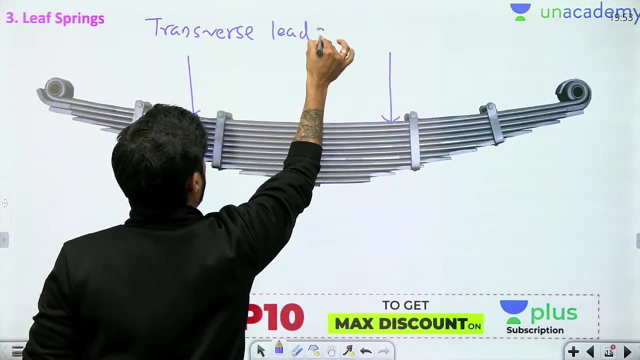 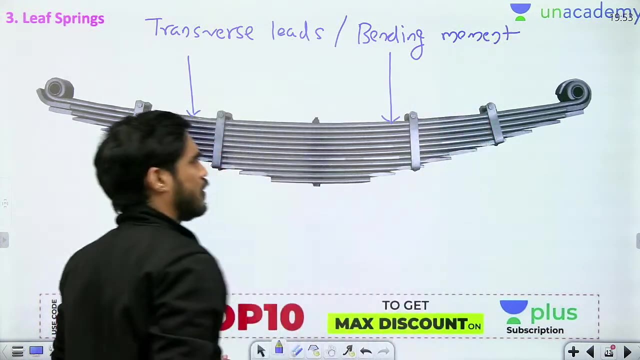 In order to sustain transverse loads. For what they are used- Transverse loads, Or you can say bending moment, Transverse load- or you can say they are used to sustain bending moment. Okay, But dear, we don't have to worry about these springs. 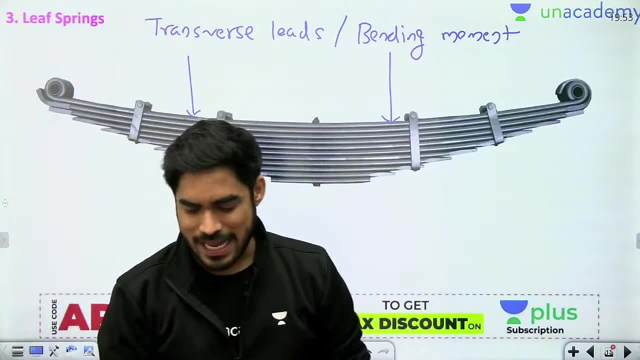 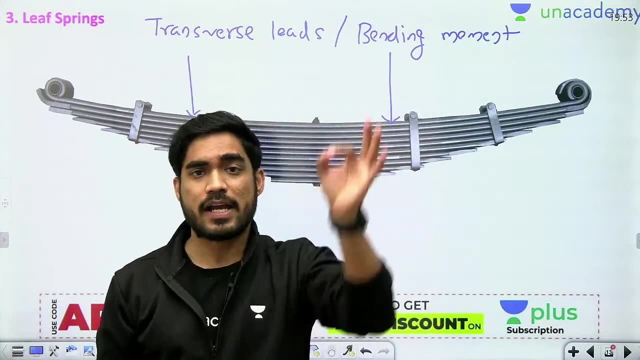 Torsion spring, leaf spring. they are not in our syllabus. In our syllabus we only have one particular type of spring: close coil helical spring. Close coil- helical spring. That's it. So, dear, you need to know different types of spring. 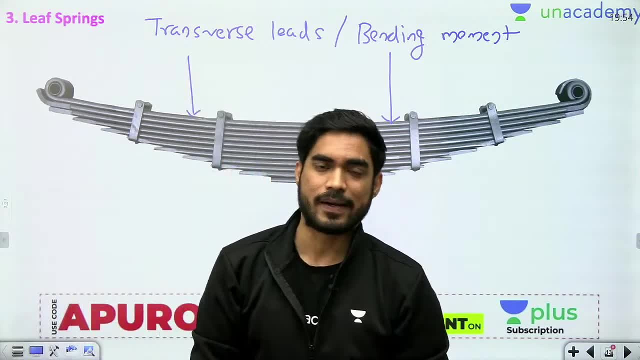 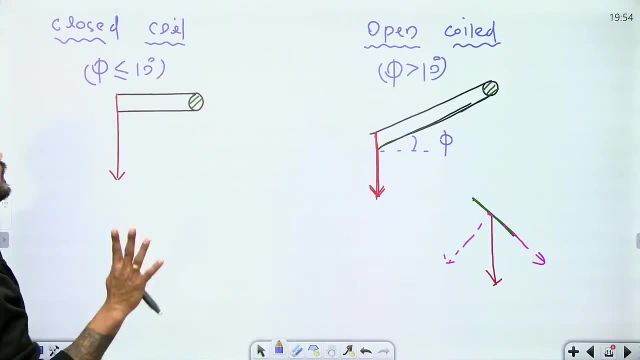 But you don't need to get into the details of each and every spring. You don't need to get into the details of each and every spring. You don't need to see their design equation. You just need to worry about one spring, and that is the close coil, helical spring. 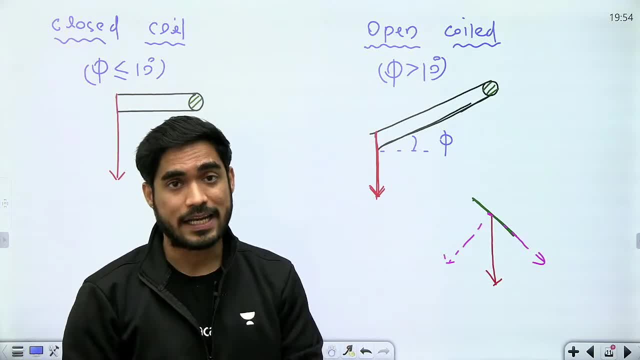 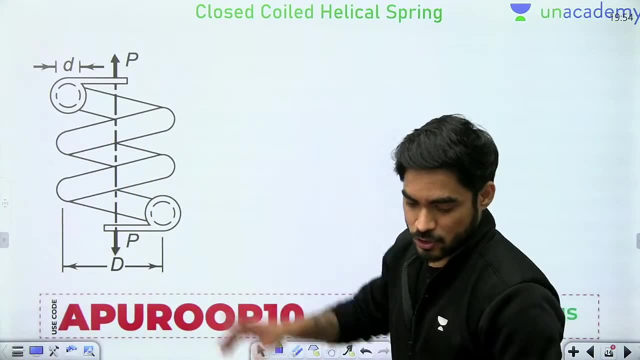 Okay, So shall we start the design of close coil helical spring. So, my dear now, what all we will get to see in the design of close coil helical spring? Let's understand that. Okay, So, close coil helical spring. 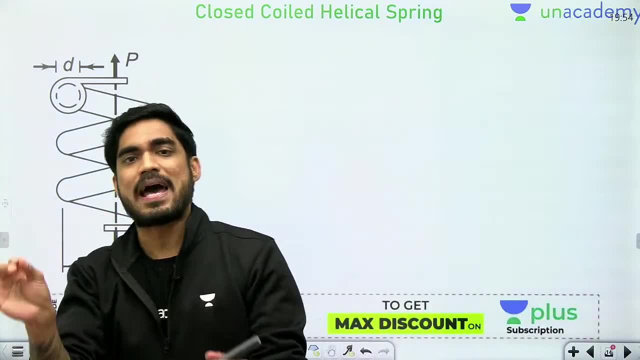 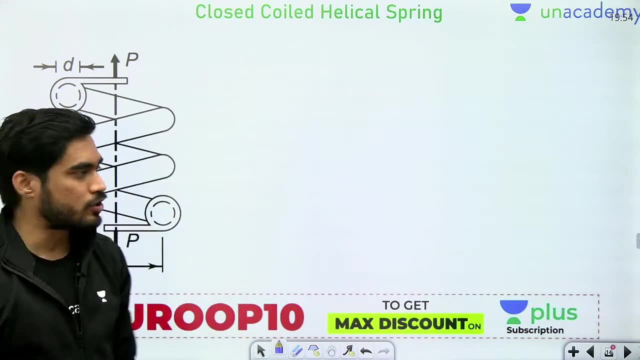 Okay Now, dear, first we will understand the different parameters based on which we are going to derive the equation. Okay, Those who are going to derive the equation in terms, first understand them. So dear, here I have shown this close coil: helical spring. 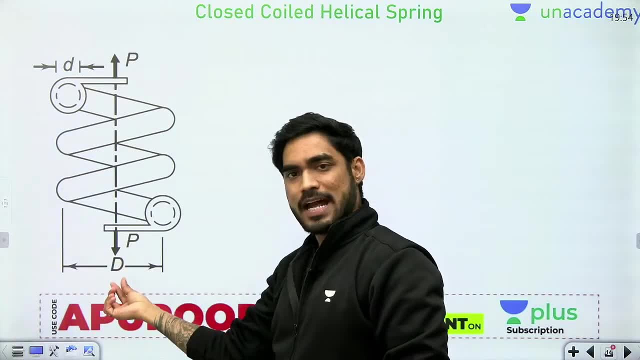 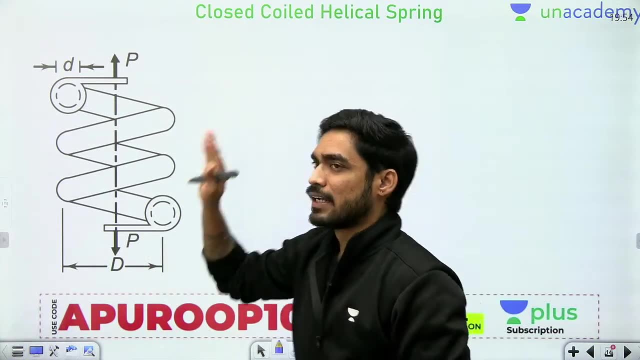 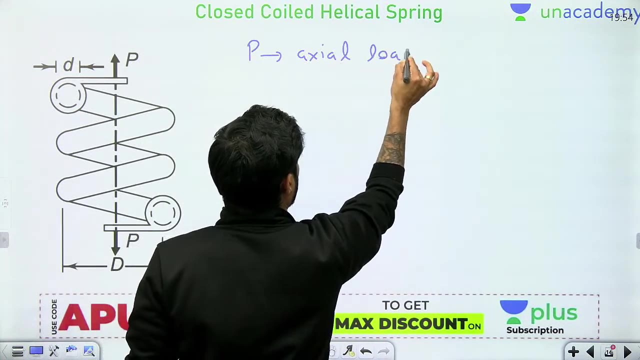 Okay, The ends of the spring are like this, So that, dear, I can show you how the load is applied. Okay, So what type of load right now we are using? We are assuming a tensile load. Okay, P is the axial tensile load. 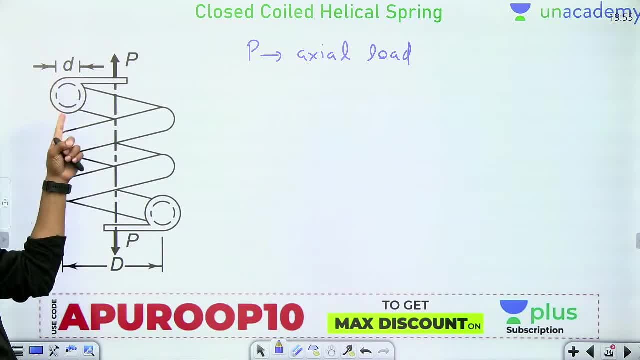 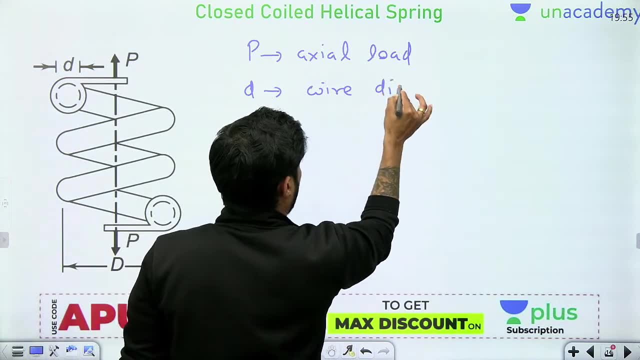 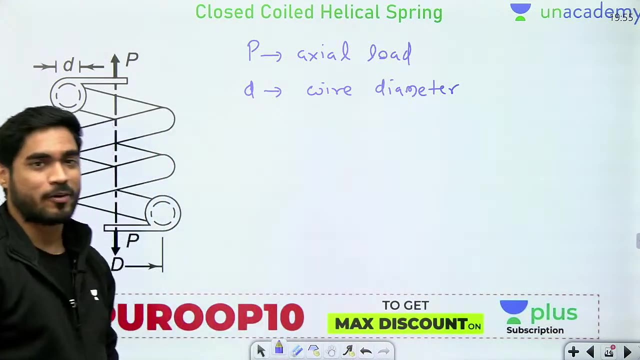 Okay, Now, dear, there is a diameter small d. There is a diameter capital D. What is small d? Small d is known as wire diameter. So sorry, Daily this is happening. Okay, Something gets dropped from here. So small d is known as wire diameter. 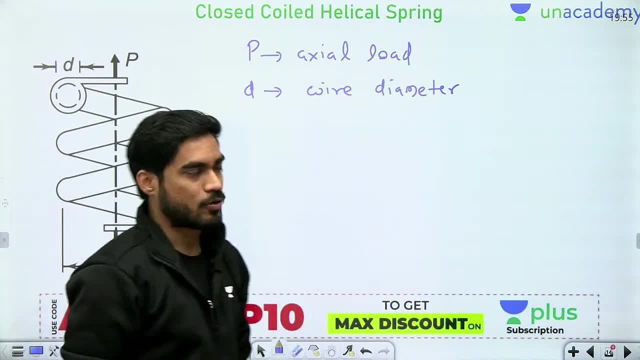 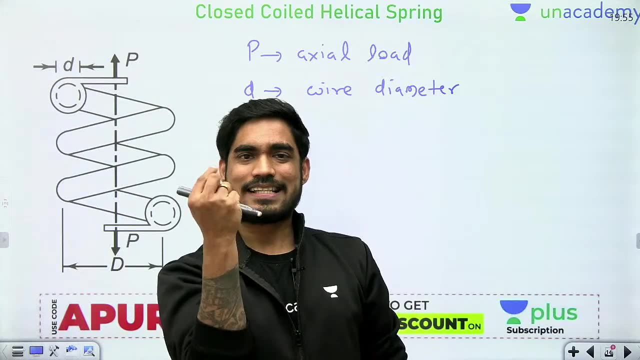 What is small d dear? Small d is known as wire diameter. Okay, Now what is wire diameter, dear? Helical spring is made of a wire. Okay, It is made of a wire. So this is the diameter of that wire and this is also the diameter of the cross section. 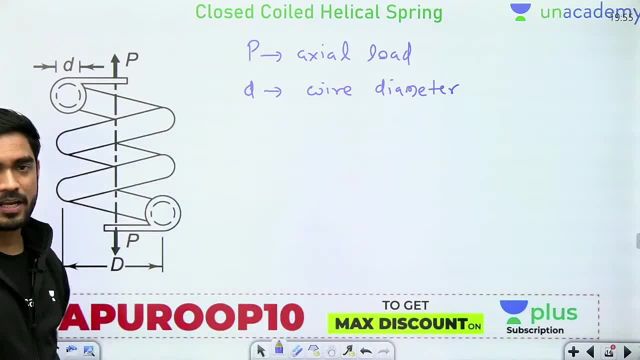 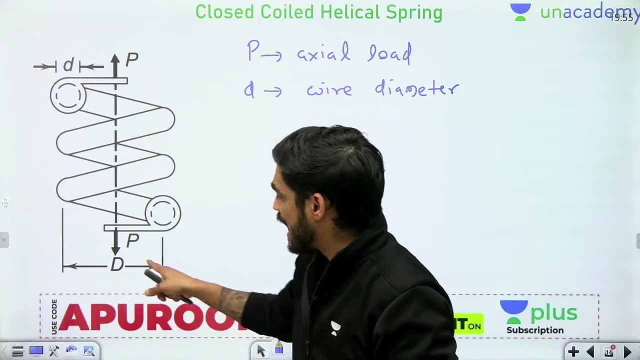 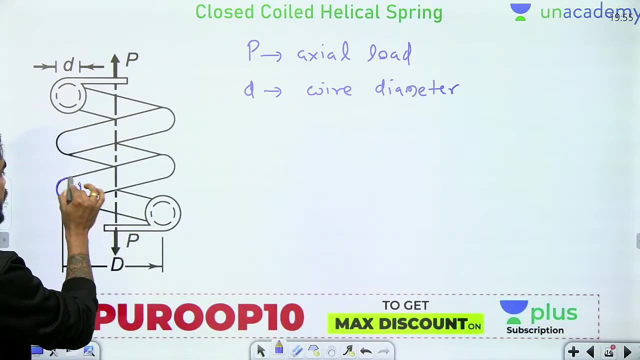 Okay, The cross section is its diameter. Okay, Now, this helical spring is turned in circles like this, Right? So the mean diameter of the circle is capital D. Now, why am I saying mean diameter, my brother? Because, dear, if you consider one circle here and one circle here, then, dear, this capital D will be measured from this center to this center. 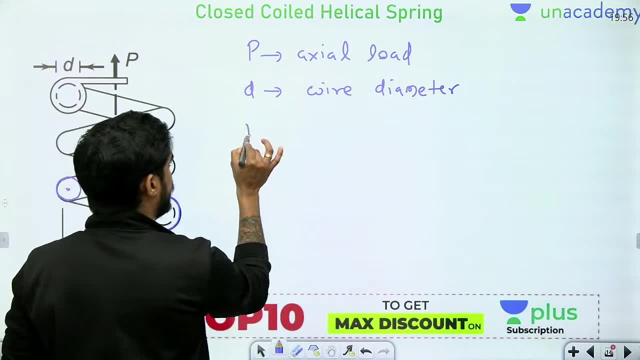 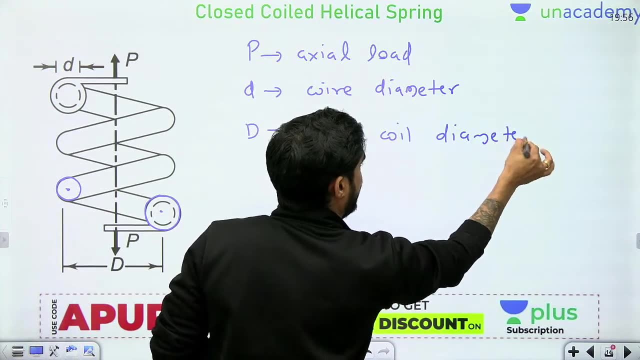 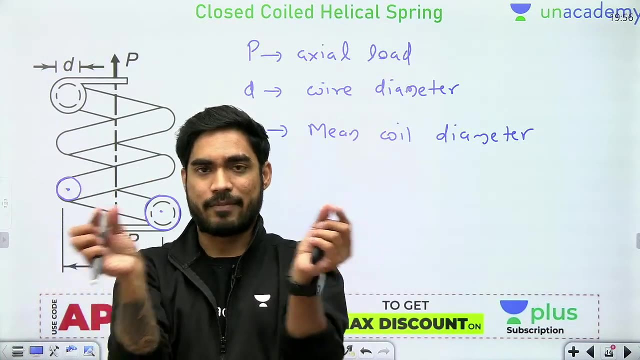 Okay, This is the distance from this center to this center, So that's why it is known as mean coil diameter. Okay, From one extreme end to another extreme end, if it is a circle like this, then from one extreme end to another extreme end, this is the diameter. 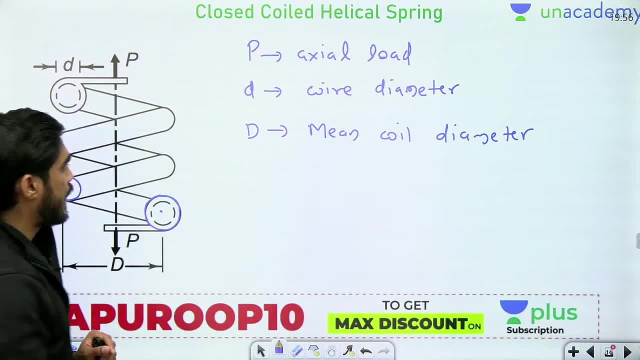 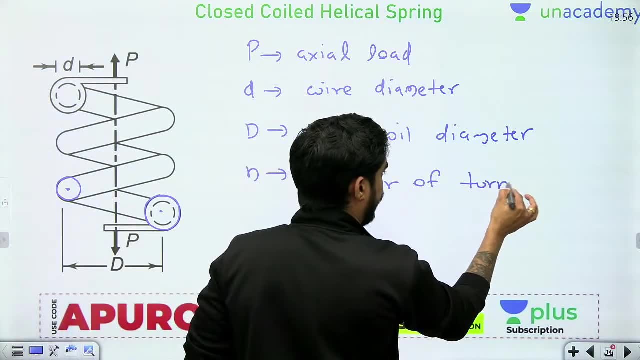 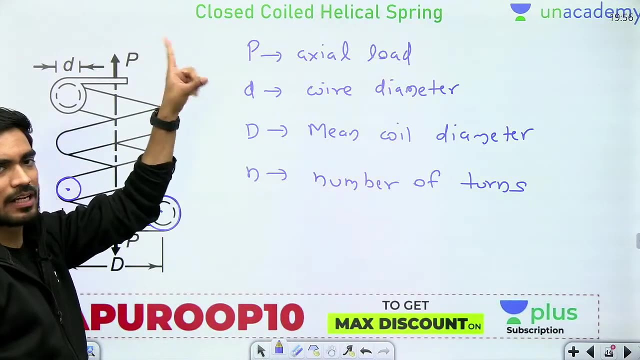 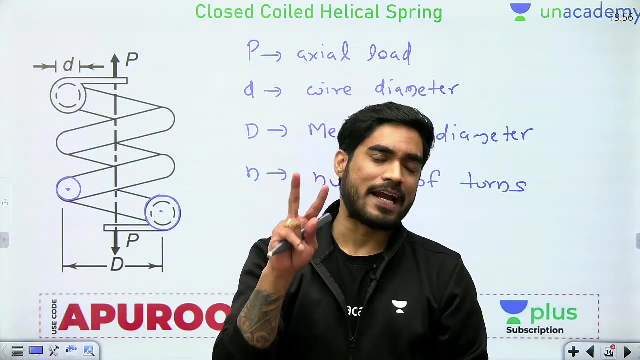 Okay, Capital D. Okay, Then dear. n are the number of turns. Okay, So dear. these are the parameters of the closed coil helical spring. Now, what is our objective here? Our objective here is to find basically two things. 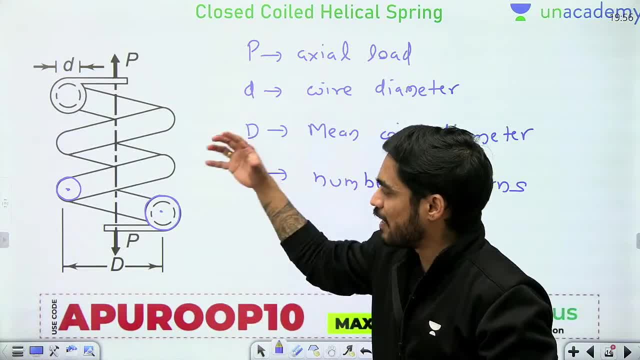 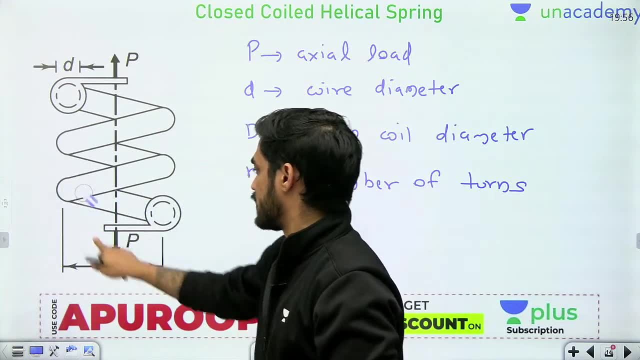 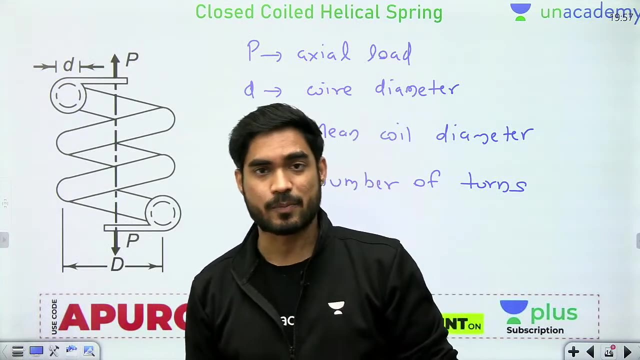 First, the maximum stress developed in the cross section of the spring. Okay, First, what do we have to find, my brother? Maximum stress developed in the cross section. Why? Why maximum stress? Because, dear, the strength of the spring will be one criteria to design the spring. 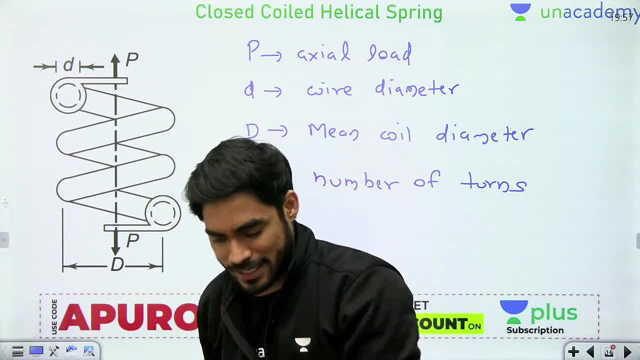 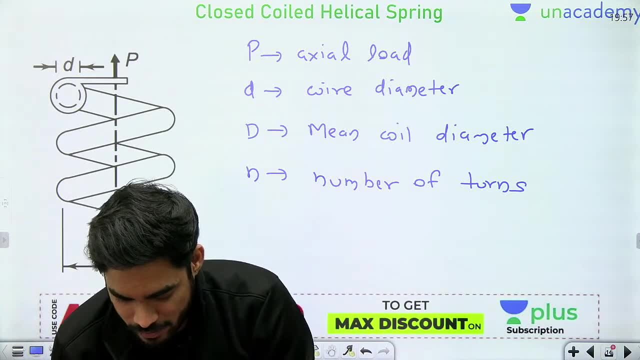 It should not break, It should not yield. Neither it should yield nor it should break, Right? Thank you so much, Anshul. Good evening Pranaav. Good evening Pranaav. This should neither yield nor it should break. 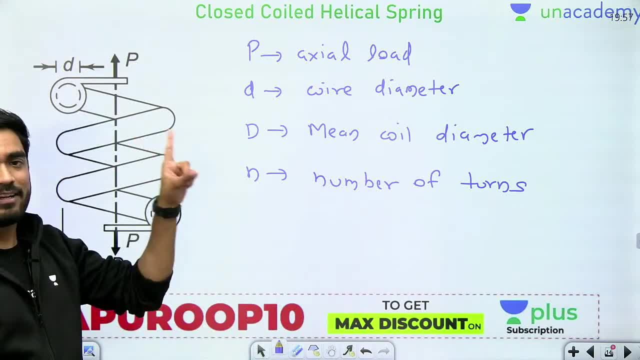 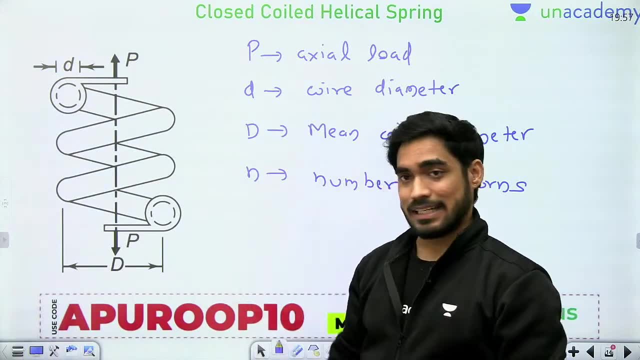 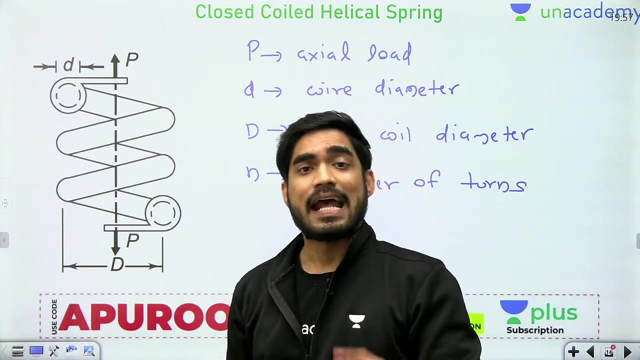 So that's why, my brother, one criteria will be maximum stress, And the second objective is to find the deflection. Now, why deflection? Because, dear in all application of spring, deflection is very important. Okay, 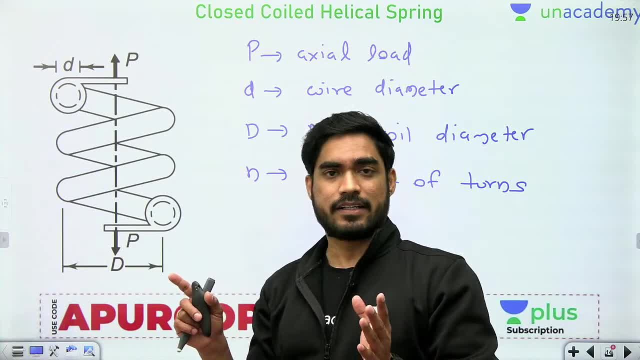 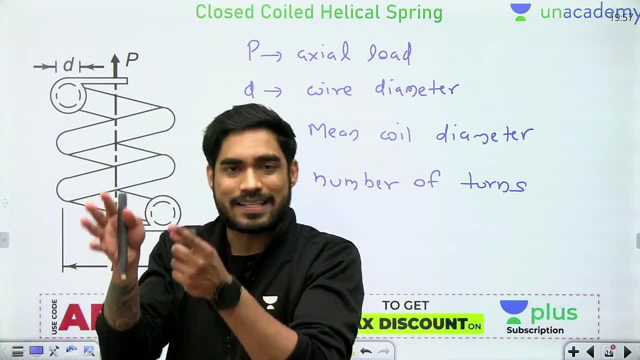 Energy stored in the spring, stiffness of the spring- all of that is calculated based on deflection of spring. So dear, here are basically the criteria Here. our basic two objectives are to calculate the maximum stress and to calculate the deflection. 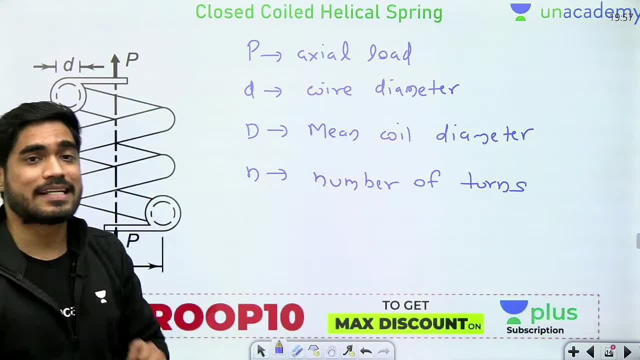 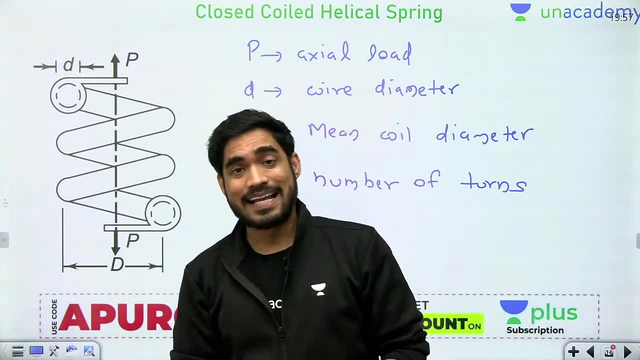 Now, dear stress, which stress are we talking about Here? which stress we will calculate Here? we will calculate the shear stress, Because dear springs are usually made of ductile material and ductile materials will fail due to shear stress. 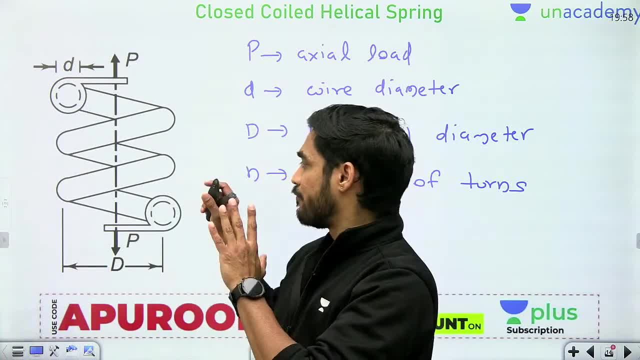 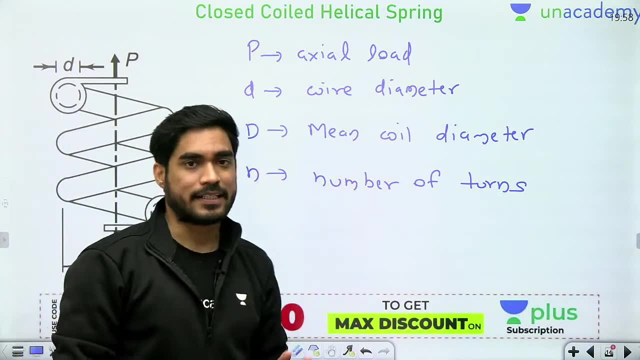 So we are going to assume that this is going to fail in shear, So we will calculate the maximum shear stress. That is our objective. Okay, So dear, two objectives: calculating maximum shear stress and calculating deflection. Now understand. 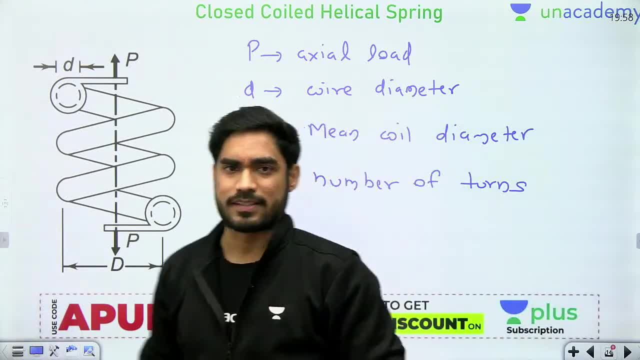 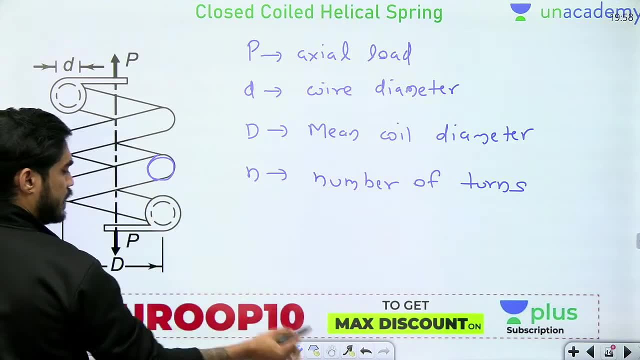 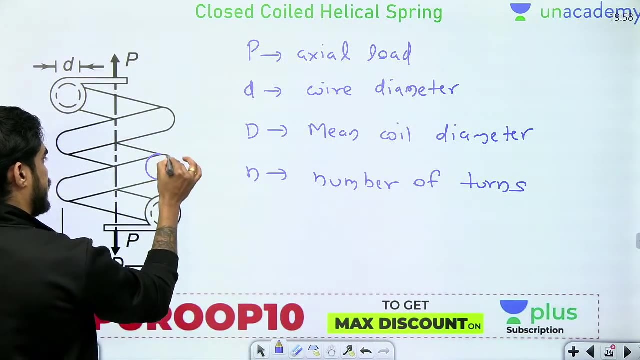 Here, if you consider any one cross section, if you consider any one cross section, let's consider this cross section. Okay, Let me consider this cross section. Let me consider this cross section. So, if you consider this cross section, dear, 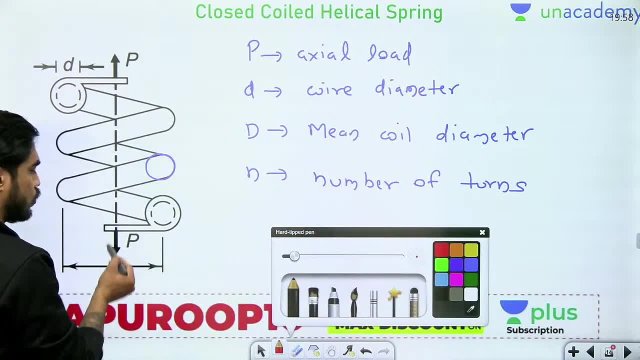 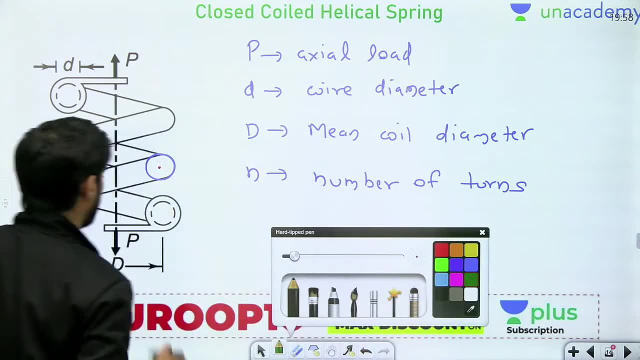 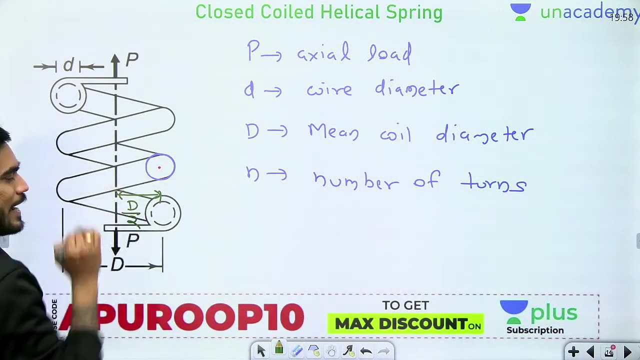 Then the load is not passing through the centroid of the cross section. Right, The load is not passing through the centroid of the cross section. It is at a distance of how much? How much distance is there D by 2.. It is at a distance of D by 2 from the center. 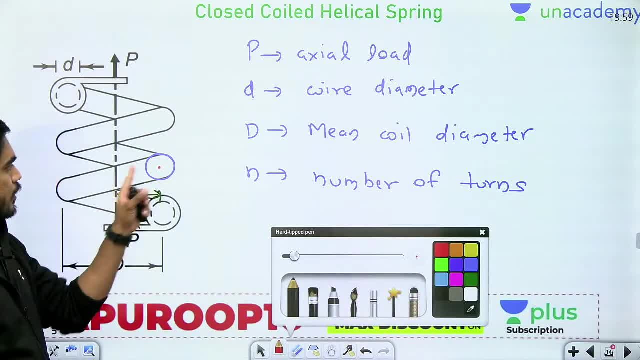 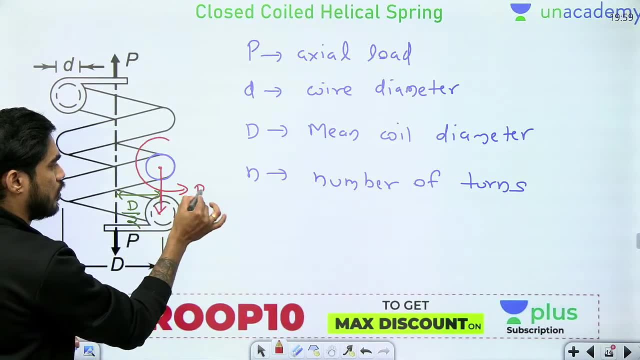 So if you transfer the force from here to here, then you will get a force P and you will get a moment P D by 2.. Right, You will get a force P and you will get a moment P D by 2.. 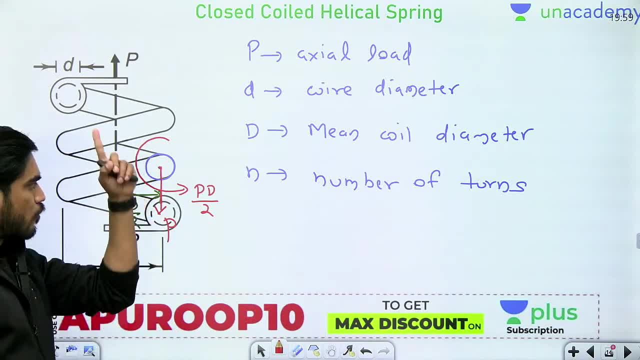 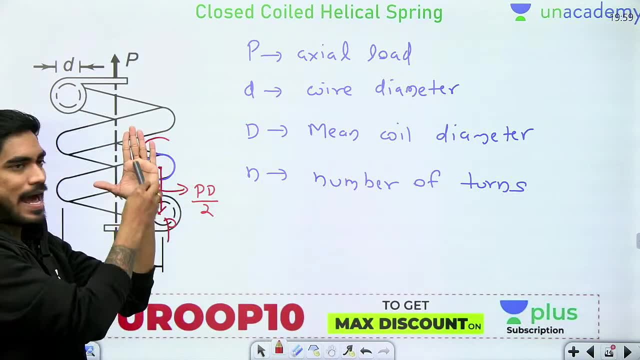 Now this force is acting parallel to this cross section. Right, This force is looking parallel to the cross section. So this will be a shear force. So it will cause direct shear stress force upon area. Right, This will be a direct shear force. 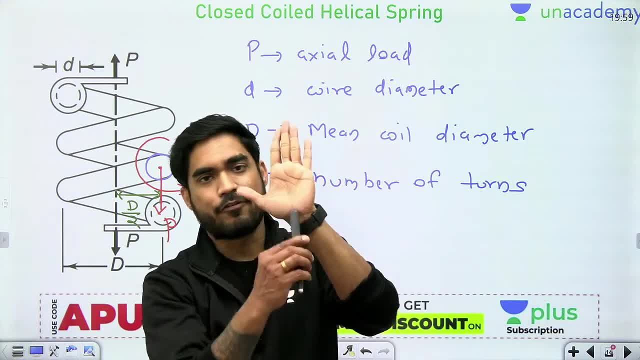 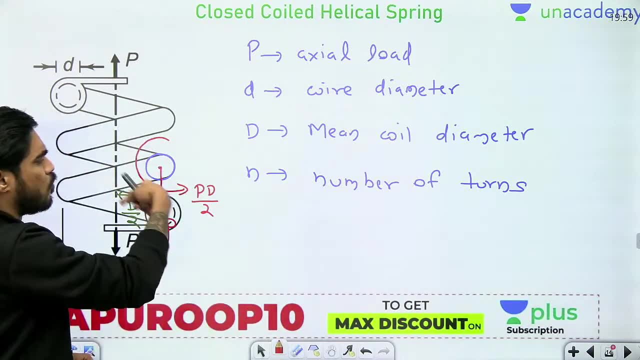 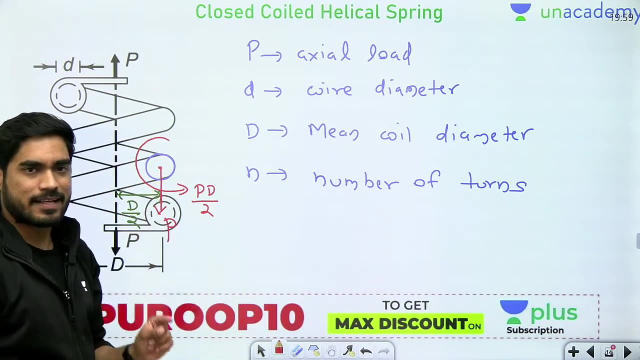 This will be a direct shear stress development force, Right, Right, This will develop shear stress in the cross section Direct shear stress force upon area. But what will be this moment? Whether it will be bending moment or twisting moment, Because if it is a bending moment, it will cause bending stress. 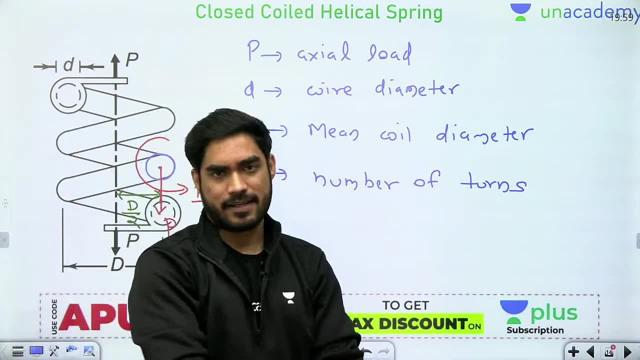 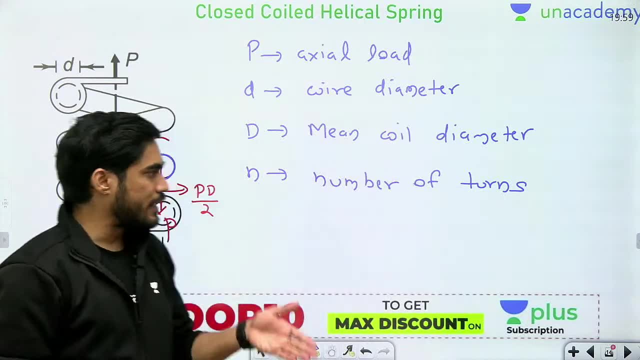 And if it is a twisting moment, it will cause torsional stress. So it is very important to understand whether it is bending moment or twisting moment. Okay, Now understand how this moment is acting. So this is my cross section. 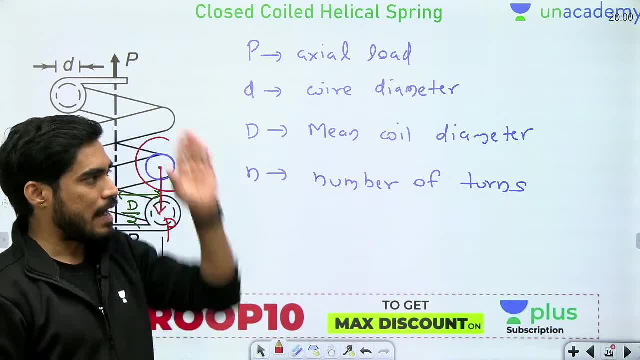 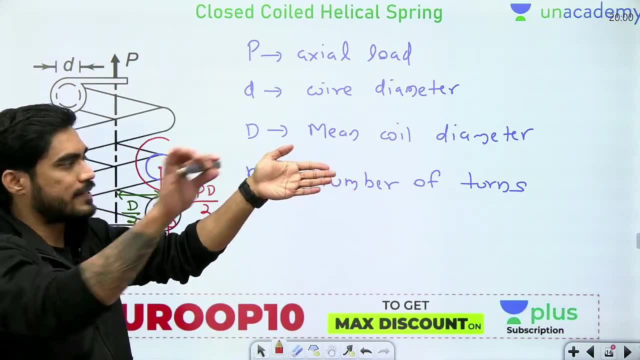 My cross section is in this plane. Your spring is cut like this. You have cut your spring like this. So this is the plane of the cross section, Okay, Which you can see from front. This is the plane Now. the moment is acting like this. 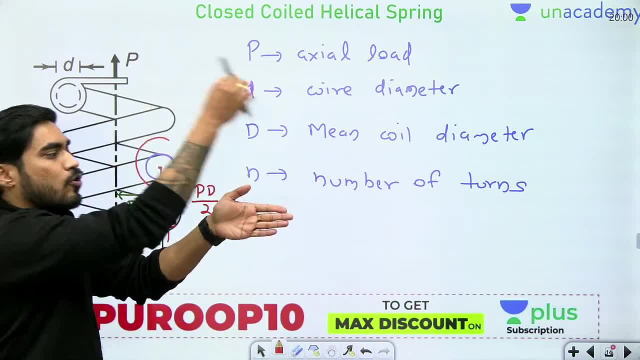 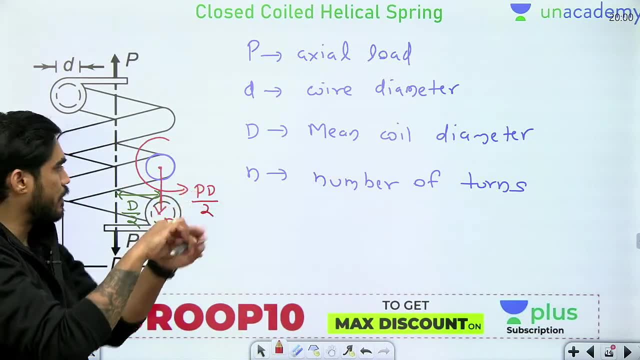 I have transferred the force from here to here. So the moment is acting like this. About which axis? This moment is acting about this axis. Okay, The moment is acting about this axis, And this axis is what? Parallel axis or normal axis? 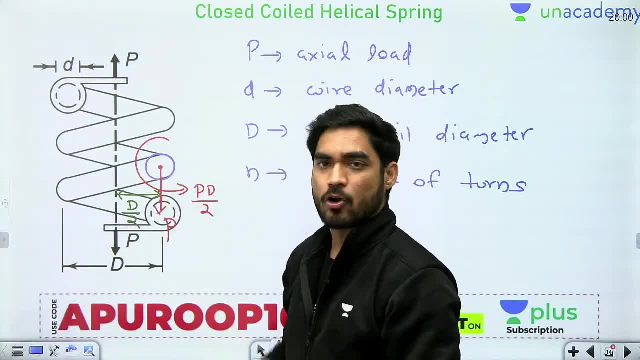 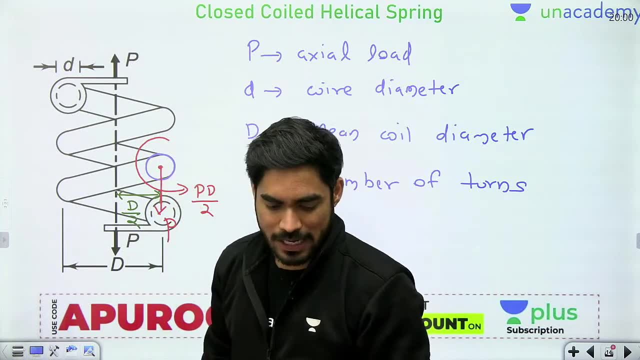 Whether it is parallel axis or normal axis of the cross section. Is this cross section's parallel axis or cross section's normal axis? Yes, this is a normal axis of cross section. So if it is a normal axis of cross section, then which moment is this? 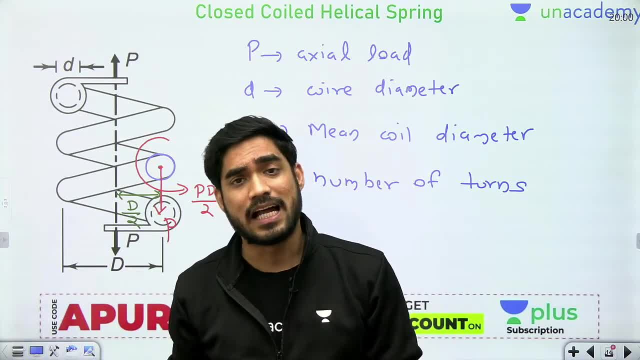 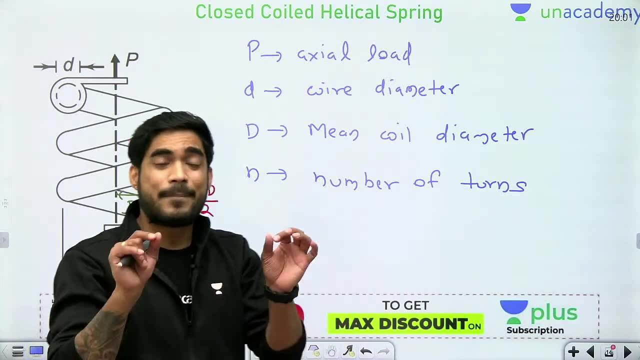 I have clearly explained, in strength of materials, What is bending moment and what is twisting moment. Very good, Ayush. Very good, Very good. So bending moment is the moment acting about this. This is the moment acting about parallel axis. 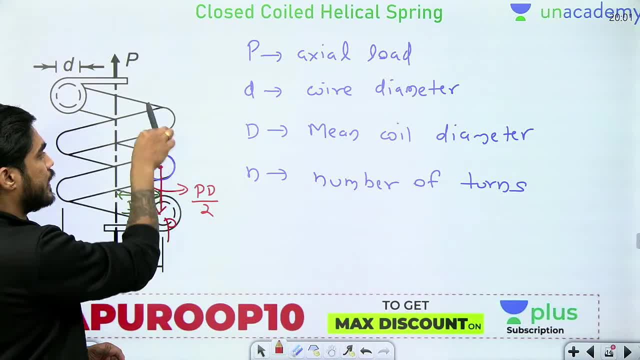 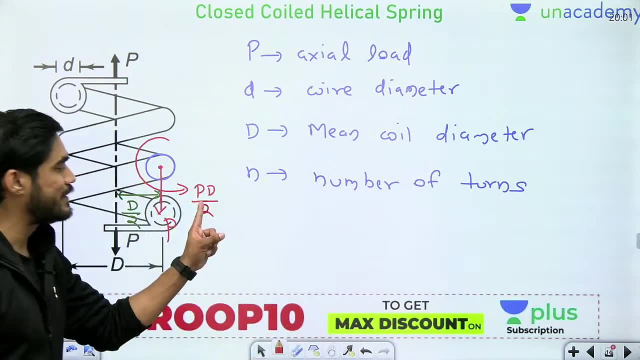 If it is about this axis or about this axis, then it will be bending moment. But twisting moment is the moment acting about the normal axis. So this is a twisting moment. And if it is a twisting moment, which stress will be developed? 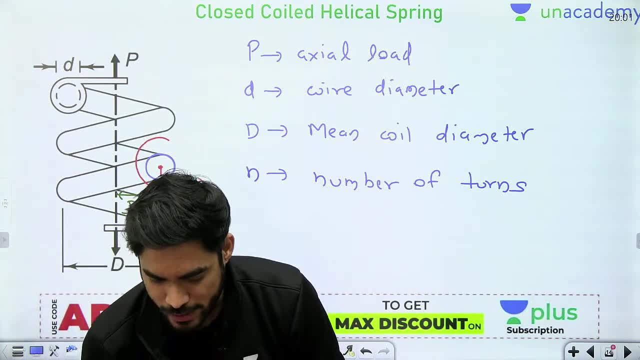 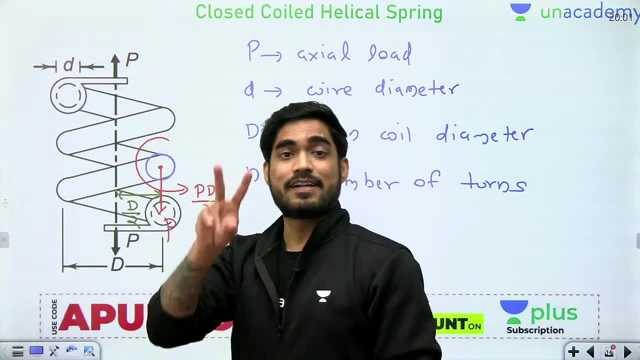 Very good. Arpit Very good, Jitendra Very good, Ayush Very good, Utkarsh Brijesh Very good. Then this will cause torsional shear stress, So we will calculate two shear stresses. 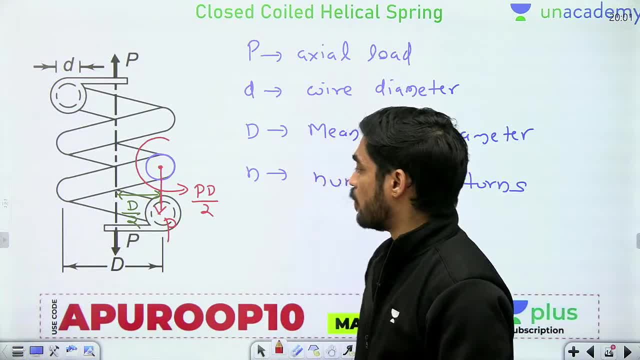 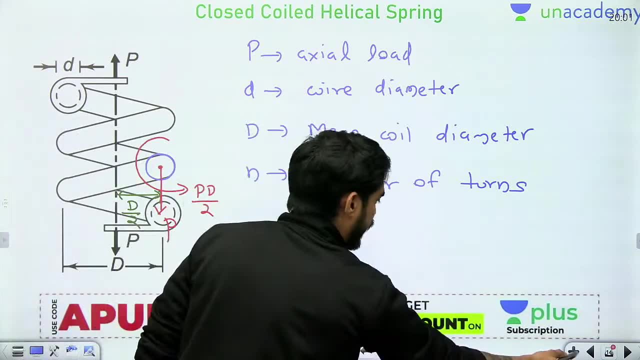 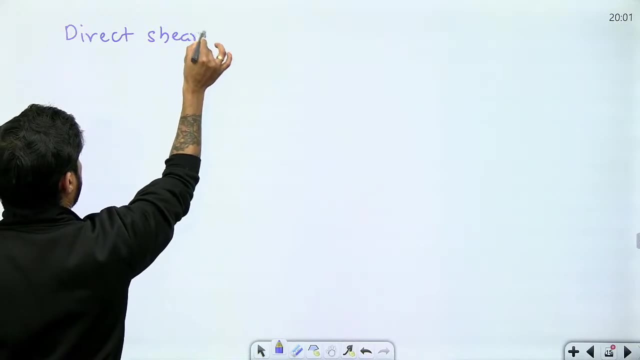 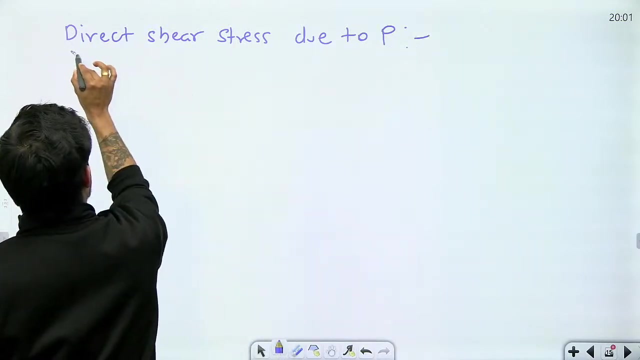 One due to force P and one due to moment PD by 2.. Now, in order to calculate direct shear stress due to P, you don't need to do anything. Simply direct shear stress due to P. How will you calculate it? 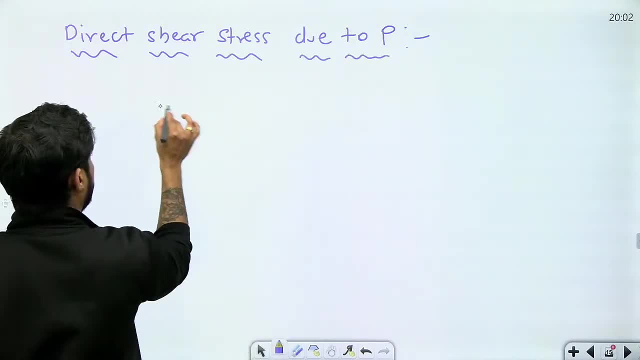 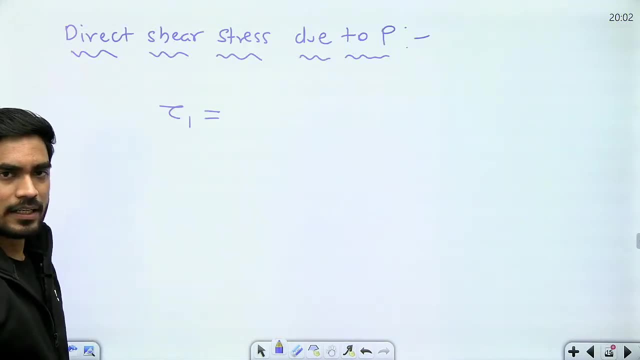 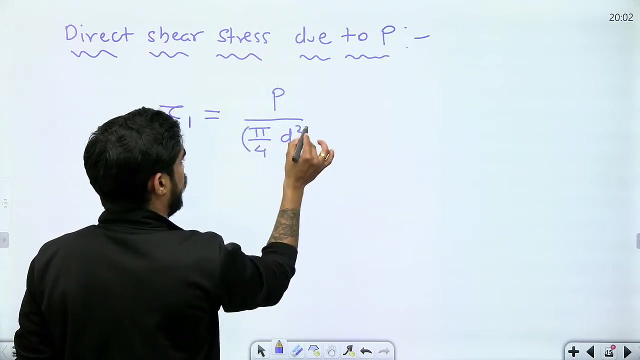 Very easy, Very easy. Let me call it tau 1. Because there are two shear stresses, One due to force and one due to moment. So I will call it tau 1.. So it will be force upon area P upon pi by 4 D square. 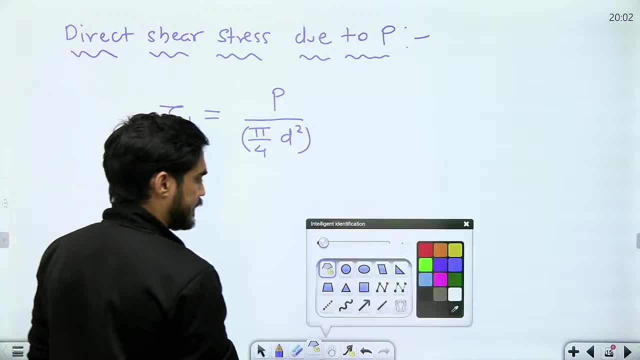 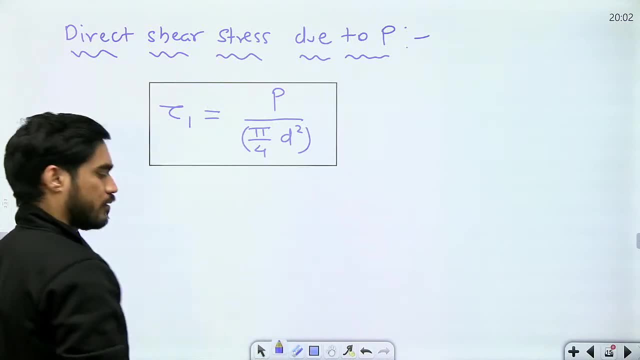 Okay, This will be the direct shear stress, tau 1.. I will call it direct shear stress, tau 1.. Okay, I will put it in a black box. Okay, I will tell you the reason later. Okay, So one shear stress is due to P. 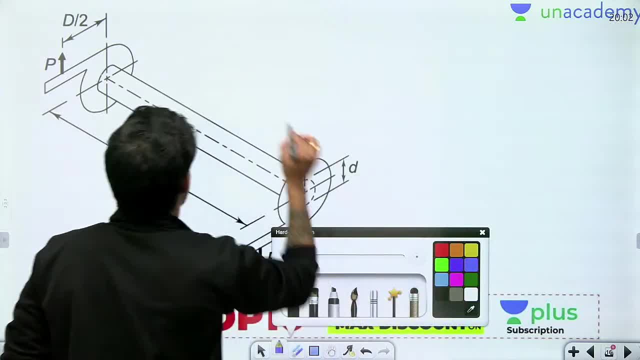 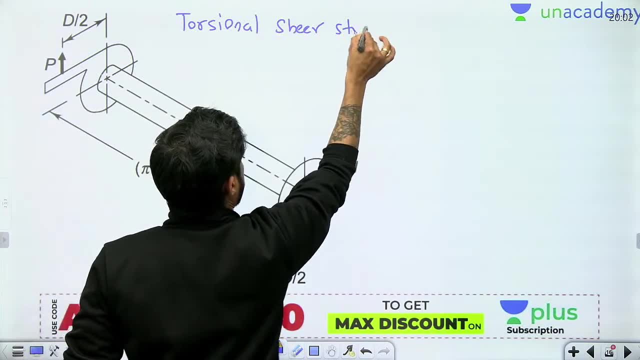 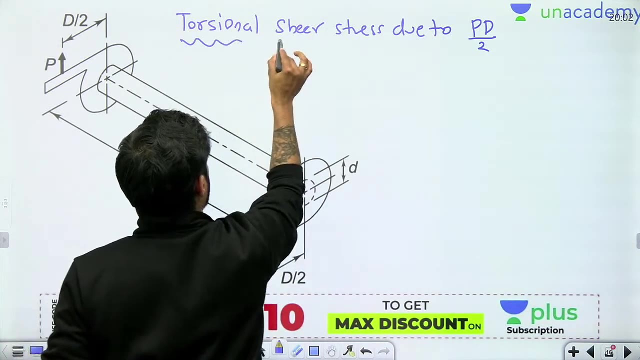 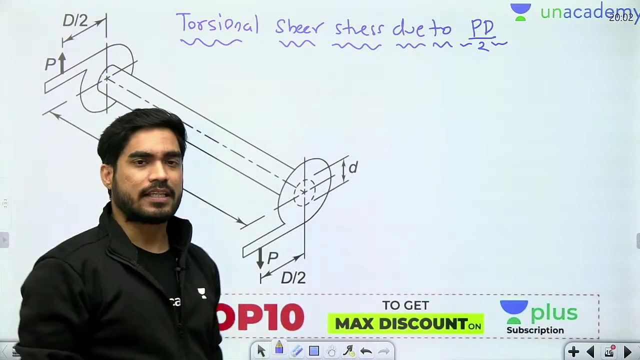 Another shear stress will be due to P into E, Okay, Which will be torsional shear stress. So torsional shear stress, PD by 2.. Now, my brother, pay attention. Torsional shear stress can be calculated using the equation TR by J. 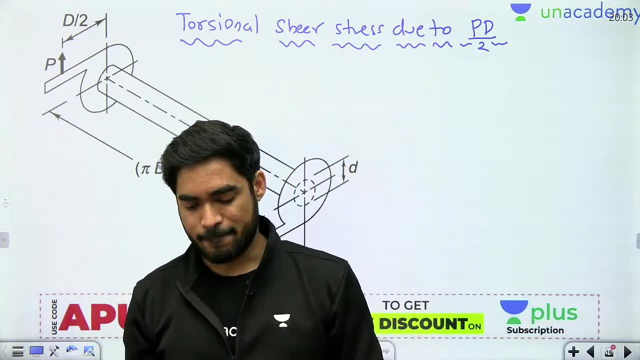 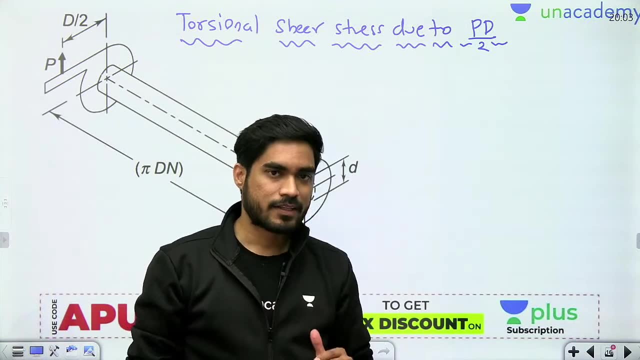 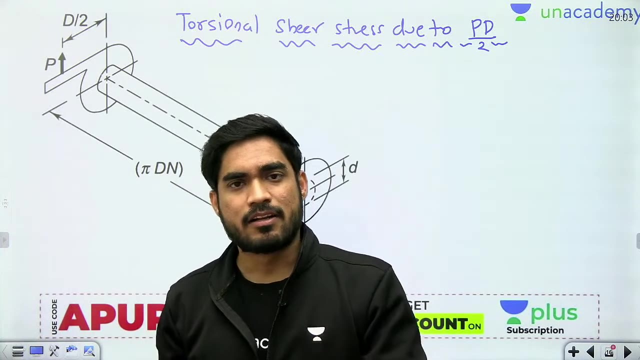 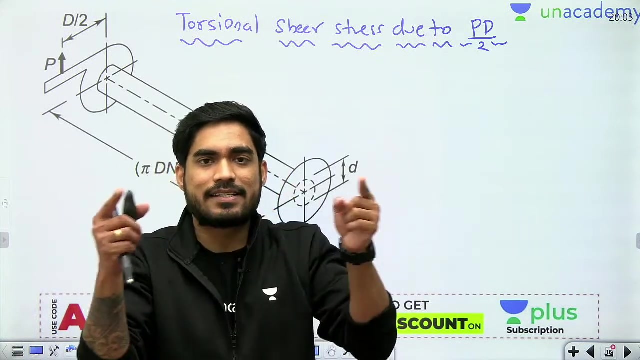 Tau equals to TR by J, But there is a problem with this equation. If you have seen my strength of material lectures, I have explained that the torsional shear stress is calculated by some using some assumption, And one of those assumption is that the shaft is straight. 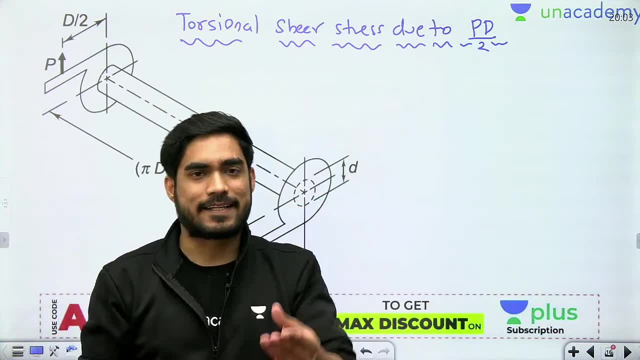 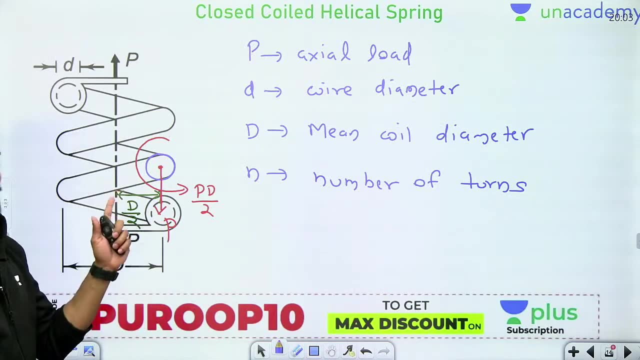 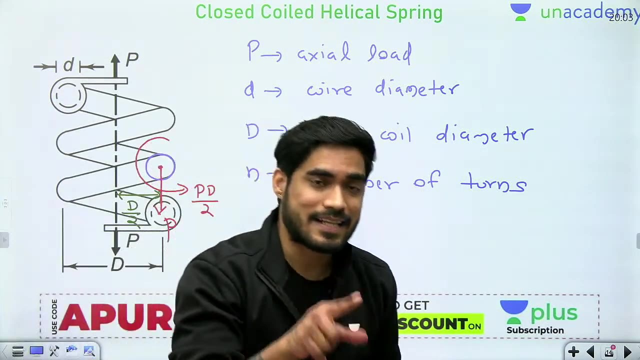 The torsional shear stress equation which we have derived. we have derived this torsional shear stress equation for a straight shaft, But the spring is not straight. right Spring is curved And the stress in curved members is more compared to the stress in straight members. 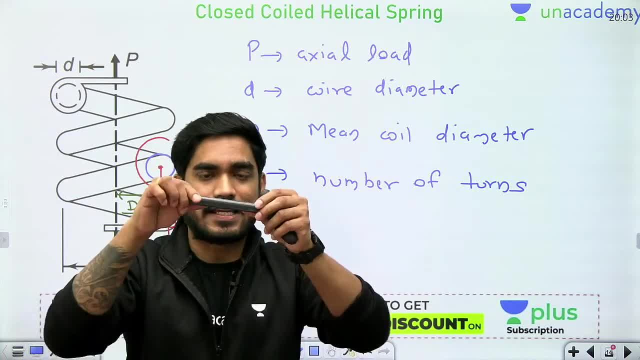 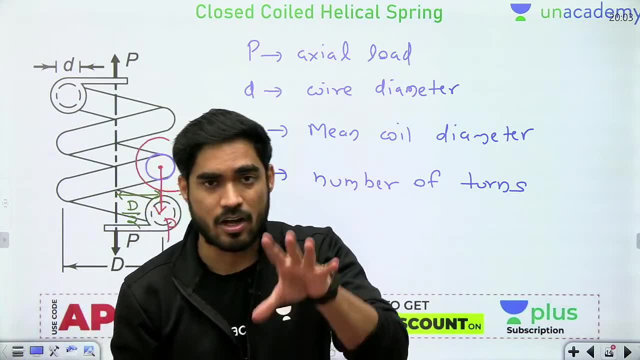 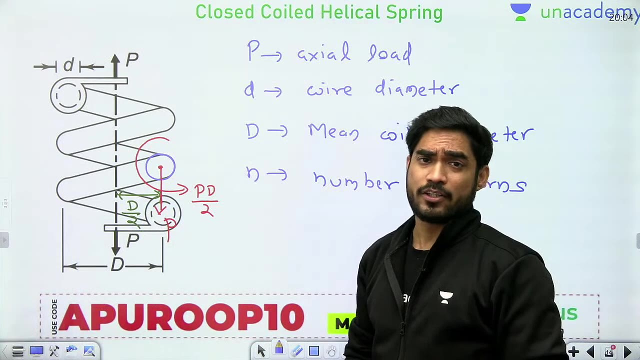 The stress in a straight member will be less. If I curve this and then calculate the stresses, it will be more. So, my brother, I know the equation of torsional shear stress, shear stress for straight member, but here the spring is a curved member. but I don't want to. 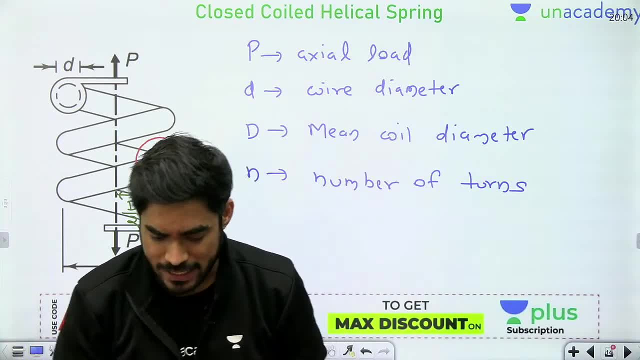 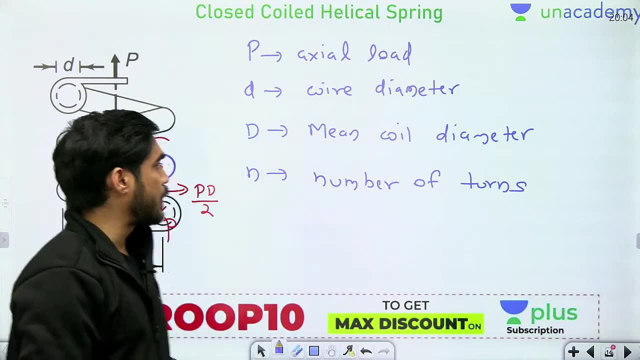 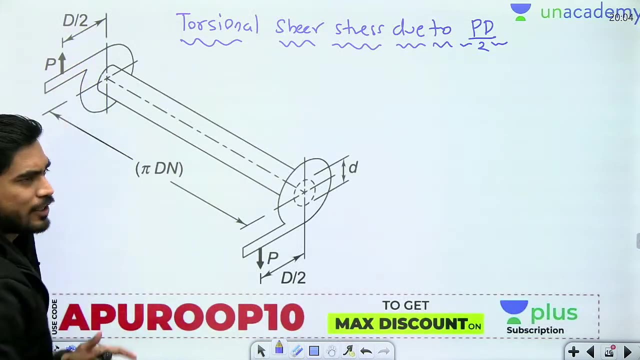 complicate my calculation. okay, I can't complicate my calculation, so I have to keep my calculation easy. so I will assume that my spring is also a straight member. so what I am doing is I am opening my entire spring in order to make it a straight member. what I did, I made it a straight. 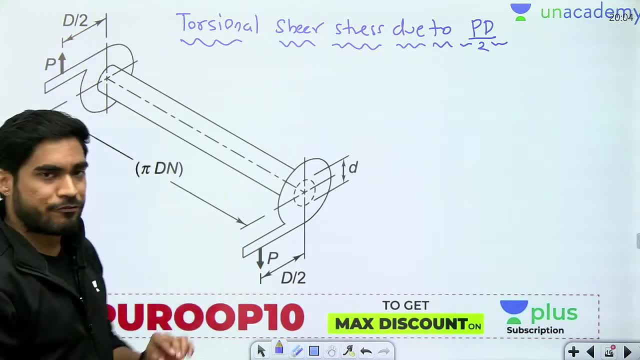 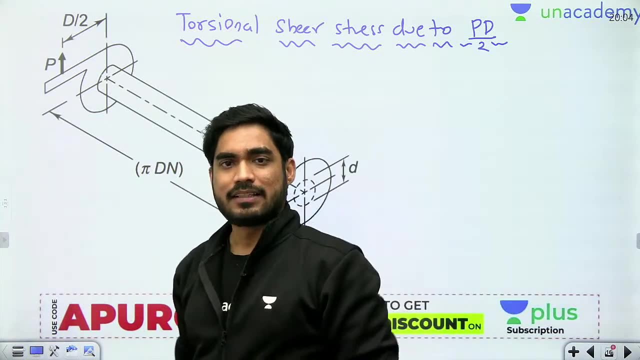 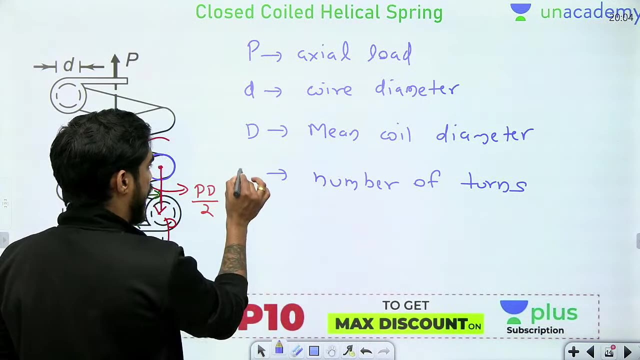 member. so if you open it it will become like a shaft, it will become like a straight shaft. what will be the length of it? the length will become pi d n. okay, here I have taken small n number of turns. write it capital n. okay, write it capital n because it is made in capital n diagram. so 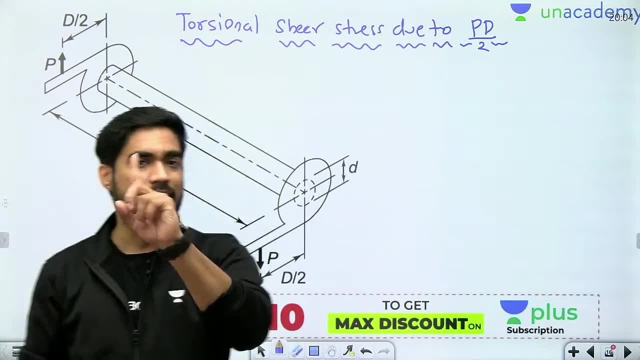 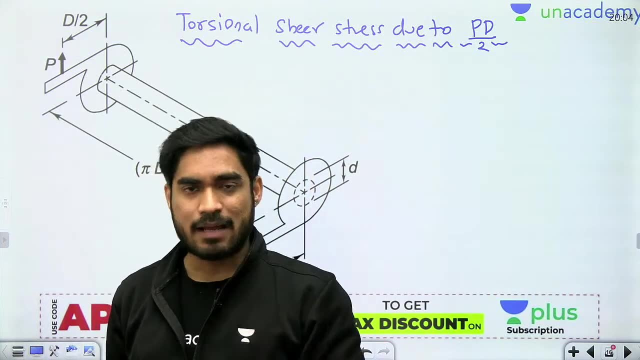 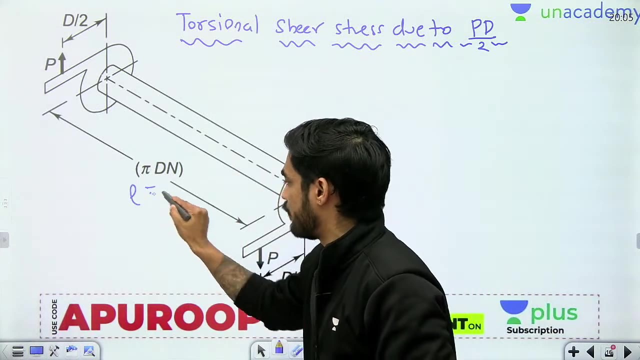 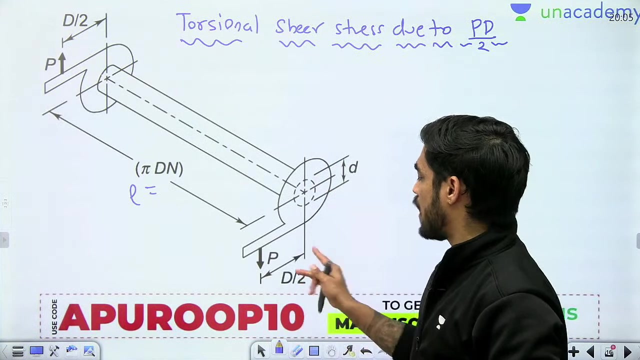 capital n is number of turns, so one turn will have a length of pi d. one turn will have a length of pi d and there are n number of such turns, so total length will become pi d n. okay, this is what. this is the length of the shaft. now understand. the torque acting on the shaft is PD by 2. the torque 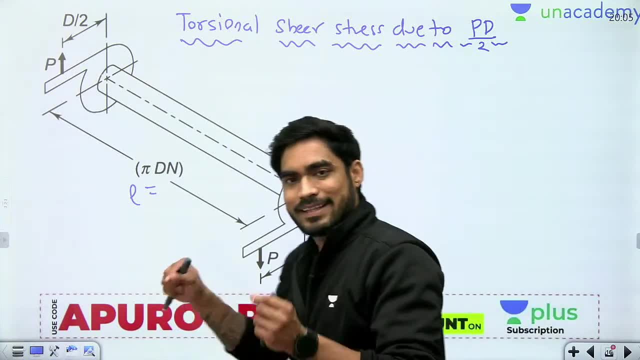 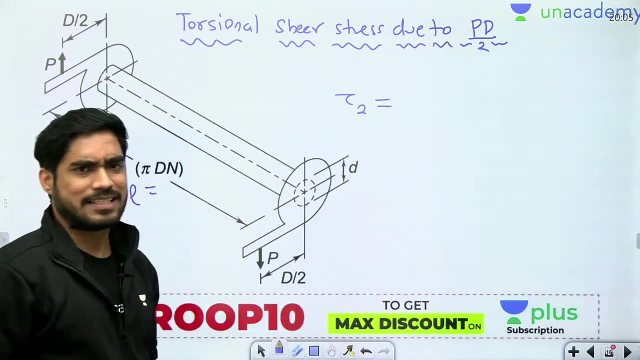 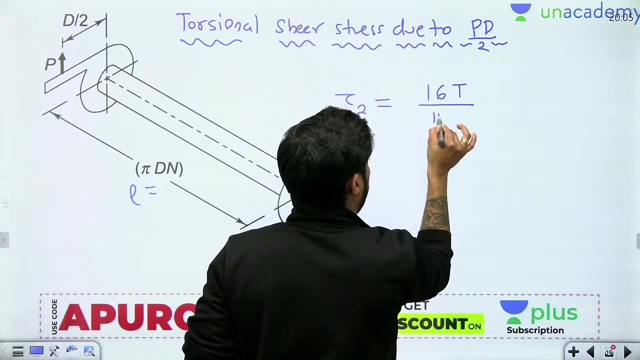 acting on the shaft is PD by 2. okay, so in the cross-section can I calculate the shear stress directly? what is the maximum shear stress in the cross-section of shaft? circular shaft: 16 t by pi d cube, right, 16 t by pi d cube and the torque? 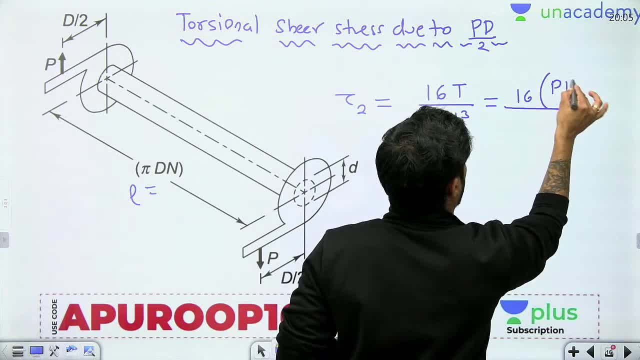 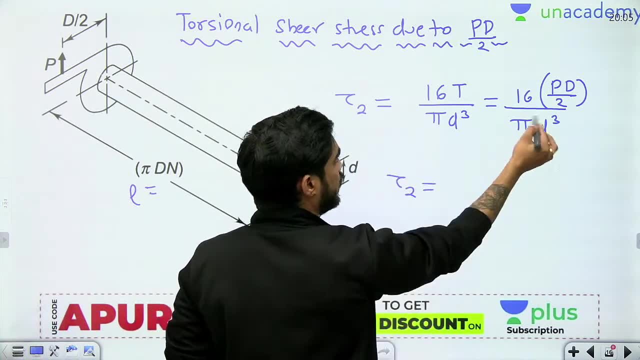 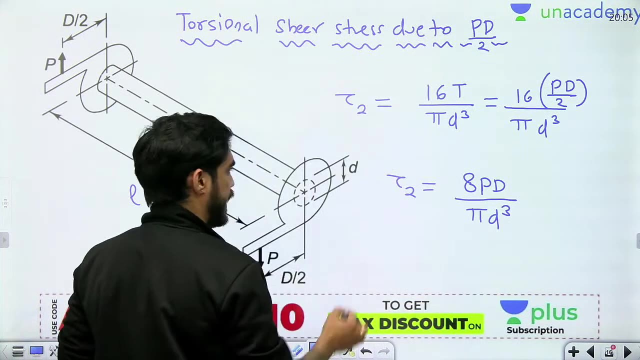 is equal to how much the torque is. PD by 2, right PD by 2. so, my brother, from here what will be tau 2? this will become 8 PD divided by pi d cube. 8 PD divided by pi d cube. 8 PD divided by pi d cube. 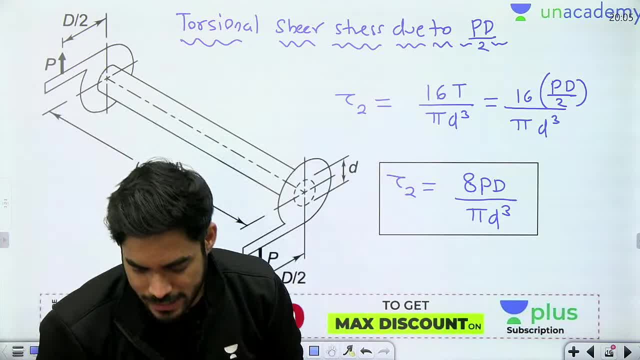 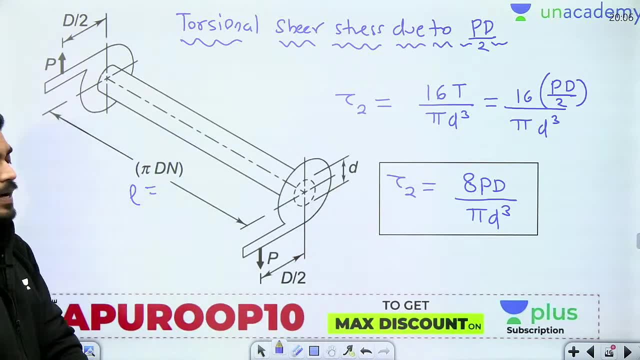 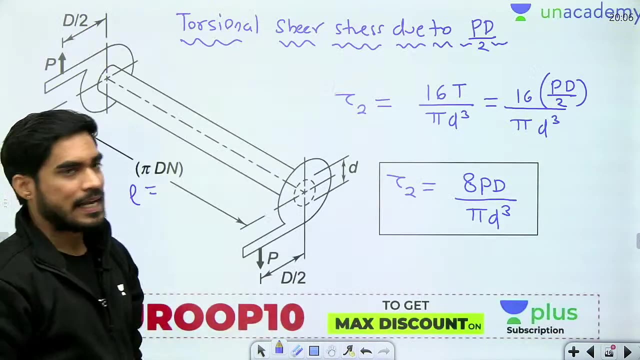 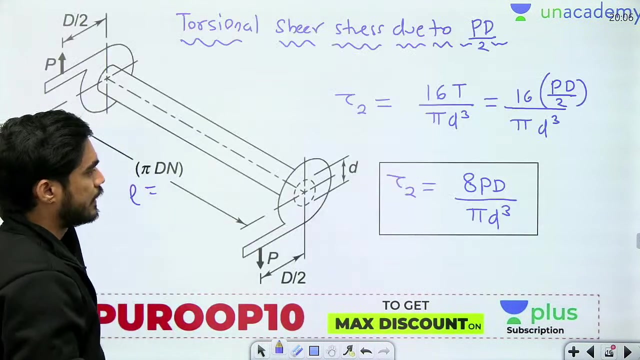 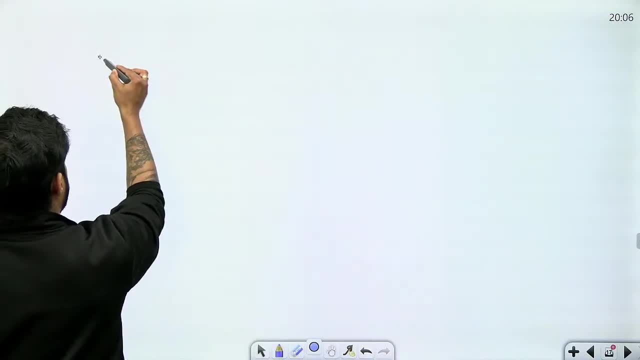 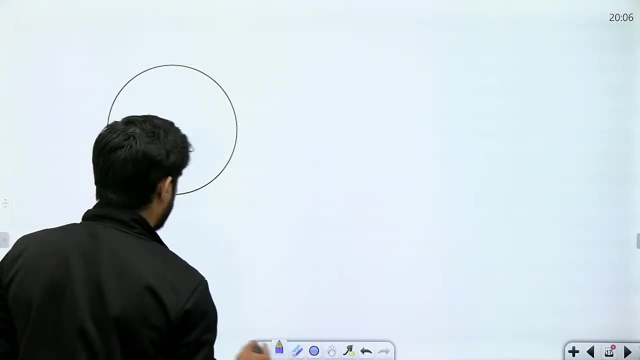 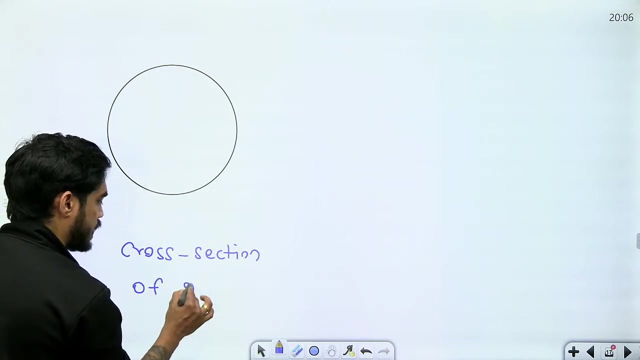 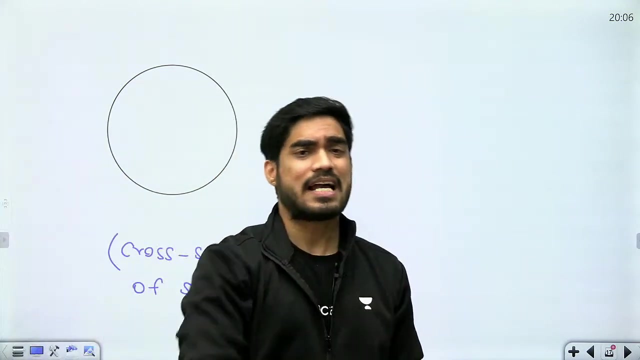 shear stress understand. let's say: this is the cross-section of the spring. tige maan lo ye spring ka cross-section hai. let's say this is the cross-section of the spring. ab jo mein concept batane wala hoon bahut mazidar concept hai aur bahut kam jaga explained hai. it is explained in very 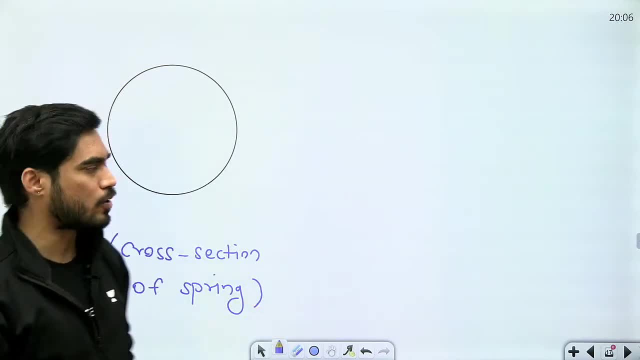 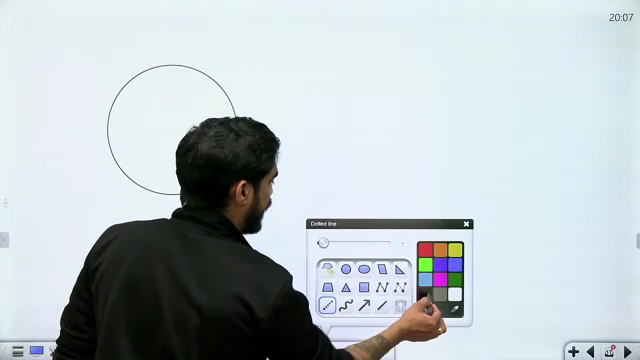 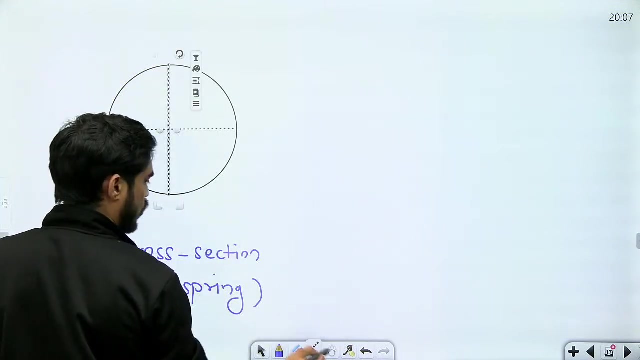 rare books. you will not find this explanation in every book, okay, so understand this very carefully. okay, understand this very carefully. let's say this is my cross-section. okay, now understand. there are two shear stresses, one due to P and one due to PD by 2. okay, my P is: 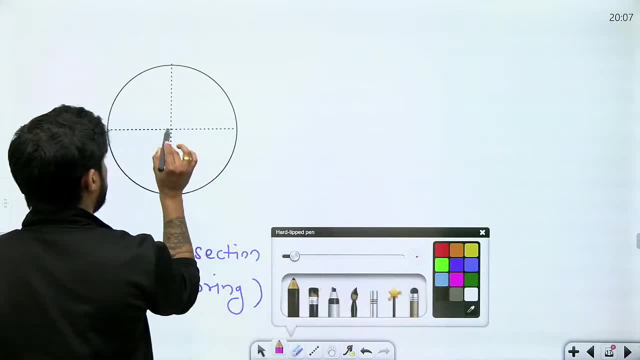 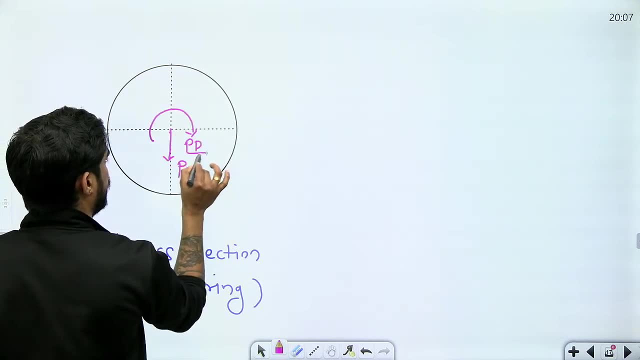 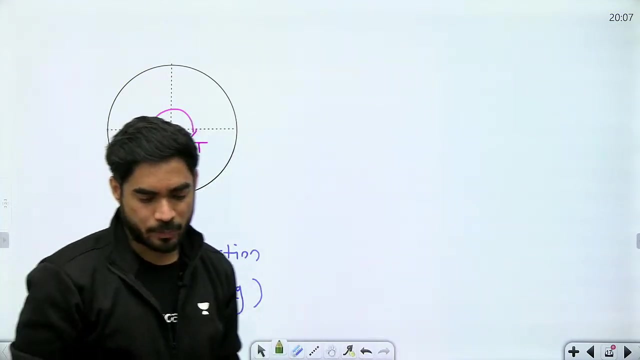 acting like this, my P is acting like this and my PD by 2 is acting like this. right, and instead of PD by 2, I will write it P as P as tornado. my torque is acting like this. okay, so I am getting shear stresses, Tau 1 and Tau2. now I want to calculate the total shear stress. 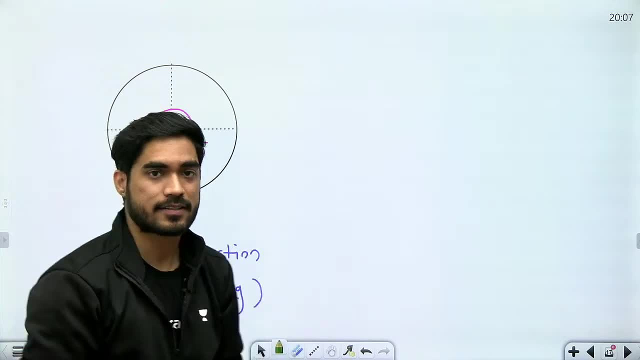 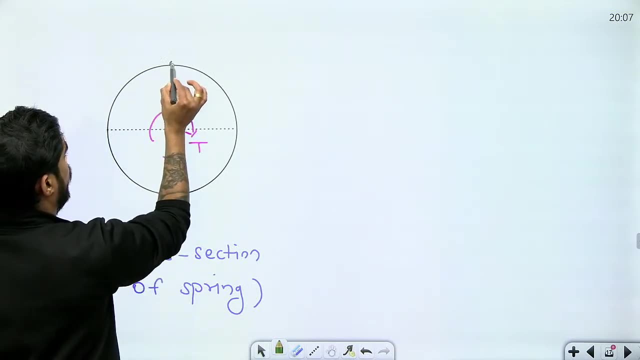 there are two shear stresses: Tau 1 and Tau 2. I want to calculate the total shear stress. so, in order to calculate the total shear stress, in order to explain the calculation, I will consider four points: a, b, b and b a and t d te. I have written four points and if I write, 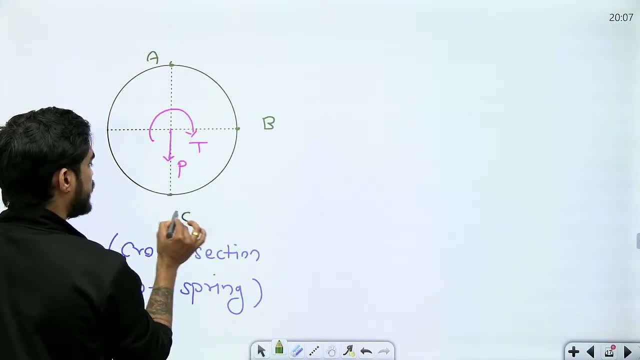 sas, so several points: a sas dressed to t y and d a c and d a c. after per point place. give three points, two points l plus n minus s. now what you should take every point you should B, C, D, because I cannot show the calculation at every point, So I am choosing four points. 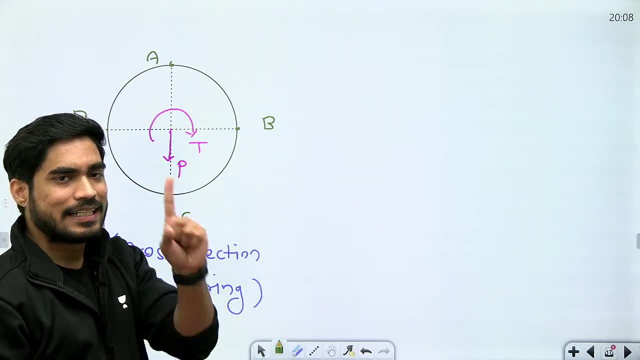 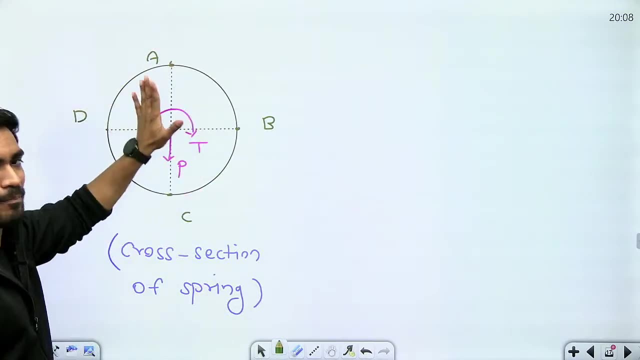 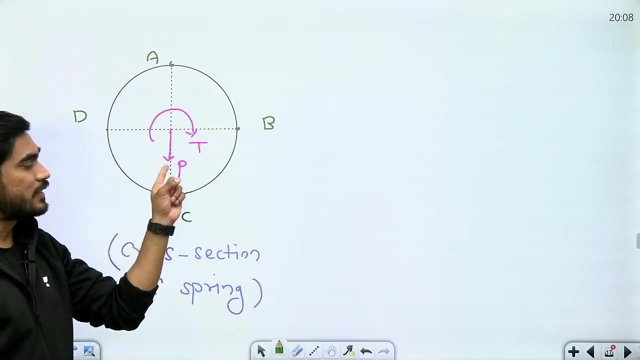 In these four points. I will first tell you the direction of tau 1 and tau 2.. Now, tau 1 and tau 2. both are acting in the same plane, They are parallel to the same plane, but their direction is different. Tau 1 is resisting the force and if you want to see the direction of stress, 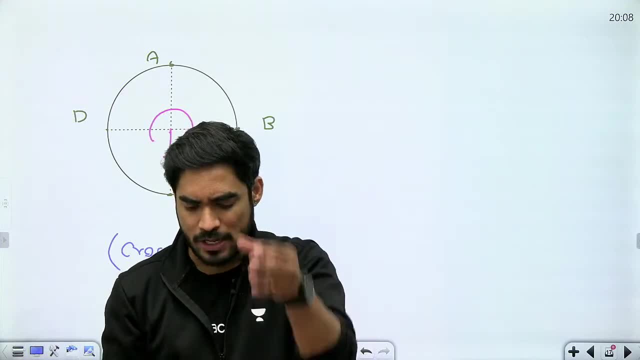 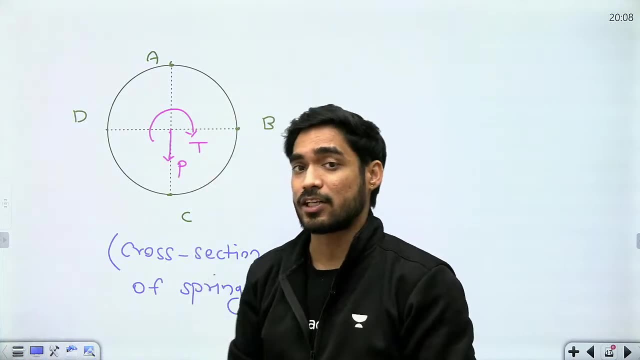 due to a force. very simple, what you need to do. I have already explained that. how to find the direction of stress due to force, how to find direction of stress due to moment, I have explained in welded joints, I have explained in riveted joints. So, my brother, 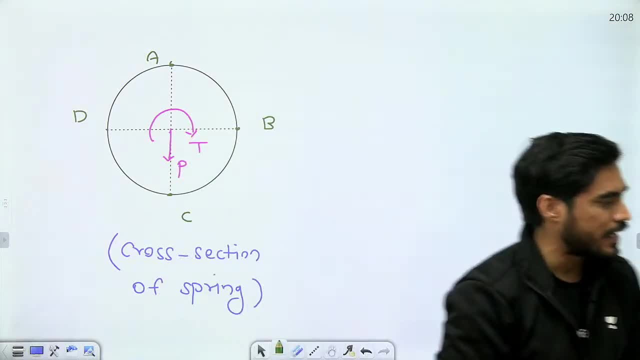 it is very important for you to know this explanation. Let me connect it with the charger. Let me connect my laptop with the charger. Let me connect my laptop with the charger. Let me connect my laptop with the charger Because I am seeing your live chat in the. 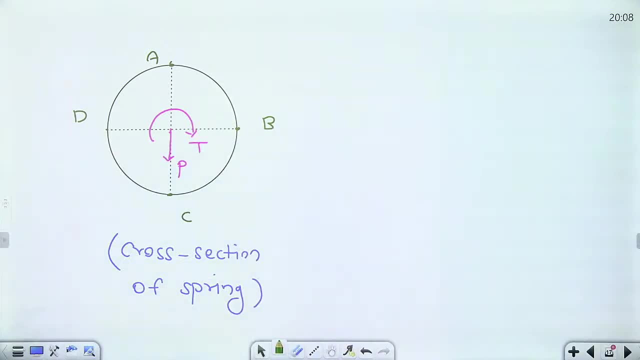 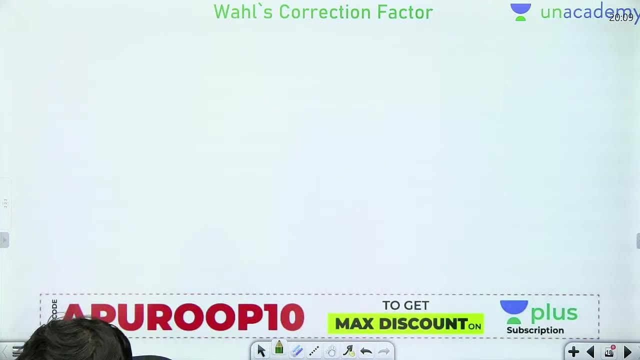 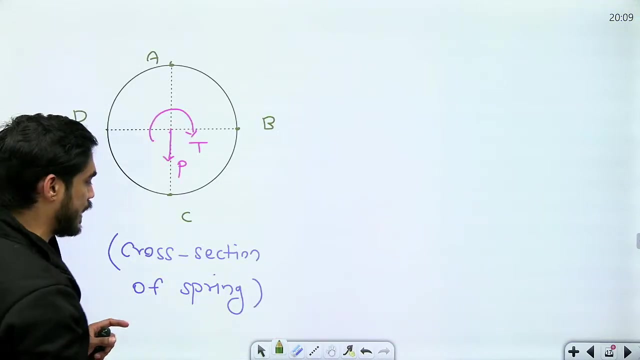 laptop. So, my brother, if the laptop will be switched off without charger, then I will not be able to see your live chat. Okay, Thank you so much for your patience. Okay, We are back online Now. how will the direction of tau 1 come? So sorry, How will the direction? 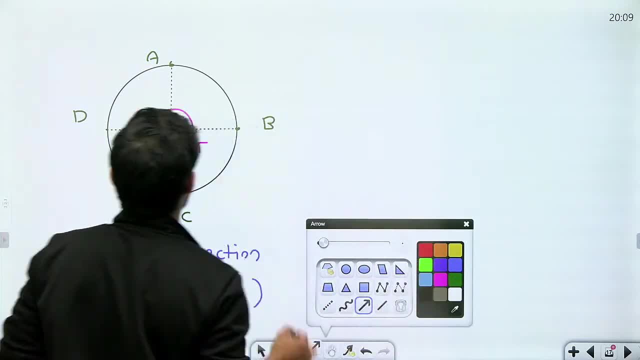 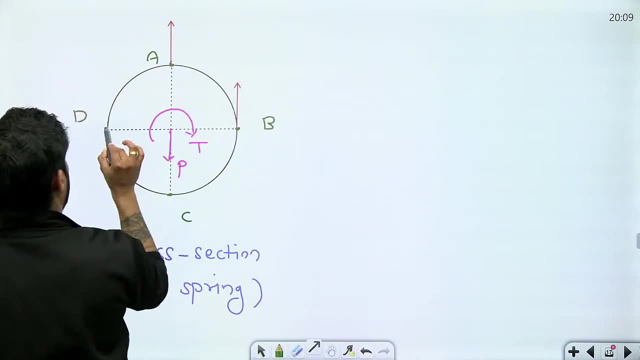 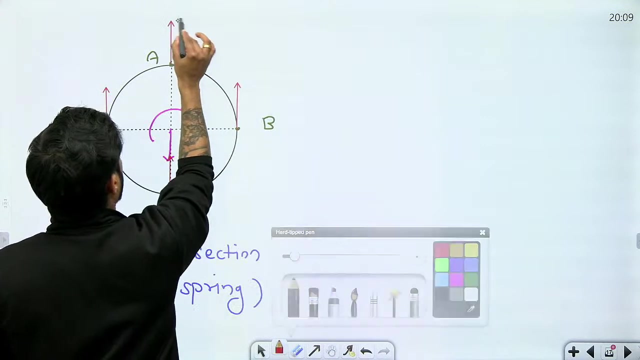 of tau 1 come Very simple. I have explained to you thousands of times. The direction of tau 1 will be like this: We can easily find the direction of tau 1.. Tau 1 will be opposite of P, Right Tau 1. 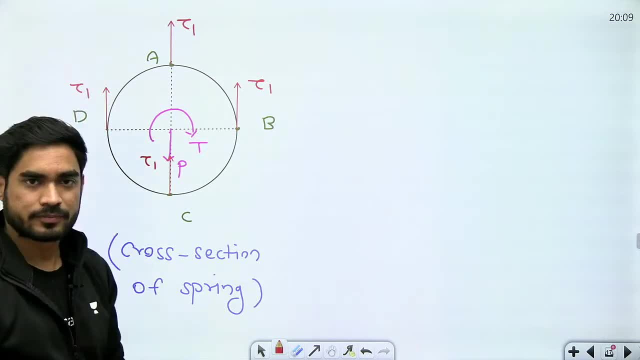 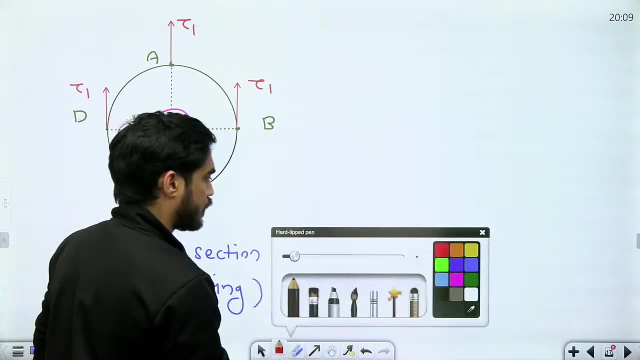 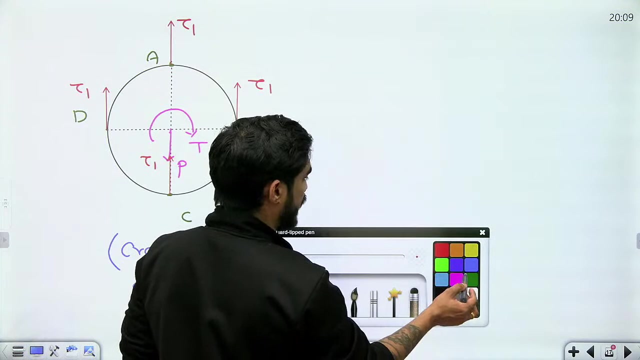 will be opposite of P. Okay, Now we will see the direction of tau 2.. Now the direction of tau 2 is a little interesting. I have also told you how to see the direction of tau 2.. Now I will explain the direction of tau 2 in a little different color. Now I will explain. 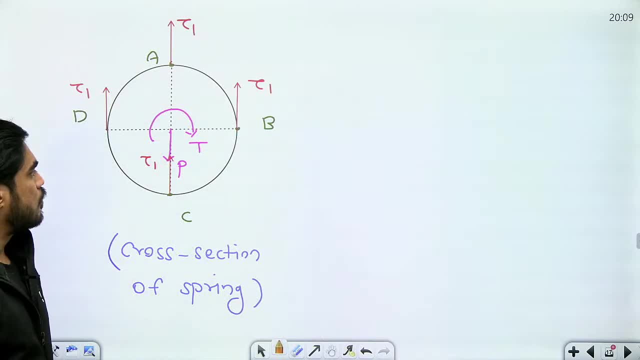 the direction of tau 2 in a little different color, So I will use this color. Okay, Now tau 2's direction. at A, if I want what I will do, I will connect A with the center. So I am getting a vertical line. Tau 2 will be perpendicular to this vertical line, If you. 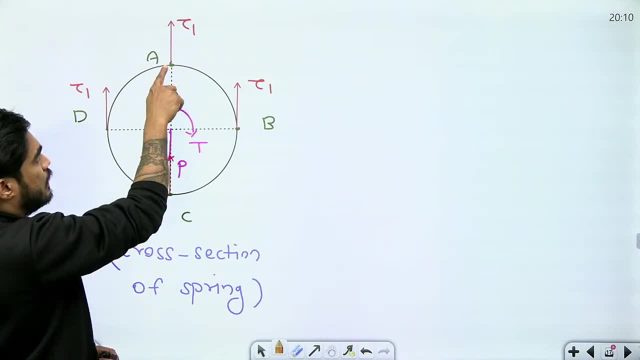 want to see on A, then connect A with the center And tau 2 will be perpendicular to this line. Now that perpendicular will be like this, It can be like this: T is acting clockwise, So tau 2 should be perpendicular to this line, So I am getting a vertical. 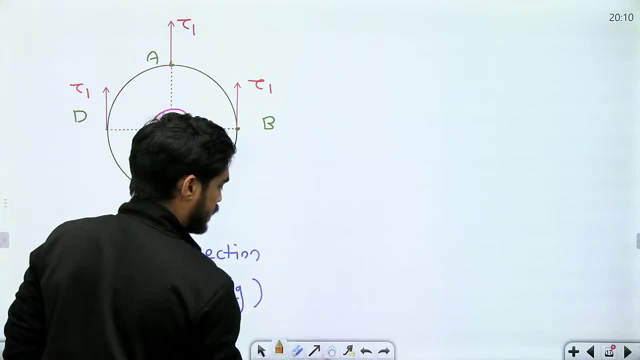 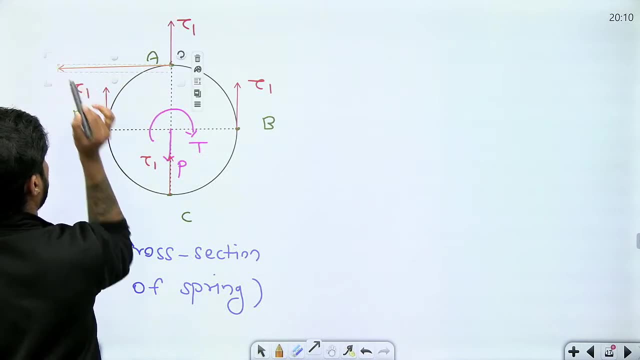 line T is acting anti-clockwise. So my brother, tau 2 will be like this: Okay, Tau 2 will be. tau 2 will be like this, Like this: Its magnitude will be very high compared to tau 1.. So that's why I am using very long arrows. So this is my tau 2.. Similarly, here it: 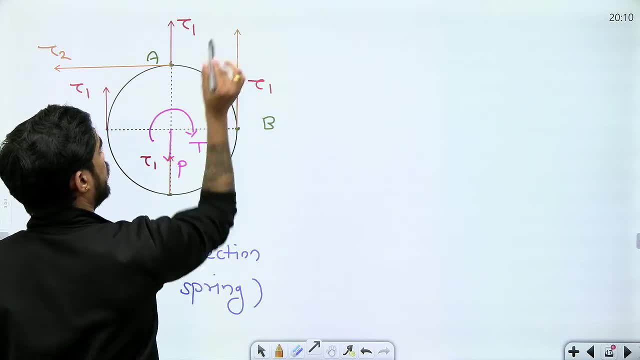 will be perpendicular to this line. anti-clockwise, So it will be like this: Okay Here. anti-clockwise, it will be like this: Okay, So, it will be like this. Okay, So it will be like this. 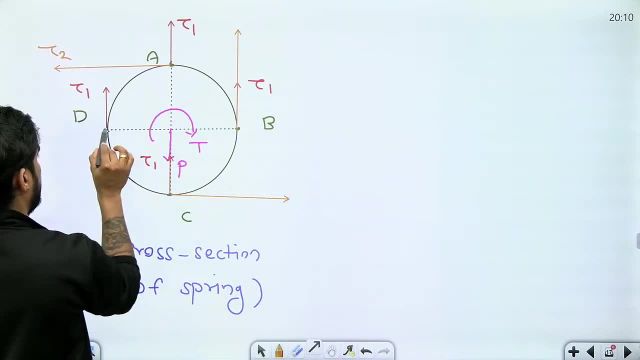 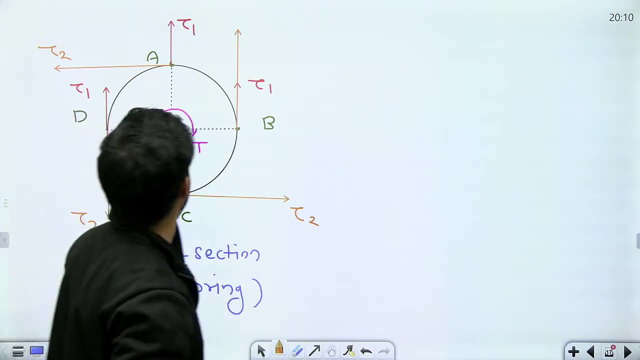 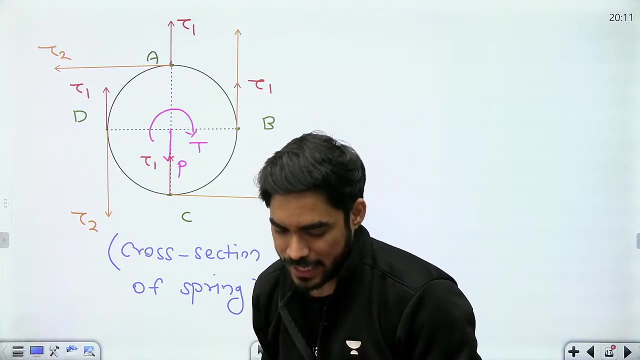 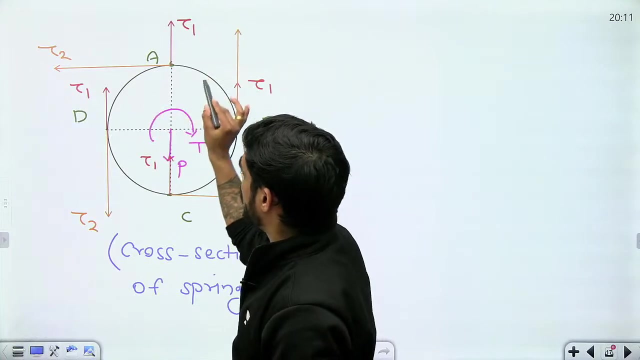 And here anti-clockwise, it will be like this: Okay, Now I have shown you the directions of tau 1 and the directions of tau 2 at every point. I have shown you the direction of tau 1 and tau 2 at every point. Now you can see at different points what is the direction. 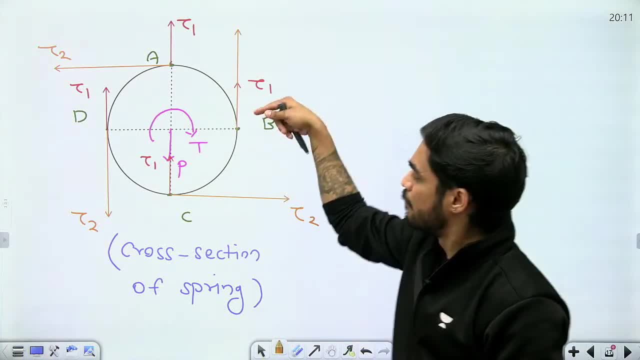 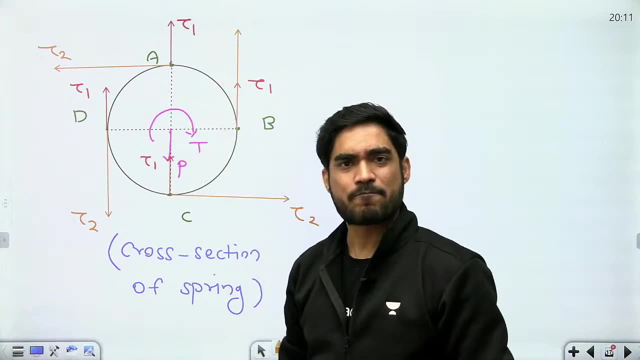 of tau 1 and tau 2.. Right, So tau 1 will always be upward, but tau 2 will be perpendicular to the line joining that point and center. Now, in all these points, where is the most resultant? There you will. 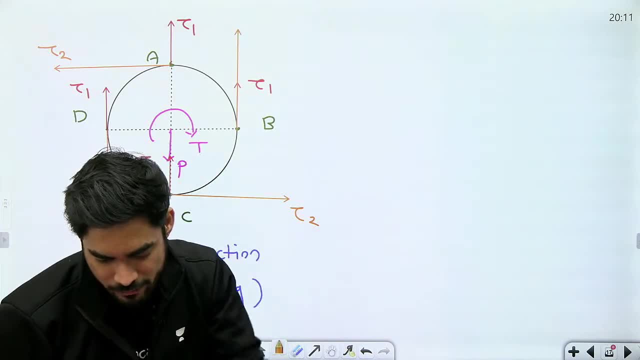 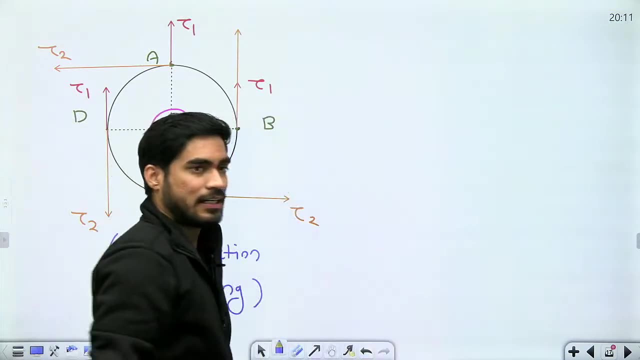 get the maximum resultant. Yes, Very good, Jitendra, Very good, Very good, Very good. So, my brother, the most resultant is going to come at B point. So, son, do you understand what will be the resultant shear stress? Maximum resultant shear stress. Now, son, in lots. 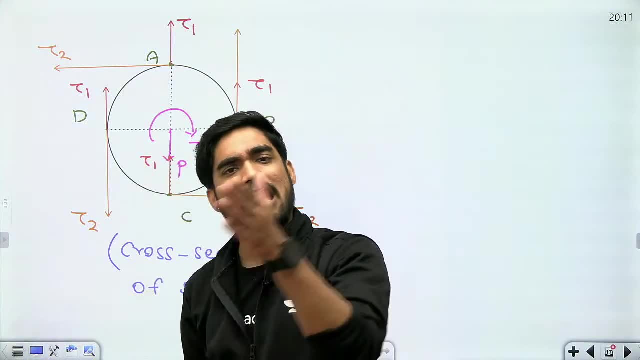 and lots of books, you will get the resultant shear stress Now, son. in lots and lots of books you will see that they will directly add tau 1 and tau 2.. They don't explain why they are adding tau 1 and tau 2.. They don't explain why they are adding tau 1 and tau. 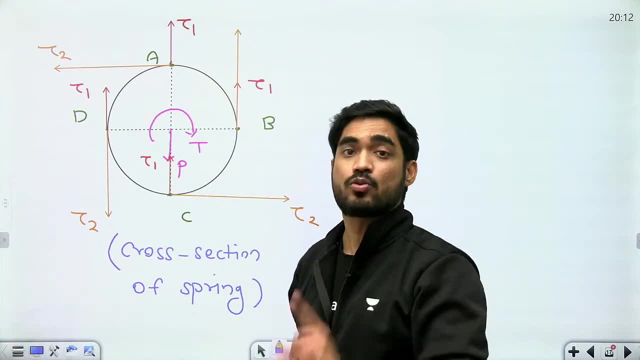 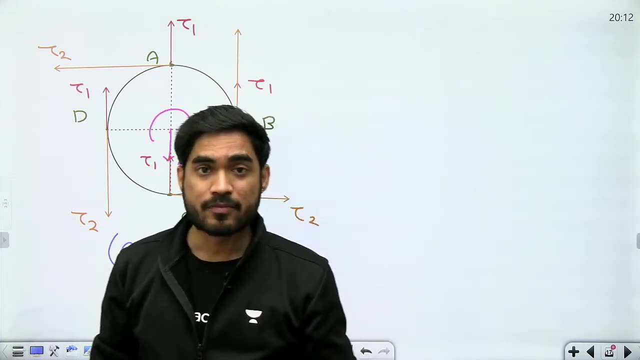 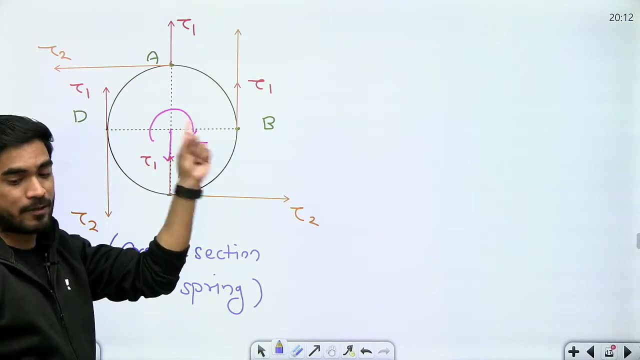 2. My brother, tau 1 and tau 2 will not be added at every point. It will be added at one particular point only And at that point you are going to get tau maximum. At other points tau will not be maximum. At this point B only tau is going to be maximum. Okay. 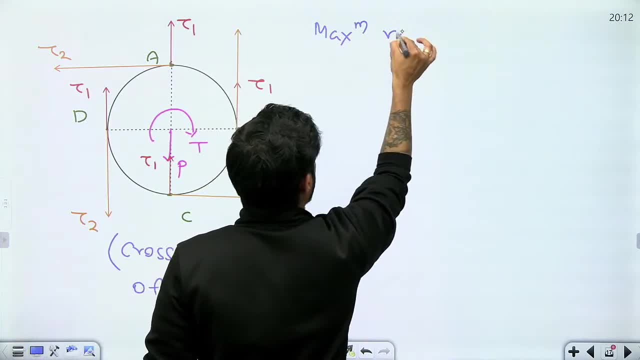 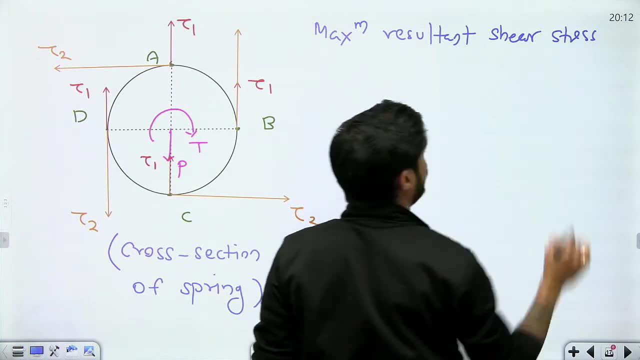 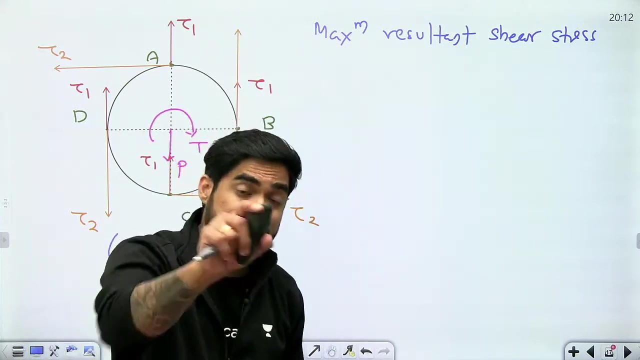 So maximum shear stress, Maximum resultant shear stress should be written: Maximum resultant shear stress. Now, my brother, there is a debate on this too. A lot of students ask me, sir, stress is a tensor quantity, Then why you are taking resultant? I have already explained. 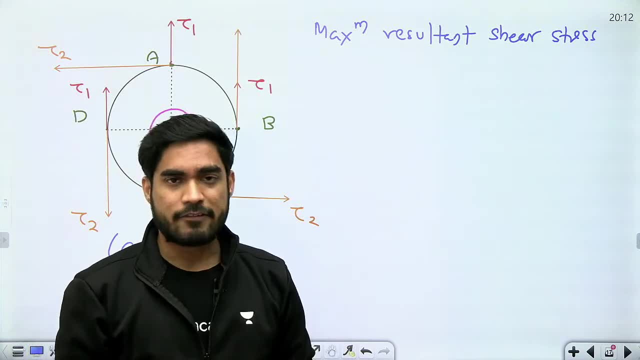 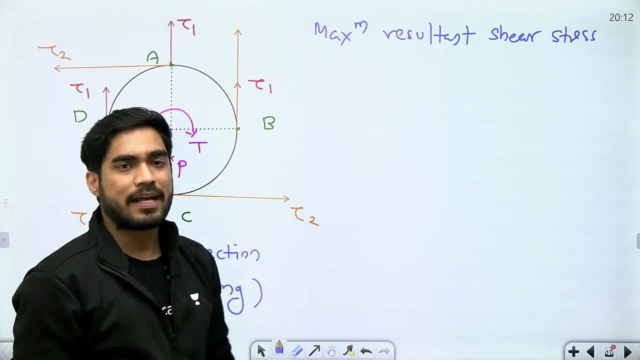 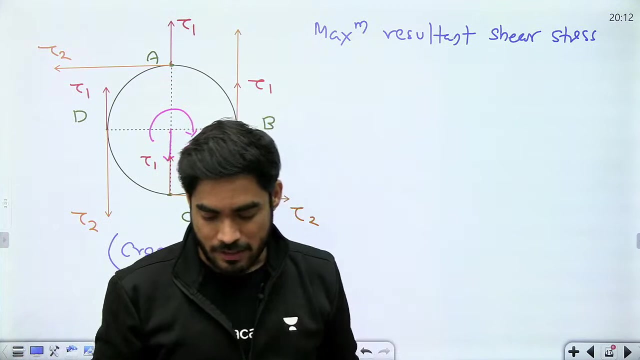 this? Yes, stress is a tensor quantity. So if the stresses are acting in different plane, if one stress is in this plane and another stress is in this plane, you can't take the resultant. But these two stresses are in the same plane, So I can consider them as vectors Then. 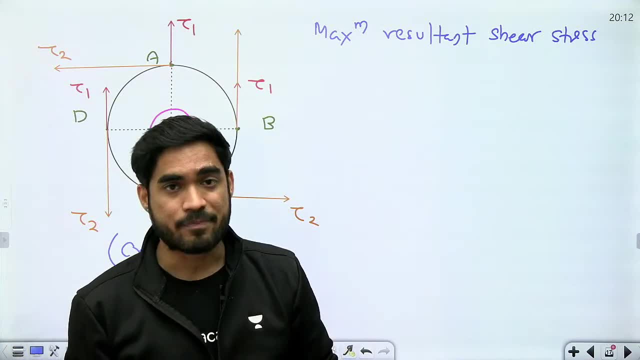 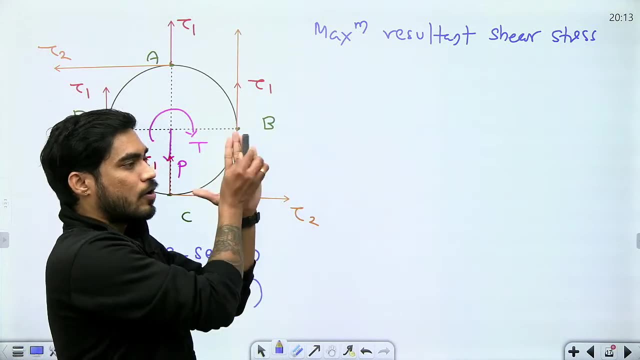 I can consider them as vectors, Then I can consider them as vectors. Okay. So that's why you can't take resultant of sigma and tau, Because tau's arrow is in a different plane and sigma's arrow is in a different plane. Right Tau's arrow is in a different. 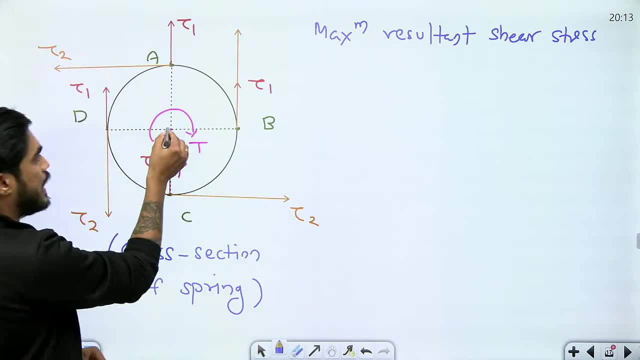 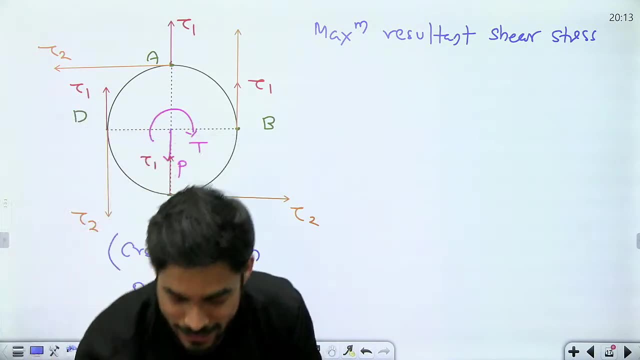 plane and sigma's arrow is in a different plane. If sigma is added here, then it will be like this And it will be in this plane. This arrow will be in this plane. So that's why you can't take resultant of sigma and tau. But my brother, both tau's are in the 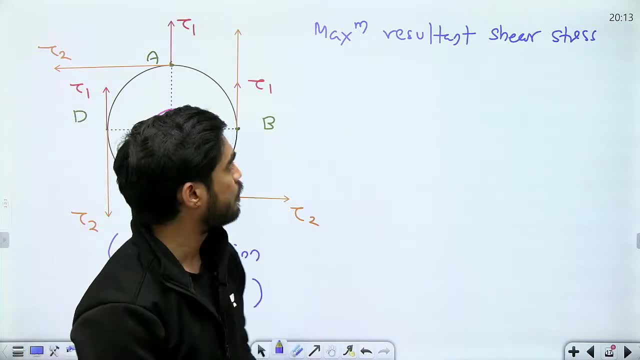 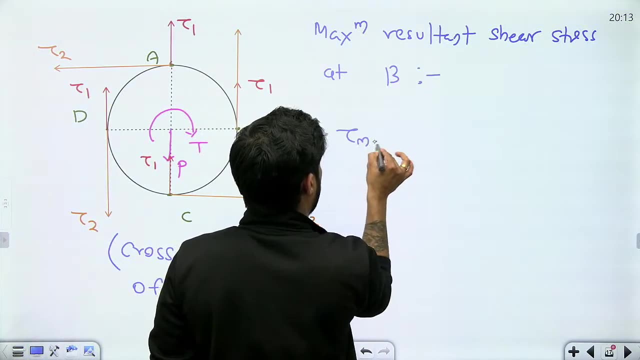 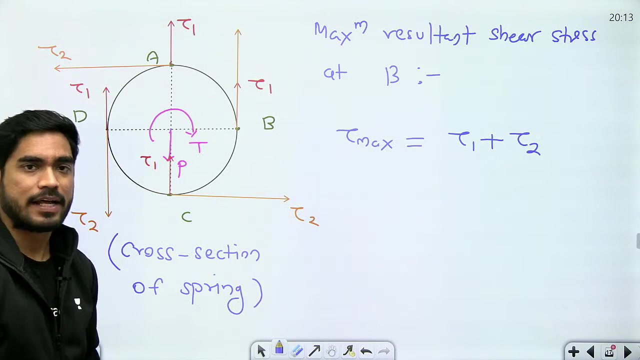 same plane. So then we can take the resultant of them. Okay, So maximum resultant shear stress at B. tau maximum will be equal to what Tau 1 plus tau 2.. Okay, Tau maximum will be equal to what Tau 1 plus tau 2.. Now I want you to put the values of tau 1 and 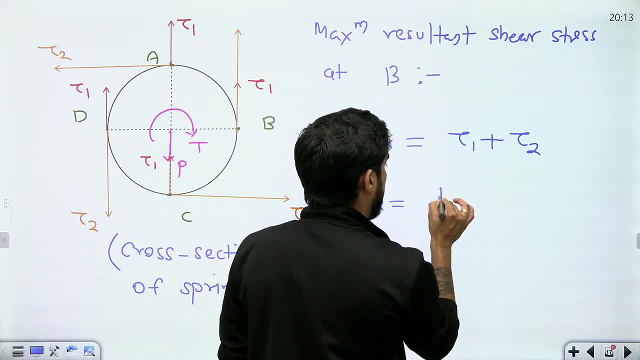 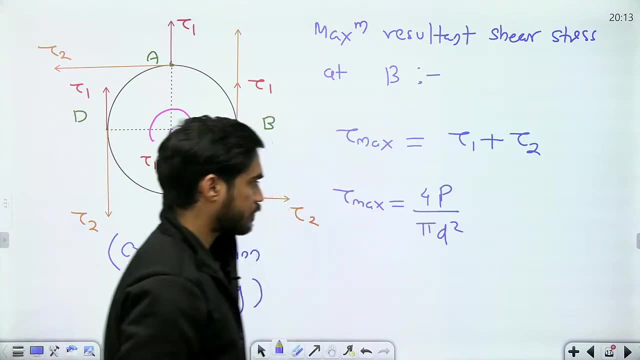 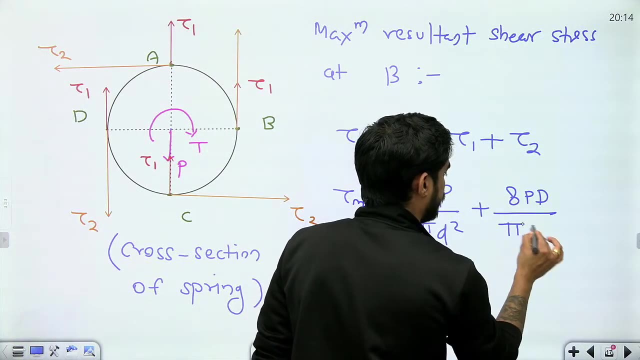 tau 2 in the equation. So what is tau 1, my brother? Tau 1 is P upon pi by 4D square. So can I write it 4P upon pi D square? I can write it 4P upon pi D square plus. this is 8P D by pi D cube. Now what I want you to do is: 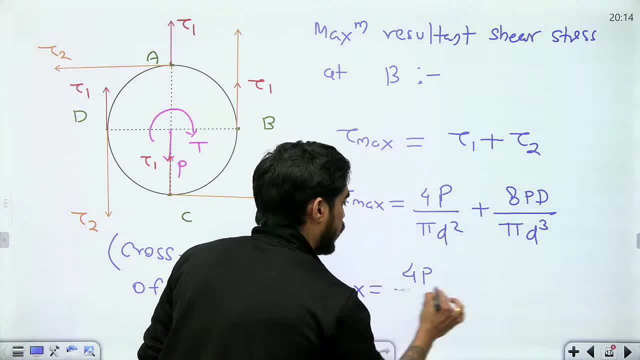 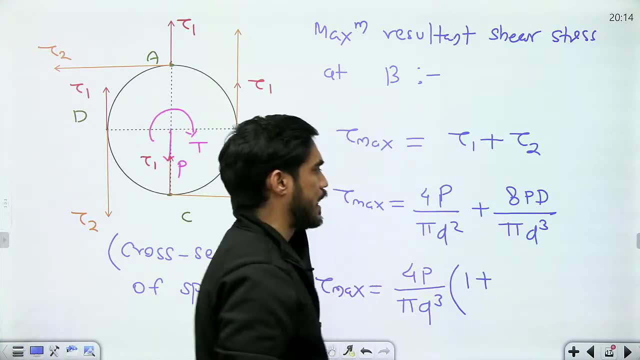 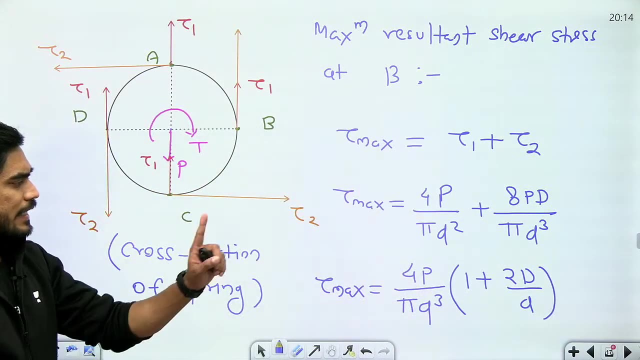 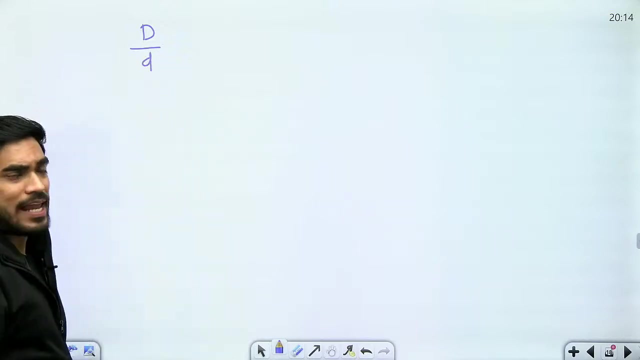 I want you to take out 4P upon pi D square out of this equation. So this will become 2 into capital D by small d. Right Now, my brother, pay attention to one thing here. Okay, The value of capital D by small D is very, very high than 1.. Capital D by small D is: 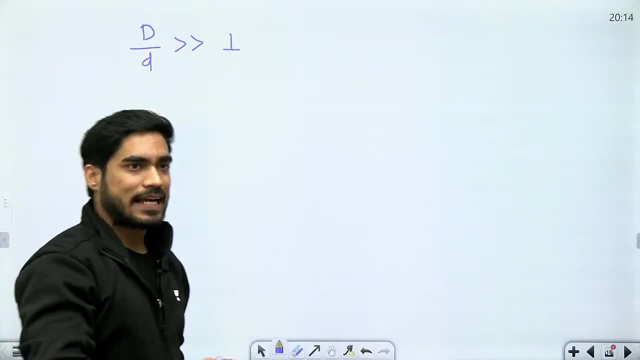 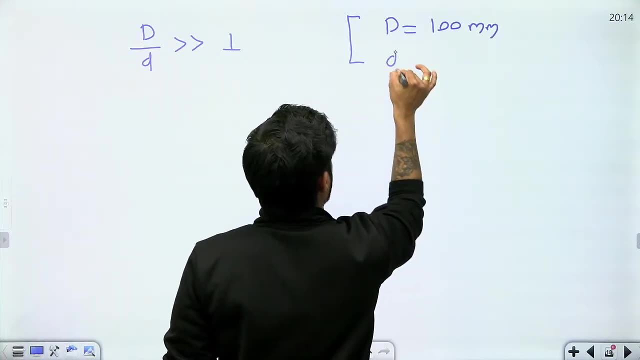 much higher than 1.. So take one example: Capital D is near to 100mm, So capital D is very close to 100. That means capital D is much higher than 1.. So this is equal to capital D by small d. Now what is 0. This value is going to be 0. That is pi by 1.. Now 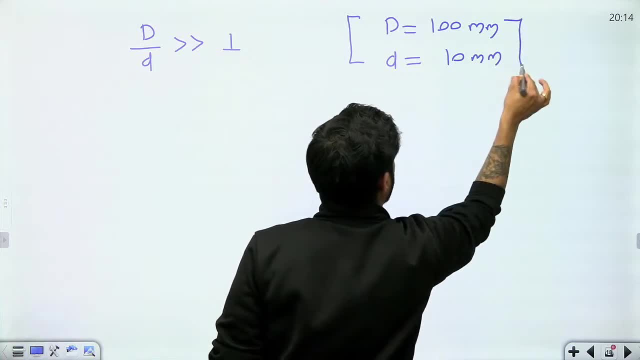 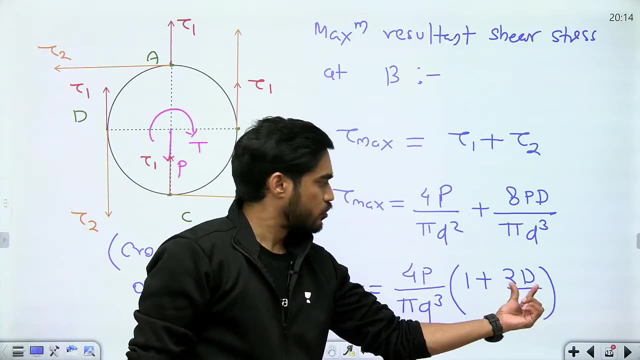 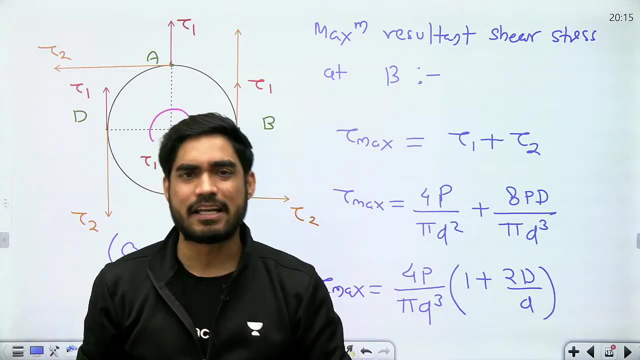 And small d is around 10 mm. So what will be capital D by D, It will be 10.. So this will become 20.. So if I add 1, it will become 21.. Now is there a very big difference between 20 and 21?. 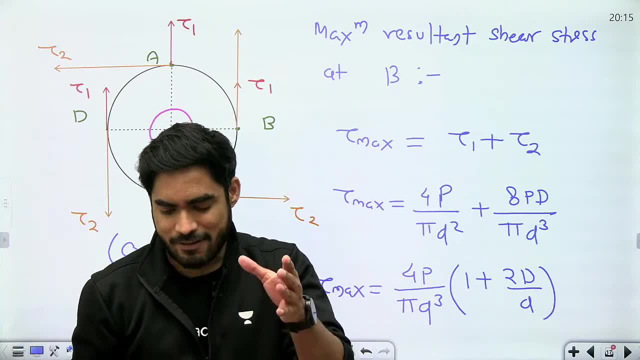 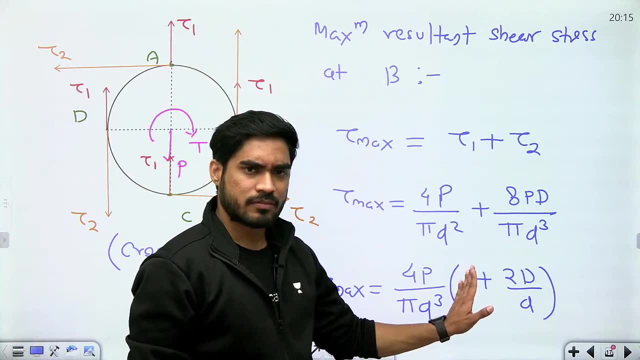 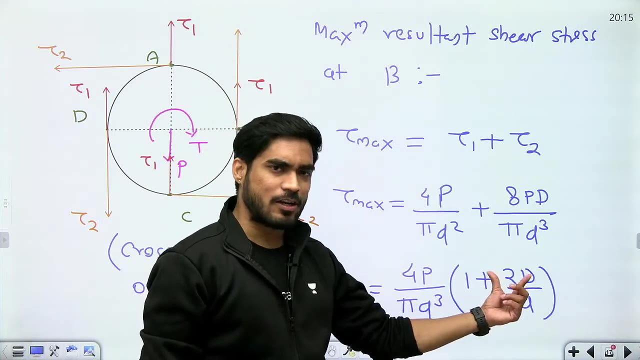 Is there a very big difference between 20 and 21?? Is there a very large difference between 20 and 21?? No. Now, even if you ignore this 1, the value will almost be same. Even if you ignore this 1, your equation will almost remain same. 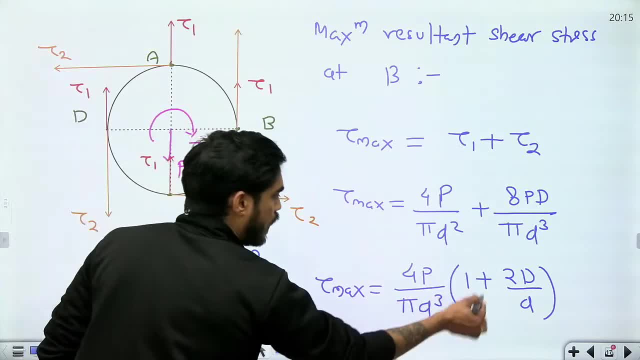 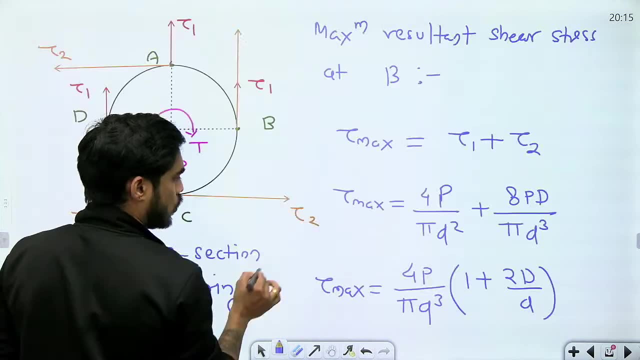 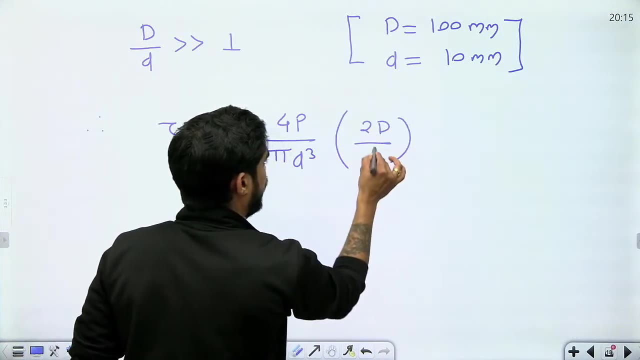 So can I ignore this? Can I ignore this? Can I ignore this 1?? So neglecting this 1,. can I write: tau maximum equals to 4p upon pi d, cube 2 into capital D by small d. So how much is tau maximum, my brother? 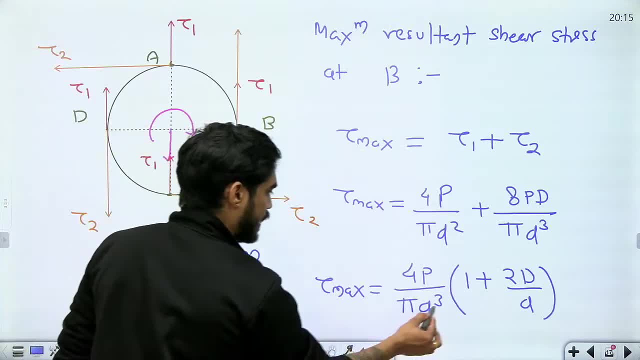 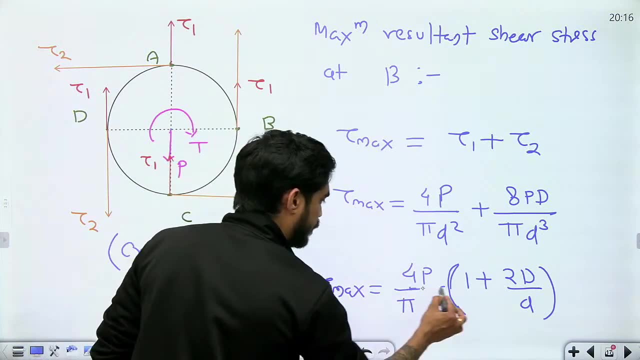 8pd by pi d. Sorry, here pi d square should come. Okay, I should write square. I should write square. Now someone will say in live chat- surely there will be a chaos here- That there will be square. 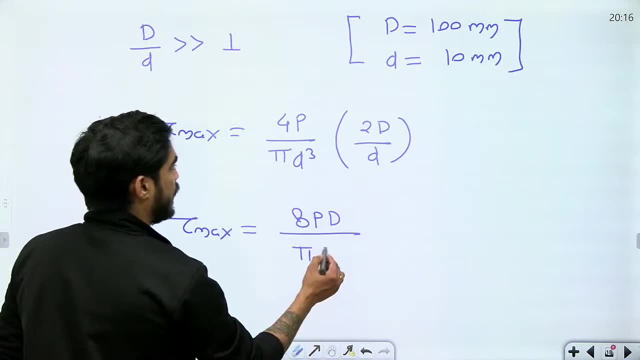 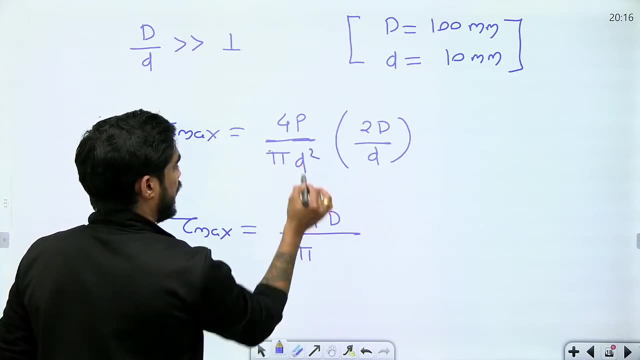 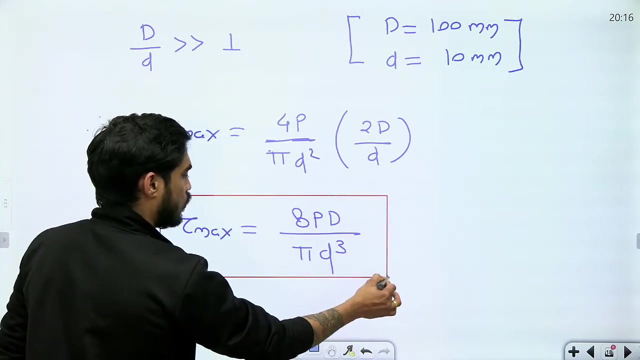 Yes, there will be square. So my brother here, 8pd by. he should have written square. Can I write this: 8pd by pi d cube. Now my brother, look at this equation. You will say that, sir, direct shear stress is gone. 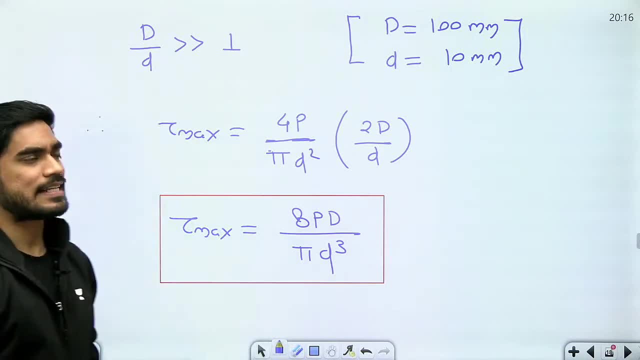 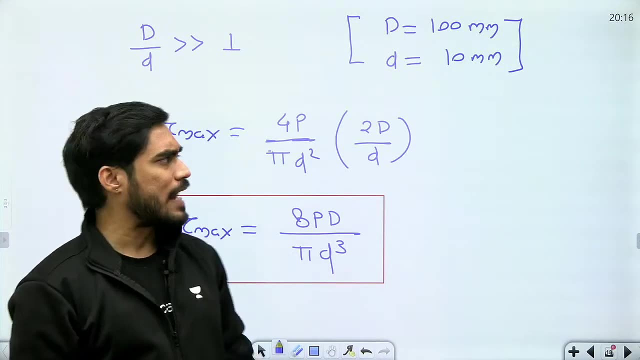 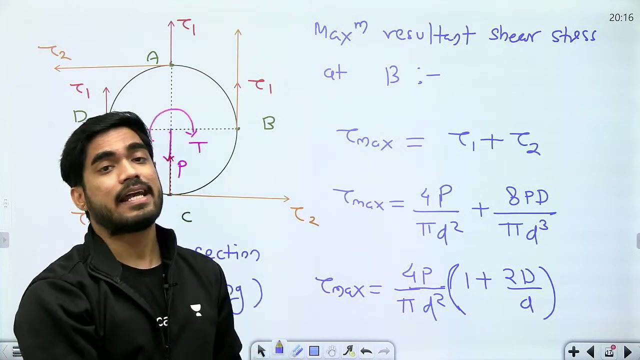 Sir, direct shear stress is gone. Yes, direct shear stress is gone. Now you will say, sir, you directly say that neglect direct stress. I might have directly told you that direct shear stress should be neglected. But, son, I wanted you to understand why we can neglect direct shear stress. 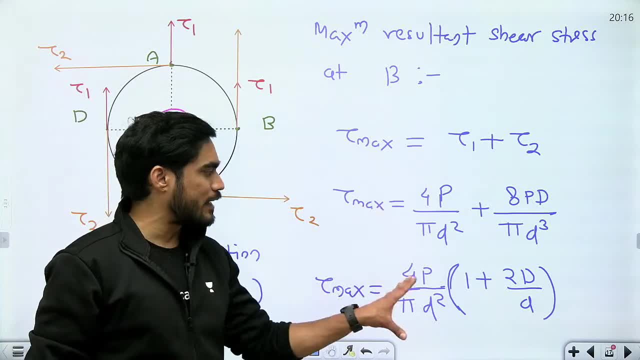 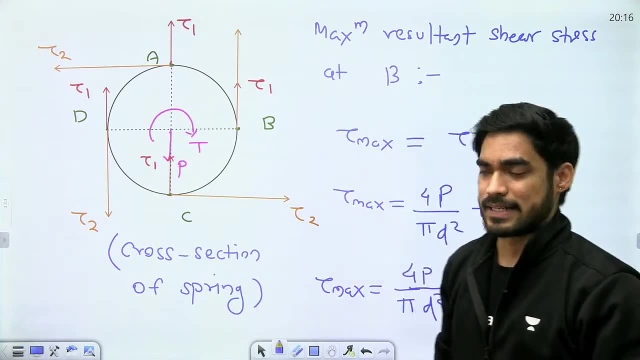 I wanted you to understand why we can neglect direct shear stress. You have to understand mathematically that by neglecting direct shear stress, why this equation will not create much difference. Okay, That you need to understand. That's why I explained this concept. 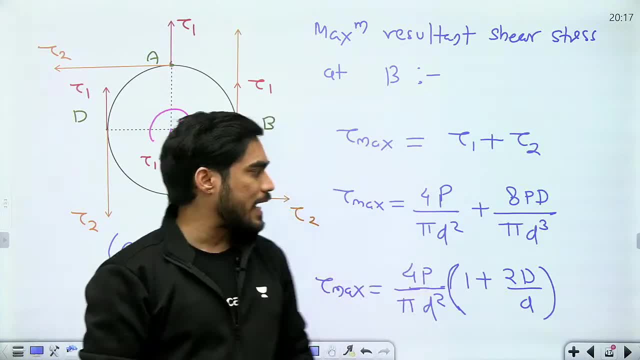 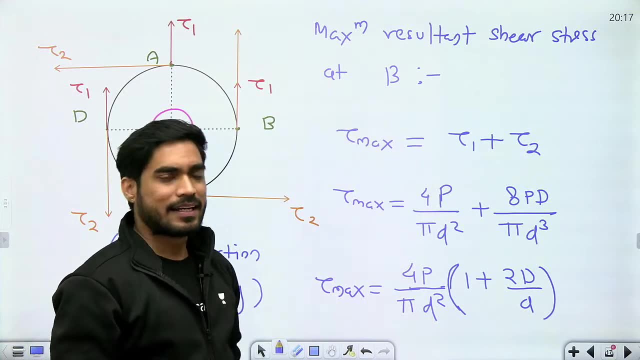 Okay. So my brother, mathematically we have seen that even if I neglect this quantity, even if I neglect this quantity, there will be not a much difference. Now you must be thinking, sir, why neglecting this, Calculating this is such, so simple. 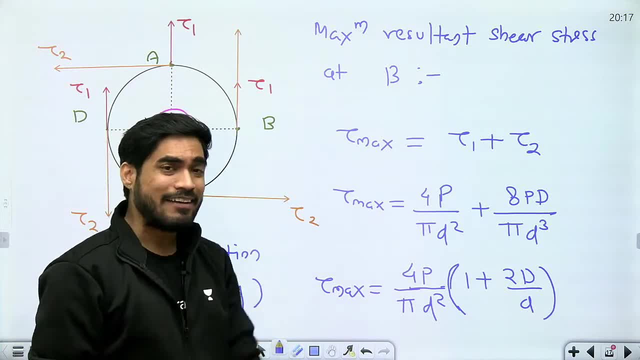 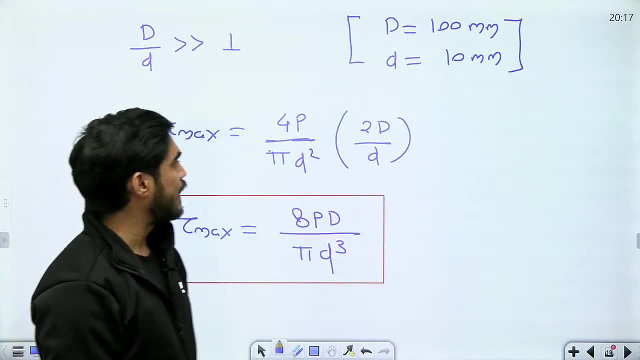 Right, Son. but you are forgetting one thing: Here we are designing the spring. Designing the spring means you don't know right now what will be the value of capital D and small d. Let's say, I give you one value. 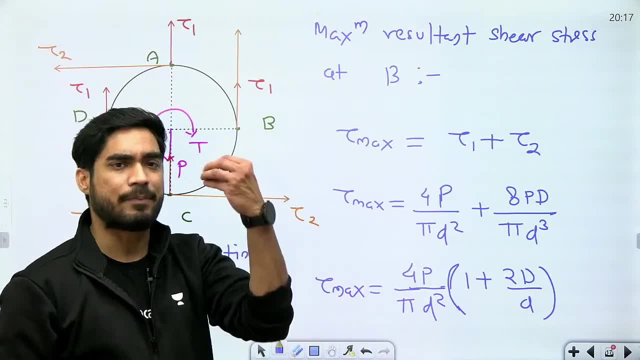 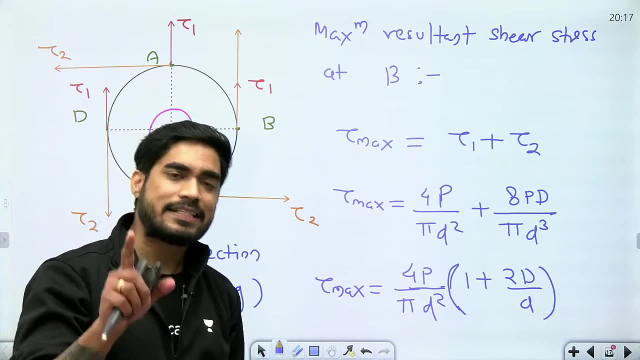 Let's say: let's say I give you capital D, Let me give you capital D. Let's say small d is unknown. Let's say small d is unknown. So, son, in the design of spring, actual design, practical design of spring, I will not know. 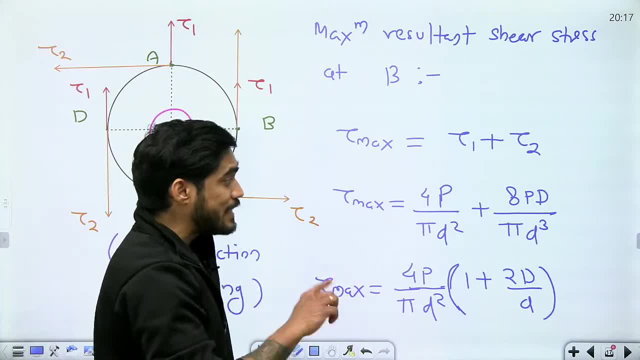 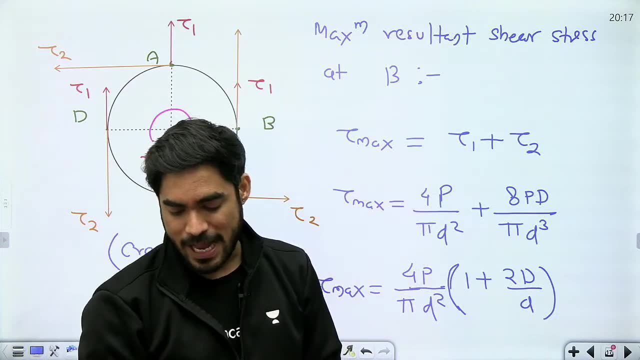 what will happen? I will not ask you to calculate tau max, I will ask you to calculate small d. I will give you tau max and I will ask you to calculate small d. Now, my brother tell me one thing. Now, my brother tell me one thing. 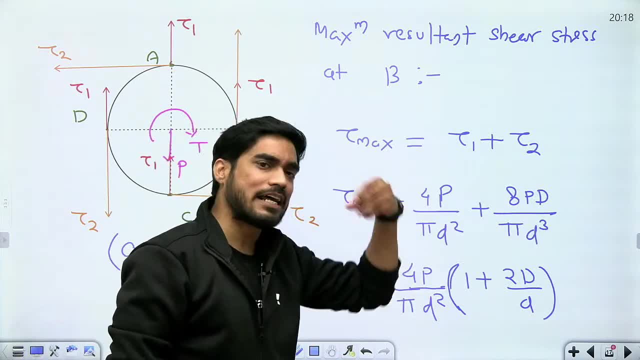 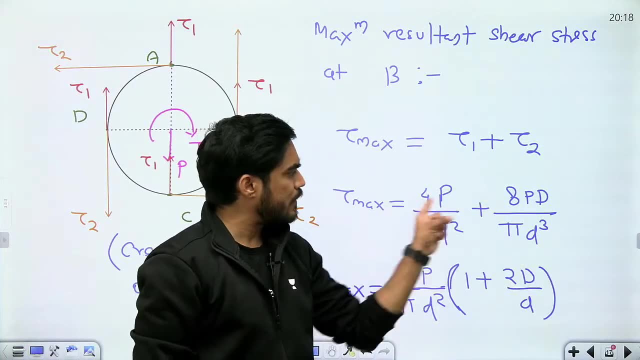 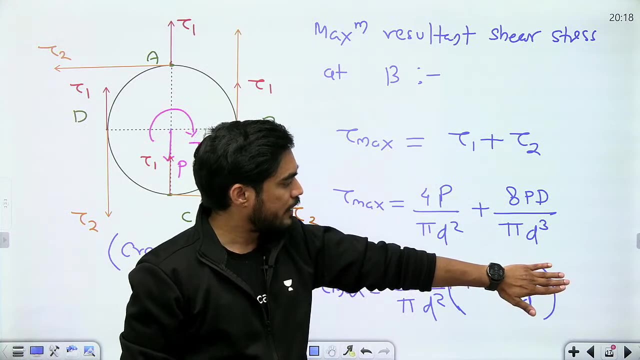 If I give you tau max and if I give you all the other values and small d is unknown, can you solve this equation easily? Can you solve this equation easily If I give you all other values? only small d is unknown, known. look at this equation and tell me whether it will be very easy to solve this equation. it. 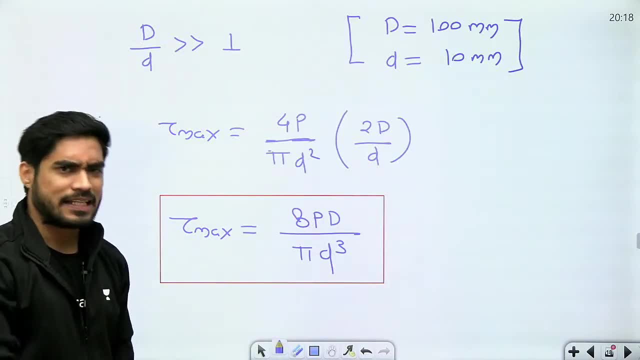 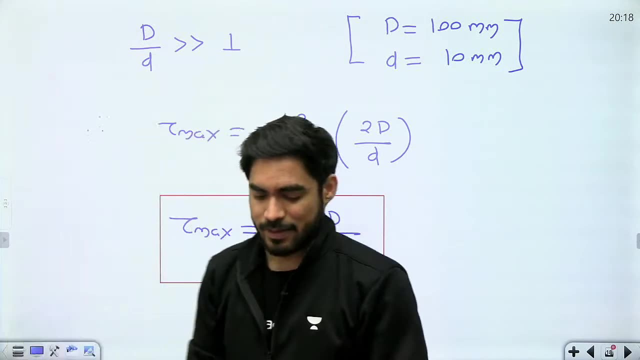 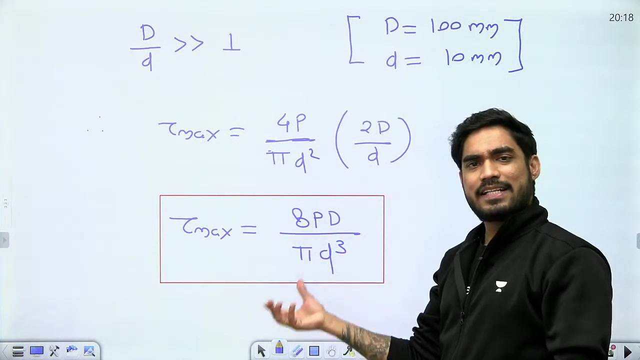 will not be very easy, but beta, if i give you all the other values and i ask you to calculate small d in this equation, it will be very convenient because beta, d cube will come here, tau max will come here. very easily you can find out d right. 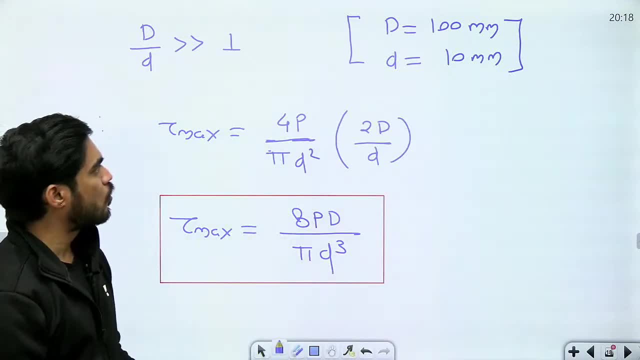 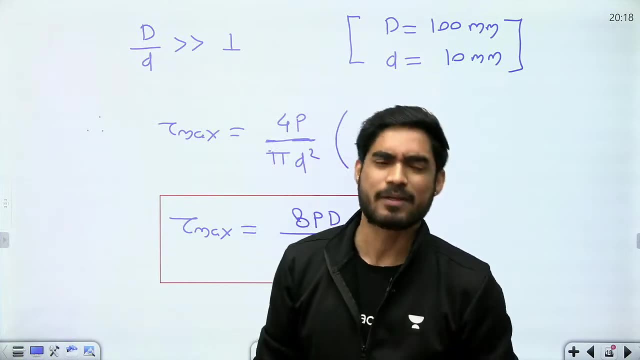 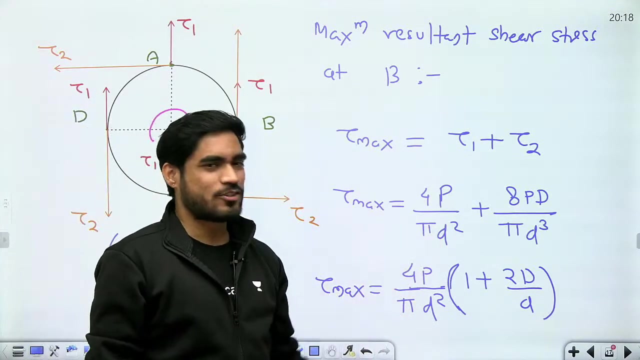 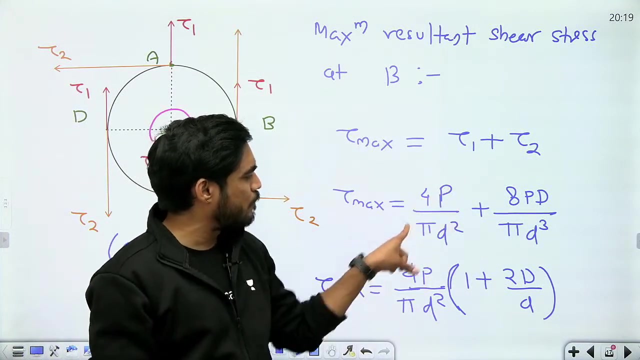 so, beta, do you understand why we need to ignore the first term and we need to simplify our equation? what is the reason behind simplification? a lot of people have asked me, of course, how easy it is. just put the value of 4 p, pi d square and you can easily get tau maximum. 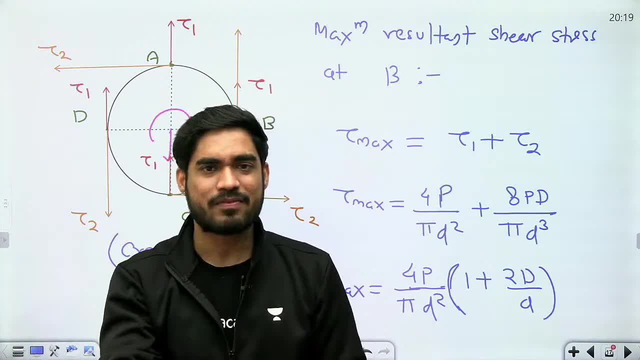 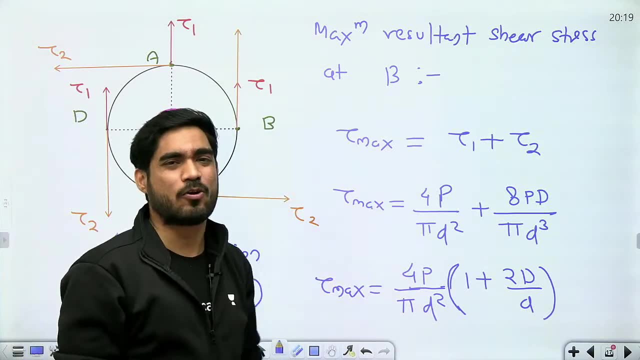 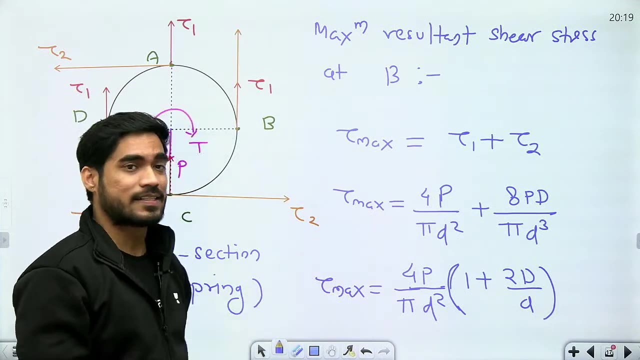 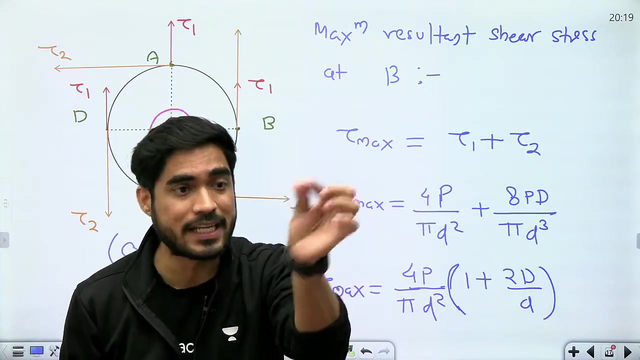 beta. when we get a question in exam there they ask you to calculate tau max, but practically in design you don't calculate tau max. so beta, you get the value of tau max. the unknown is small d. that is the unknown. small d is the unknown. and in the calculation of small d 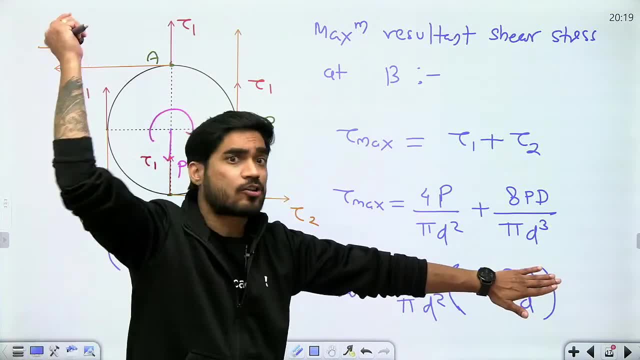 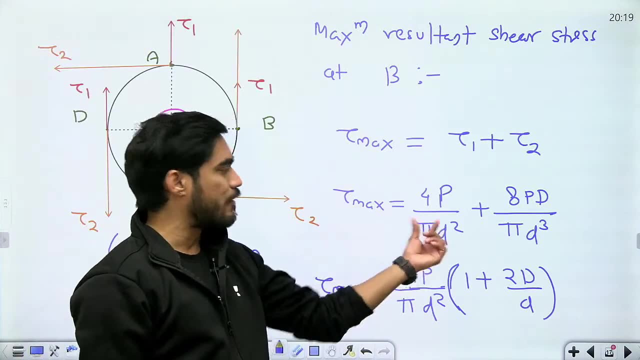 this equation will be very easy to solve, but this equation will be complicated- not that complicated, but it will be complicated. right, but this equation will become so easy, so that's why we ignore the first term. so i hope that this is very clear to you now. you will never forget the logic behind this right beta. yes. 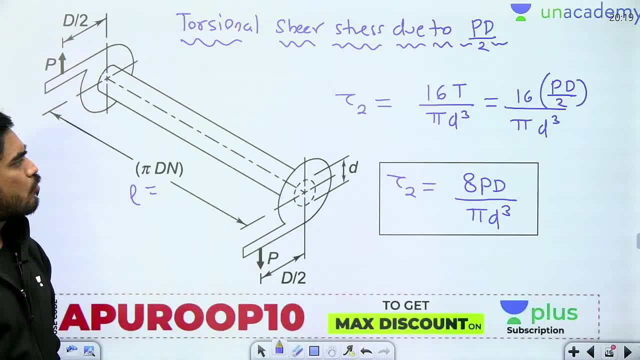 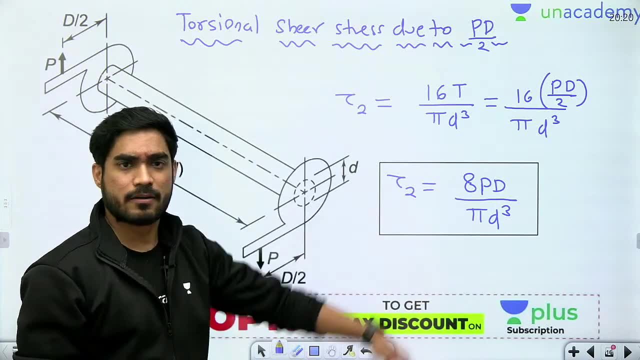 i could have said all this in one line when we got tau 1 and tau 2. i could directly write that tau 1 will be negligible compared to tau 2. neglect tau 1, use this, but beta there. you will not understand all of this. 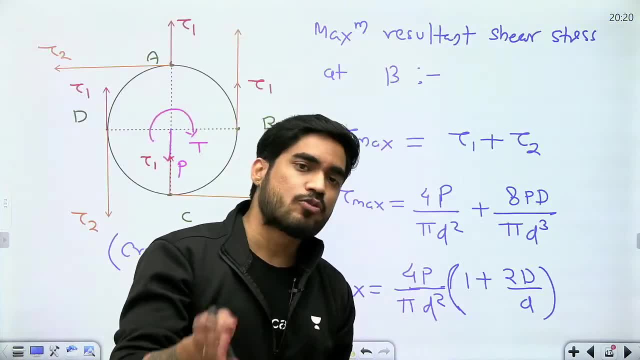 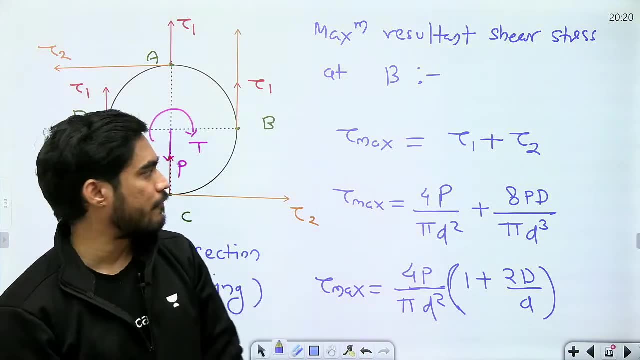 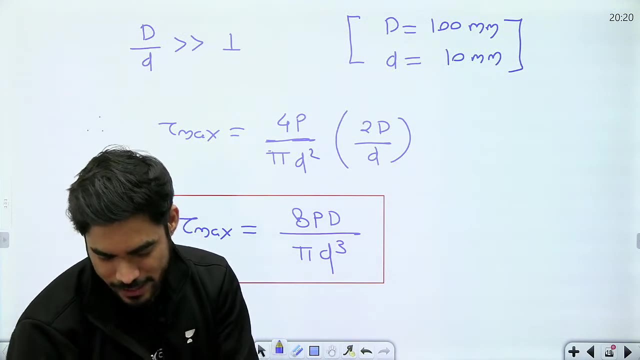 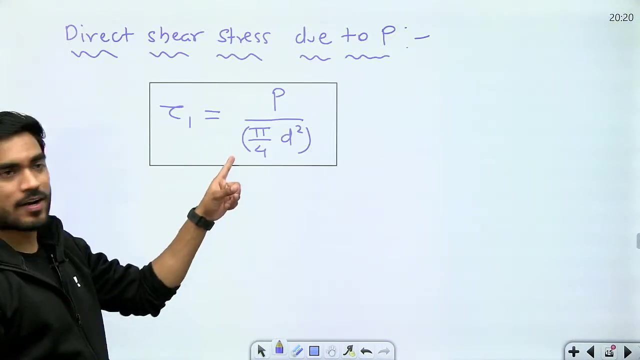 why did you neglect tau 1? exactly what? if we had kept it, then the calculation would have been very complicated. all of this, all of this you will not understand if i directly tell you. okay, so from this you might have understood, right. yes, very good, beta, very good. yes, very good, very good. so, beta. i hope that this is clear. now, beta, why i have used black boxes for them. 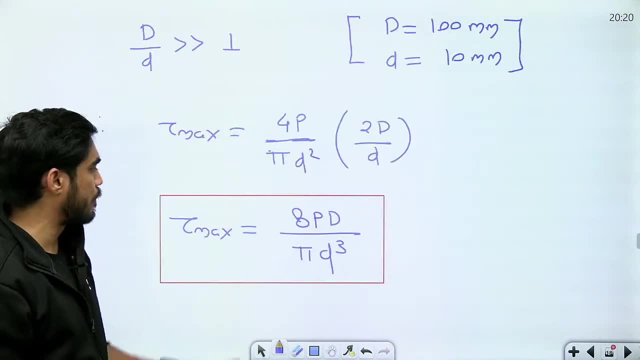 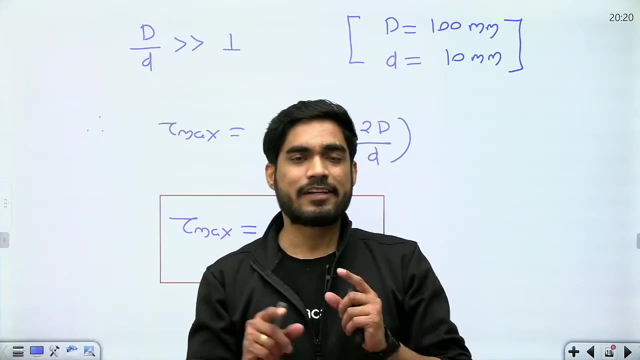 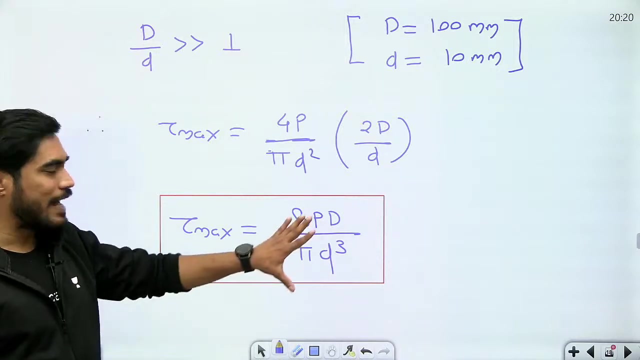 because you don't have to remember this equation and this equation. you have to remember this equation: tau max equals to 8pd by pi dq. okay, now beta in gate exam. they will not tell you that. ignore direct shear stress. they will just ask you find tau max. so beta by default. you have to use this. 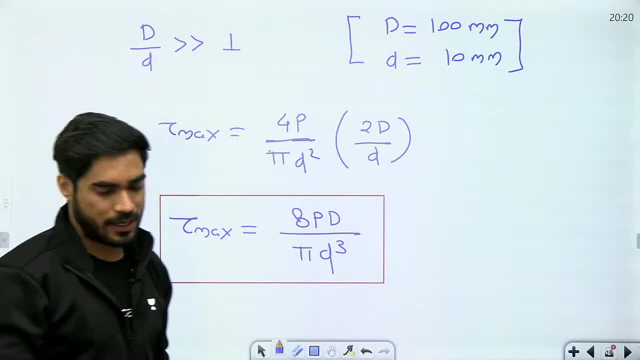 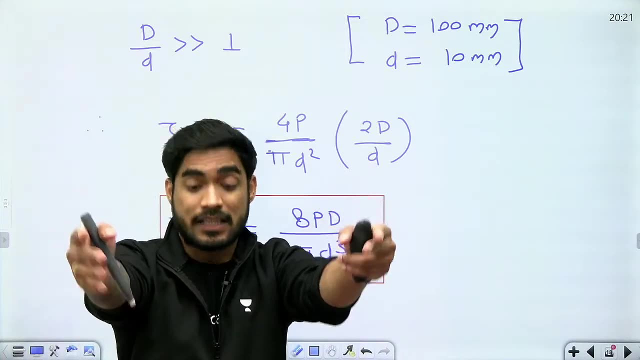 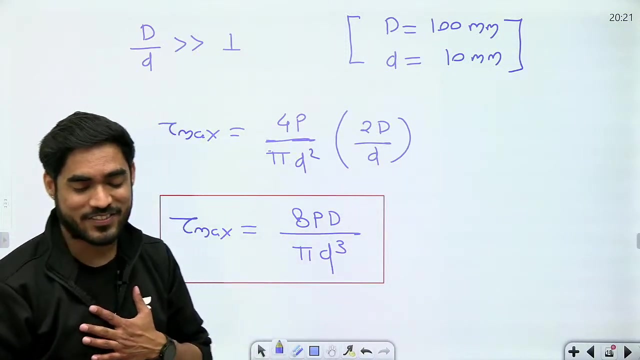 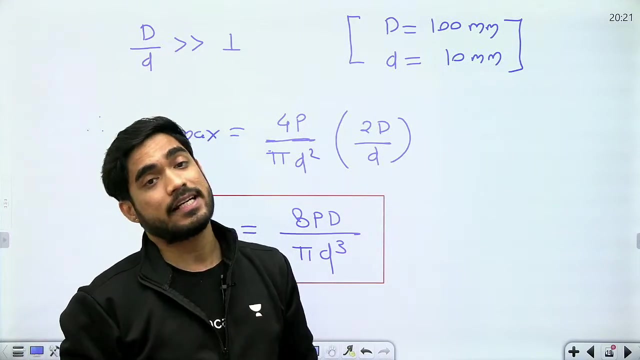 equation. only by default you have to use this equation. so, my brother, maximum shear stress has come. shear stress value has come. now what is our second objective? beta, quickly press like button. do half century. please hit the like button right now and complete my half century, complete my half century now. my brother quickly tell me: what more do we want? we want the deflection. 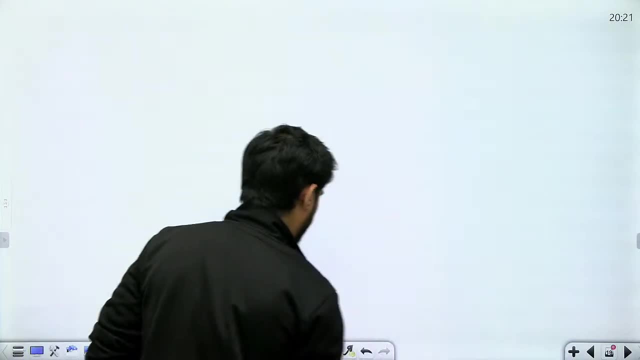 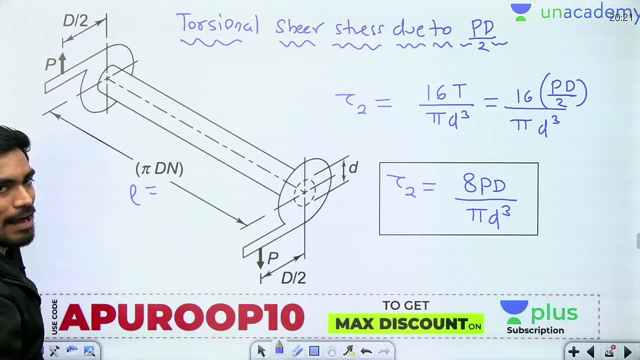 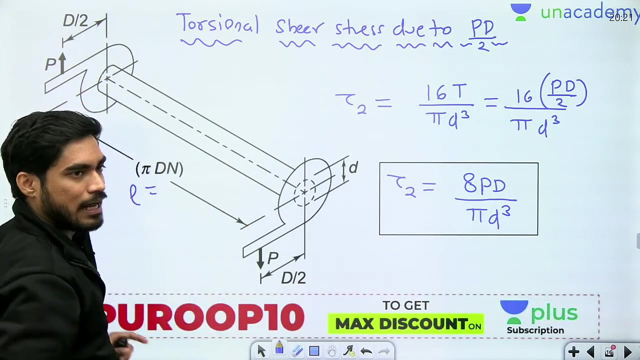 right now, beta. what are we going to do to find out deflection? okay, in order to find out deflection, what we are going to do, understand right now. we are assuming that this is like a shaft. now I am considering it as a shaft. okay, now, if this is a shaft, then what will come in it? because of torque. 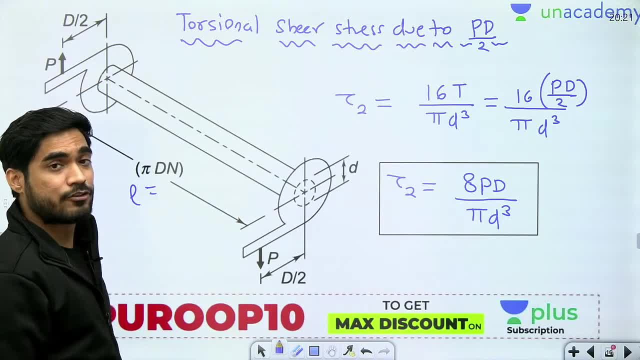 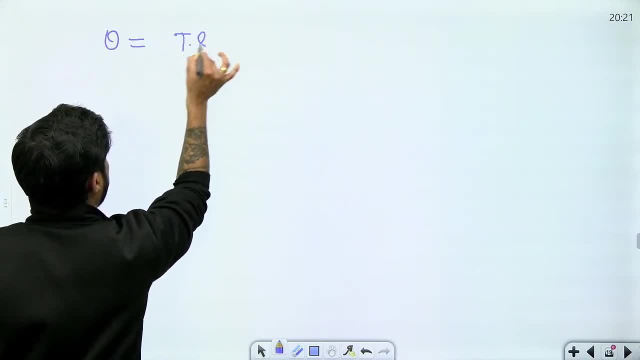 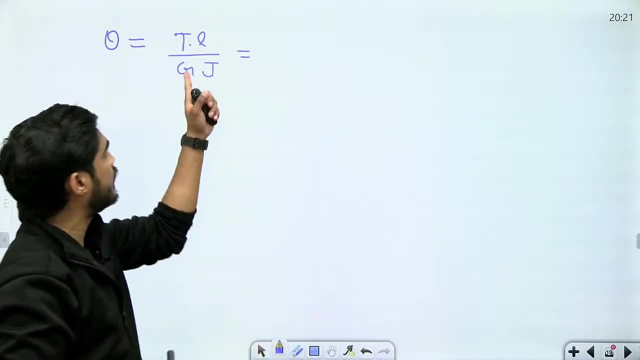 what will be there? due to torque, there will be angle of twist right and what will be the angle of twist? angle of twist theta will be equal to t into l by g into j. right now, assume this is as a shaft. now consider this as a shaft. we will make spring later, so torque. 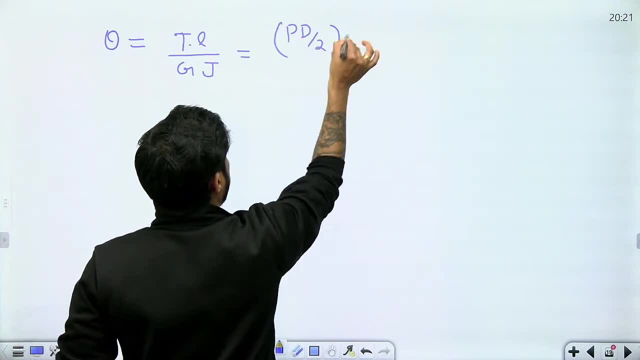 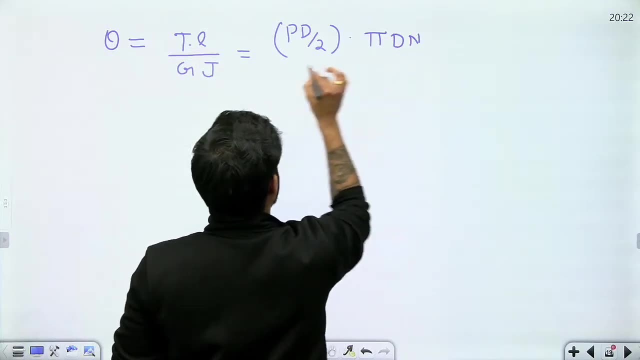 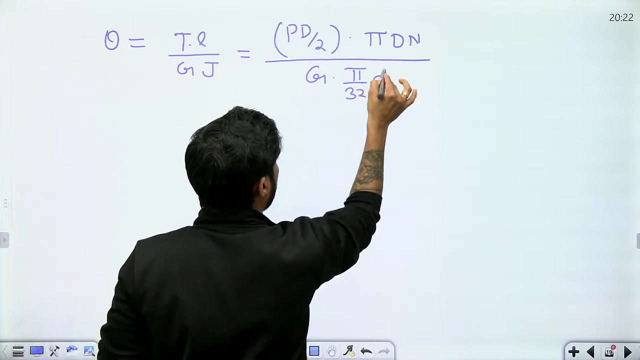 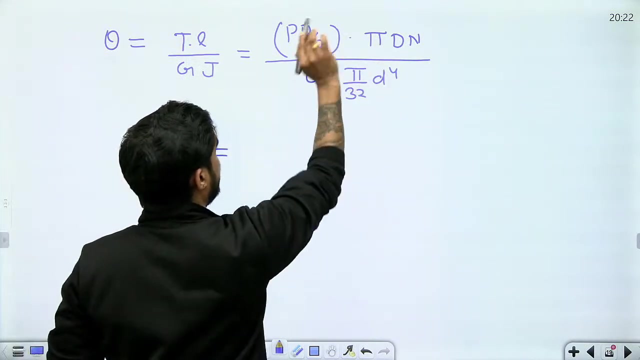 is how much. pd by 2. length is how much. I have already explained. length is pi d n, pi d n g is material property and j will be. polar moment of inertia will be pi by 32 d to the power 4. now do this up and down. you will get theta equal to beta. 32 will go up, 2 will come down. 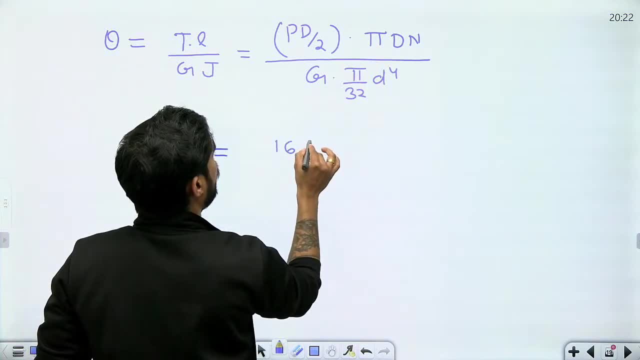 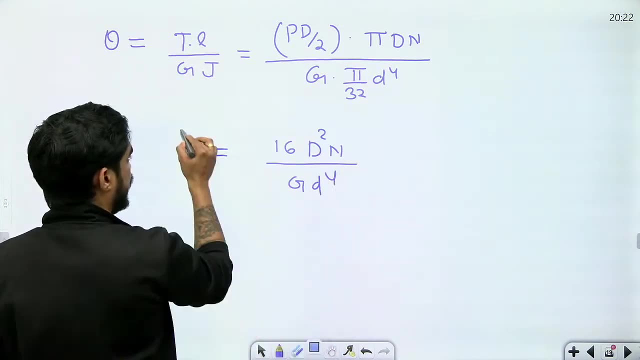 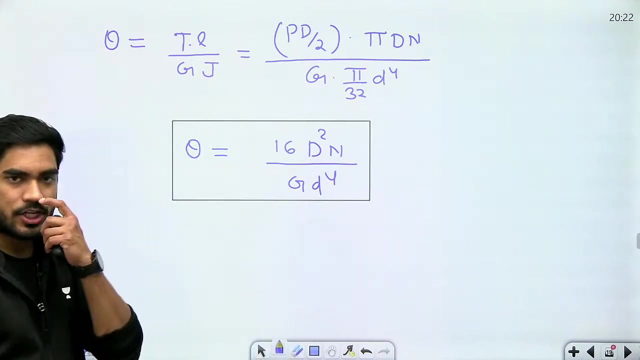 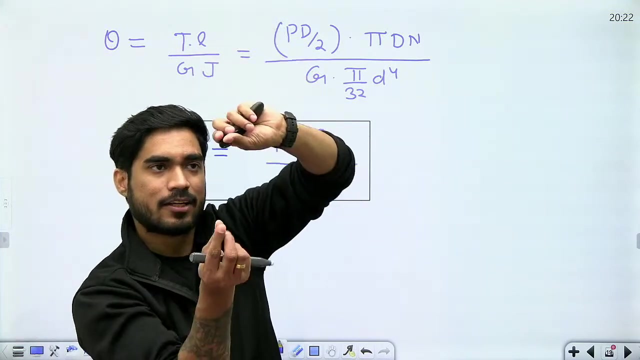 so this will become 16 pi pi cancel. this will become 16 d square n by g d to the power 4. this is the equation of angle of twist. okay, now, my brother, angle of twist. what i want? deflection of the spring, spring may, axial force like a, but it. 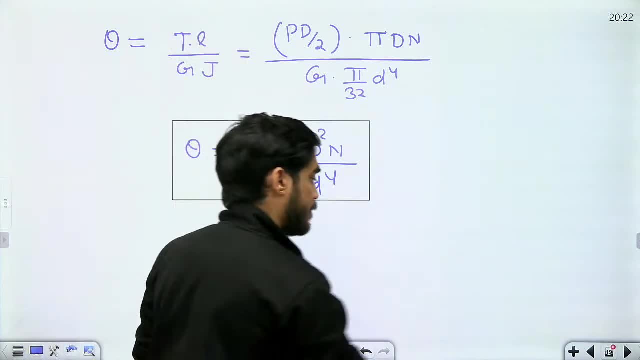 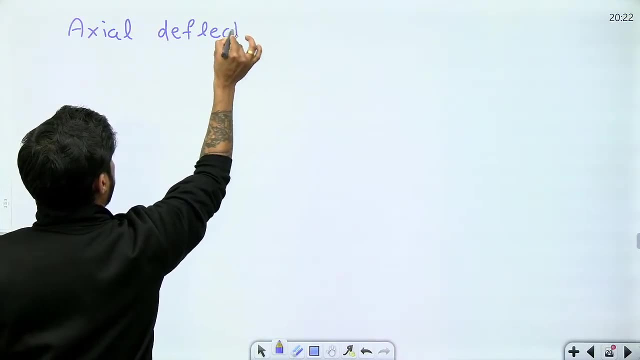 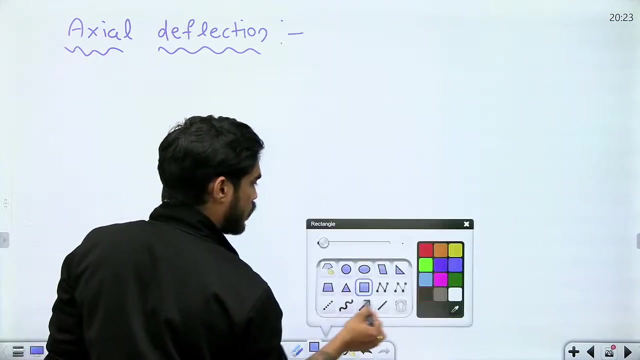 in a paradise how much it is deflecting in axial direction? okay, outside axial deflection: nikal name, I want the axial deflection. axial deflection of axial deflection. nikalнул wordt concept. they Veu okay, both N Gber the concept okay. 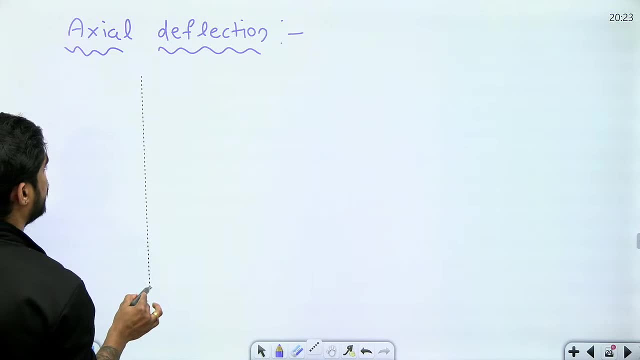 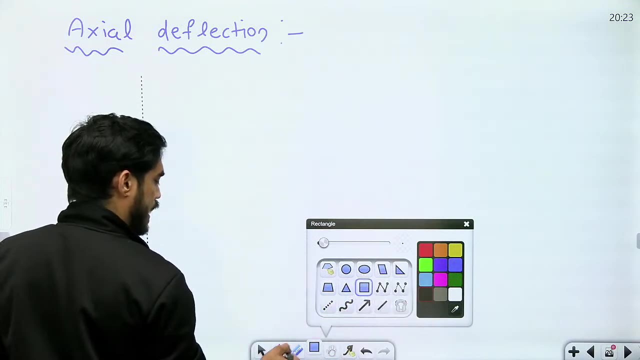 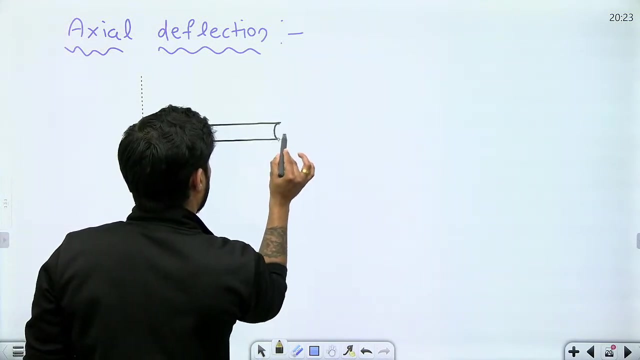 propia wallah. So understand the concept behind the axial deflection beta. So right now, right now, my spring is like this: okay, Right now, my spring is like this: okay, This is the axis of the spring. 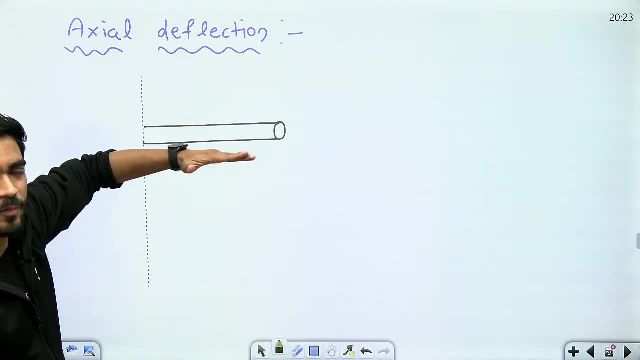 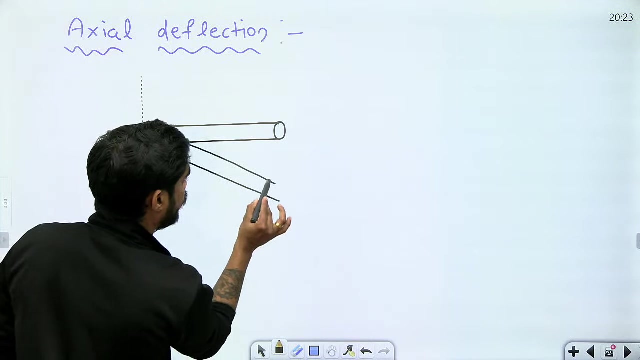 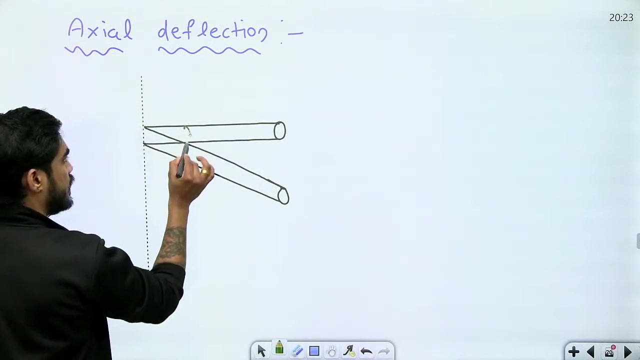 One turn I am considering. okay, Now, I was assuming that it was just like a shaft. okay, Now, my son, this turn twisted by some angle theta and it got here. When there will be twisting in this spring, then it will be twisted by some angle theta, right? 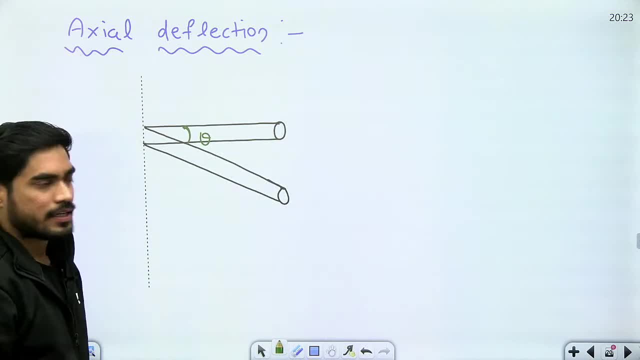 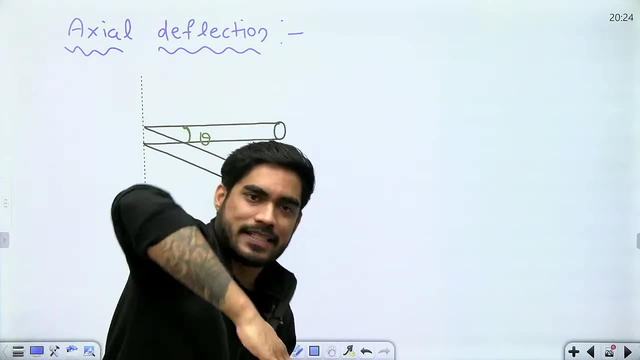 This will be the angle theta and it will come here Now, my son, I have already calculated this theta. right Now, when you will rotate the spring, my brother, then this turn will rotate and go down like this right. 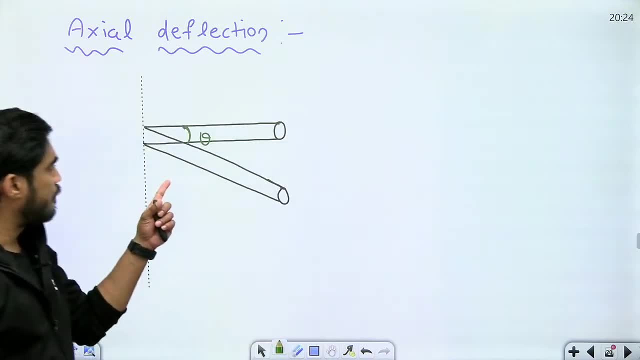 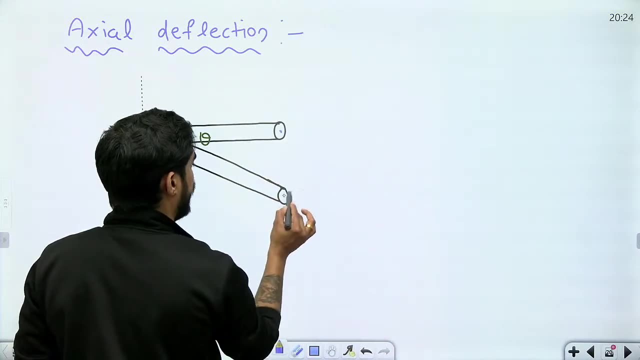 This turn will twist and it will go down, okay. So, beta, do you want this angle of twist? No, I don't want this angle of twist. What I want, I want this, I want this. I want this delta, okay. 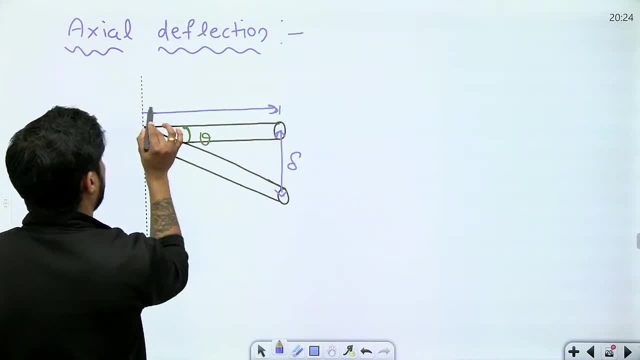 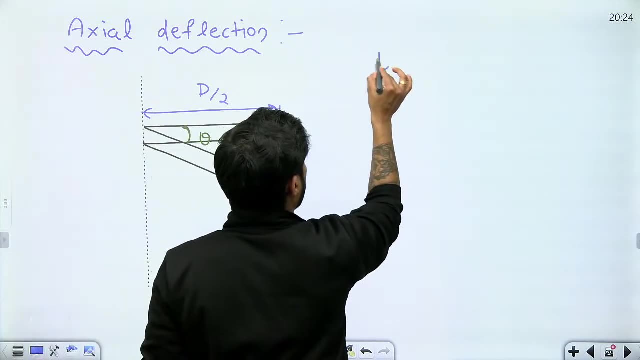 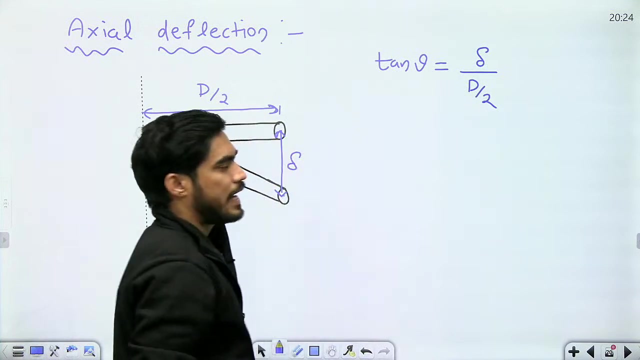 Now, what is this distance? beta? This distance is how much This distance is d by 2.. So in this triangle can I write 10: theta is equal to delta upon d by 2.. And if theta is very small, then can I say it is almost equal to theta. 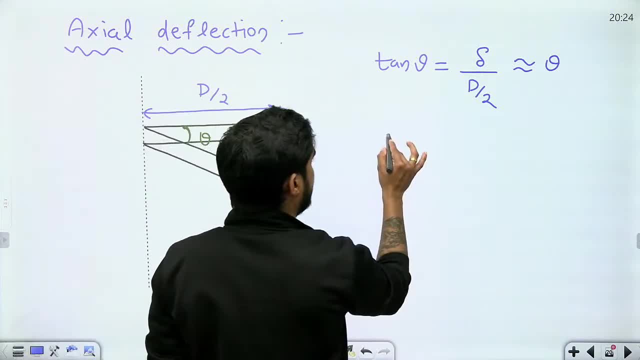 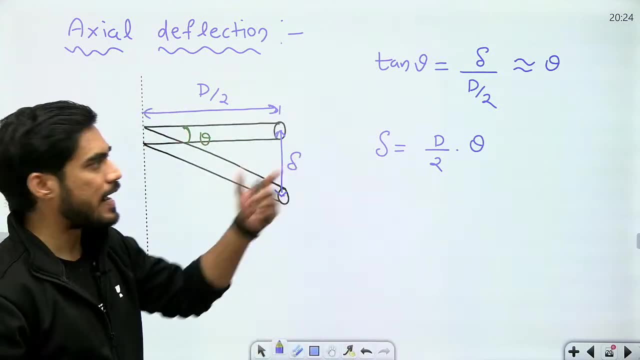 Yes, I can say it is almost equal to theta. So, my brother, can I write delta as d by 2 into theta? Yes, obviously I can write it right. So my son from here, how much will be delta? 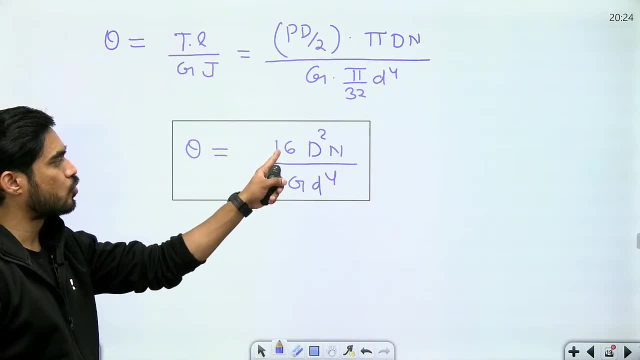 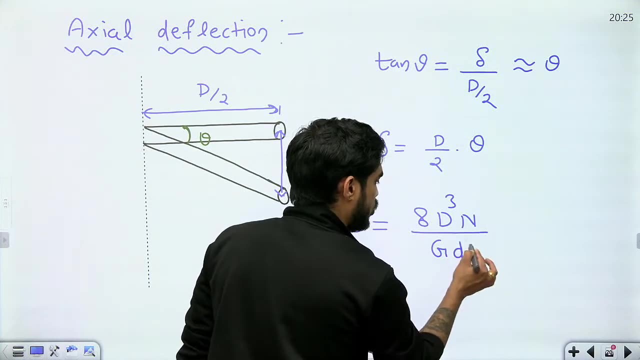 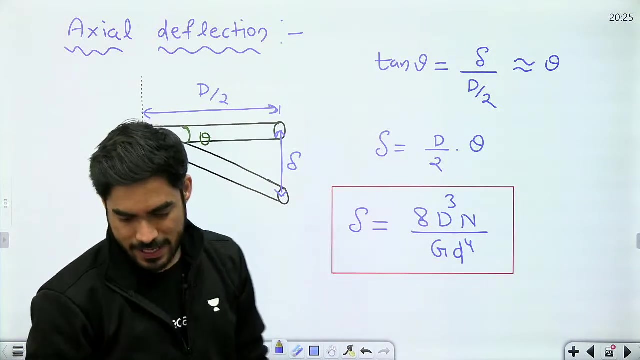 d by 2 multiplied by this, d by 2 multiplied by this, So this will be 8.. d cube n by gd to the power 4.. This is the equation of axial deflection. This is the equation of axial deflection. 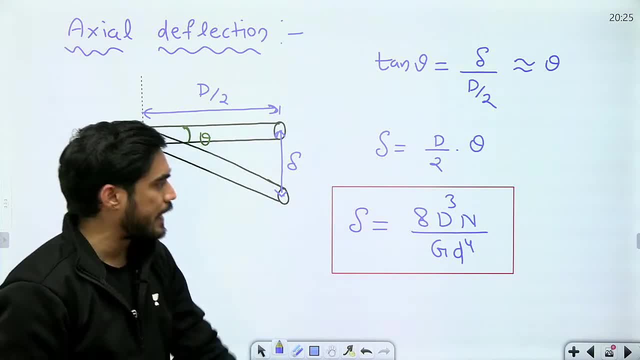 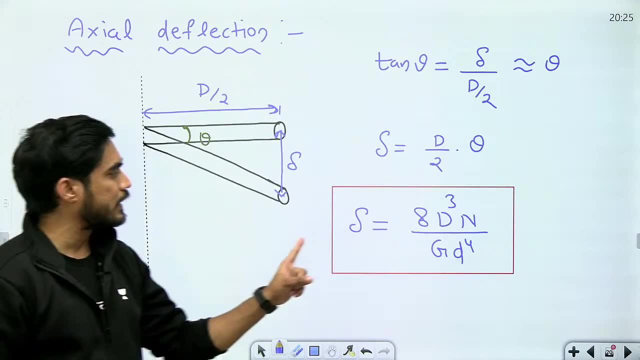 Yes, Very good, beta Very good, Very good, Very good. So my brother just remember two equations. You need to remember only two equations: Tau max equation and delta equation. We have derived both of them, okay Now, from delta equation. 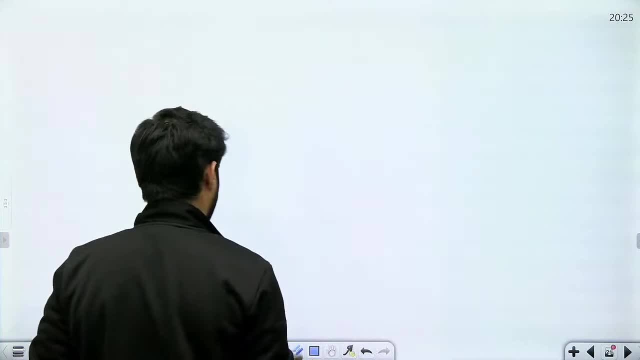 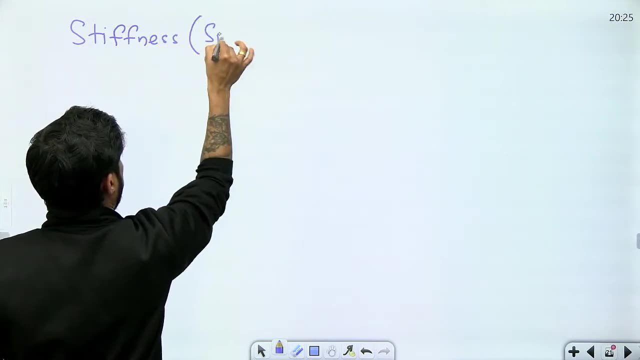 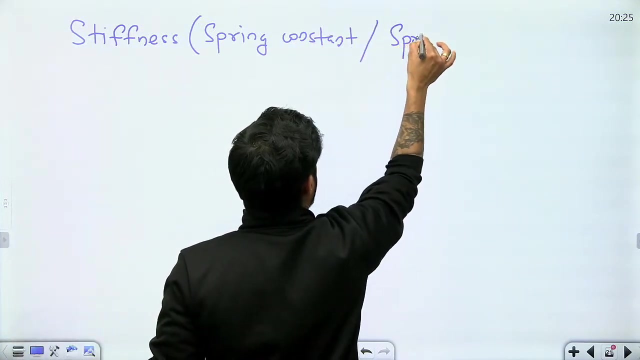 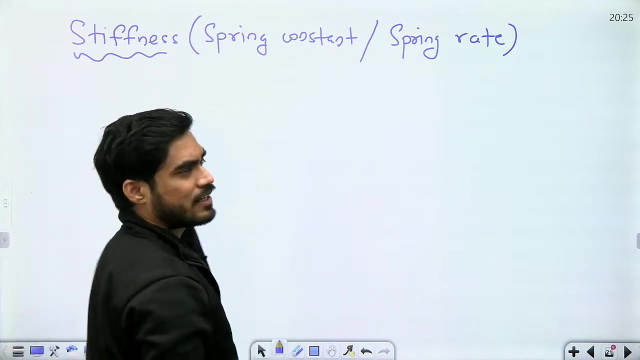 we can calculate two very important parameters of spring: What The first is stiffness, also known as spring, constant, also known as spring rate. Why I am saying this is because in some exams, in some cases, they have asked: calculate spring rate. 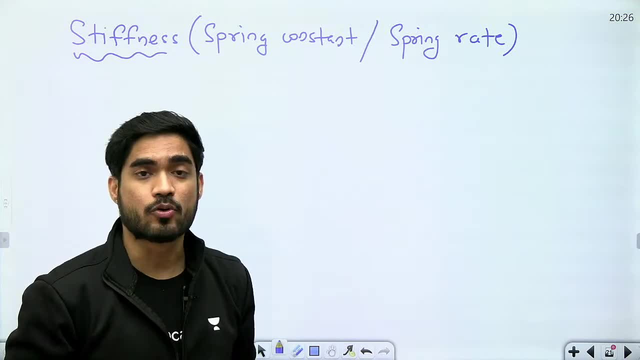 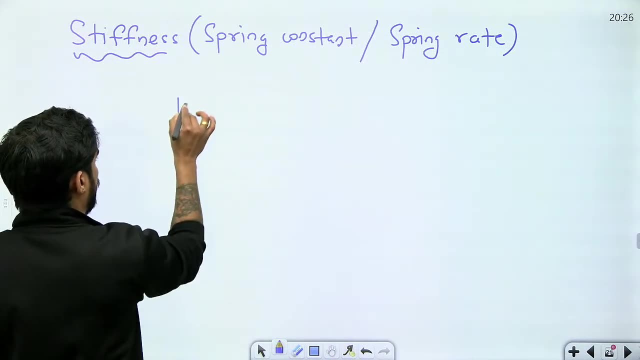 or calculate spring constant and students get confused. What is spring constant? What is spring rate? So spring rate and spring constant are one and the same thing. They are stiffness. only Now, what is stiffness? beta Stiffness is the force required for unit deflection. 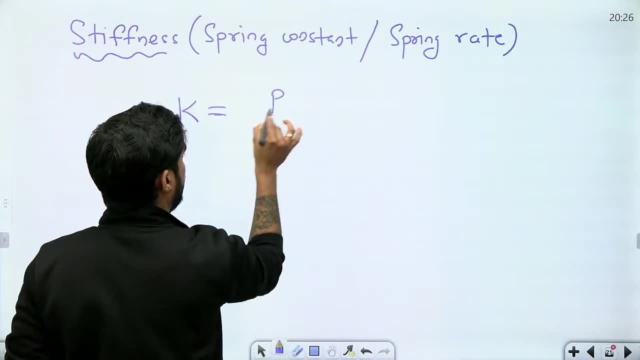 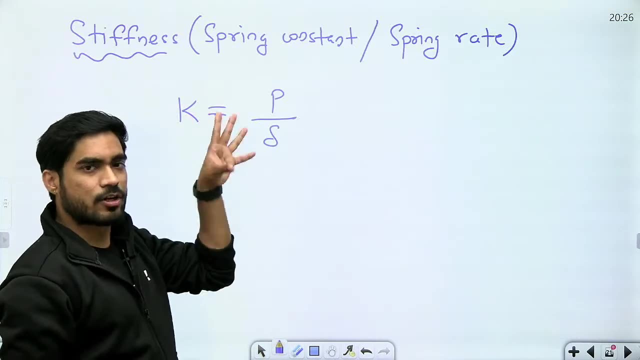 What is stiffness Force required for unit deflection? So it is p by delta. Now beta understand. If you remember the equation of delta, you don't need to remember the equation of k. You can just use this p by delta. 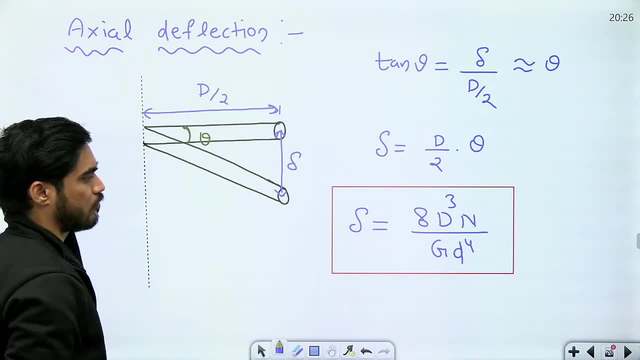 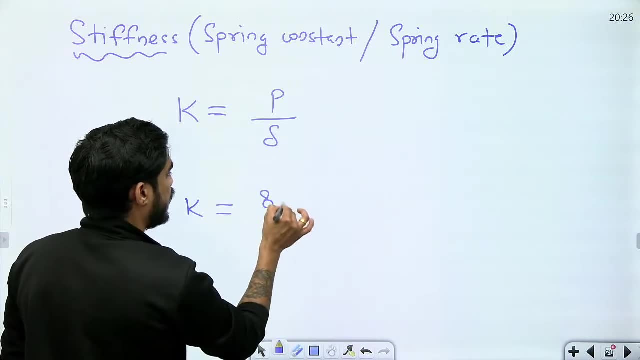 Or if you put delta in this equation, what you are going to get beta. It will go up, it will come down and one p will come. So it will become 8pd, cube n by gd to the power 4.. 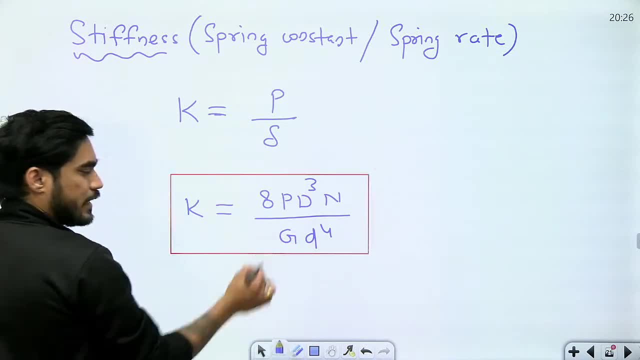 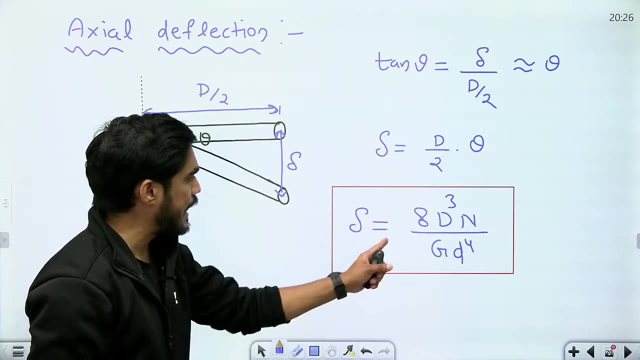 Now what I am telling you. you don't need to remember this separately. If you remember this, you can always find this p by delta will give you this. Okay. So, my brother, you don't need to remember this. 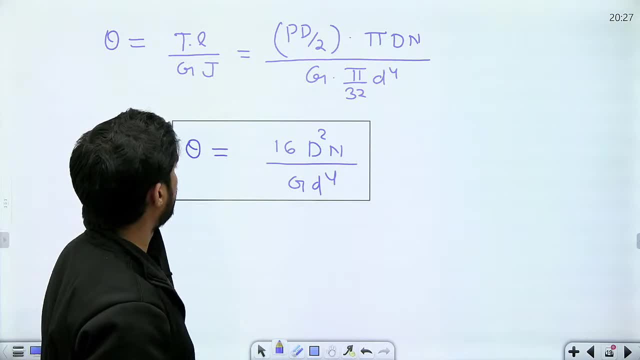 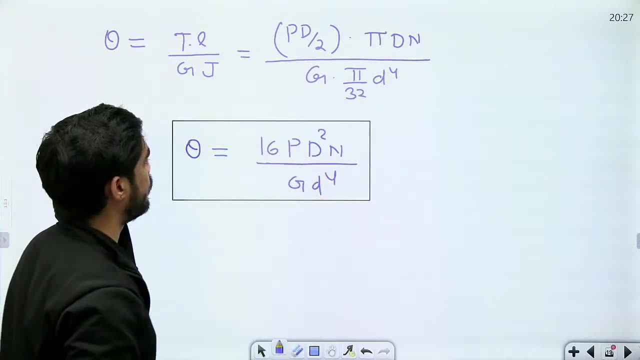 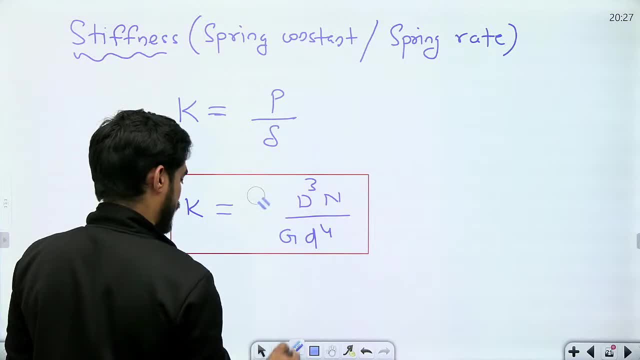 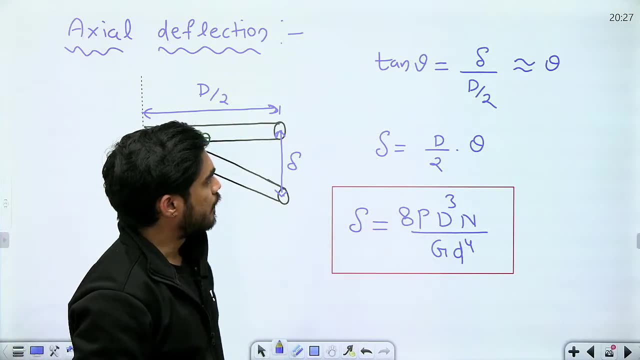 So now I am thinking: how is p coming in the equation of k? Yes, So sorry, So sorry. Yes, There was p here. Yes, There was p here, There was p here. I ate p. So, my brother, I have brought p back. 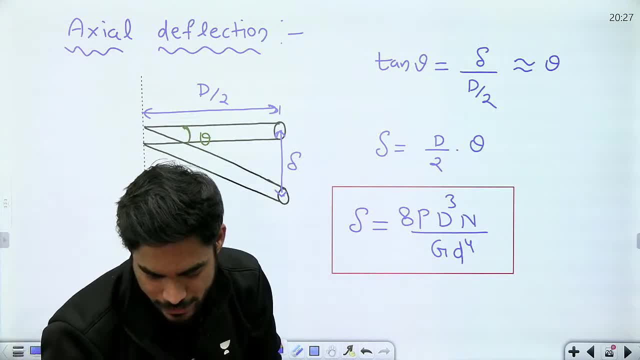 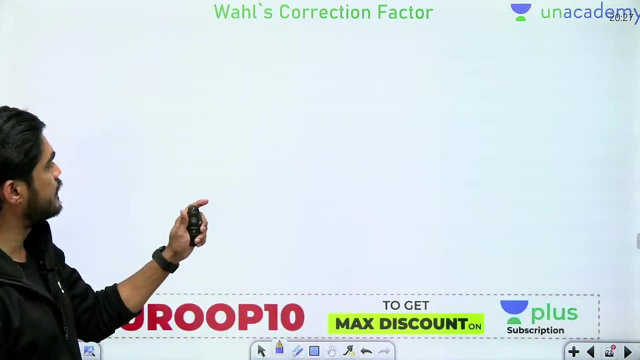 So there is no need to worry, No need, No need to worry, No need to worry, No need to worry. So sorry, So sorry, So sorry. I ate p, But I have brought p back. So, my brother, this is the equation of stiffness. 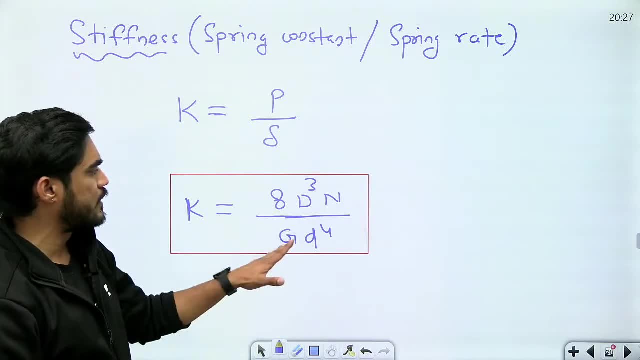 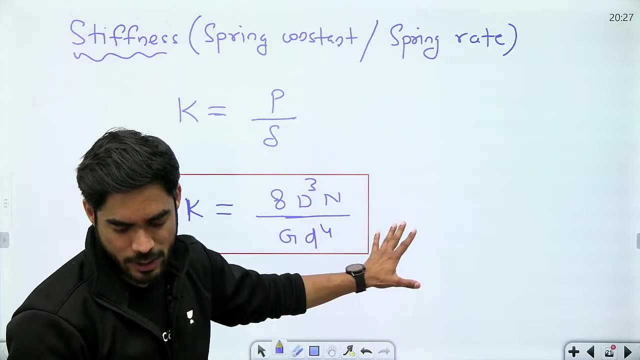 If you want, you remember this. Otherwise, no need of remembering this Because, son, if you remember the equation of delta, you can always find the equation of k. Or if you remember the equation of k, you can always find the equation of delta. 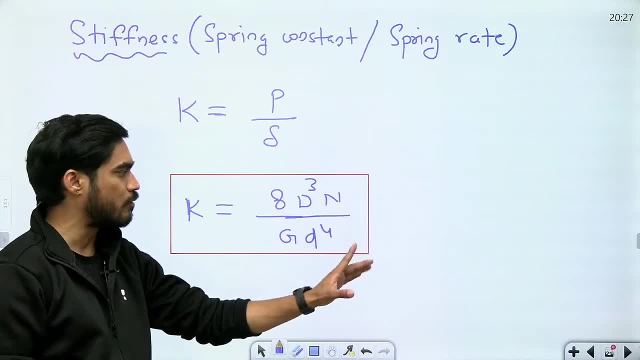 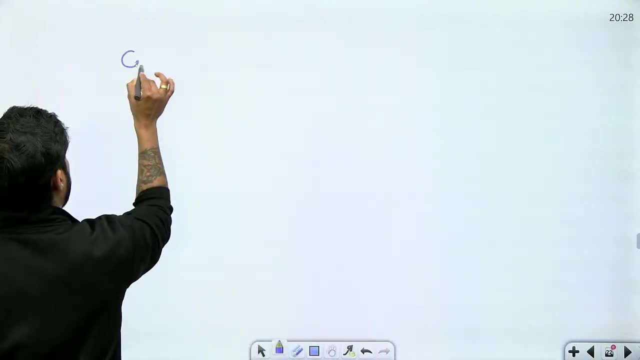 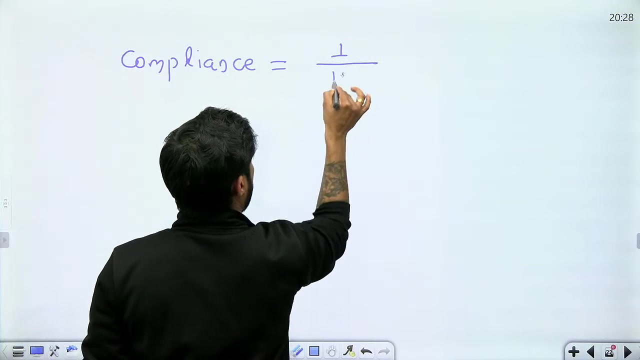 Okay, So don't worry about memorizing both these equations. Memorize any one equation, Okay. What is the opposite of stiffness? The inverse of stiffness is also known as compliance. So remember this too, my brother: It is inverse of stiffness. 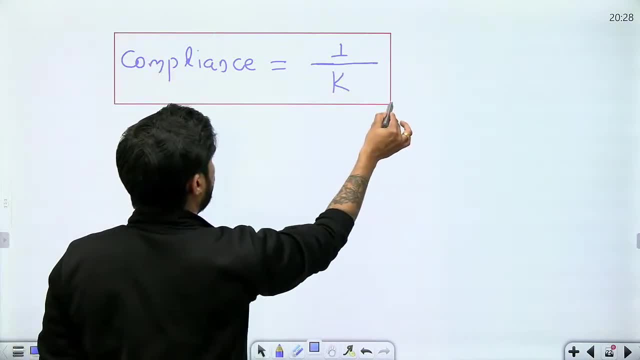 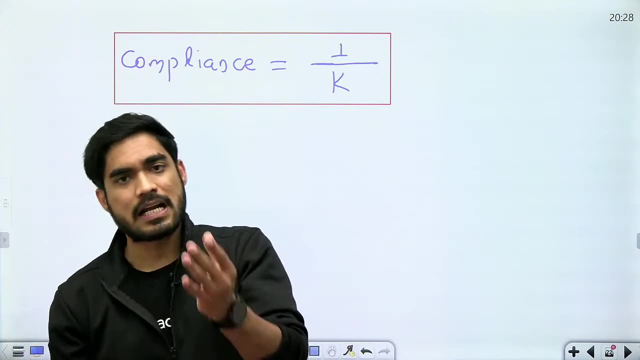 Okay, Why I am telling you this? Because, son, in one exam they asked: what is compliance? What is compliance? They asked, and the children were confused: What is compliance? So, son, compliance is nothing but one by stiffness. 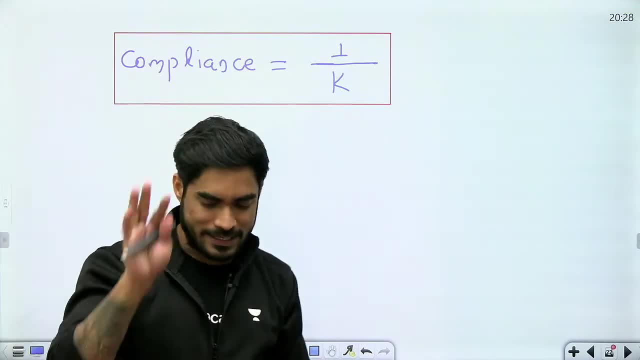 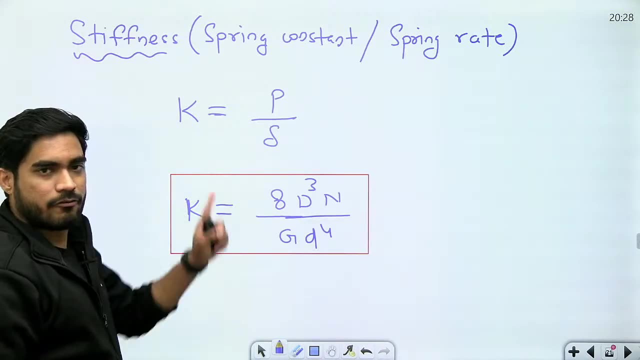 Okay, Now, what is the use of this? Don't get into all this. Don't get into all this. Just know that compliance is one by one, One by stiffness. Okay, Compliance is one by stiffness. Okay. Now, my brother, we have derived the equation of stiffness. 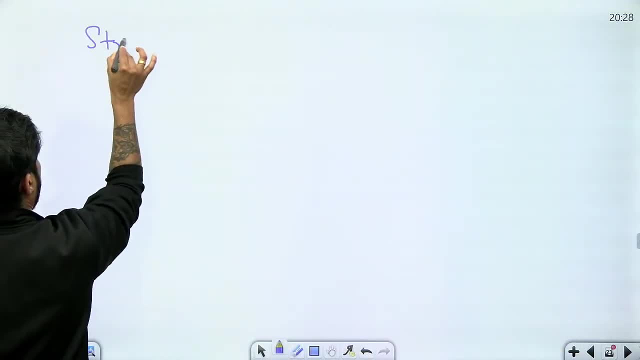 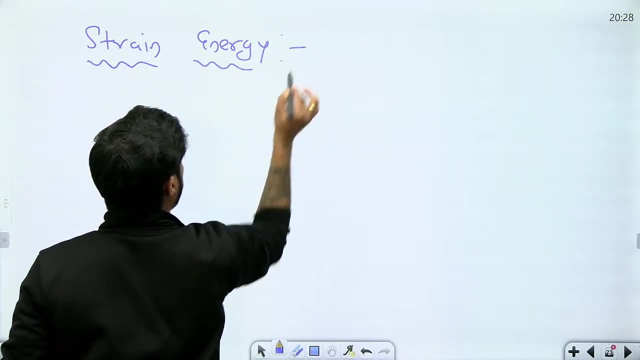 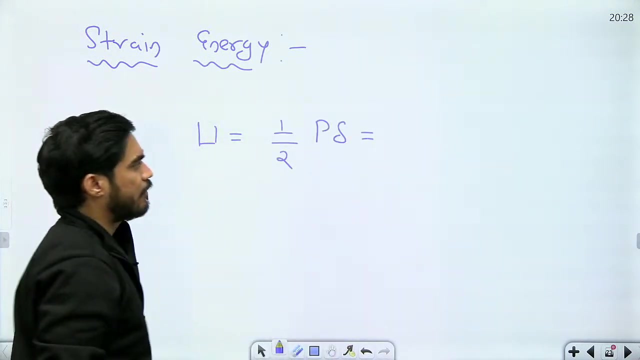 Now what is the next important parameter? Strain energy stored in spring. So how can we get strain energy stored in spring? U is given by half- into P, into delta, Or if I put the value of P in terms of delta, 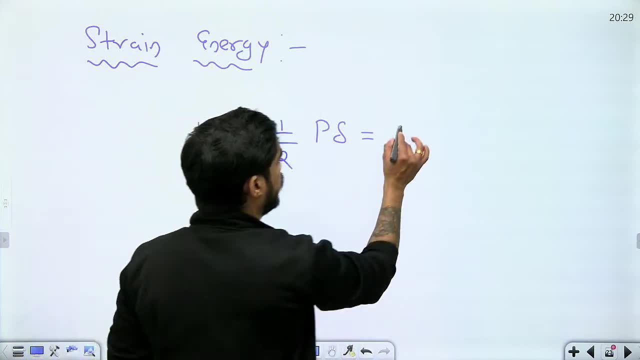 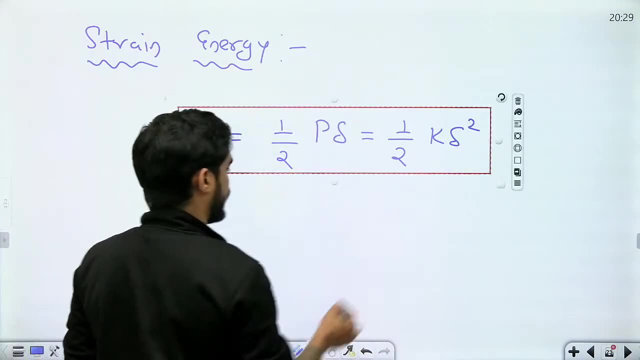 then son P will be K delta. If I write K delta, then how much will this be? It will become half K delta square. Now there is no need to remember the equation of strain energy separately. You just need to remember this. 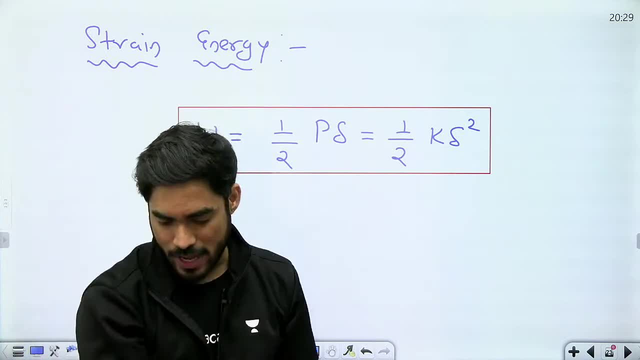 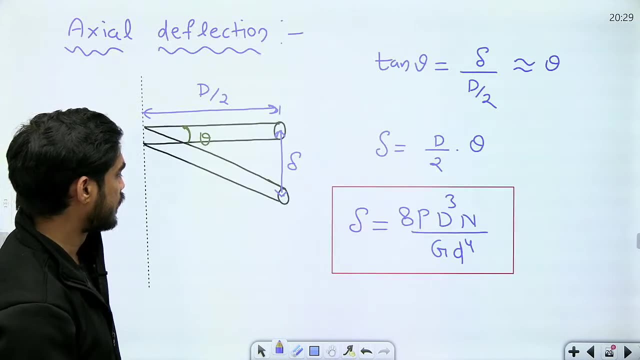 Half P delta and half K delta square. Is it clear? Is it clear? Is it clear? One second son, Did I do something wrong? So sorry, son. What am I doing wrong today? What am I doing wrong today? 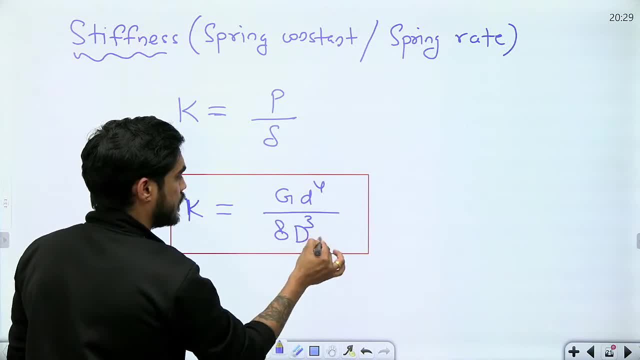 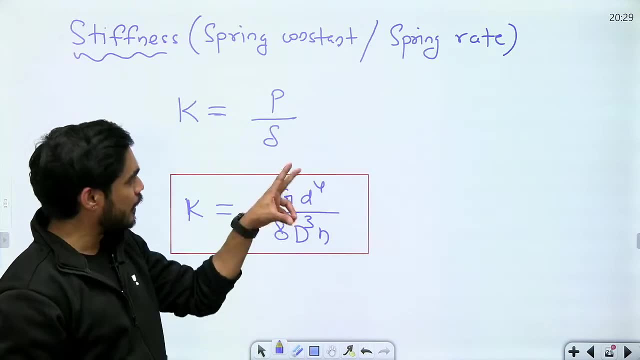 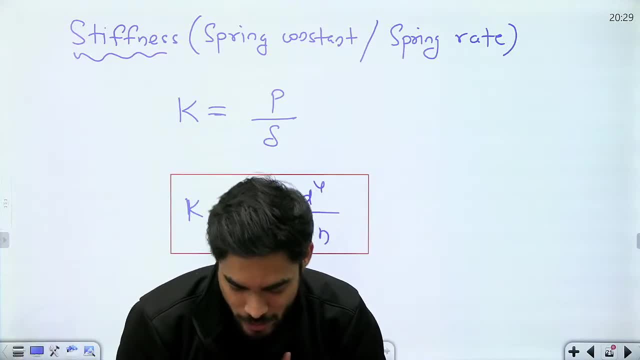 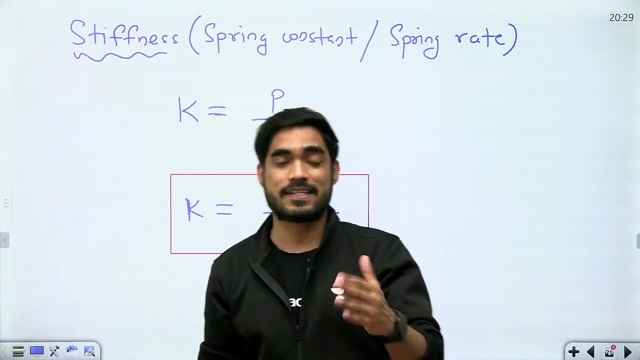 So this will become GD to the power 4 by 8D cube n. I am so sorry for my mistake. I apologize, my brother, Today consider the excitement of the last class or consider the fatigue of many classes. Okay, 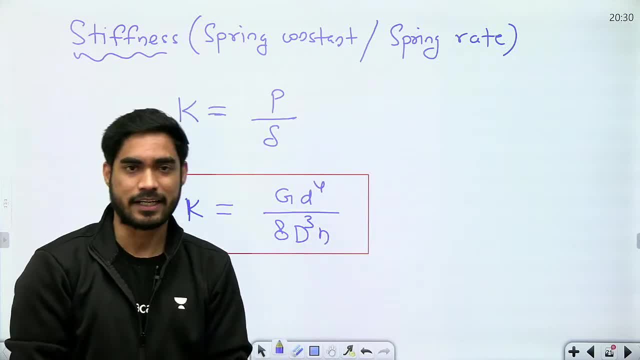 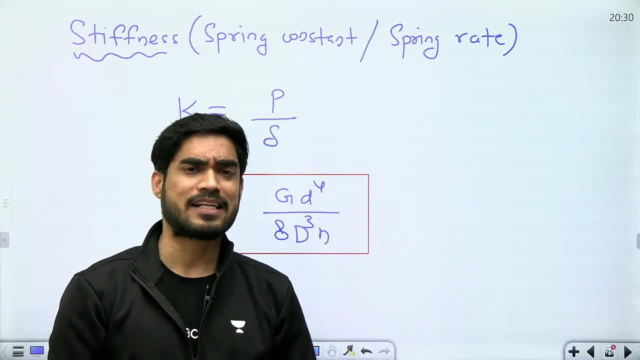 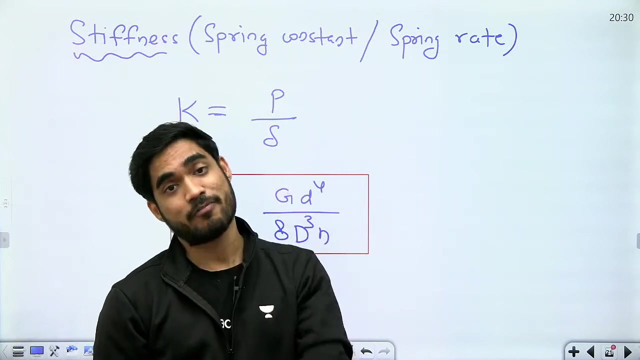 Because, son, this month has been very hectic for me. Continuously, I have taken classes on YouTube, I have taken classes on special, on academy special, And, son, this week particularly has become very hectic for me. Okay, And tomorrow I have 8 hours of marathon class. 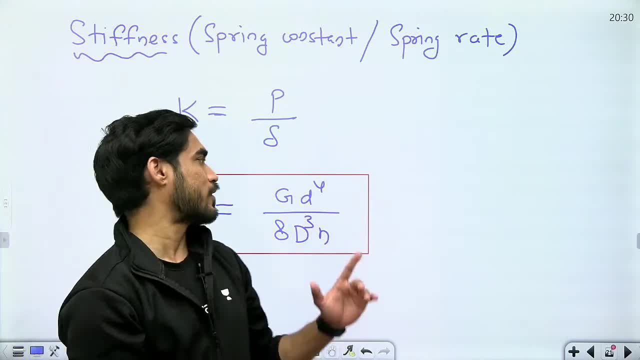 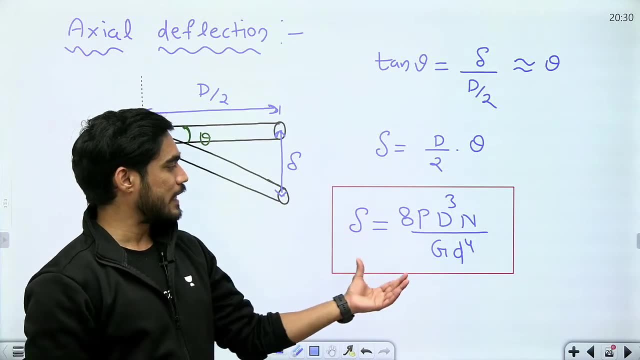 So you can imagine how much pressure I am handling, Okay So, so, sorry for these mistakes. Okay, My brother ignore these small mistakes Ultimately, but I am correcting my mistake, Okay. So, son, I have written delta by inverting P here. 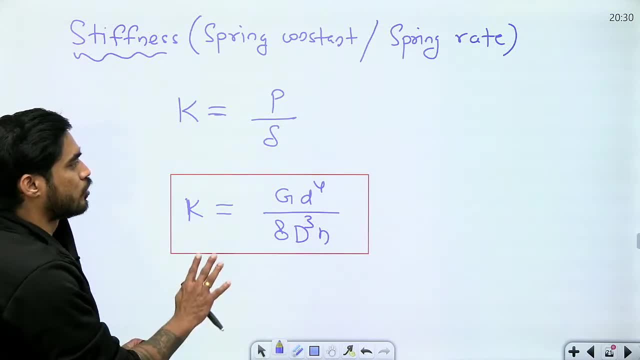 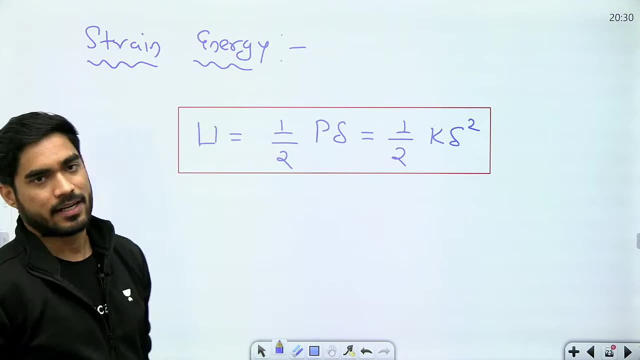 Okay, So sorry for this. Thank you so much for understanding. Okay, So my brother, invert the equation of K. Compliance has come. Keep the equation of K here. Or keep the equation of delta here: Strain energy has come. 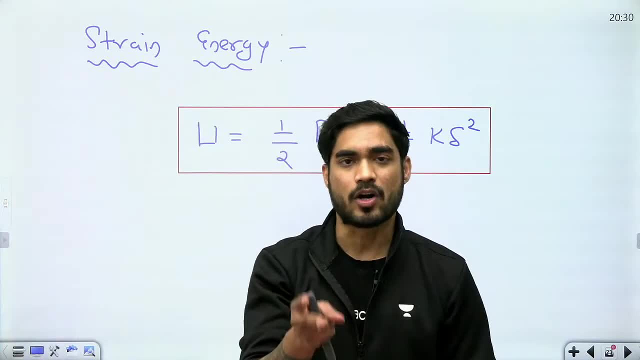 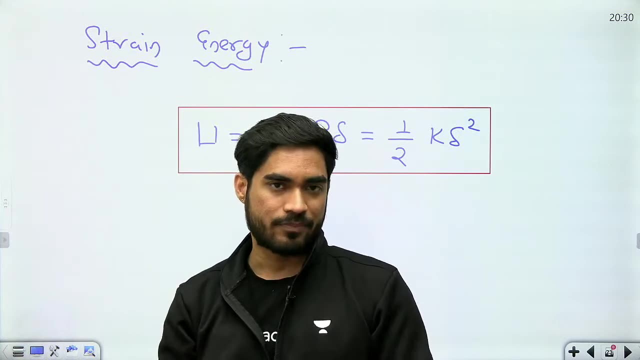 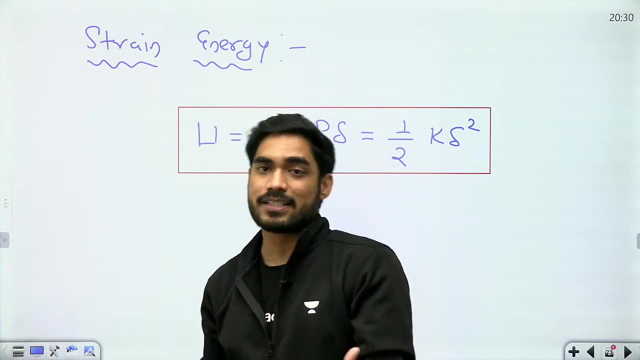 Okay, So strain energy and stiffness are two very important aspects of spring. In the applications of spring, stiffness and strain energy have a very big role And we have seen this in different applications. For example, son, if you are using it to absorb energy, then strain energy will be very important. 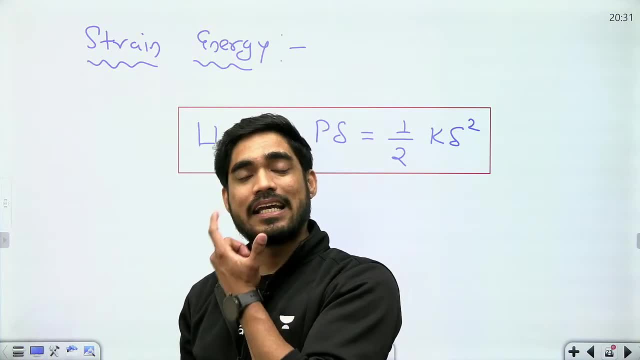 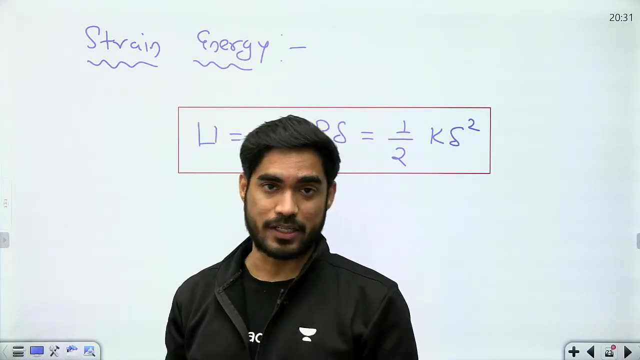 And if you are using it. If you are using it, If you are using it in case of giving force, if you are using it to keep the contact between two elements, then stiffness is very important. Okay, For example, in clutch. 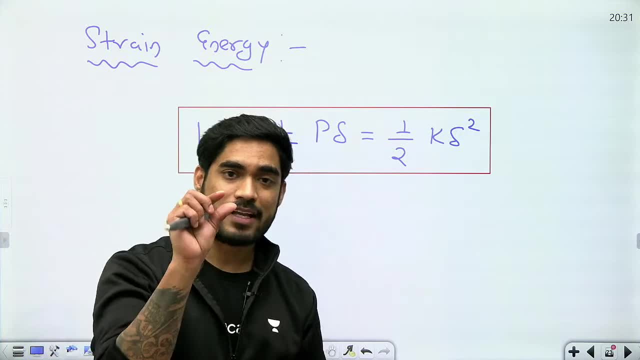 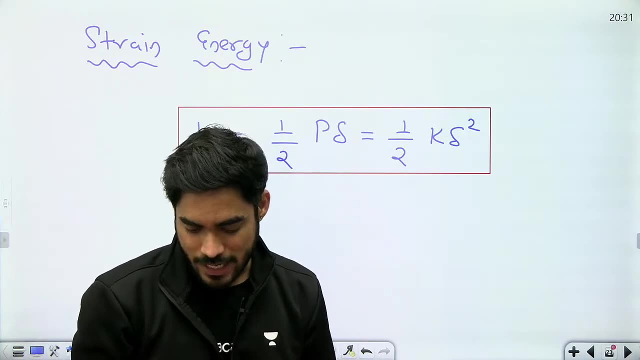 In clutch, you have seen that stiffness plays a major role. Right Stiffness will decide what will be the speed at which engagement starts. Thank you so much, son. Thank you so much for understanding. So, son, in the case of clutch, why do we use stiffness? 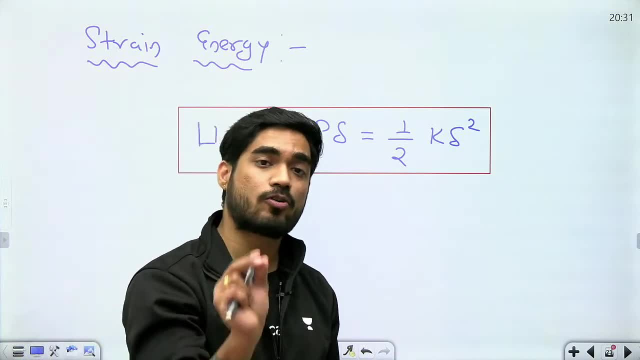 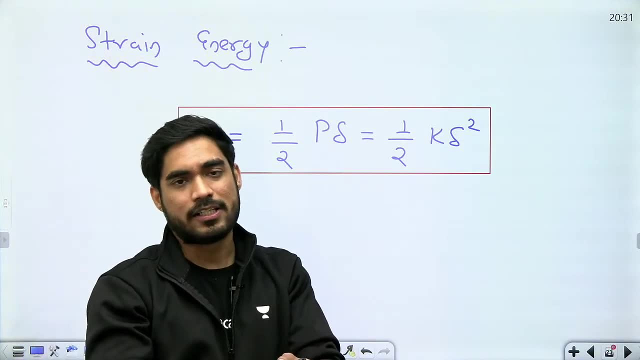 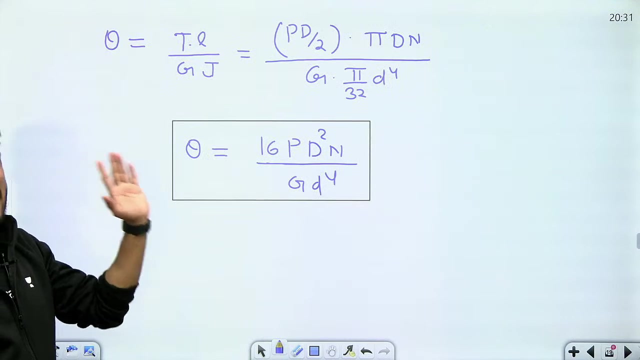 We use stiffness to increase engagement speed. In order to modulate engagement speed, we use stiffness. Okay, So stiffness and energy stored in spring, These two are very important parameters of spring. Okay Now, my brother, I have derived all the equations that you have to remember. 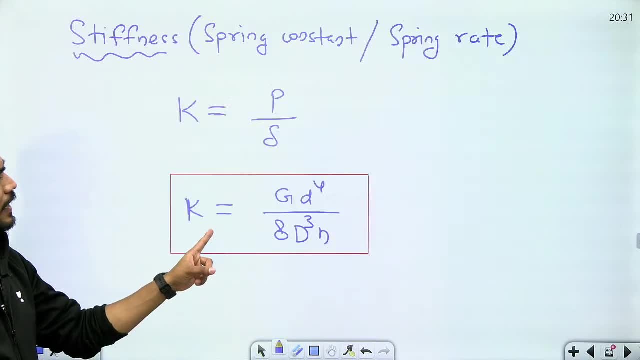 Whatever equations you need to remember, you need to remember this equation And you need to remember either this or this. So sorry, Where did it go? Yes, Either this or this. Okay, If you remember delta, you can use. 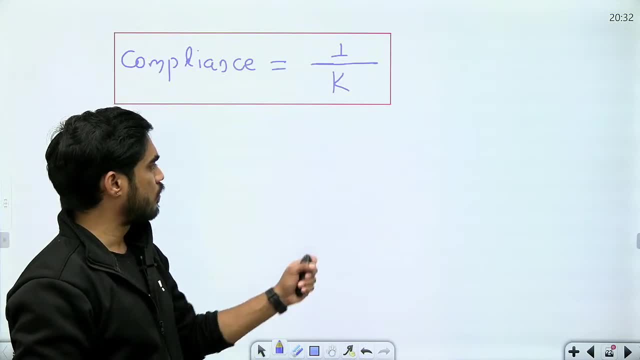 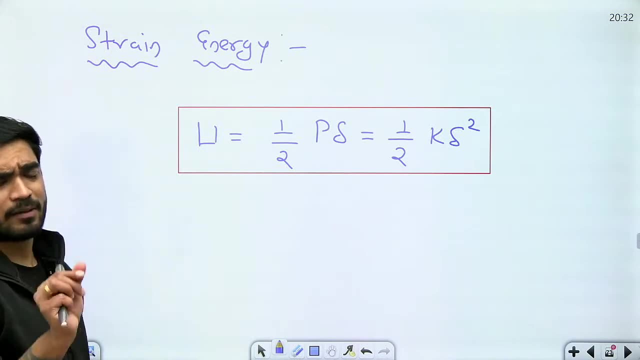 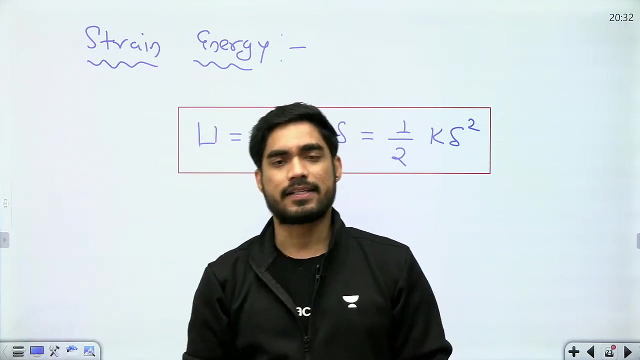 Find K, You can find energy stored, Okay, So no need to remember each and every equation. Okay, Now my brother. here one very important thing: When we were calculating tau max, we ignored two things. We ignored two things. 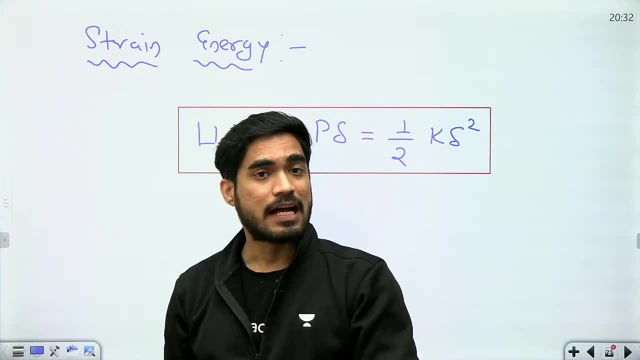 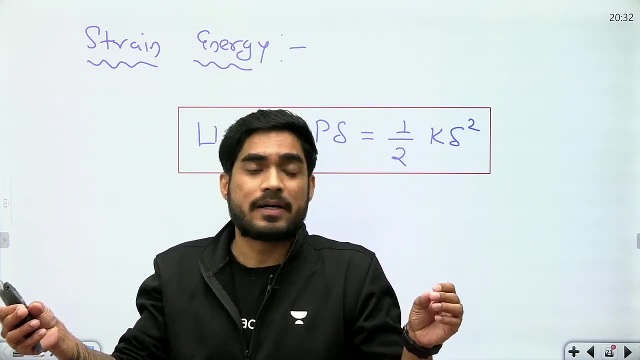 We ignored the curvature of spring. Remember, I told you that when we were deriving the equation of tau 2, we assumed that spring is a straight member, But actually spring is not a straight member, It is a curved member. So we ignored the curvature of spring. 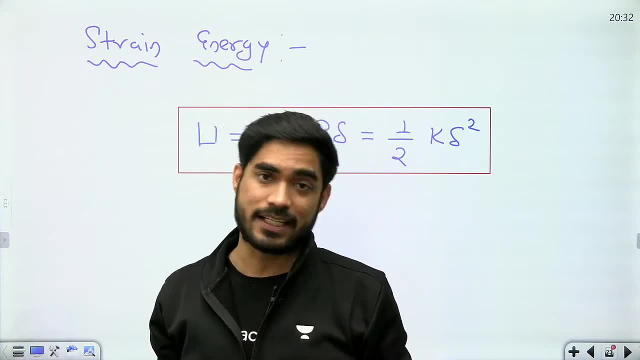 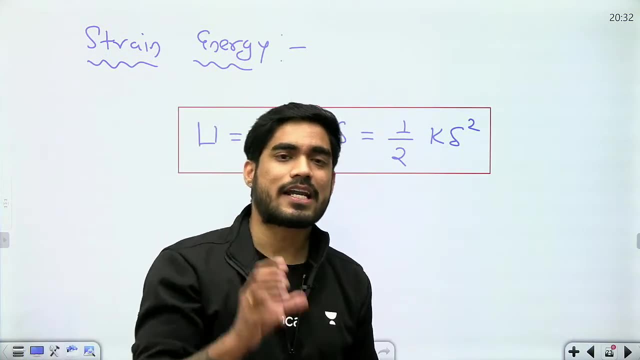 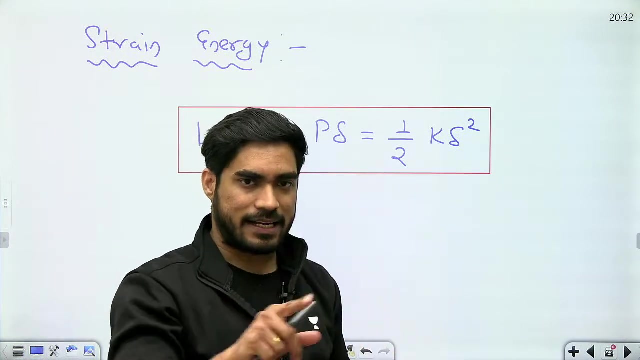 And second thing, in the final equation we ignored the direct shear stress. So, my brother, when we ignore direct shear stress and curvature, then whatever tau max we are getting, it is less than the actual value. Actual value of tau max must be greater than whatever we are getting in this. 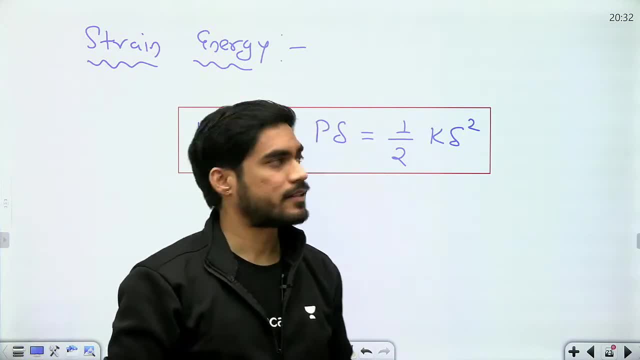 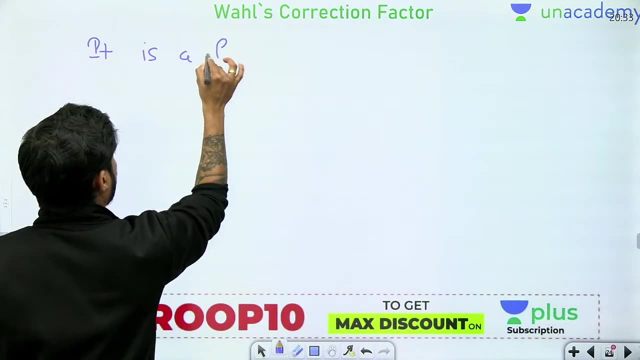 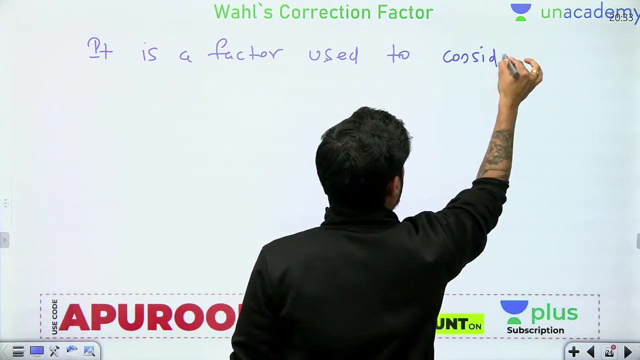 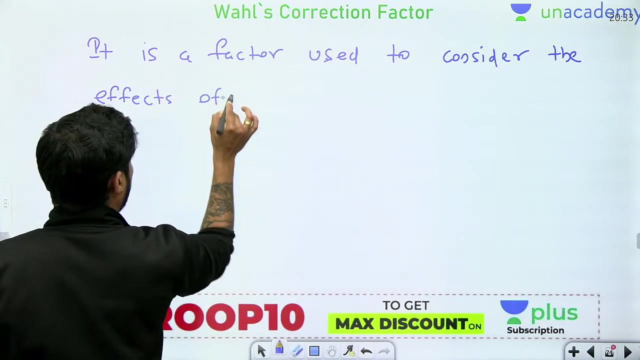 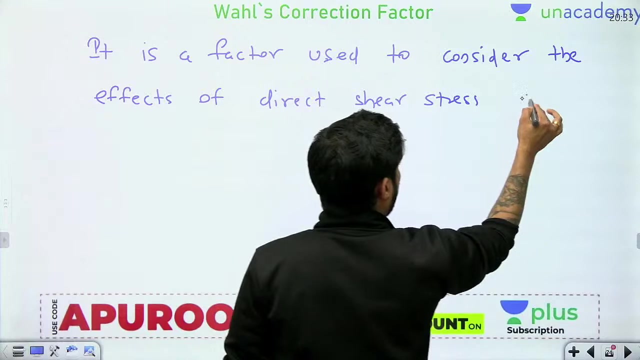 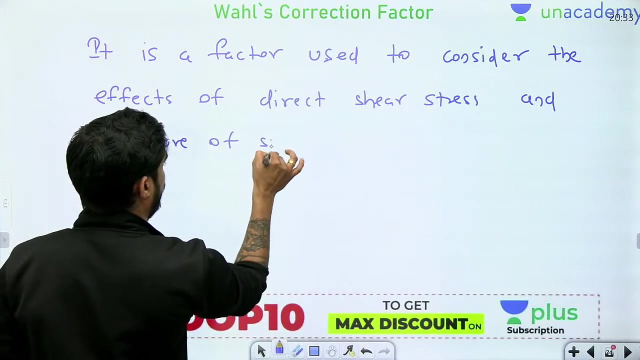 So, my brother, how do we consider those two effects? by using Wall's correction factor. So it is a factor used to consider the effects of direct shear stress and curvature of spring. It is denoted by Kw. I will denote it by Kw. 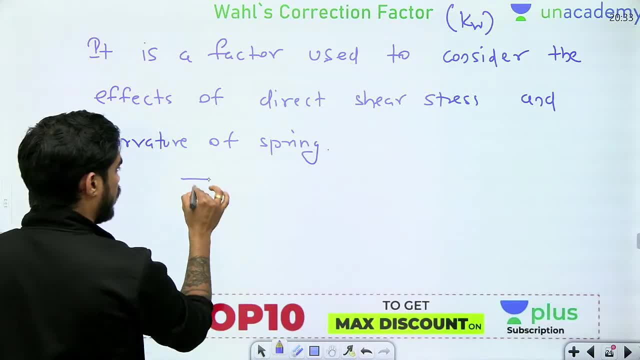 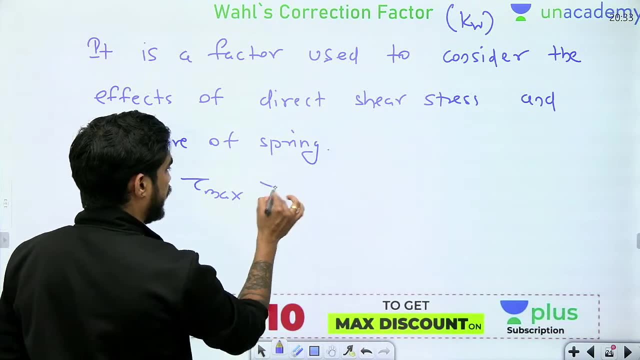 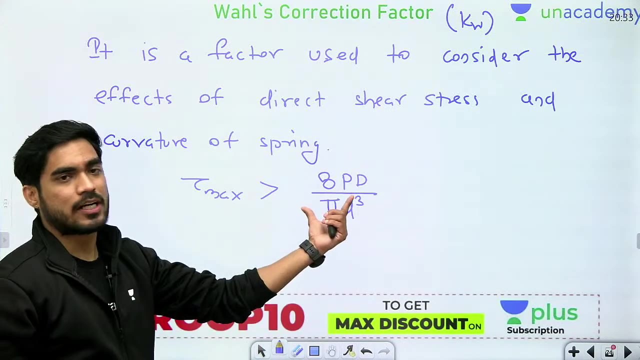 So, my brother, tau maximum should be greater than 8pd by pi d cube right. This is not the actual tau maximum, This is just a theoretical value. This is the actual value of tau maximum which we got from some assumption. okay, 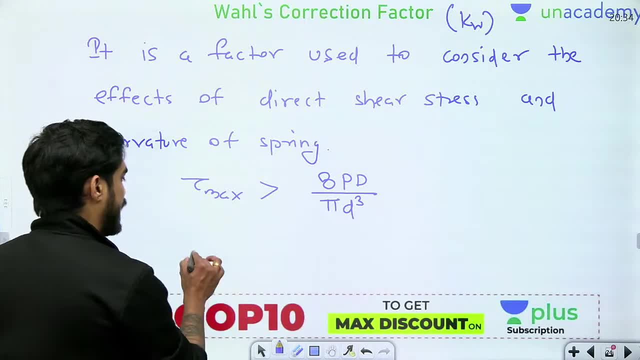 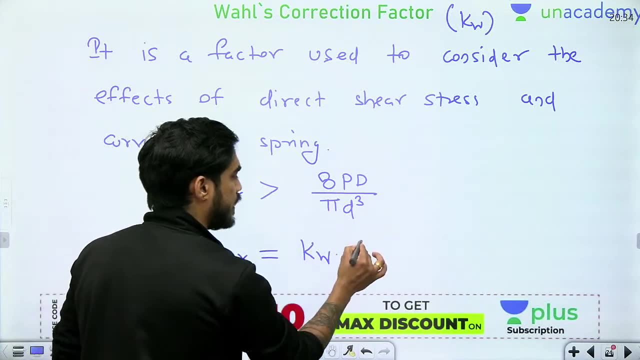 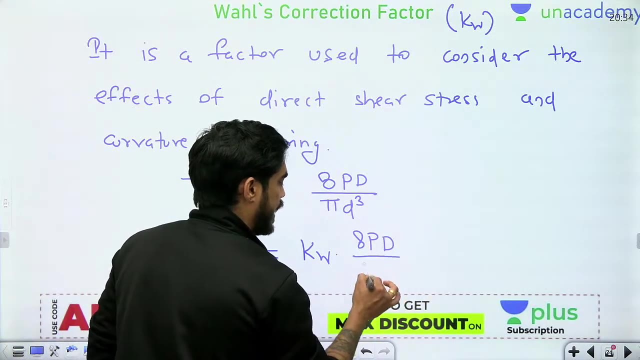 So, my brother, actual tau maximum should be greater than this. So, my brother, what will I do? I will multiply Kw in this in order to consider the effect. Now here, obviously, Kw will be greater than 1, right? 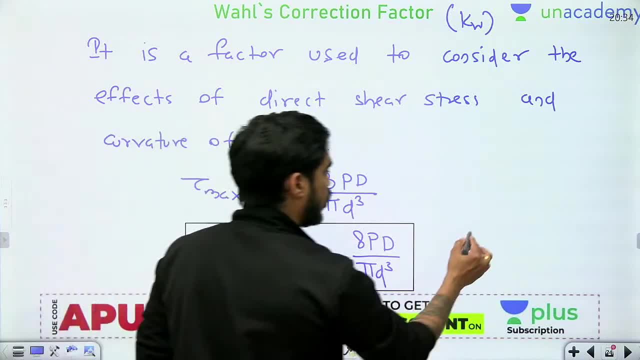 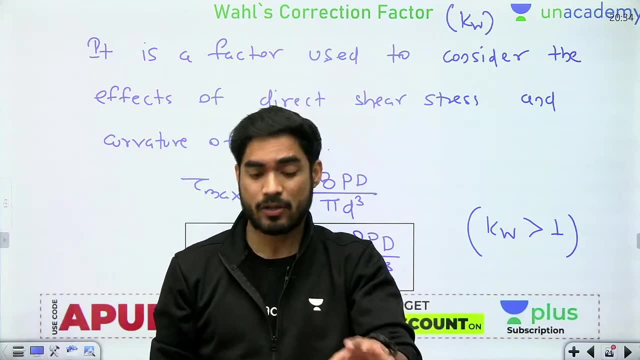 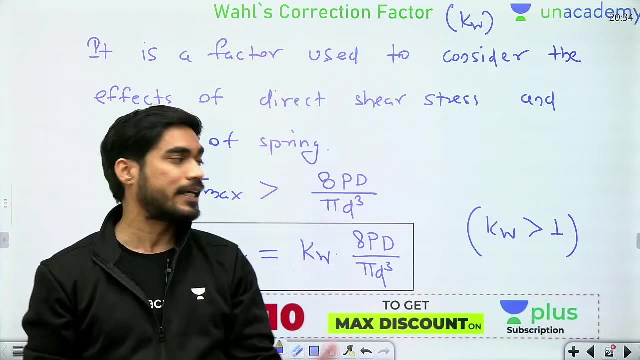 Kw will be greater than 1.. Kw Must be slightly greater than 1,. okay, Not very greater. What is the value of Kw 1.25,, 1.35,, 1.45,? okay, It will not be 10,, 20, 30.. 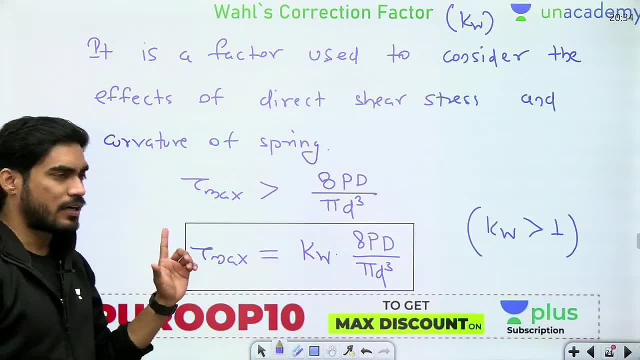 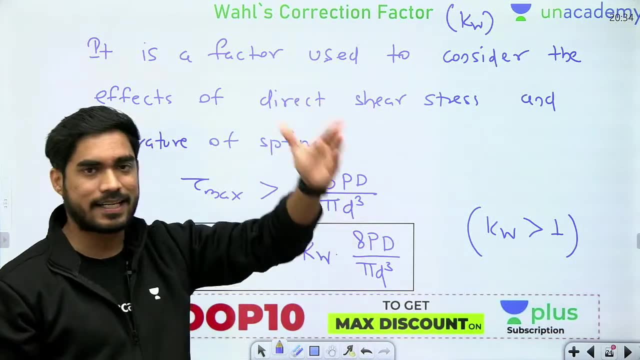 Kw will be slightly greater than 1.. So, my brother, do you understand? what is the use of Wall's correction factor? It is used as a factor to consider the effect of direct shear stress and the effect of curvature. okay, Now how do we calculate Kw? 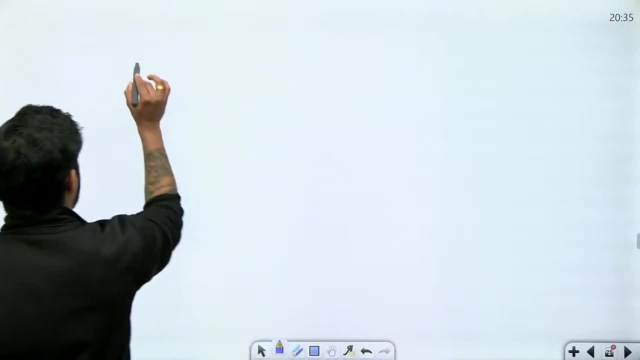 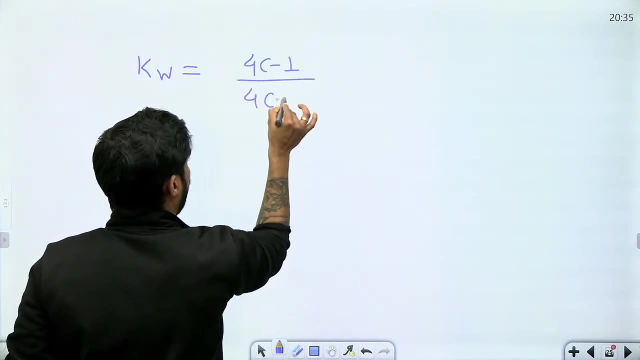 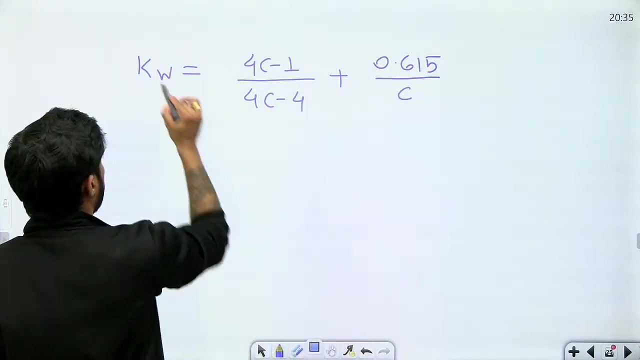 So there is an equation to calculate. Now, how do we calculate Kw? okay, What is that equation? Kw is 4C minus 1 by 4C minus 4 plus 0.615 by C. It is 4C minus 1 by 4C minus 4 plus 0.615 by C. okay, 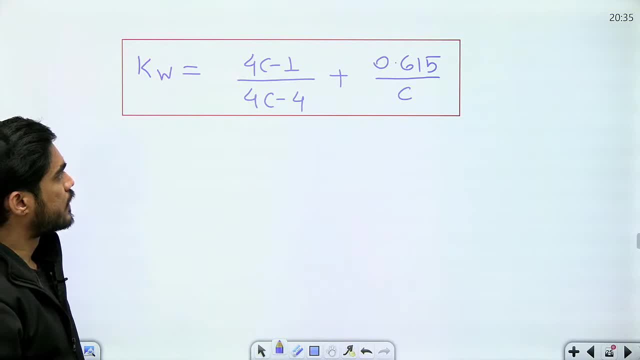 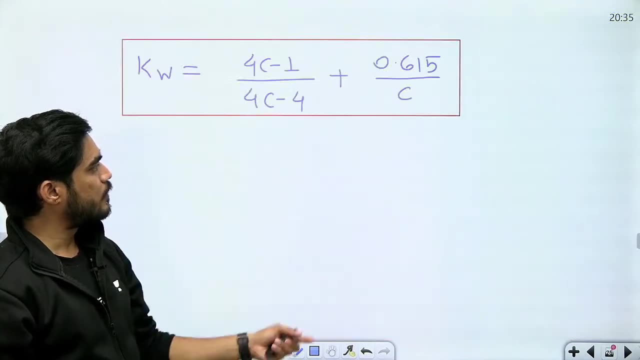 Now understand two things here. First of all, this equation is important. This is not. This equation is very important because in exam they will directly ask you: what is Wall's correction factor? okay, So it is very important to remember this equation. 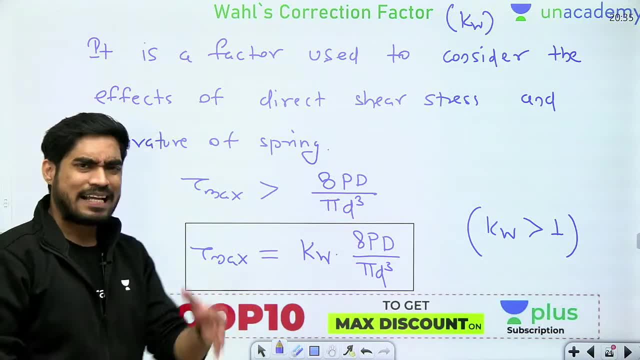 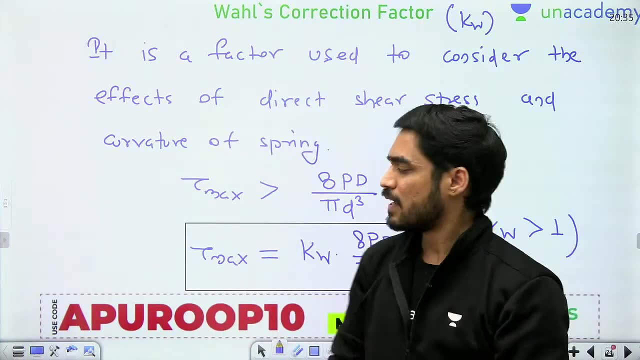 But this equation you don't have to remember. Why? Because they will never ask you to calculate tau maximum using Kw. It is never said to use Kw to calculate tau maximum. I am telling you this so that you understand what is Kw. 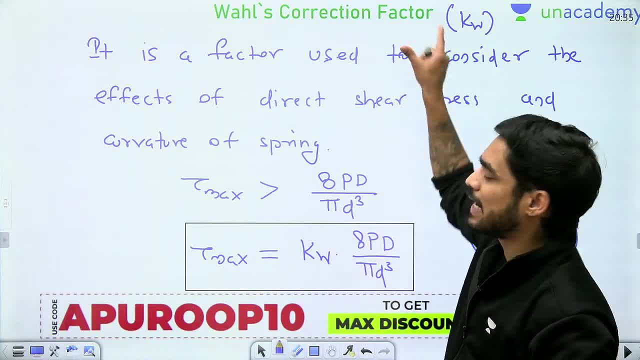 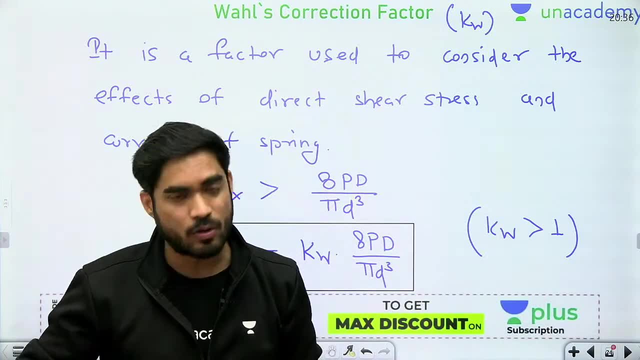 I am just telling you this so that you will understand where Kw is used. Otherwise, you will never use Kw in the calculation. You don't have to take Kw in the calculation. You don't have to take Kw in the calculation. In the calculation you always need to use. sorry, 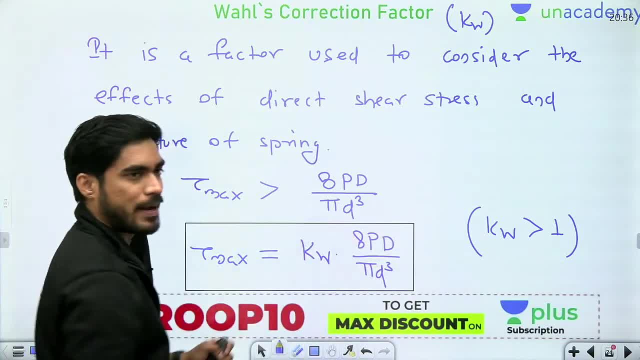 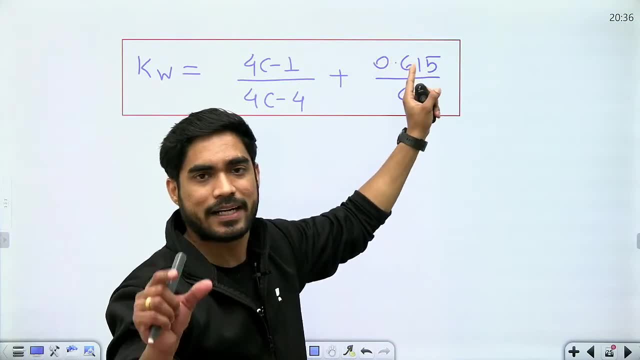 In the calculation you always use this direct value, 8Pd by Pi d cube. But you need to remember this equation because they will ask you to find, they will ask you directly, in theory, what is Wall's correction factor, What is the equation? 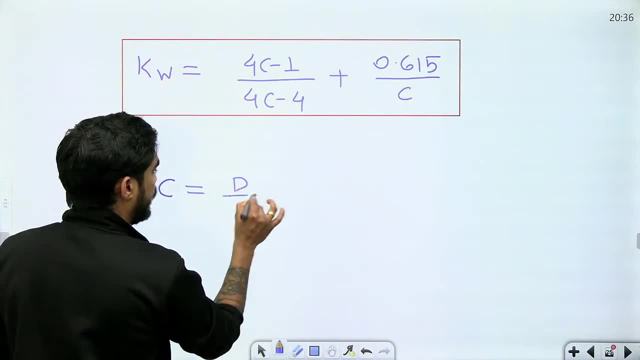 Okay, Now in this equation C is capital D. Now in this equation C is capital D. Now in this equation C is capital D, And this is known as spring index. Now, this is very important. why? 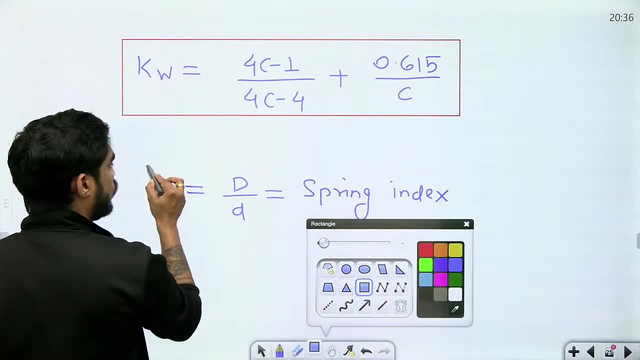 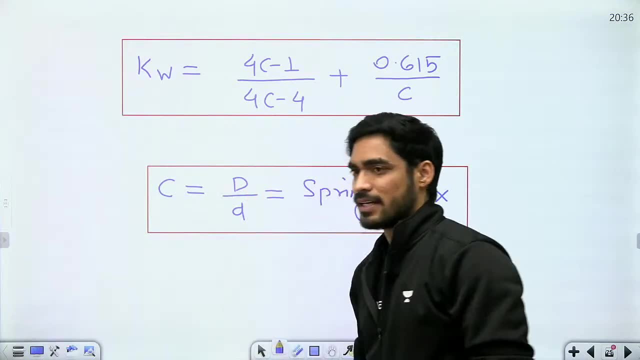 Because when you're designing the spring, you need to make sure that this value is greater than 10.. This value should be higher than 10, okay, Whenever you design the spring, always the spring index should be higher than 10.. That we need to ensure, okay. 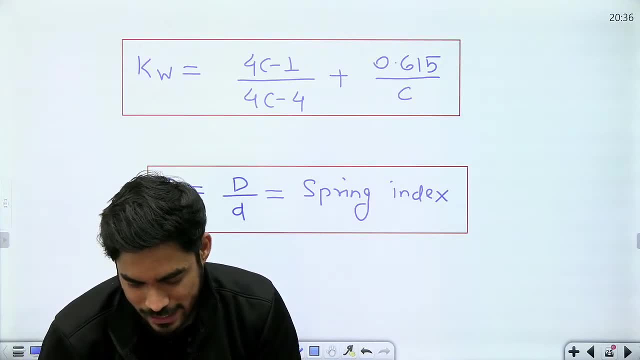 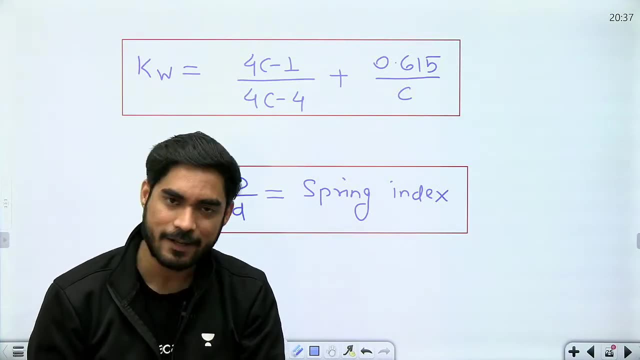 My brother, you take torsional, shear stress. Talking about torsional, you know how to derive the entire derivative right. see the entire derivation. you will not understand anything if you enter from the middle. Mahendra Reddy, you just look at the entire derivation. Okay, You just look at the entire derivation. 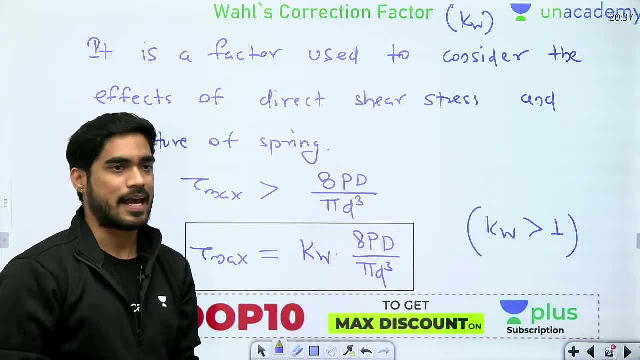 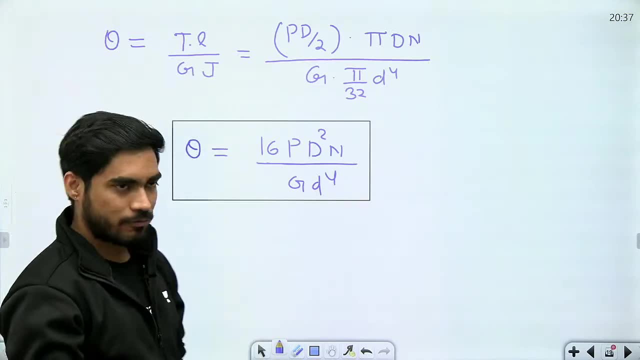 Brother is still not clear that this is torsional shear stress. So see the entire derivation. You get up from the middle and see this equation, Sir, where is torsional shear stress in this? So, my brother, look at the entire derivation, look at the entire lecture. Okay, Follow the. 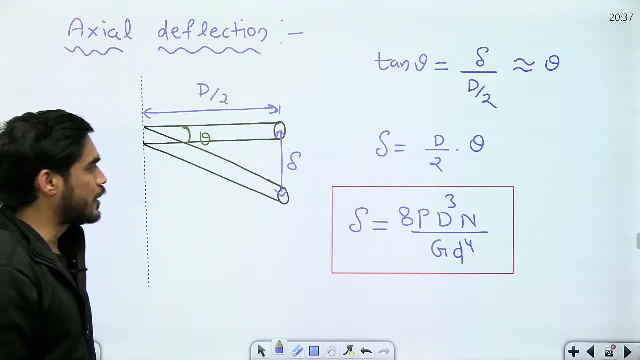 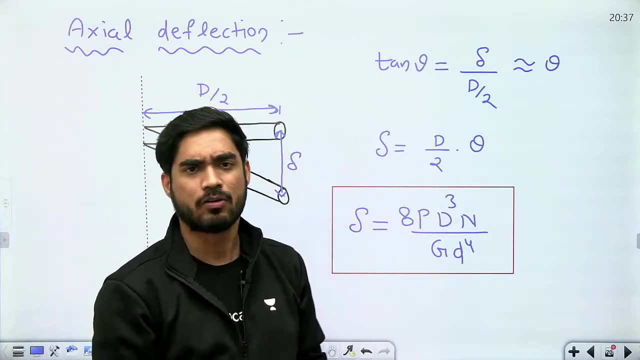 lecture: Don't get up after sleeping in the middle. Okay, You have taken a nap in the middle and then you are saying: where is torsional shear stress? I will ask questions on it. I will check on it. So, my brother, first look at the entire derivation. Okay, So now my 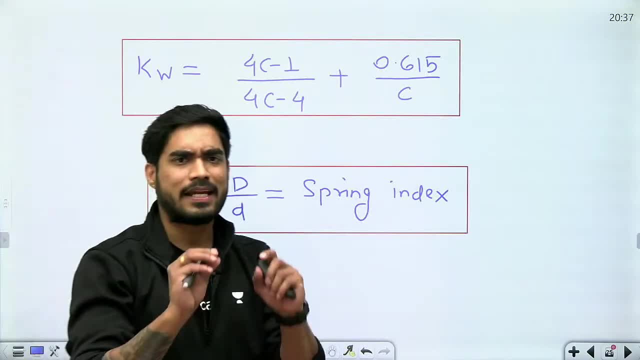 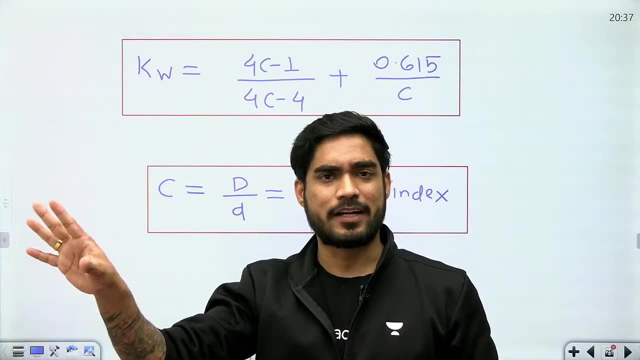 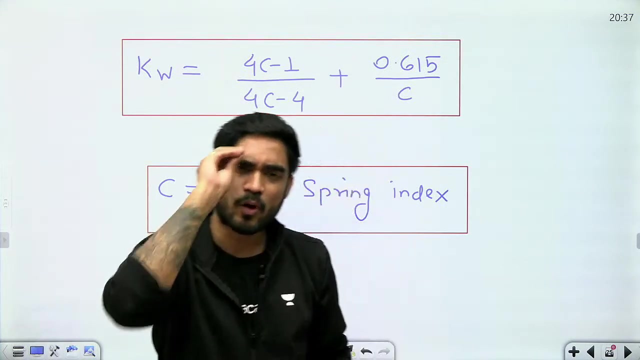 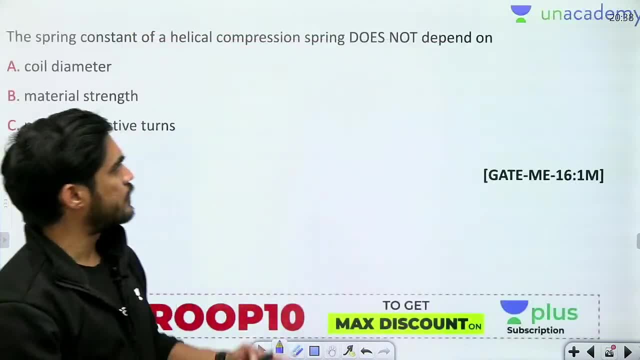 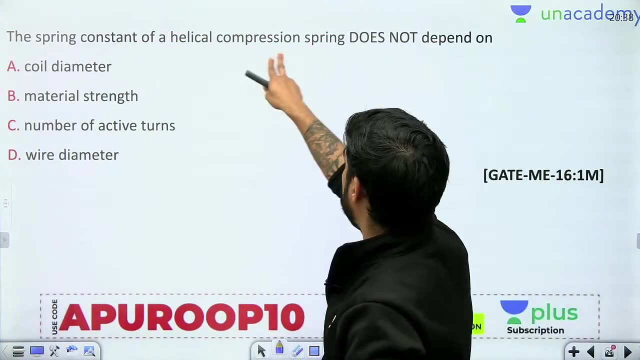 there are 5-6 questions, Okay, So let me solve those questions for you. Okay, So this is the first question in GATE 2016.. One more question: The spring constant of a helical compression spring does not depend upon. Now look at this term: Spring constant, Okay. 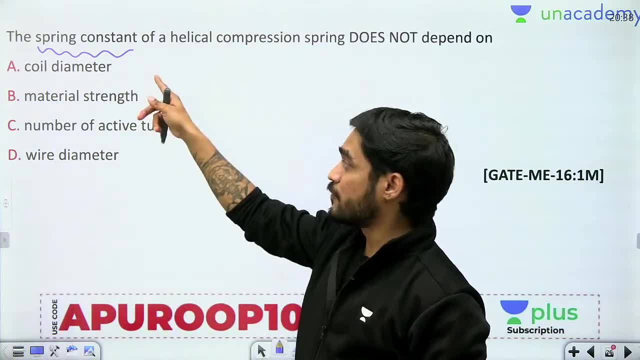 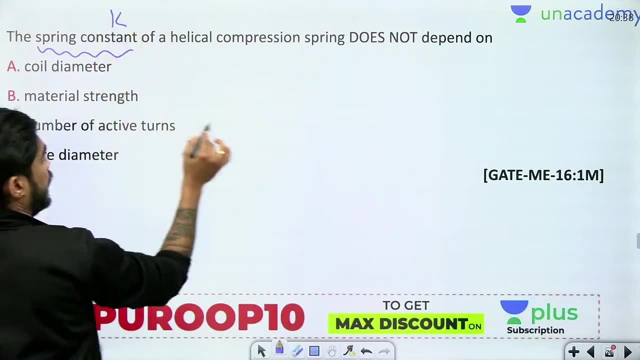 This is what I was talking about. In this year, a lot of students could not solve this because they did not know what is spring constant. So spring constant means K. Spring constant means K. Now, if you remember the equation of K, then, my brother, what is the? 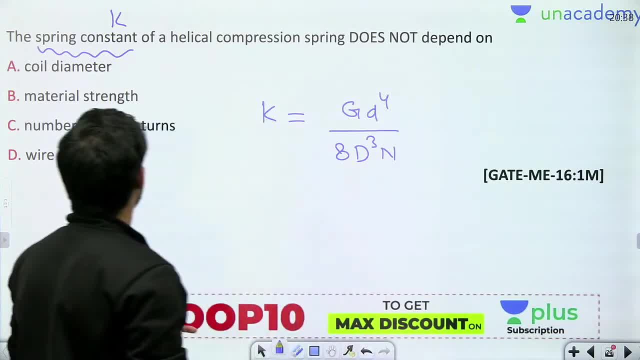 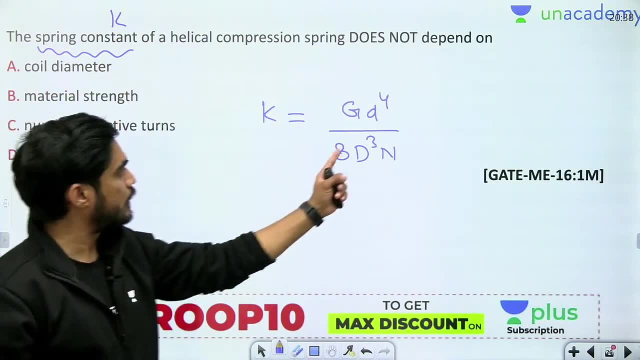 spring constant, So GD to the power 4 by 8D cube N. So, my brother, spring constant does not depend upon which, So it depends upon coil diameter. Material strength means material strength is visible in this equation. What is material strength? Tau maximum is: 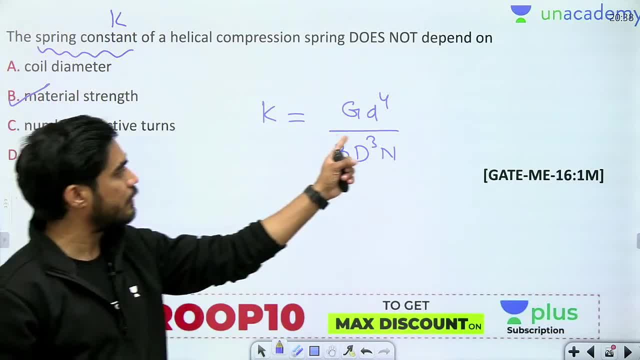 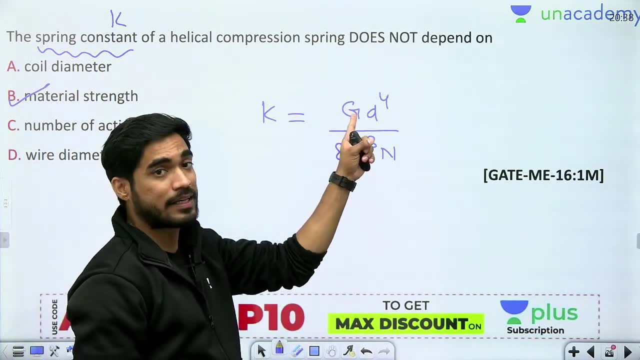 material strength. So, son, it does not depend upon material strength. Number of active turns depends upon yes. Wire diameter depends upon yes. Okay, This is not material strength. This is G is not material strength. Material strength means, my brother, what? 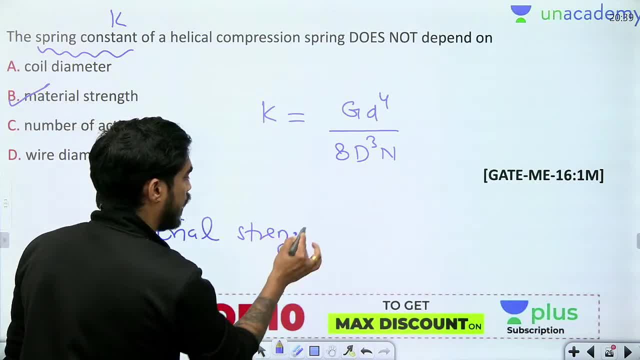 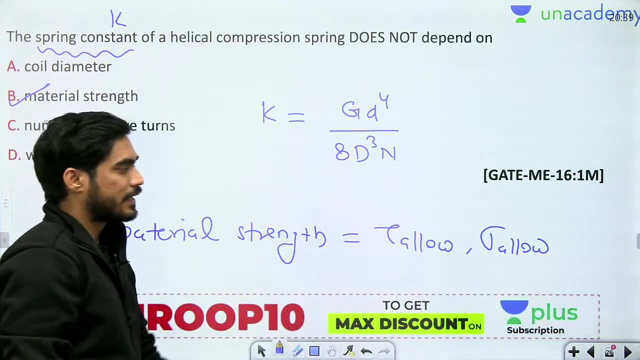 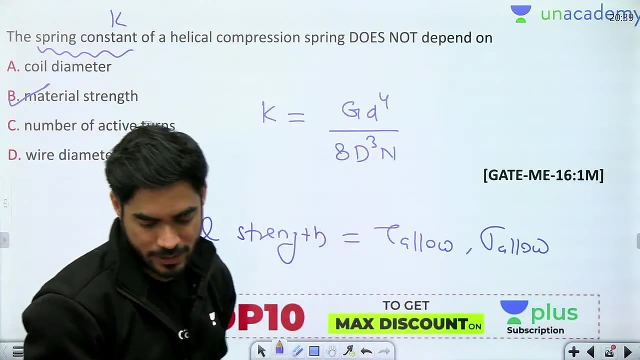 Material strength means tau allowable, Tau allowable, sigma allowable, that is material strength. Okay, How much stress you can allow, that is material strength. But material strength is not G. Okay, Don't think that G is material strength. G is material property, but it is. 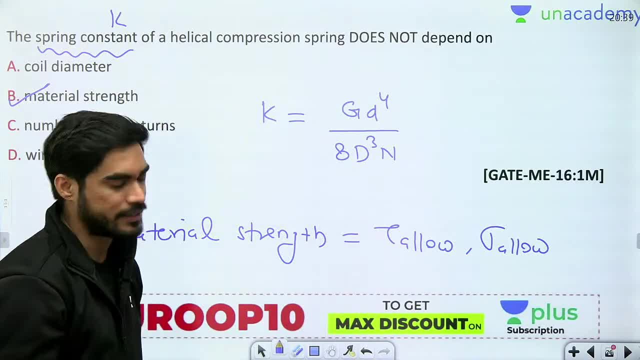 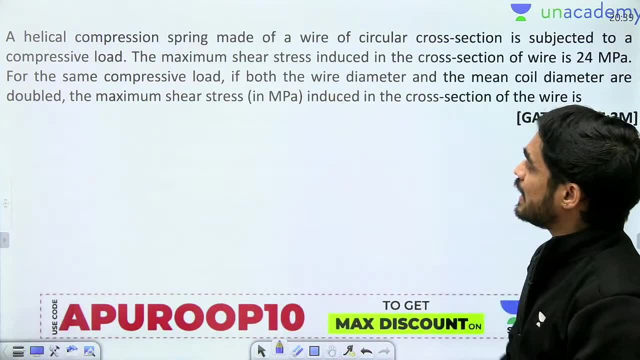 not a strength property. Okay, It depends upon stiffness, not strength. Yes. Next question, my brother, This is from Gate 2017, 2 marks question: A helical compression spring made of a wire of circular cross section is subjected to. 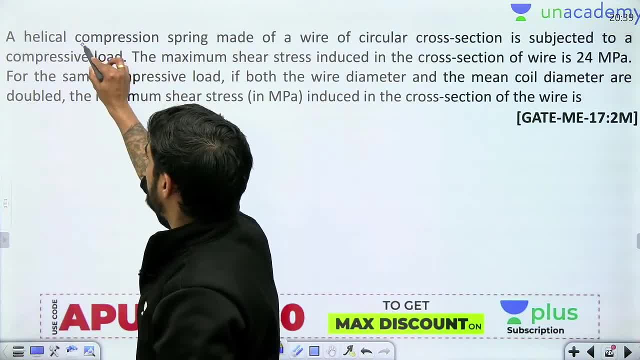 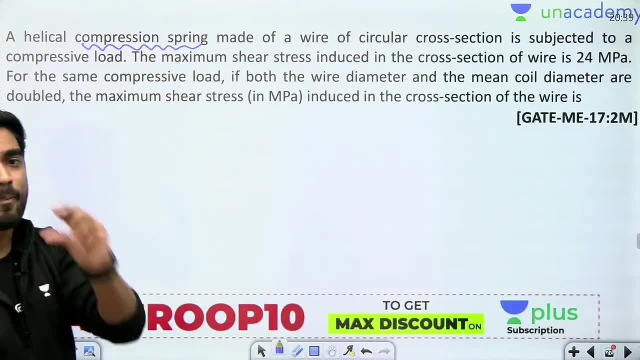 compressive load. Now, one thing to be taken care of here is that they have said that compression spring. But, son, you don't have to worry, Compression spring is actually open coil spring. So a lot of people think that this is a question of open coil, How we are going to solve it. 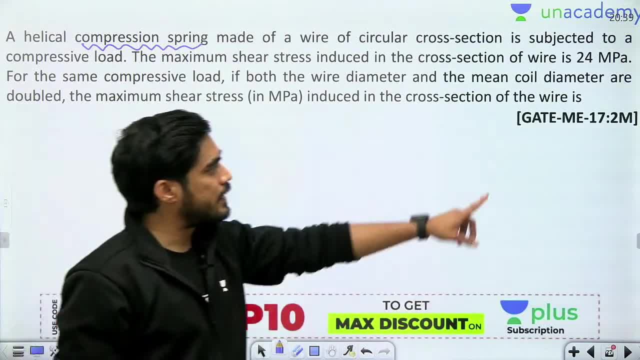 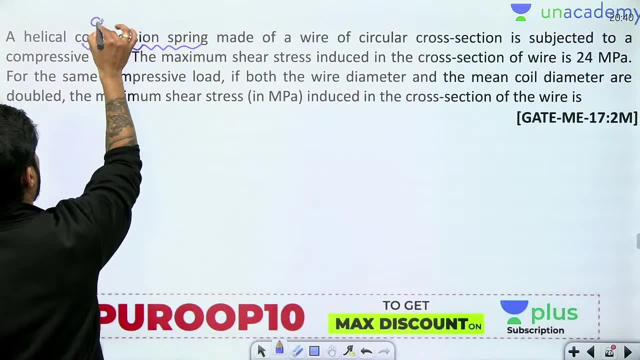 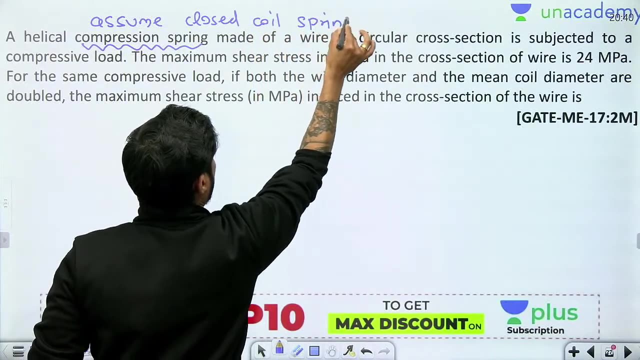 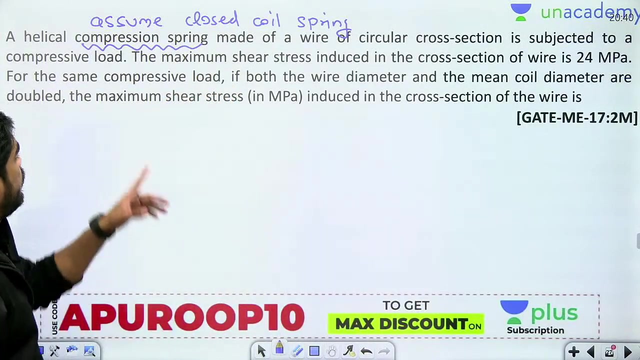 But, son, you need to understand. if there is a question of spring in gate or any exam, always a close coil spring. Okay, Assume close coil spring only. Whether it is compression spring, open coil, write anything, Assume close coil only. Okay, So my brother maximum. 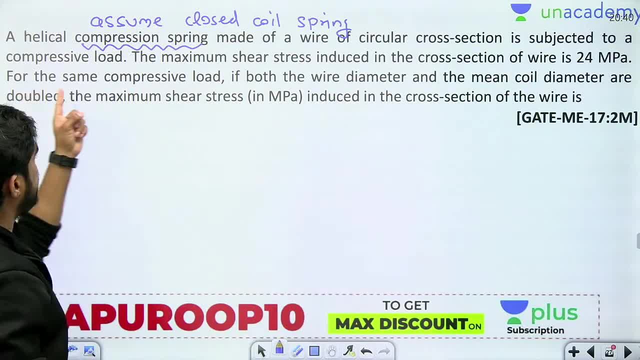 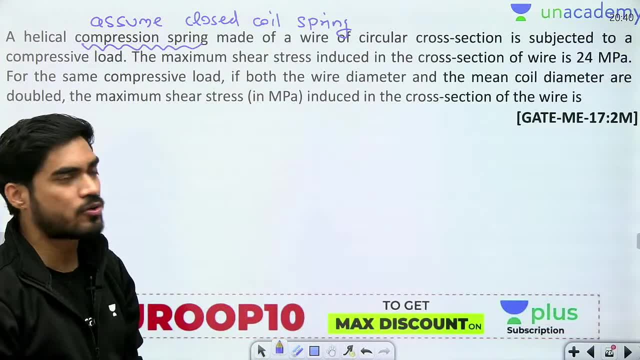 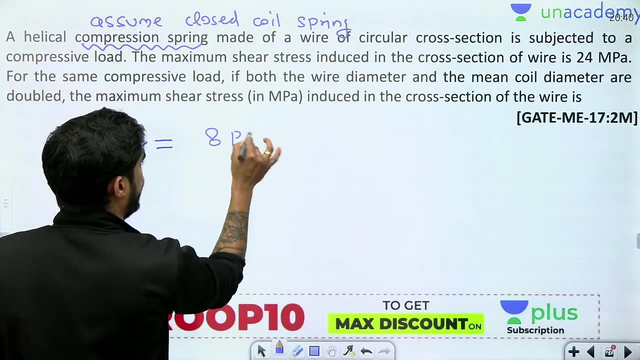 shear stress is 24 MPa. Now for the same compressive load. if both wire diameter and mean coil diameter are doubled, then the maximum shear stress induced will be: So understand my brother. Tau maximum is equal to what 8 PD by pi d cube. Right Now, tau maximum, 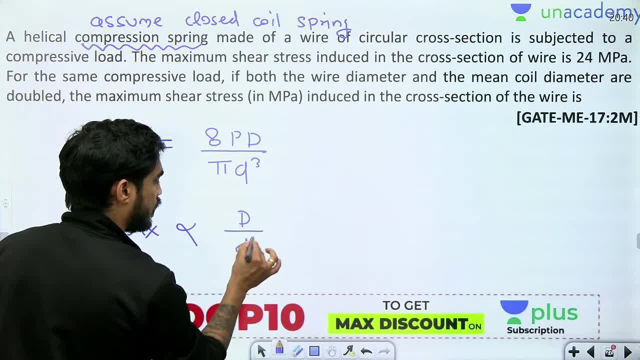 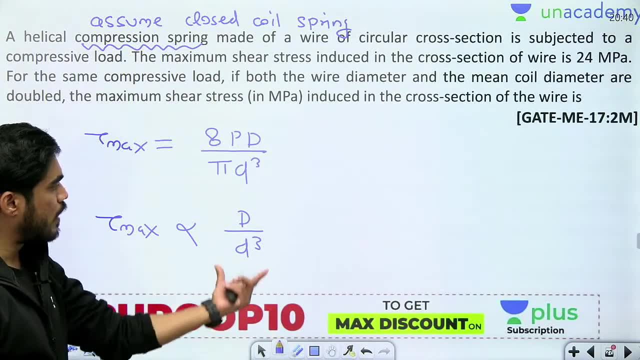 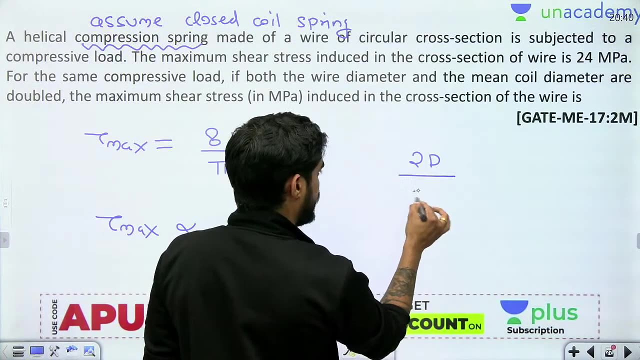 can I say it is proportional to capital D by small d cube: Yes, Now if I double both these things, then what will this quantity become If I double this, if I double this too, if I double this too, or if I double this too? 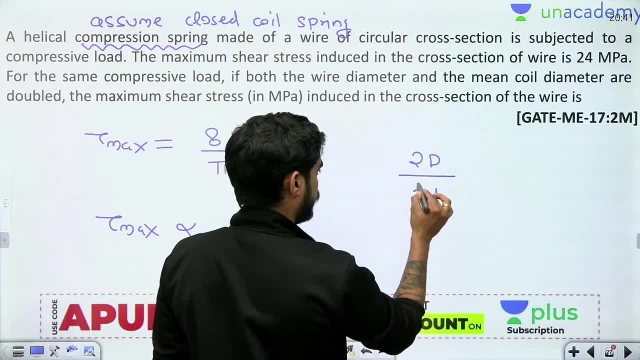 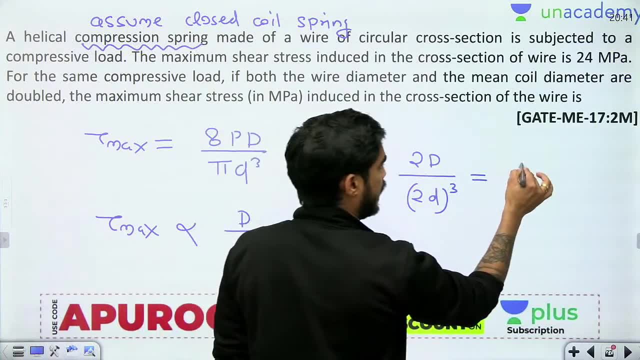 So what it will become? So this will become 2 by 8 means 1 by 4.. It will become 1 by 4, right? So, my brother, 24 divided by 4 will be the answer, If I double this too. 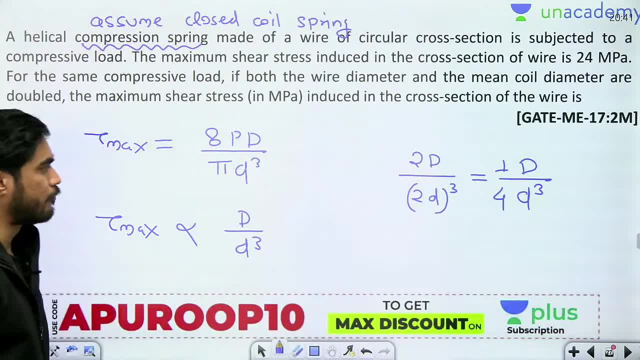 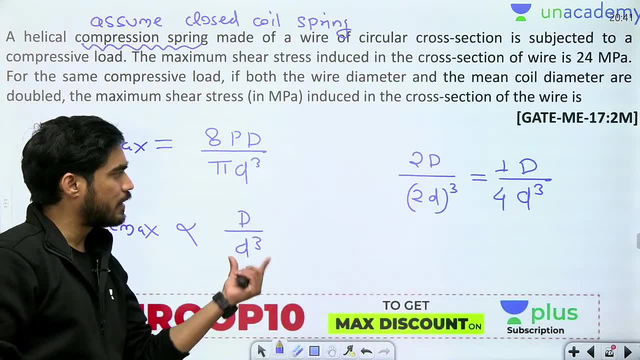 if I double this too, what I will get below W will get 4, means my tau maximum will be 1, four. So my brother, 24 divided by 4 will be the answer. Now what it will become. 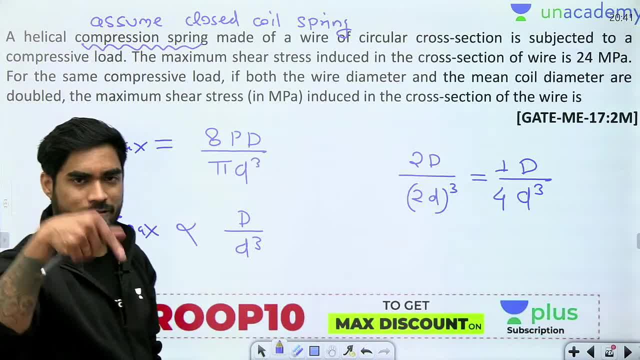 If I double this also, this also, then I will get 4.. It means my tau maximum will become one fourth, then also Hebrew. So I am Now whatever I have, but I forget to write what. So now my answer will be 6 MPa. 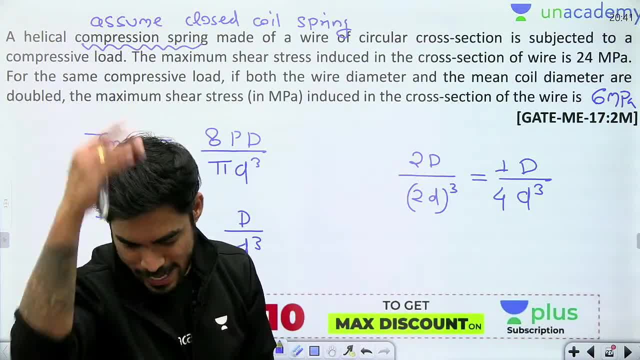 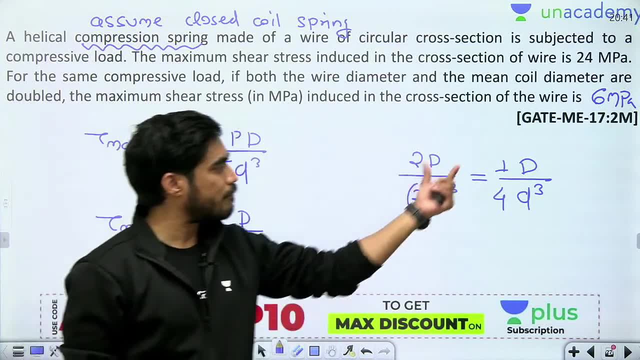 Simply 6 MPa. Yes, it was 6 MPa. Yes, it was 6 MPa. Very easily Double capital D as well as small d. So my brother, 1 by 4 will be the answer. 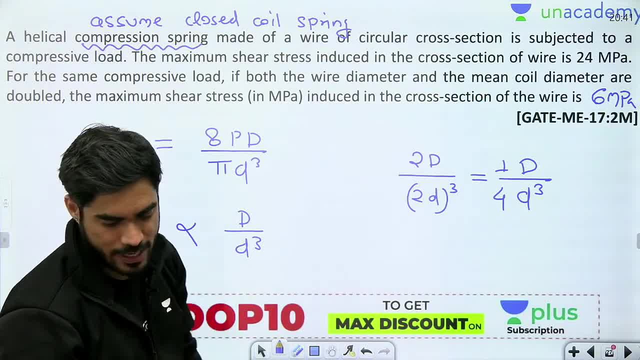 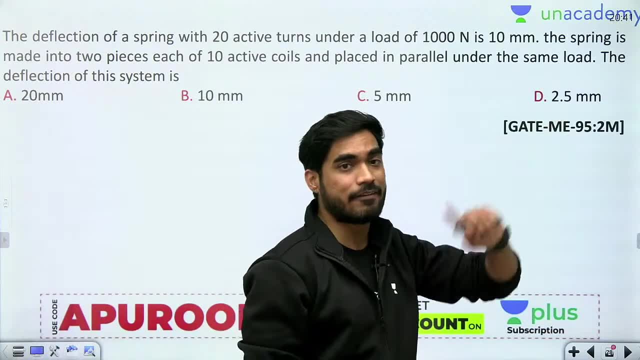 So 1 by 4th of 24 means 6 MPa. Very good, Very good, Very good, So simple. Gate 2017's 2 mark question. Next question is from gate 1995.. Now you might be thinking: why did you take such an old question? 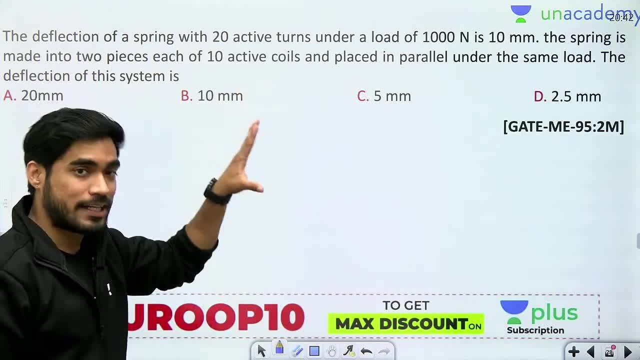 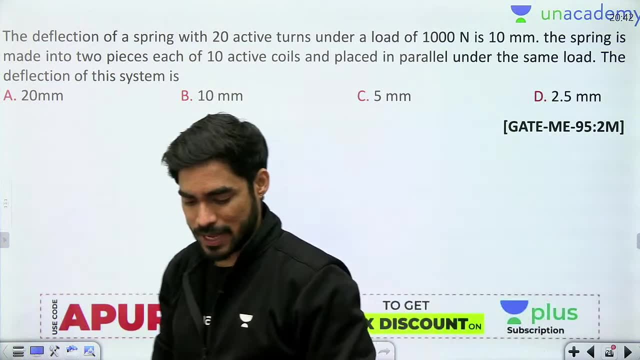 We were not even born then. But, my brother, this is a very interesting question and it is repeated in quite some exams, Not in gate, but in other exams. it is repeated quite sometimes. Okay, So, my brother, let's see what is this question? 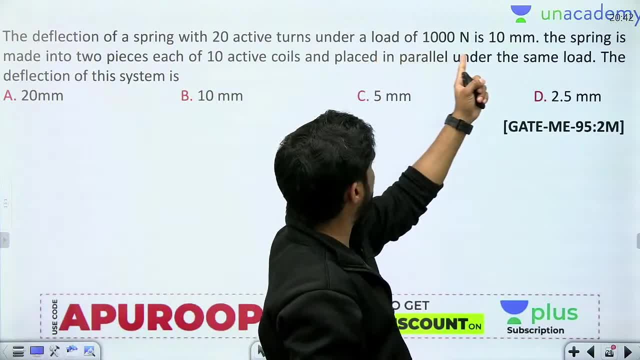 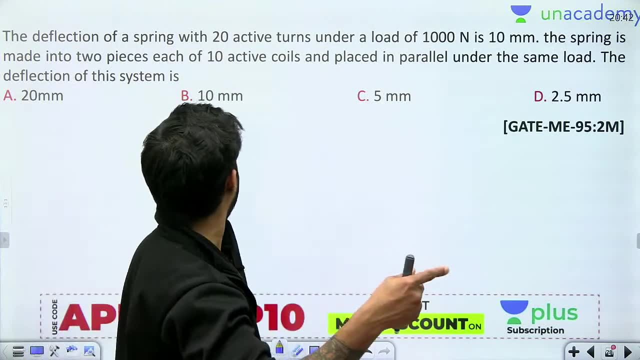 The deflection of spring with 20 active turns under a load of 1000 Newton is 10 mm. The spring is made into two pieces, each of stiffness, each of 10 active coils and 20 active coils Placed in parallel under the same load. the deflection of this system is 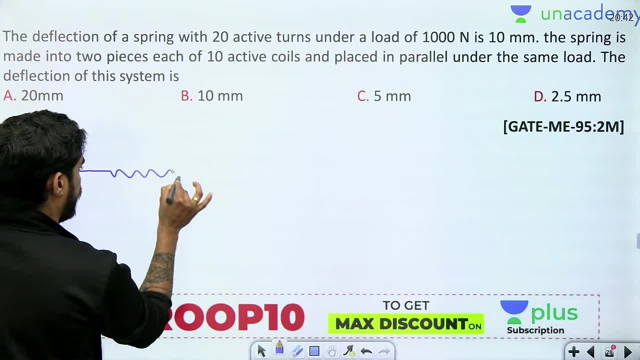 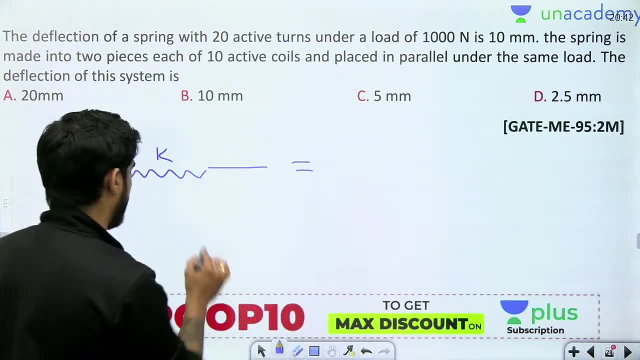 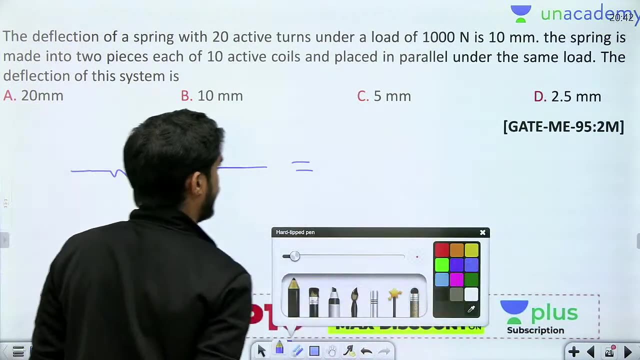 Now understand. What is happening is right now. I have a single spring, Okay. Now what is he saying? I have cut this single spring into two parts. Okay, I have cut this spring into two halves. Okay, I have cut this spring into two halves. 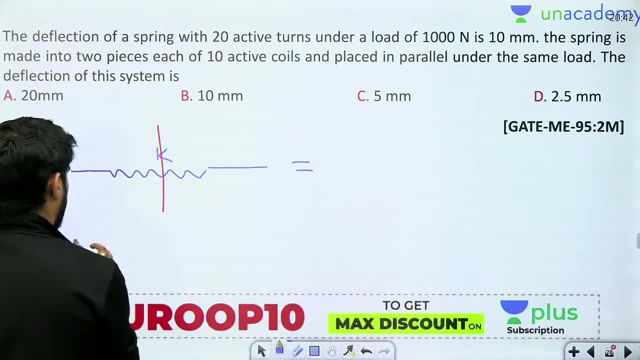 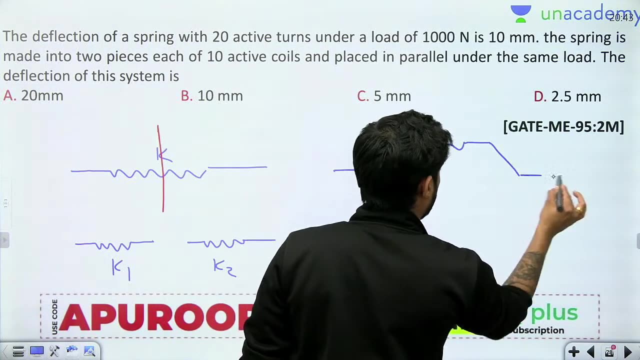 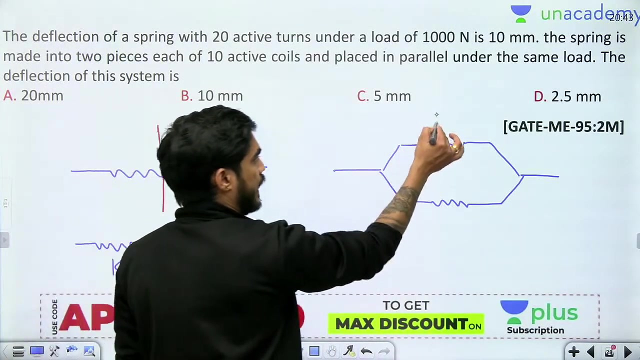 I have cut this spring into two halves. This is what happened: K1 and K2.. Now, what I did is I connected K1 and K2 in parallel. Okay, Like this Now my brother: I connected K1 and K2 in parallel. 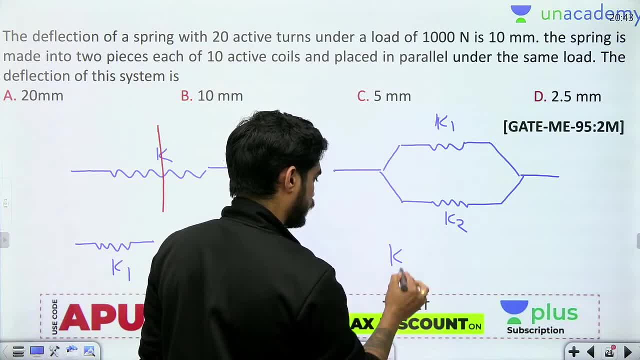 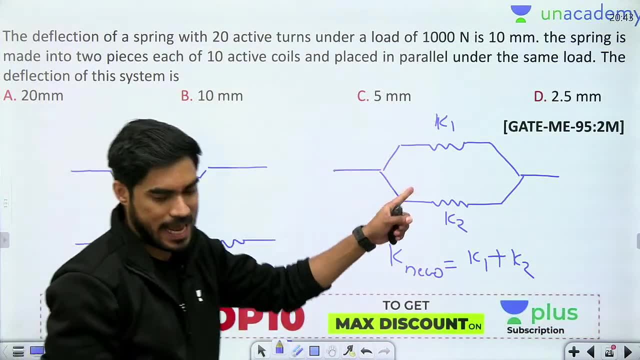 So what will be? K equivalent, K, new, K new will become K1 plus K2.. Okay, In parallel connection I directly add In series connection: 1 by K equals to 1 by K1 plus 1 by K2.. 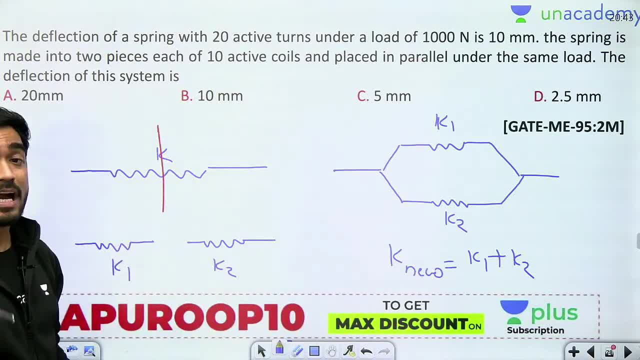 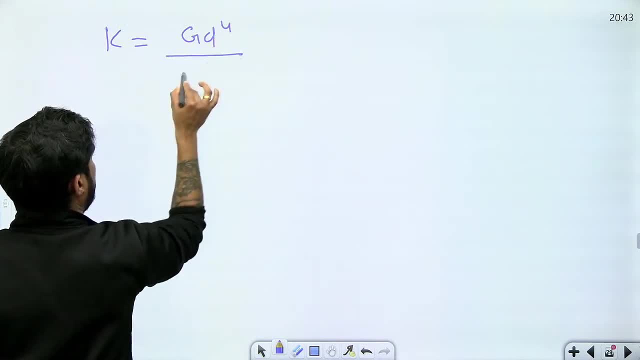 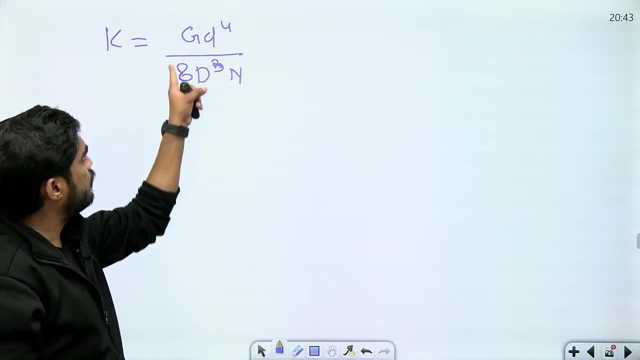 That all you remember. right Now, my brother, what will be the value of K1 and K2?? Understand: K is GD to the power, 4 by 8D cube N. Now, when you cut the spring, then all of these parameters will remain same. 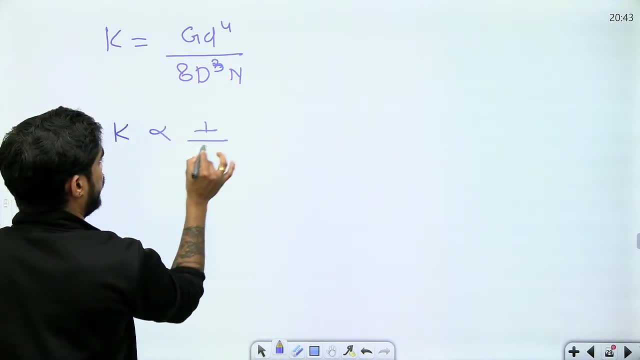 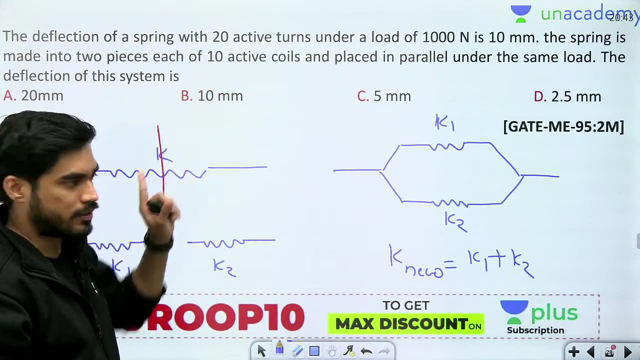 Only N will change. K will be inversely proportional to N. Now my brother. Initially there were 20 turns And now in the new springs there are 10 turns. So my N is becoming half N new. 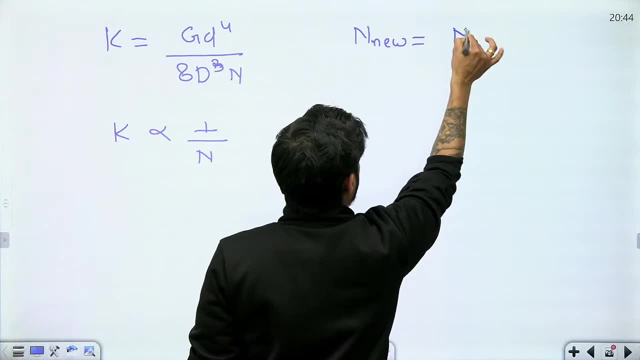 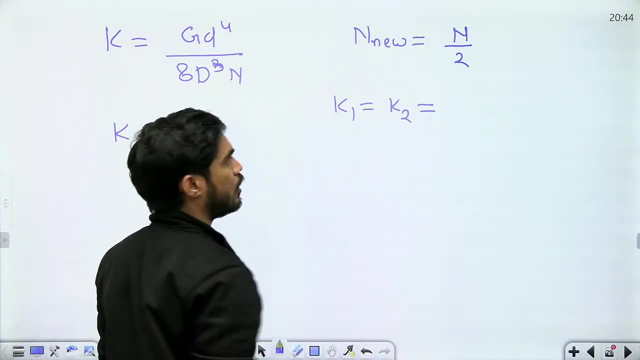 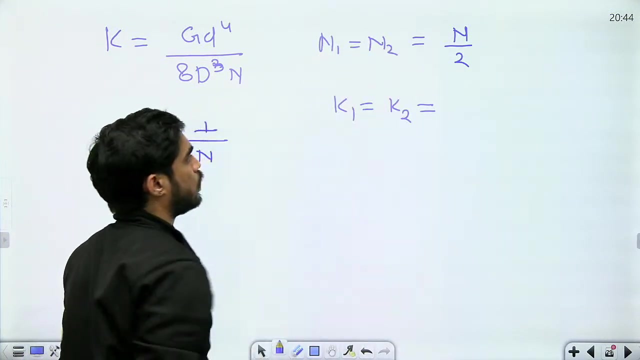 N new is N by 2.. Right N new is N by 2.. So K1 and K2 will be equal to what? Okay, I don't write N new like this. N1 and N2 are N by 2.. 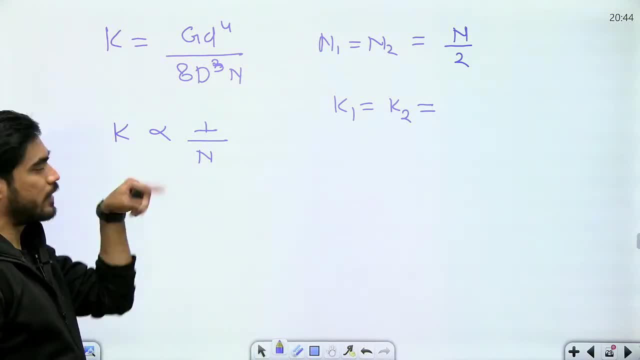 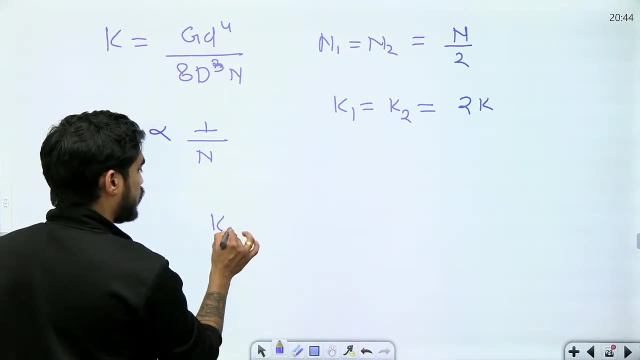 So K1 and K2 will be what? If you write N half, then what will be K? It will be double right. So K1 plus K1 and K2, both are 2K. So K new will become. how much? 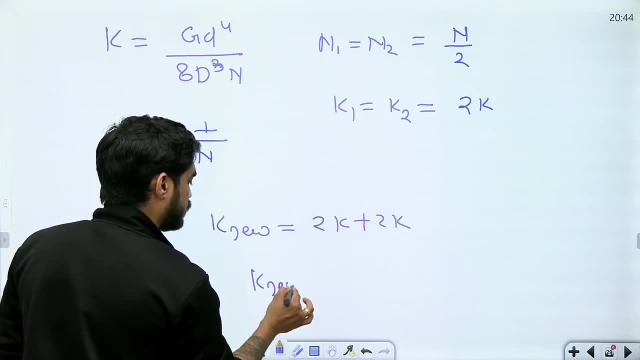 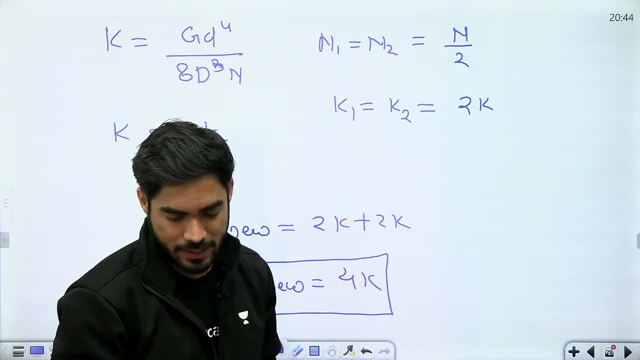 2K plus 2K, 4K. So, my brother, what is the stiffness? It has become 4 times. Stiffness has become 4 times. Initial stiffness was K And now new stiffness is 4 times K. 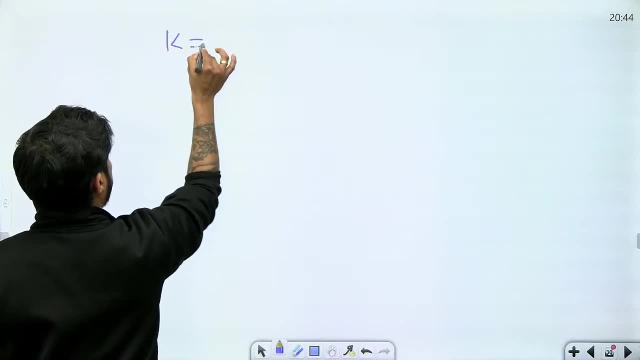 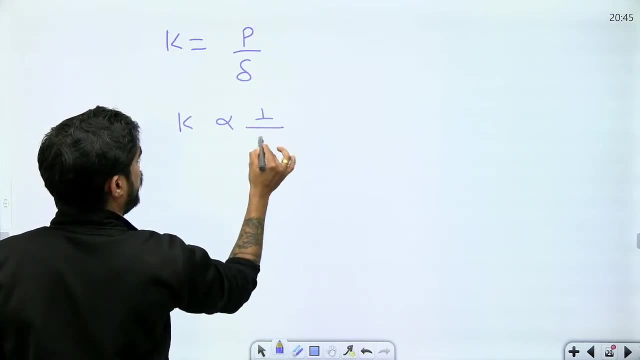 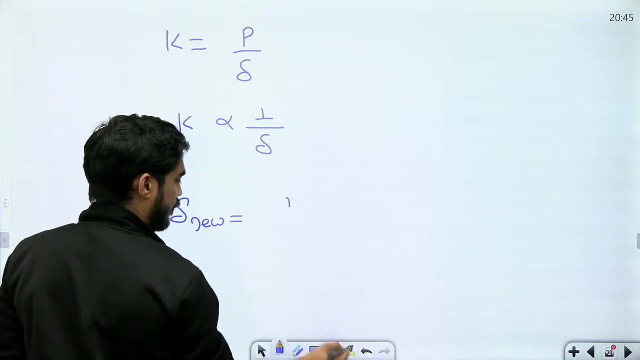 Now my brother. K is equal to what P by delta, So K is inversely proportional to delta. So if K new is 4 times, then delta new will become 1 by 4 times delta K. It is simple. 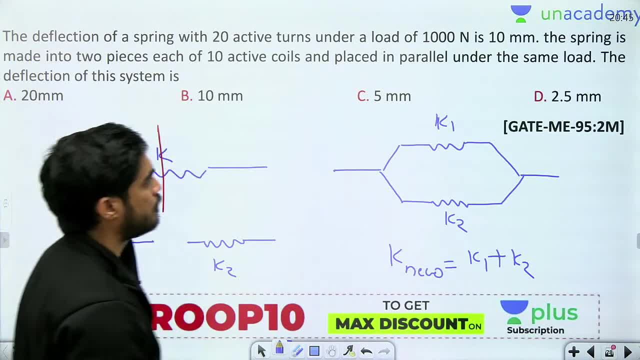 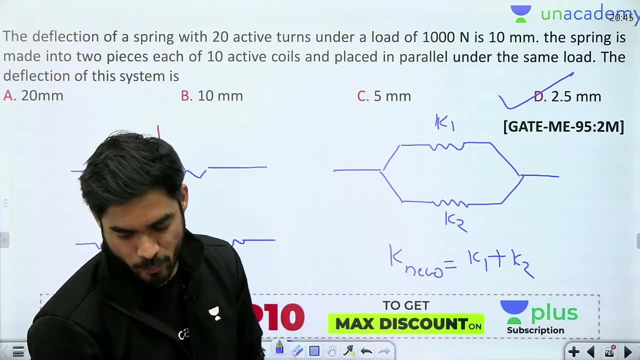 So what will be the answer here? Initial deflection was 10 mm, So new deflection will be 2.5 mm. Easy, Easy, Yes, Kalpesh, Yes, MH, Yes, Partha, 2.5 mm. 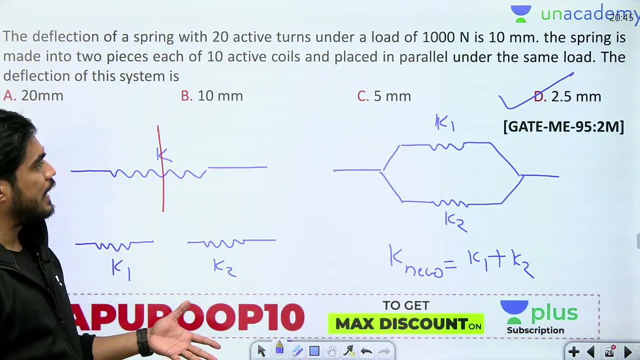 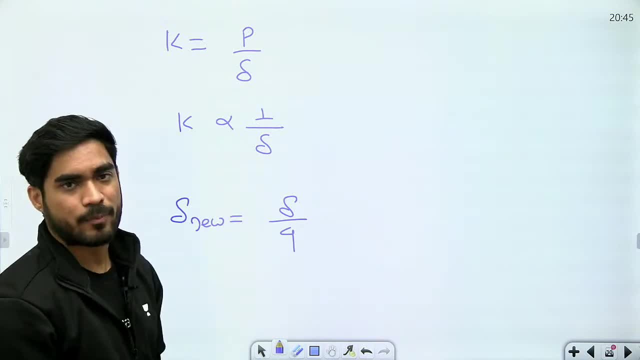 My brother look. K is 4 times, So delta will become 1 by 4.. If K is becoming 4 times, delta will become 1 by 4 times, Because delta is inversely proportional to K, Right? 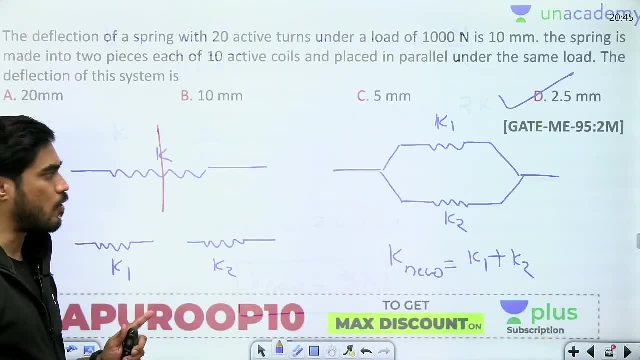 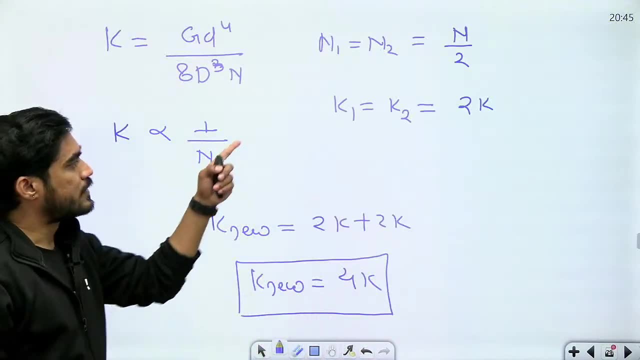 So, my brother, first we understood the concept of new K Son, if you cut the spring into two halves, the stiffness will become double. If M becomes half, stiffness will become double. Okay, Now if you connect these two in parallel, 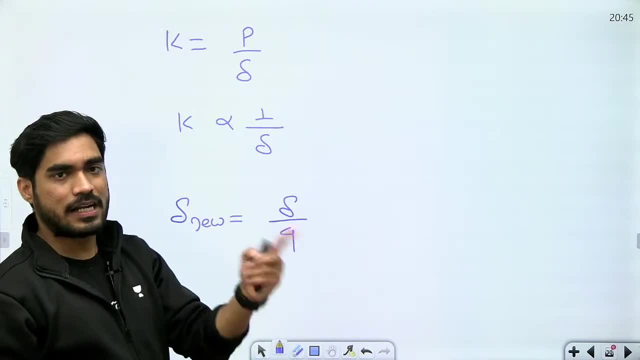 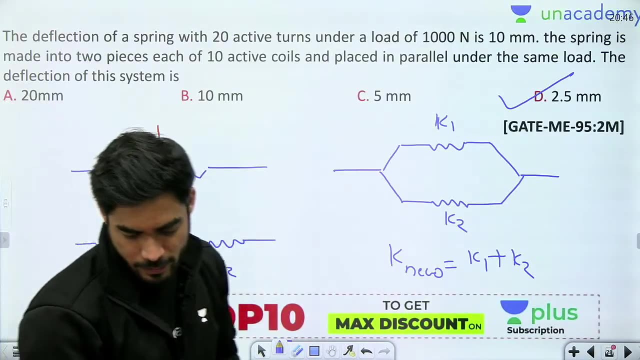 then stiffness will become 4.. If stiffness is becoming 4 times, delta will become 1 by 4 times. So that is the correct explanation. That is the correct explanation. 2.5 mm will be the new stiffness. Sorry, new deflection. 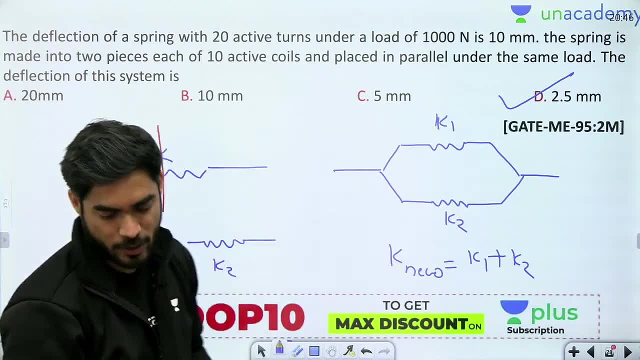 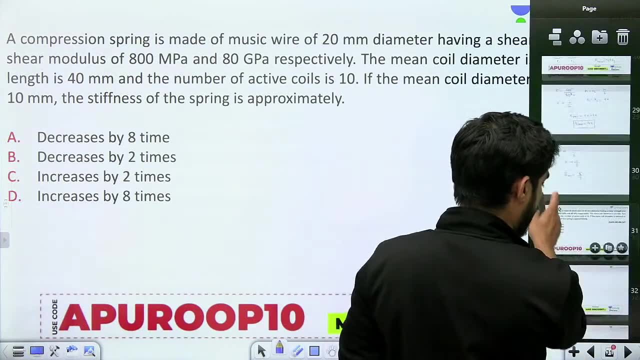 Yes, Gino, Very good, Very good, Very good. Dibyanshu, Very good, 2.5 mm. Okay, Next question. This is the next question: Gate 2008,. 2 marks, question Okay. 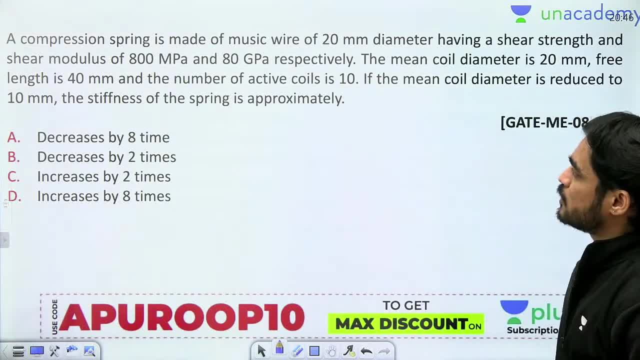 Gate 2008, 2 marks. question: my brother, A compression spring is made of music wire off 20 mm diameter, having a shear strength and shear modulus of 800 megapascal and 80 gigapascal. Mean coil diameter is 20 mm. Pre-length is 40 mm and number of acting coil is 10.. If the mean coil diameter is reduced to 10 mm, stiffness of spring is approximately. Now, my brother, what is he saying? All this is given for nothing. All this is given for nothing. 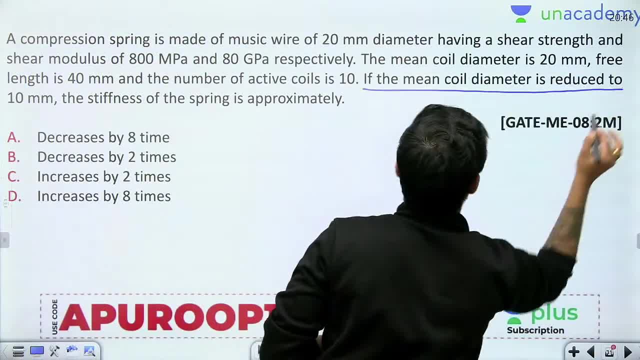 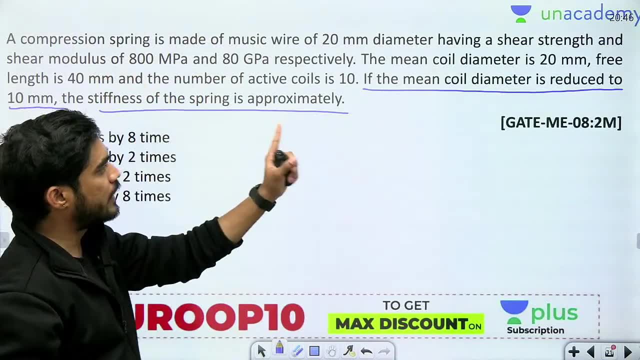 You only mean by one line. If mean coil diameter is reduced to 10, stiffness of spring is approximately. Everything else is rubbish. Everything else is rubbish. So mean coil diameter means capital D if it becomes half. Initially, mean coil diameter was what. 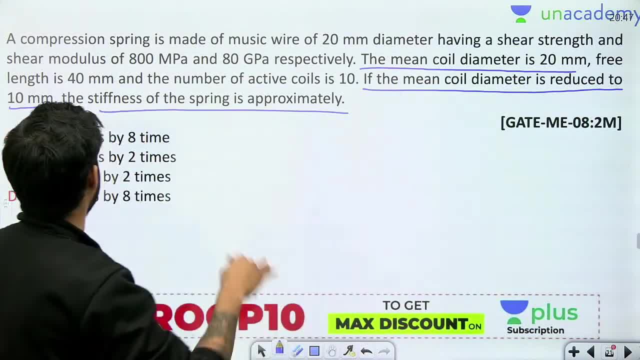 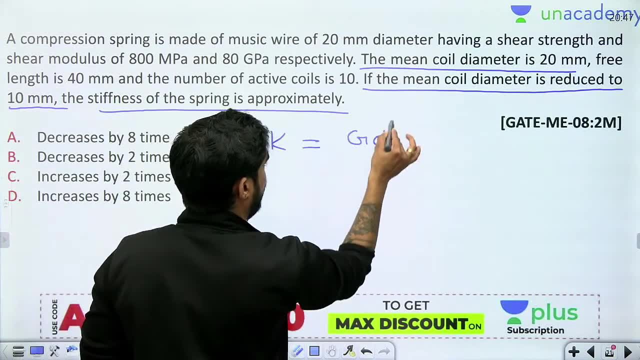 Initially, mean coil diameter was 20 mm. Now if it is reduced to 10 mm, if it is reduced to half, then what will happen to the stiffness? So K is what GD to the power. 4 by 8 D cube N. 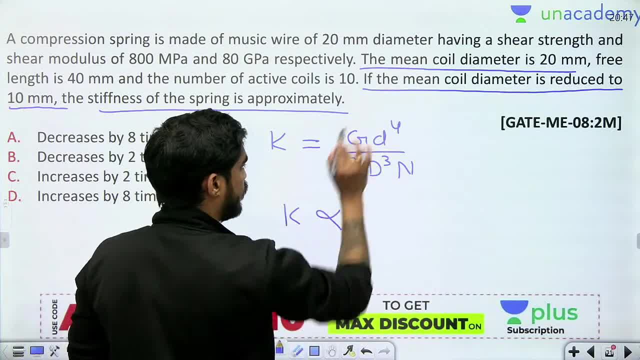 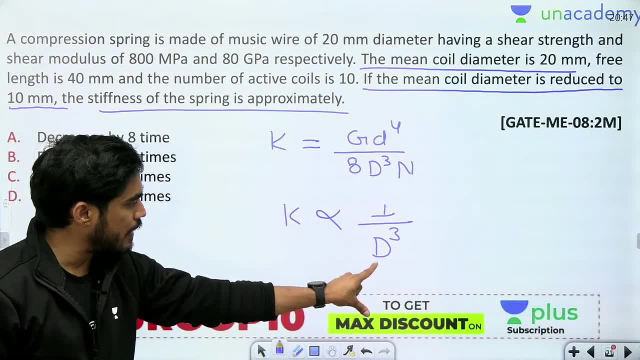 So if everything else is same, If only D is changed, then if D is reduced to half, then what will happen to 1 by 2?? It will be 8 times. This will become 8 times. Yes, Gino. 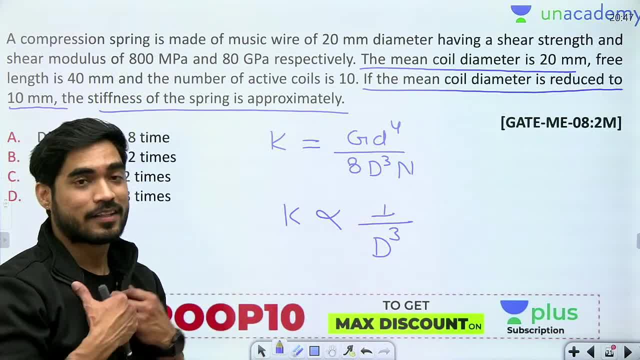 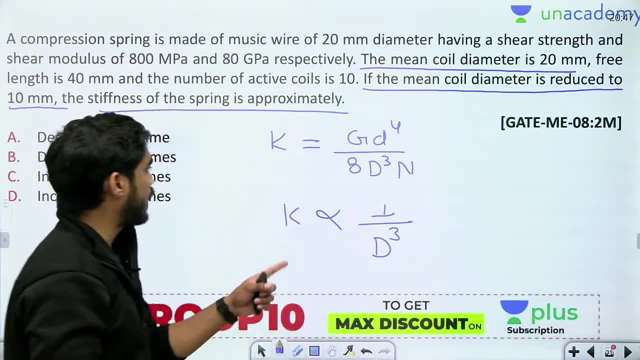 Yes, this will become 8 times. Yes, we have crossed 50.. Thank you so much for such love and support. my brother. Keep showing love like this, Keep liking and sharing such lectures. So, my brother, if you reduce D to half, then what will happen to K? 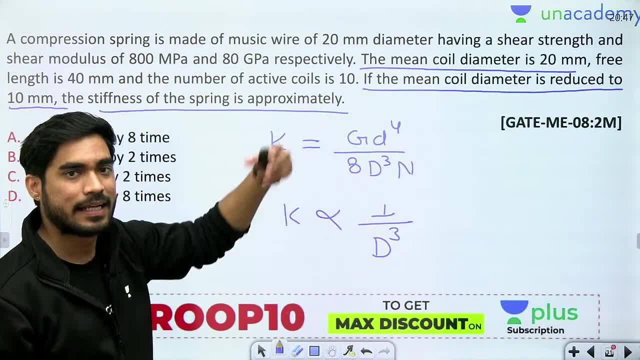 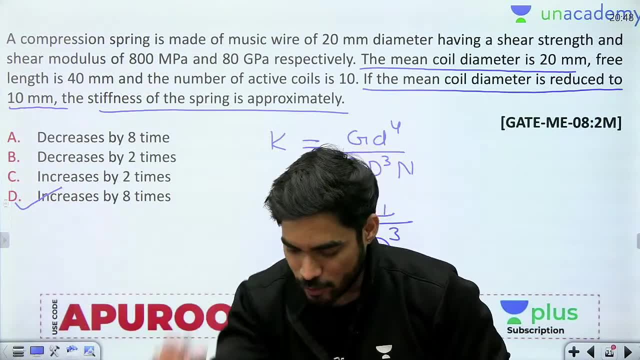 1 by 2.. What will happen to 1 by 2 cube? It will become 8 times. So it will become 8 times, Increasing by 8 times, Increasing by 8 times. Very good, Partha. 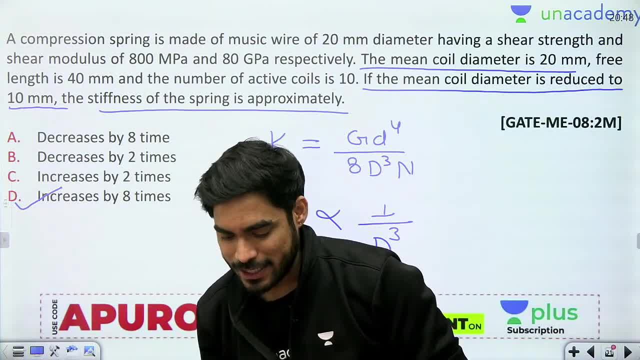 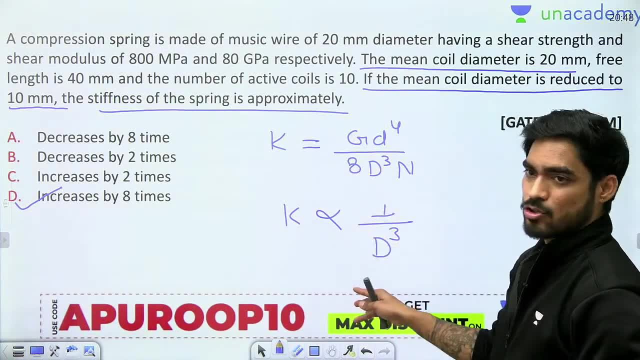 Very good. It does not decrease, but it will increase. We have not reduced D to 2 times, it has been reduced to half. If we reduce D to 2 times, then it will decrease, But if we reduce D to half, then it will increase. 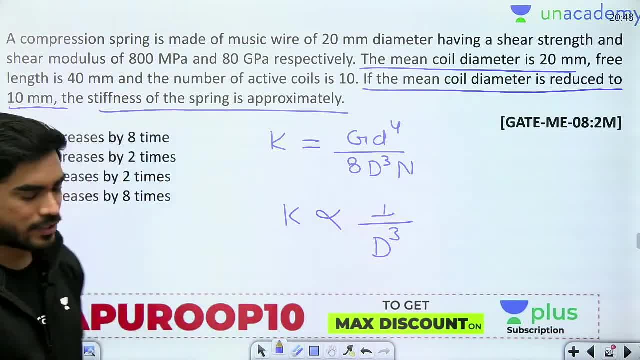 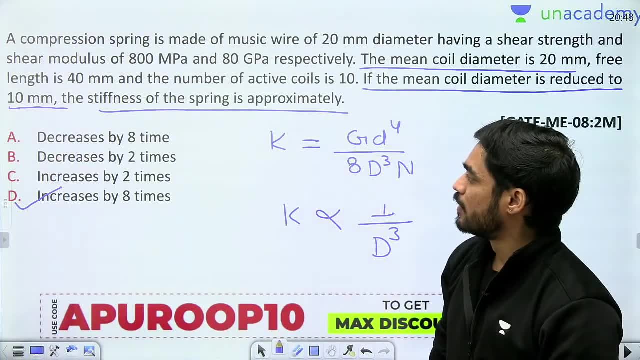 If we increase D to 2 times, it will decrease. If it is reduced to half, it will increase. increase by 8 times, it will increase by 8 times. yes, very good, very good. so, my brother, it is clear questions will be made of spring now, all the questions of gate. i have seen. 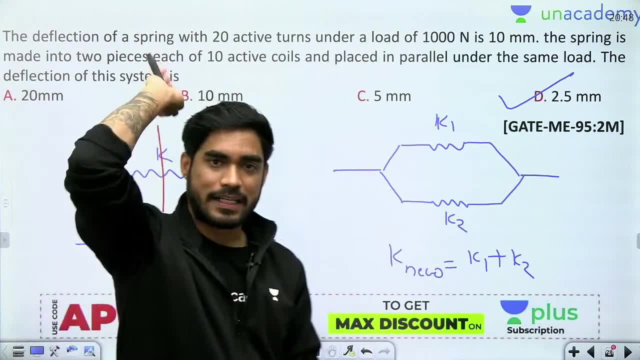 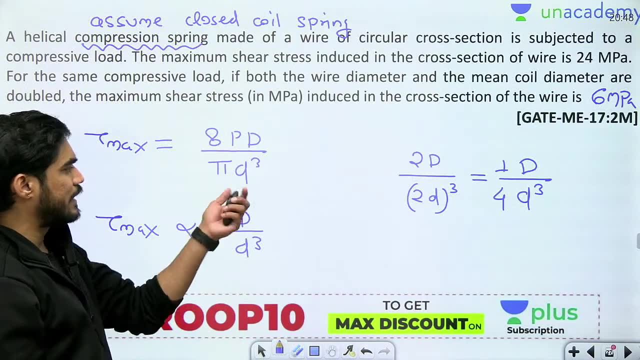 i have shown all these questions have come- you won't believe- from 95 till now. only these questions have come. ok, and you can see all the questions are made from stiffness equation and tau max equation. if you remember tau max equation and stiffness equation, you can solve. 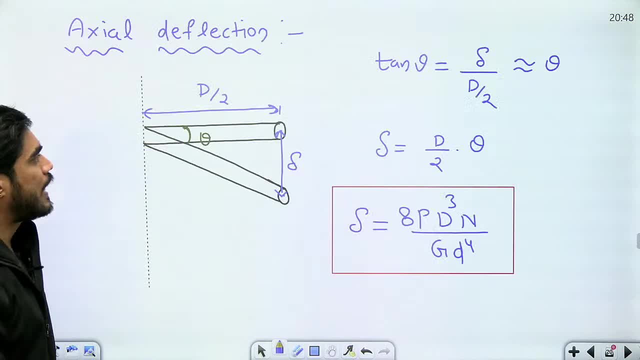 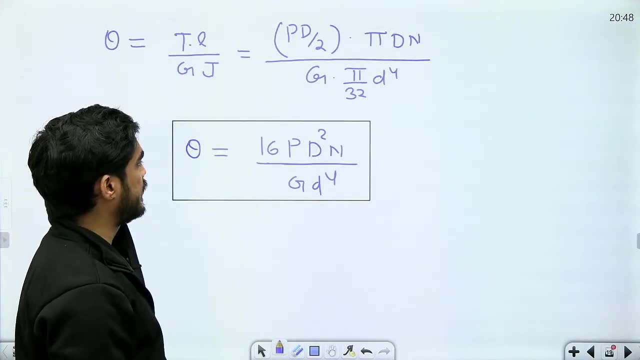 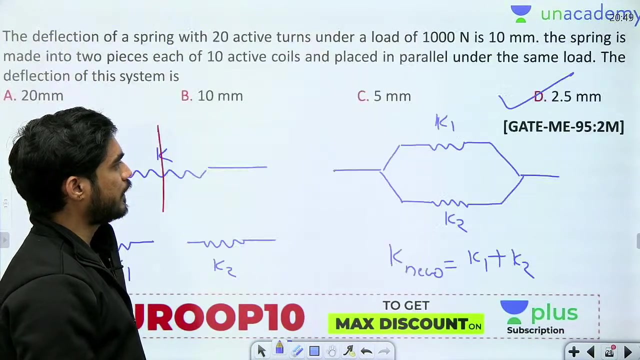 all the questions of spring, so this was all about spring. and with this we announce the end of machine design syllabus. machine design syllabus. i will announce the end of machine design syllabus- one second, let me reach to that page. so this is the end of this is the. 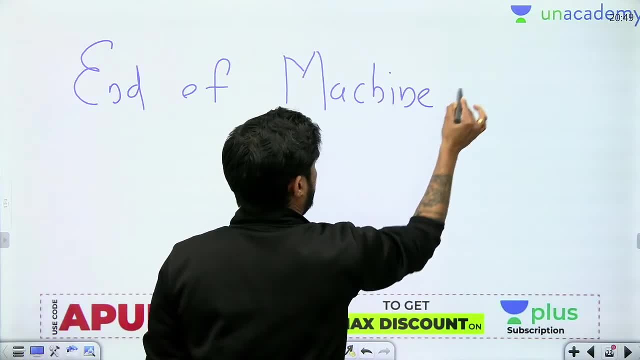 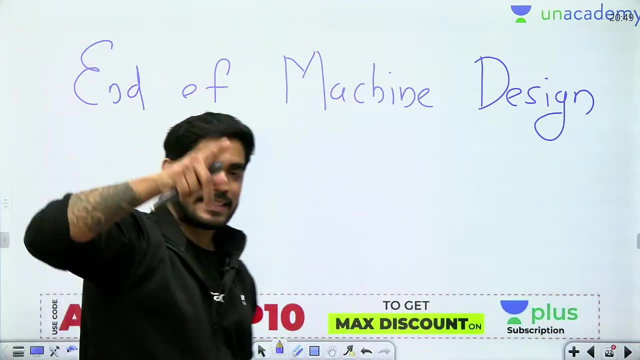 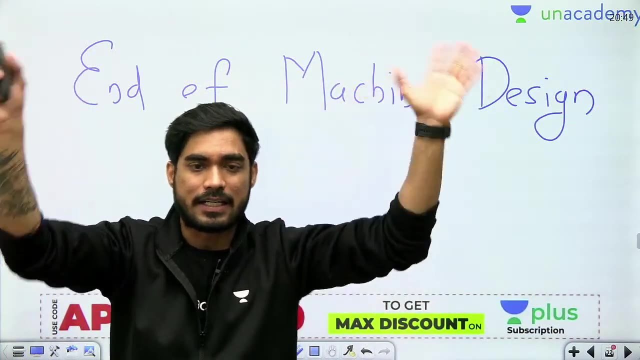 end of machine design syllabus for gate 2021, for gate 22. next year i will come back with machine designs again and i will update all the examples, i will update all the content. so, my brother, it will be a new playlist, ok. so, my brother, thank you so much for all the love and support you have. 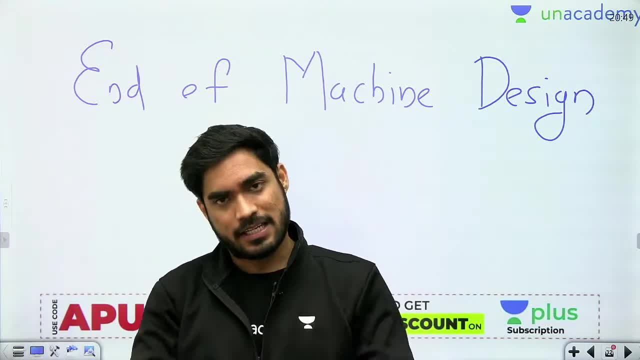 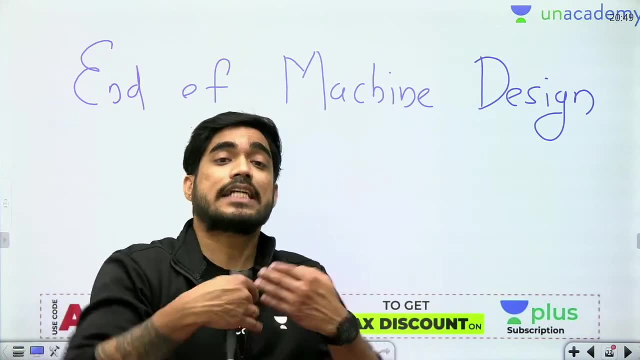 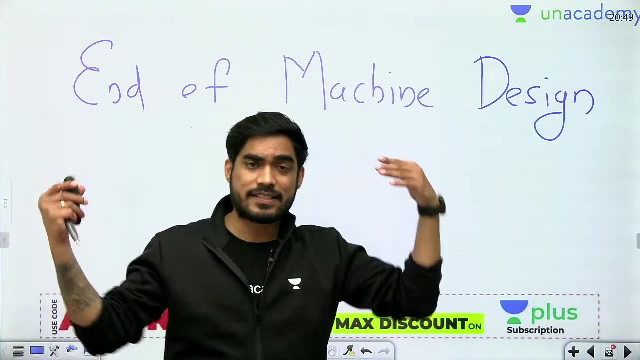 shown till now, all the love and support you have shown till now. thank you very much. and don't watch these lectures by yourself. only share them with your friends and family, because this is our moral duty, why we are doing all this, why we are taking these lectures every. 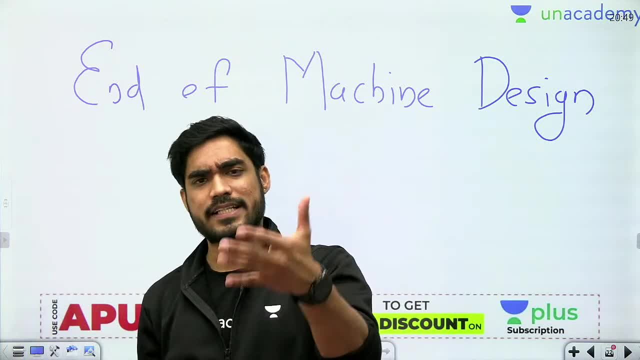 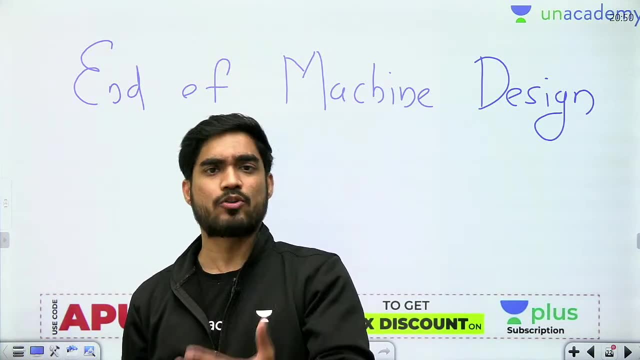 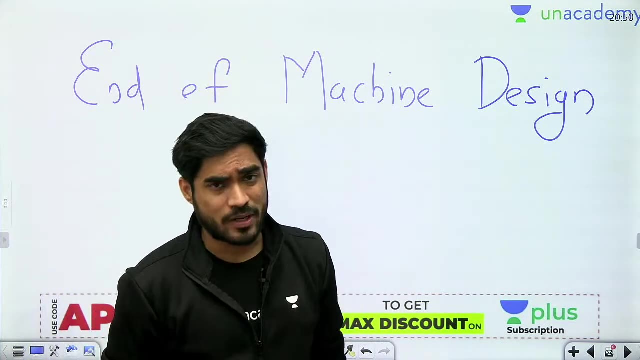 day why we are putting so much effort. you see all of the teachers in this channel: devyendra negi, sir pallab, sir alok, sir, manish sir, all of these faculties come together. vishwajit, sir sandeep sir, all of these faculties, all of these teachers, these educators, come together. 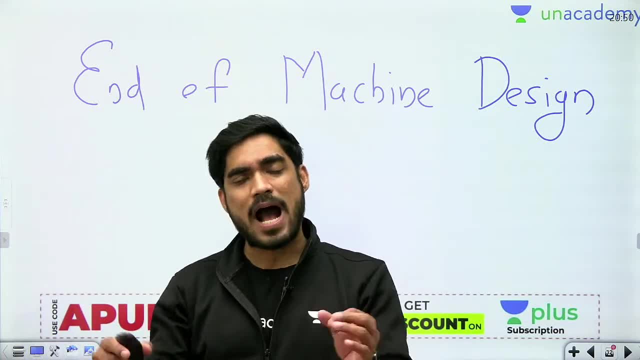 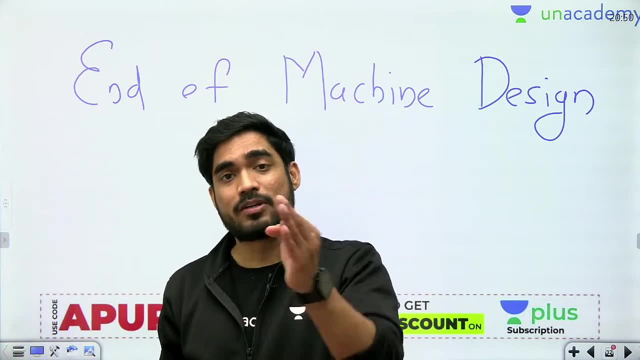 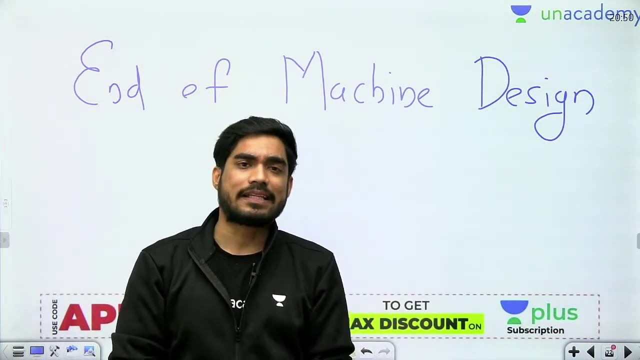 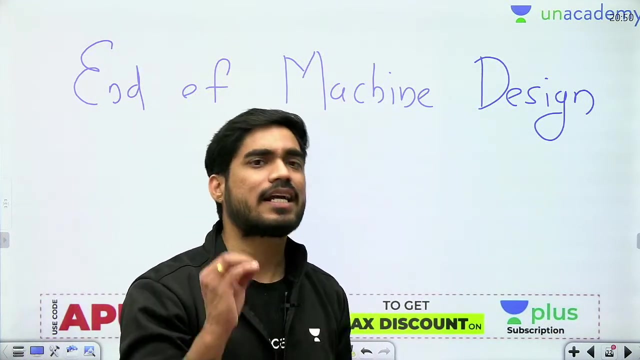 every day and they take hours and hours of lecture. why they are putting so much effort? So that in India, every engineer who is trying to crack GATE will get quality education online completely free. Why are we doing all this? So that every engineer in India see. my brother is doing engineering with a scholarship. even the poorest kid is doing engineering today. 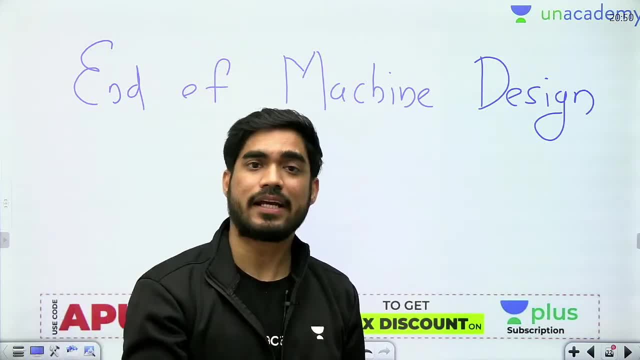 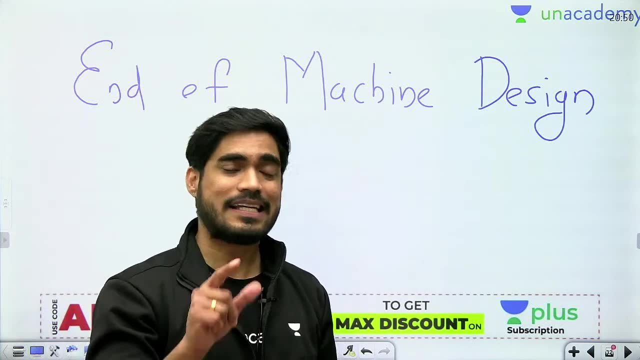 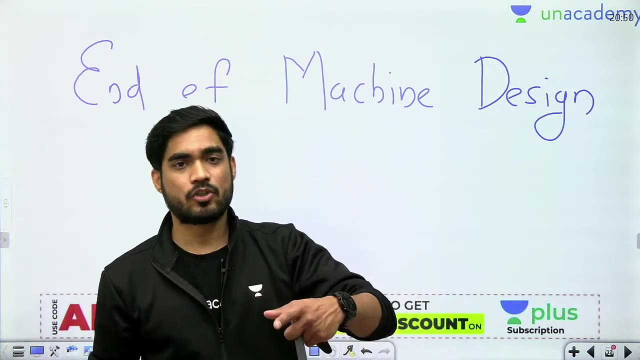 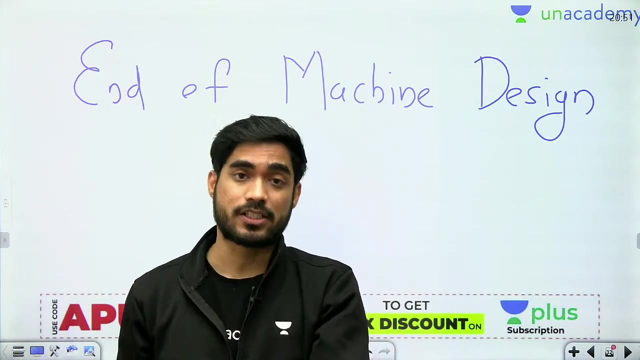 But when he goes to prepare for GATE, for higher education or for PSU, then he has to pay a lot of fees. He doesn't get a scholarship there. So these people who are not getting enough money in order to get into the institutes, in order to pay for them to study for GATE, these people should get high quality, free online education. 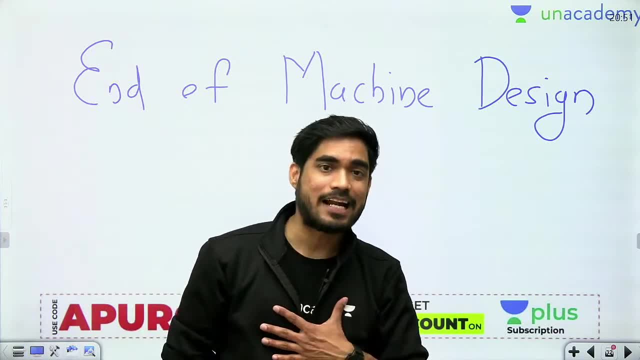 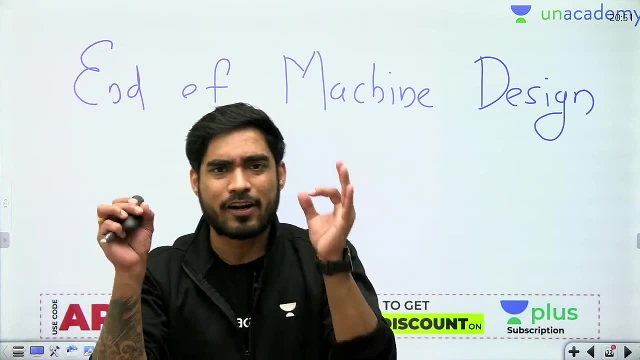 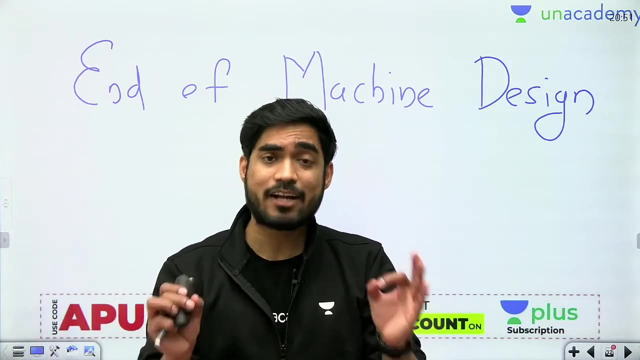 So the revolution that is brought by an academy is that now every student of India who is preparing for GATE can have the access to free, high quality online learning. high quality education, not only free education. free education is always there. free education was always there, okay. 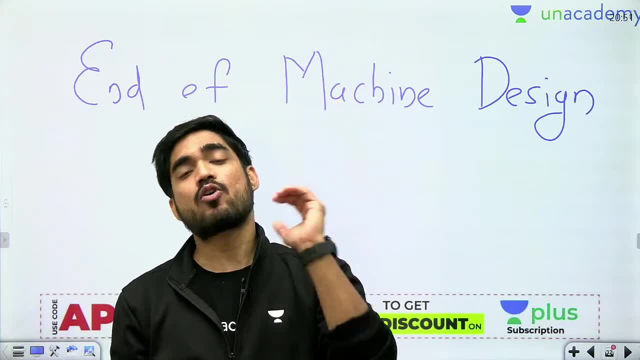 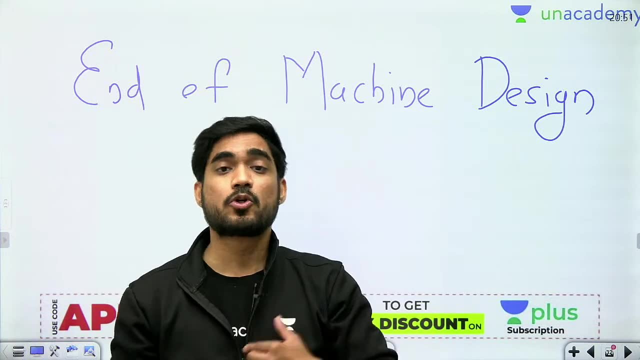 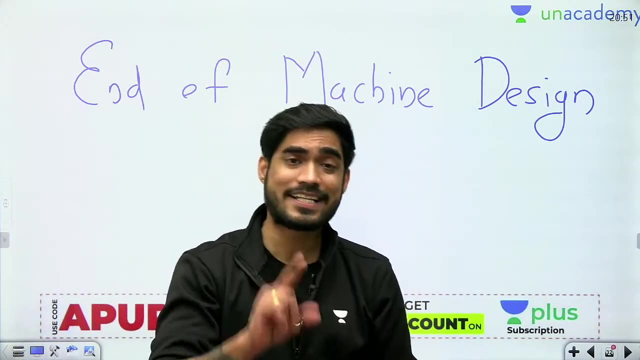 From years there is free education, but beta, high quality, free education accessible to all the students. that revolution is possible due to an academy. okay, So thanks to an academy, each and every educator on this platform is now able to reach. 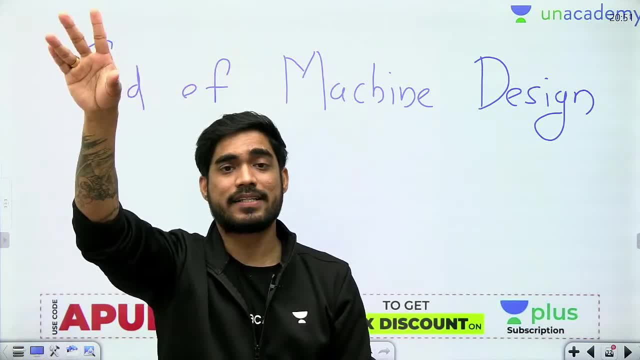 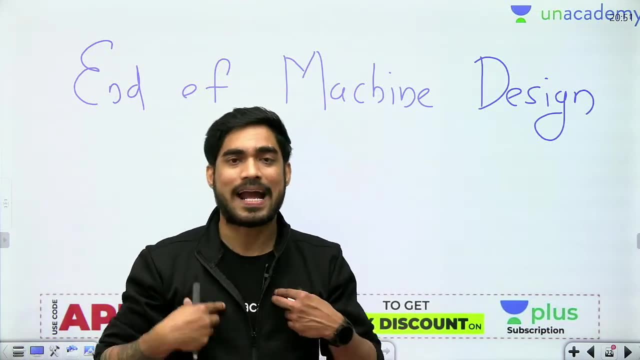 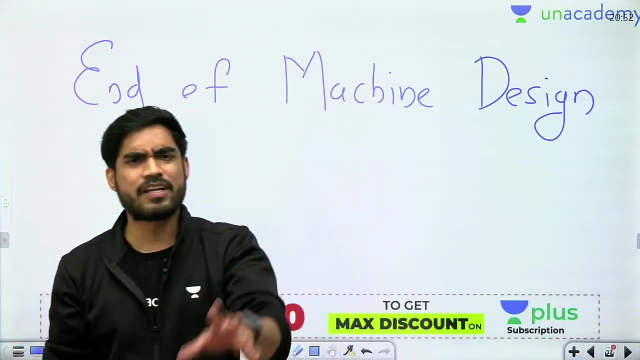 to all the students of India, and now all these students can access high quality, free education. okay, I am not just talking about my lessons. I am not just talking about my classes. I am talking about all the classes taken by every teacher, and not only in this channel, in every Youtube channel, not only by an academy educator, by all the educators. 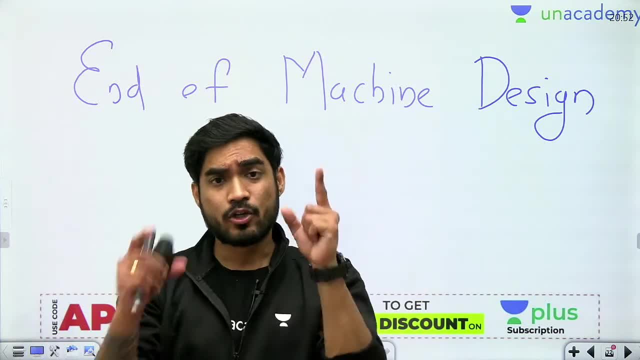 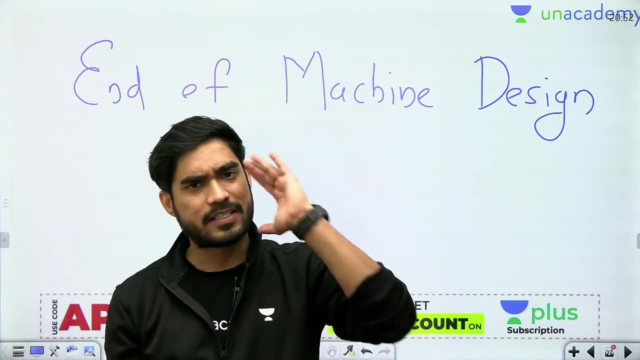 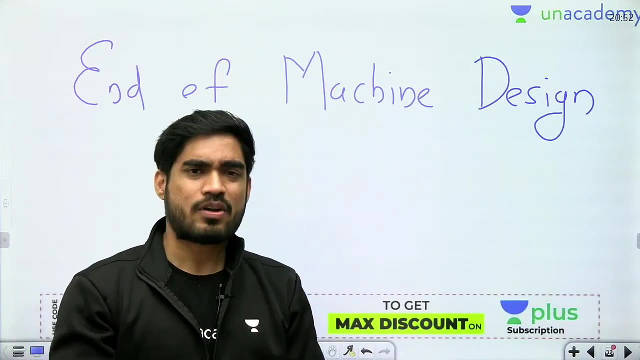 whoever is coming and putting their efforts on a daily basis beta. you need to appreciate them. been online and then going to youtube. Don't look at what he thinks about it. don't ever doubt the intentions of the educators. If someone is working so hard for you, then don't look at what he wants to do. 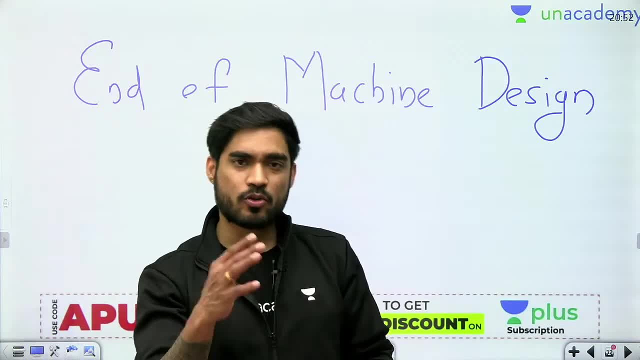 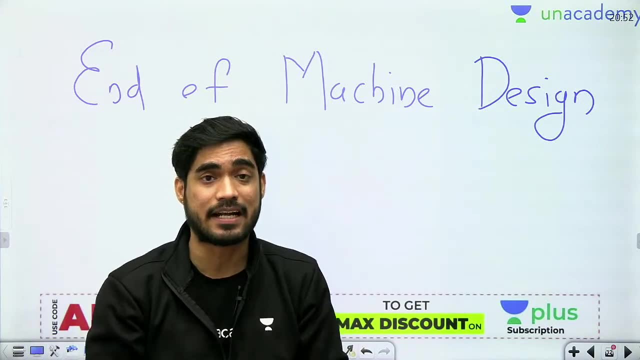 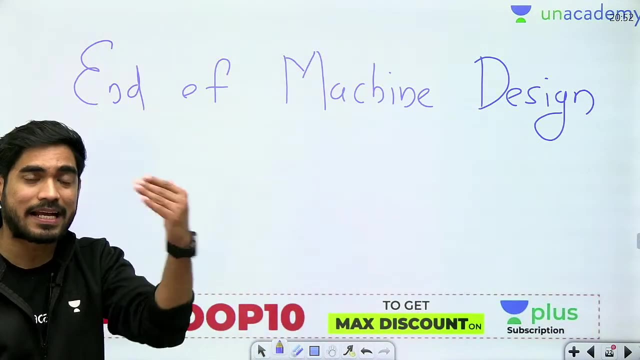 Look at what benefits you are getting from it. You are getting options between different educators. you are getting free online learning. you are getting free online content. everyone is getting free guidance, which was not there earlier, Before this. did anyone know what to study in machine design? No, 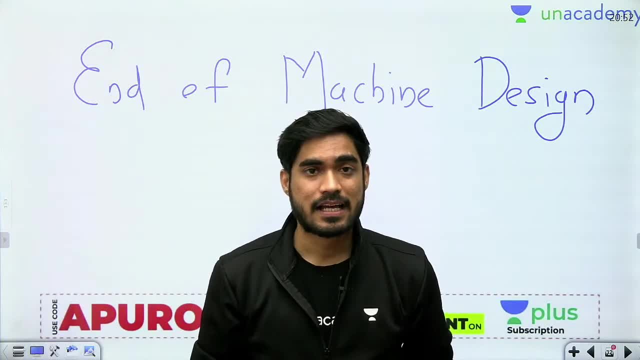 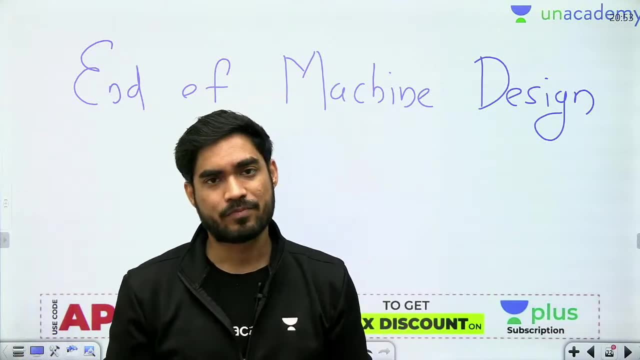 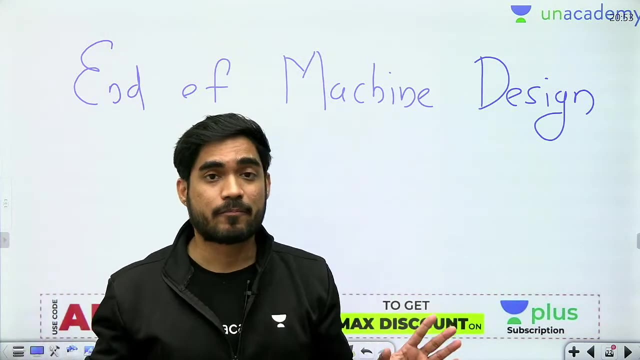 But now look at how many lectures there are in machine design. You all know exactly what to study, from where and how much to study. So all this has been possible through this platform. Now, the war does not end here. Just by making these lectures, our work is not done. 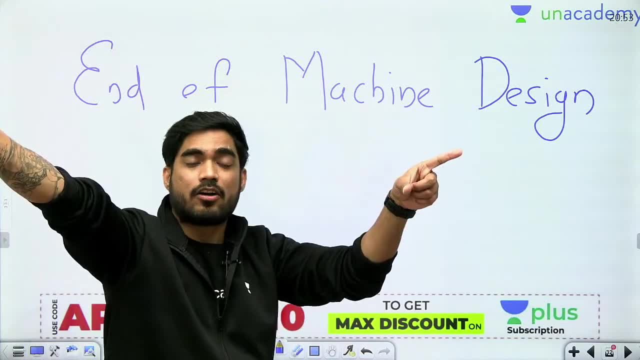 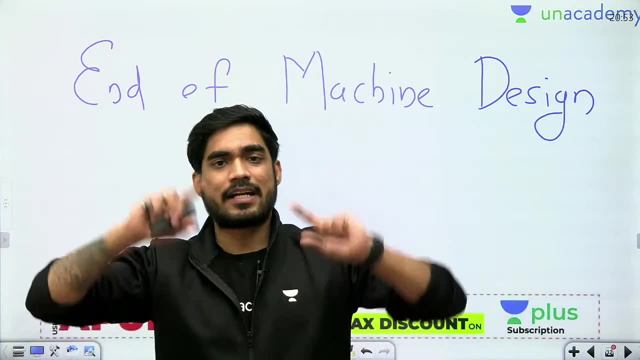 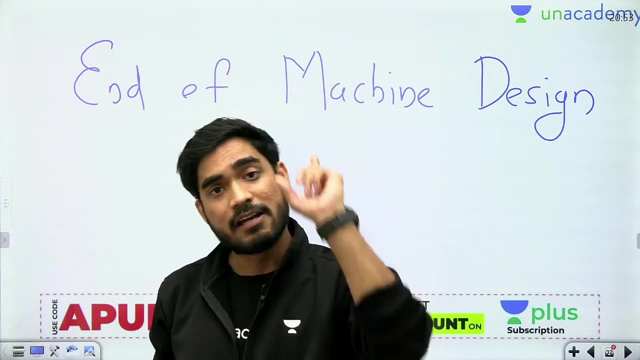 Making these lectures reach to each and every student of India. that is another step that we need to take, Thank you, We have taken one step that we have made content. Now this content should reach children. It should reach every house. Every engineer who is preparing for GATE, who does not have any means, should reach there. 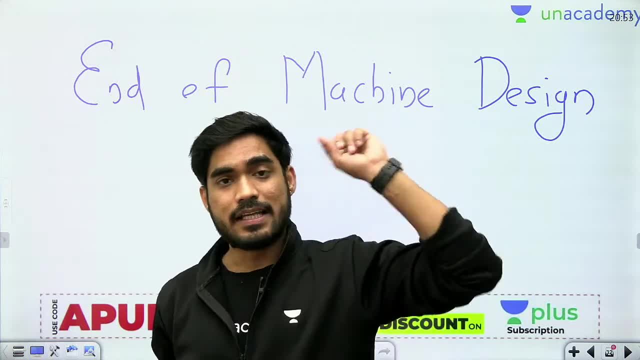 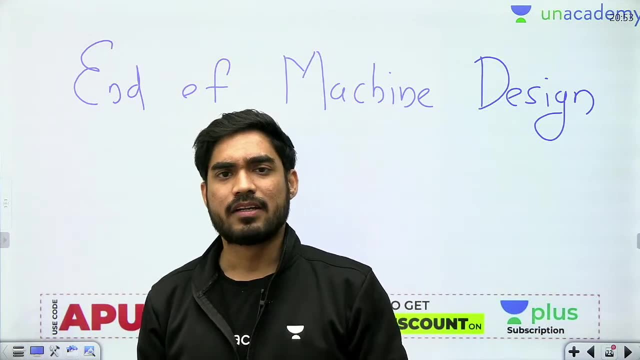 Students who have lack of resources. these lectures should reach to them, And how it will reach to them They will not be able to find out by searching on YouTube. You have also seen that it is not so easy to get lectures on YouTube by searching. 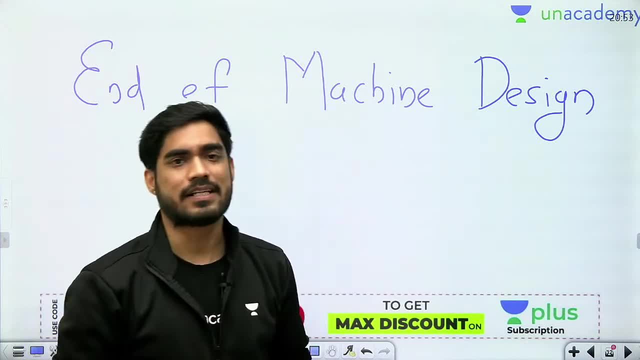 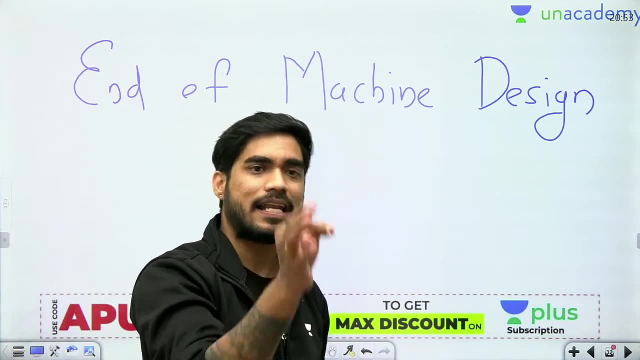 So we need to make them aware. Make them aware of these lectures. So please share these lectures, Not only mine, But whenever you come across a good lecture series, Whenever you see a good lecture series, you feel that this is a good lecture. 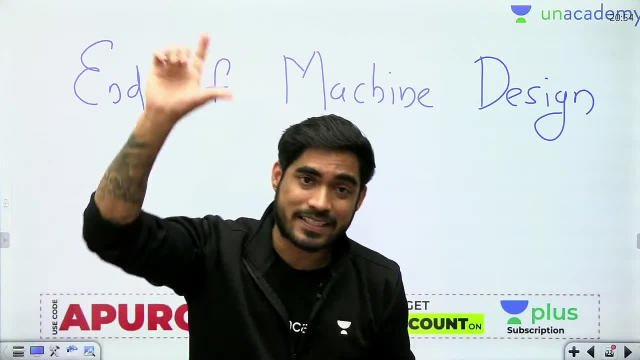 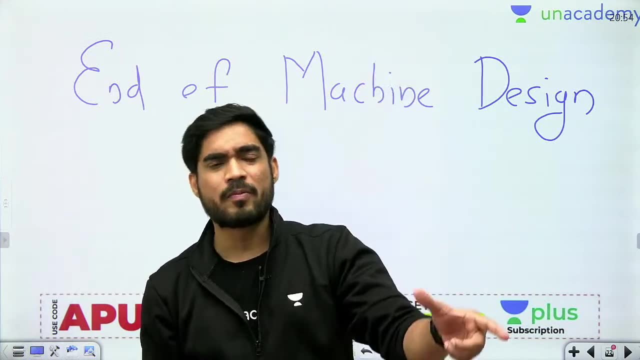 Everyone should see this. Then please share the link of that lecture to all your friends, all your groups. Don't think that it will be a waste of time. No, my brother, If you are sending it to a group of 100 people, and one of them started following it after seeing it. 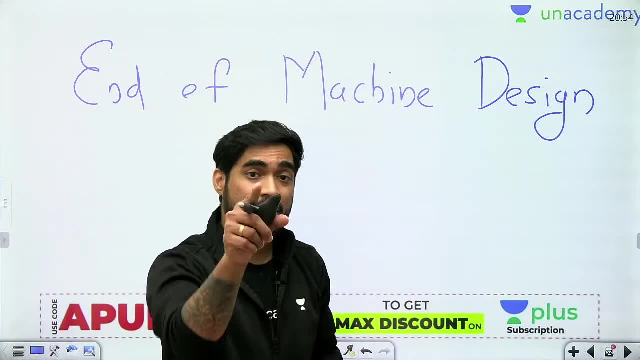 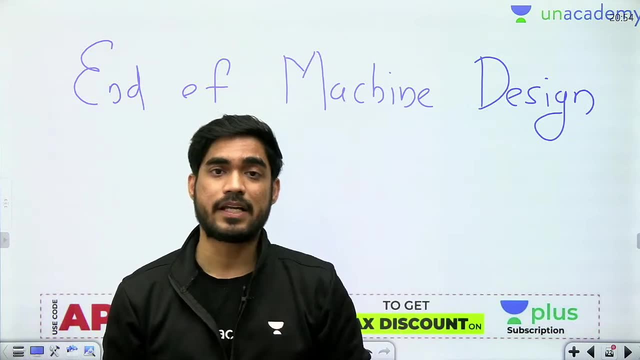 So this means that one child needs that lecture series And you have reached there. So, my brother, Even for that one child, If you have to share in 100 groups, Then never think I do it. I do it daily. I come here daily. 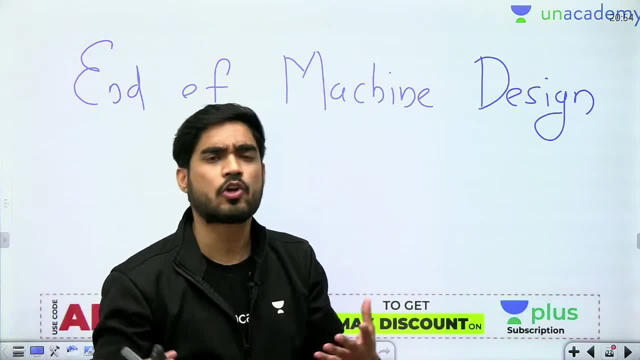 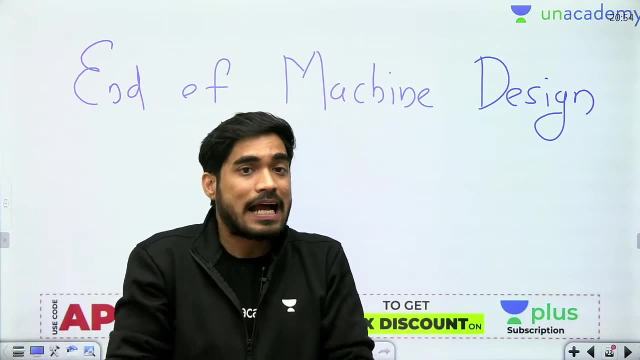 Press the like button. Press the share button. Share it. Share it. Why do I say I am not getting any pleasure by your like? If you like my videos, I will not get paid for it. I will not get greetings. 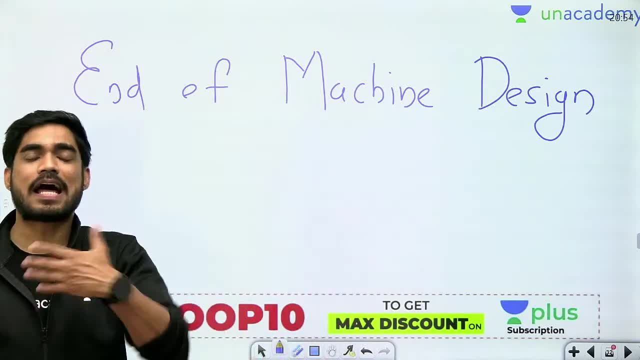 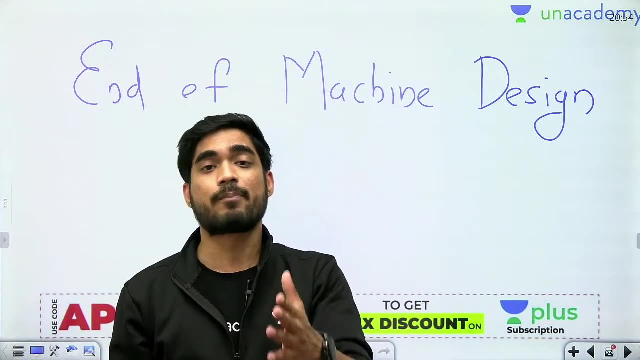 I will not get thanks for, I will not get praise. People will not congratulate me. People will not praise me because of the likes, Number of likes. Okay, I am not doing this for praises. Why I am asking you to like and share is so that these videos will be shown to everyone. 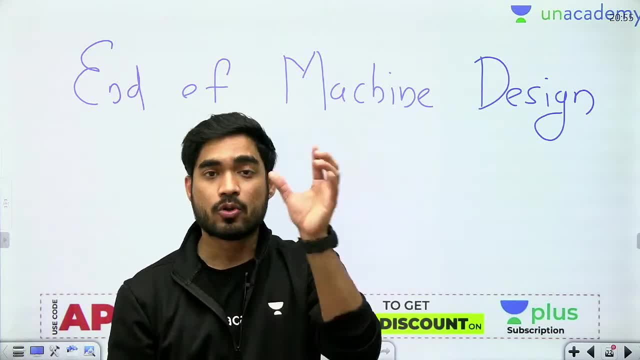 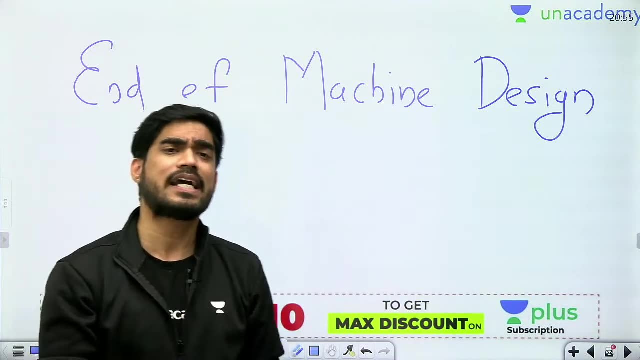 The more likes there will be, the more people it will show, The more people will believe in it. So, my brother, Whenever I come here to take a lecture, You see I speak 20 times in one lecture. I repeat every 10 minutes. 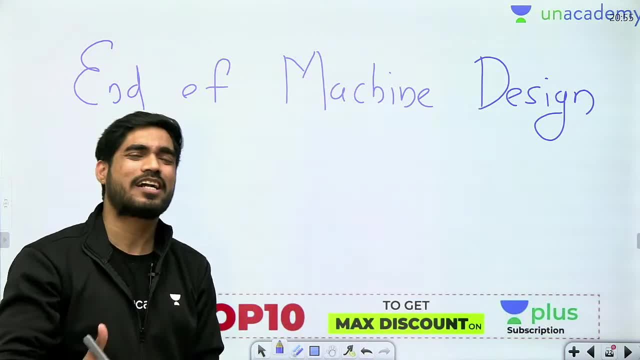 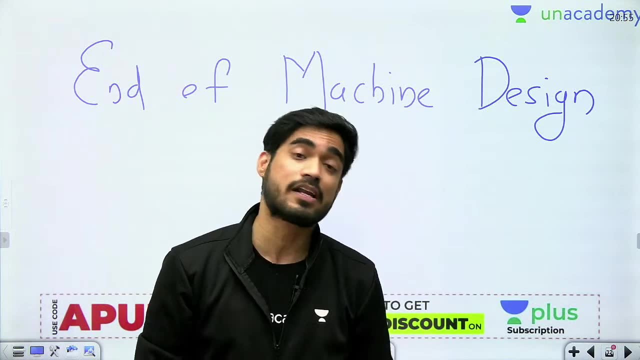 You must be thinking, Sir, why do you keep asking for likes and shares every 10 minutes? Sir, why do you keep begging for likes and shares like beggars? But, my brother, You have to do it. Why do you have to do it? 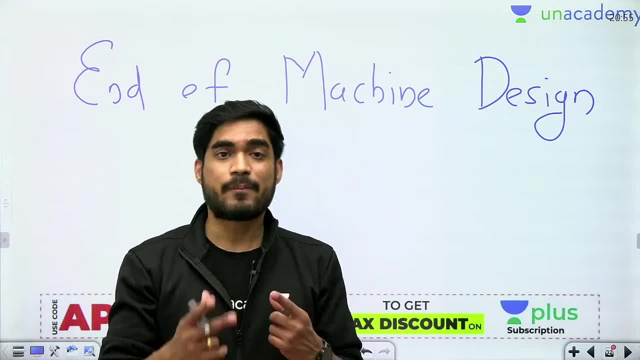 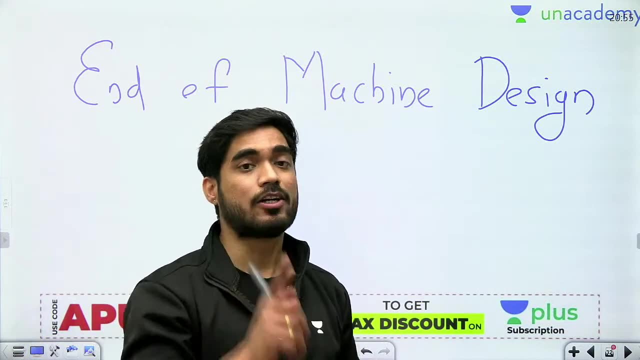 This is not for me. This is for every student, For that student who does not know about this lecture, It is for all those students who are not aware of this lecture series And I want these lectures to be available to them Now, watching them or not watching them. 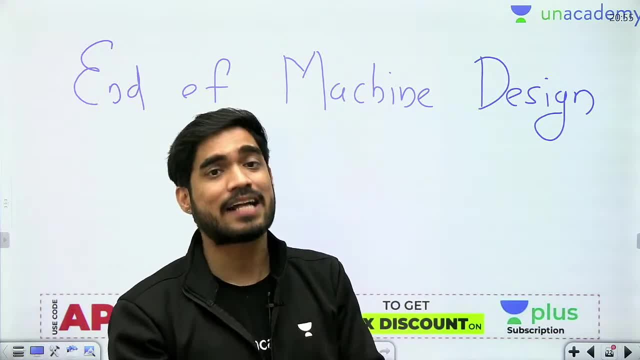 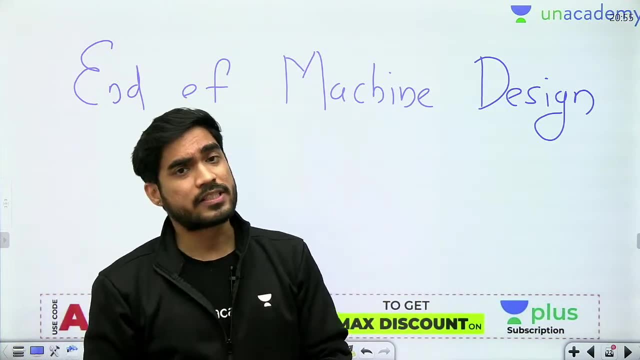 That is their decision, But at least they should get a chance to see these lectures. If they get a chance, If they do not like it, Then they will not watch it, But if they reach there. So for that, my brother, If I have to come every day and speak 20 times, 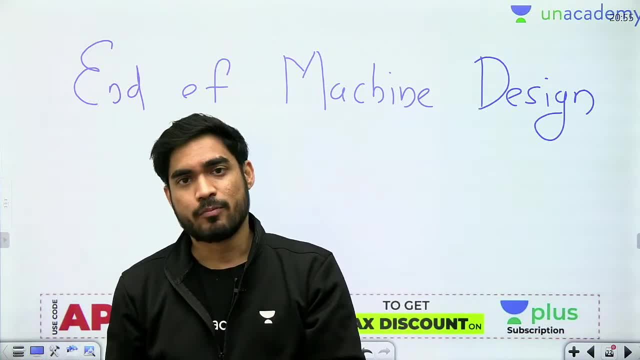 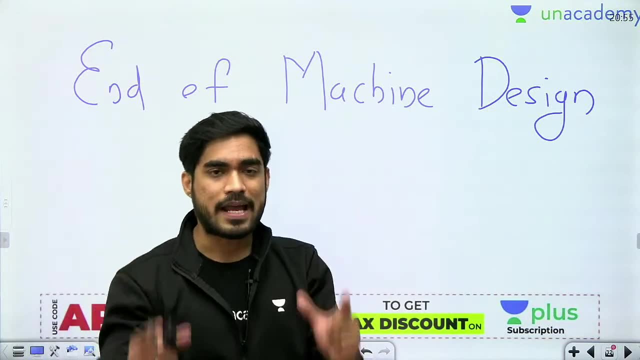 I will speak. I have no shame Because my brother, I know what my work is If I am coming here with so much effort and taking lectures. So I want That, son, These lectures should be seen at home And after that. 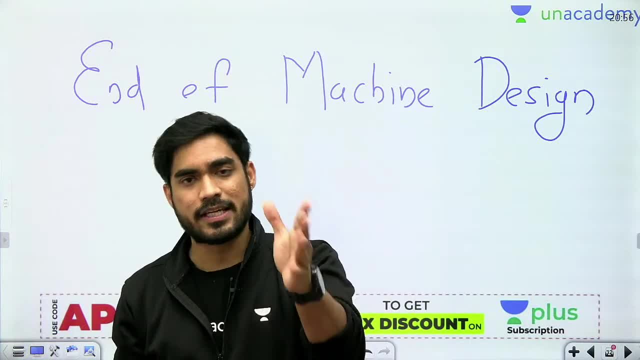 The child has to see. The child has to understand That he is liking this lecture, So it is fine. If not, Then see some other lecture. There are many options. So, son, At least watch these lectures And after that, 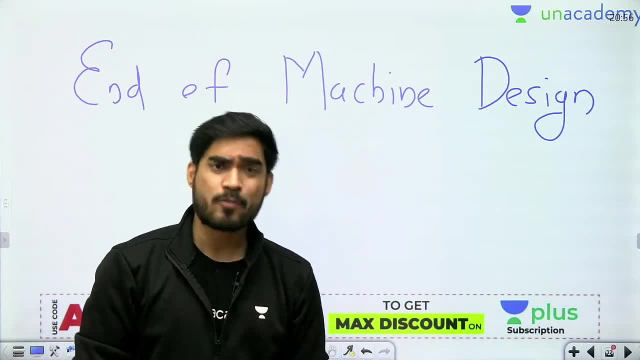 So, son, At least get that opportunity. You also know, my brother, Because of lack of guidance, How much loss there is If you are studying from a private engineering college. Then you would know that If someone would guide me from 9 to 10 in school, 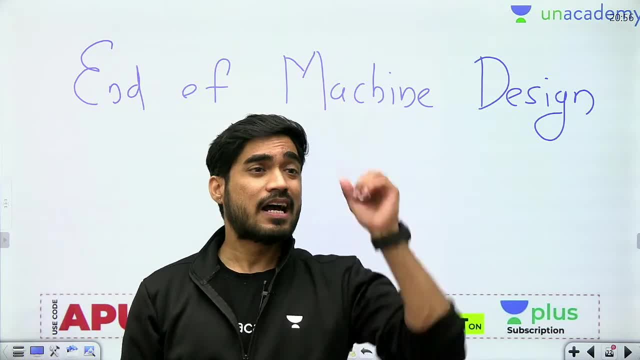 Then maybe in today's date, I would be studying in a good engineering college, Right? So, my brother, This lack of guidance Which is It creates a lot of problems. Because of this, A lot of people suffer, So this thing should not happen. 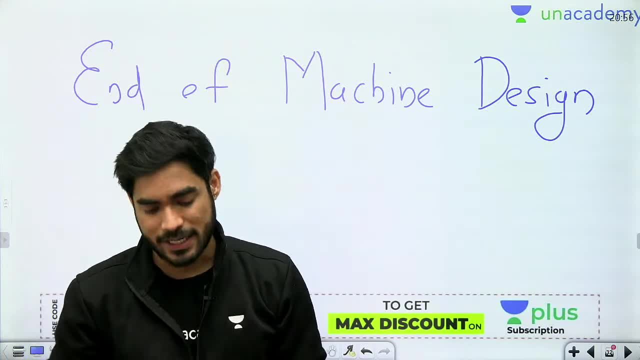 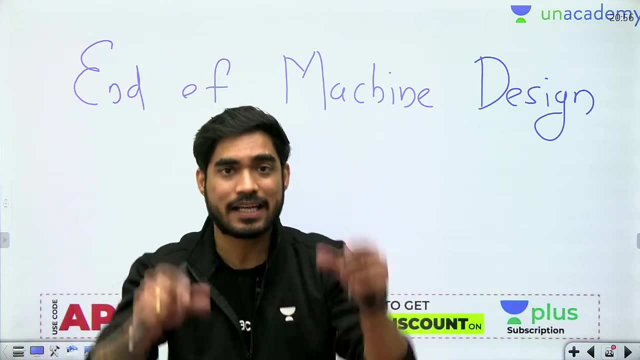 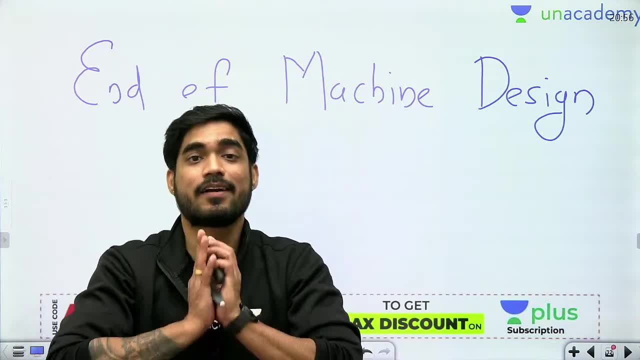 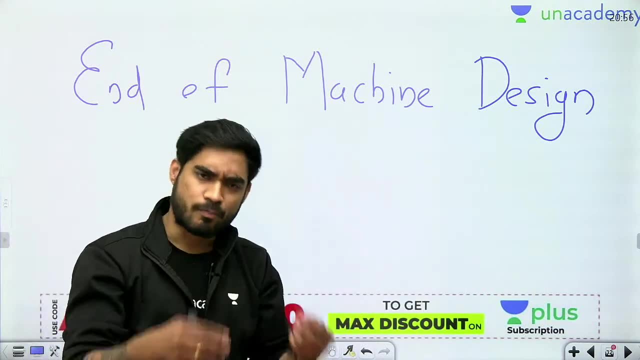 I say it with my hands joined. Please hit the like button. Please share the link. Please share the link And, son, I will keep doing, Will do, Will do, Will always do, No matter how much. Now I Reached a very few people. 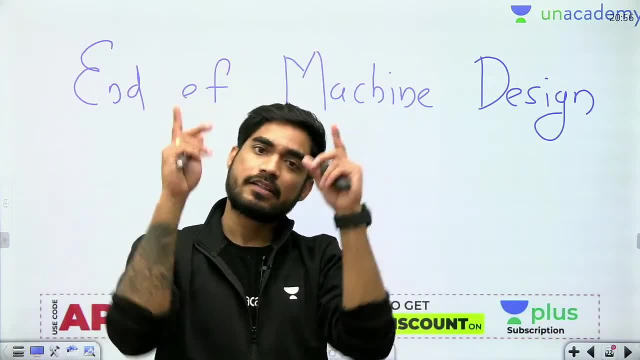 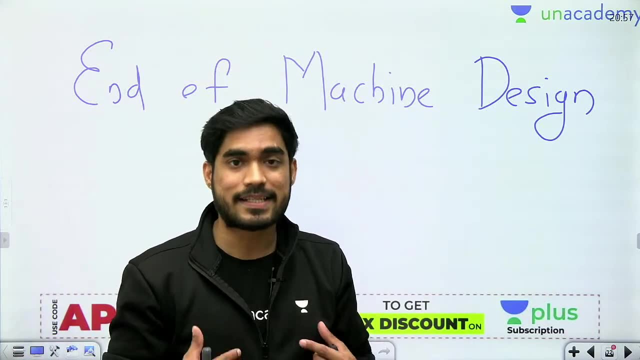 But if I Go, even to India, Then still I will come and do this work. I will always ask people to like And share my videos Because- Not Because of the praises I will get, It's not like. 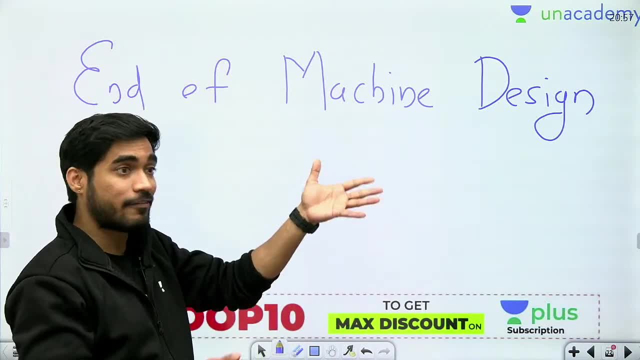 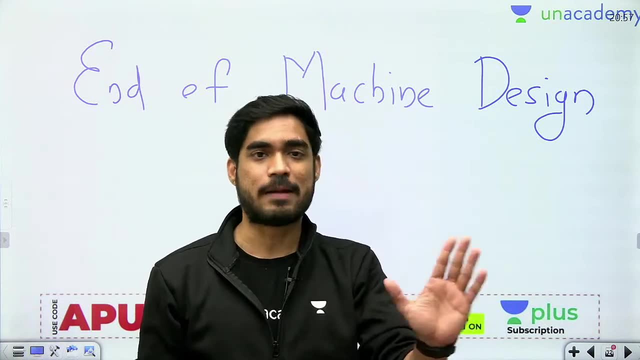 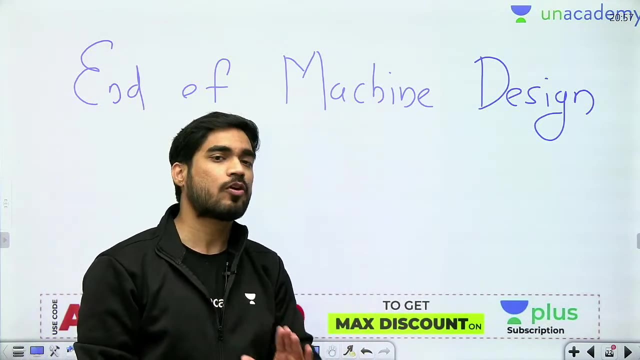 See, See, How many views are there in my video. See, How many likes are there in my video. No, I don't even share my videos with my family members, okay, I don't show them how many likes I am getting, how many views I am getting. no, that is not what I am looking after. that is not what. 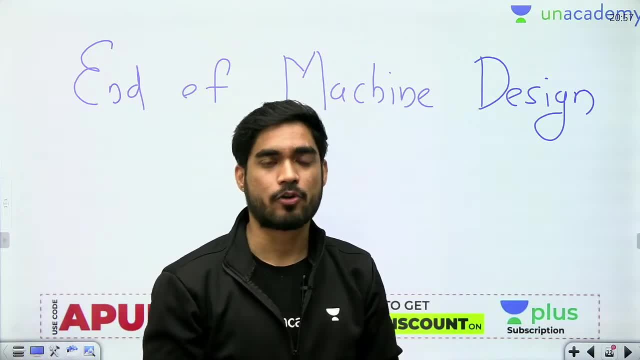 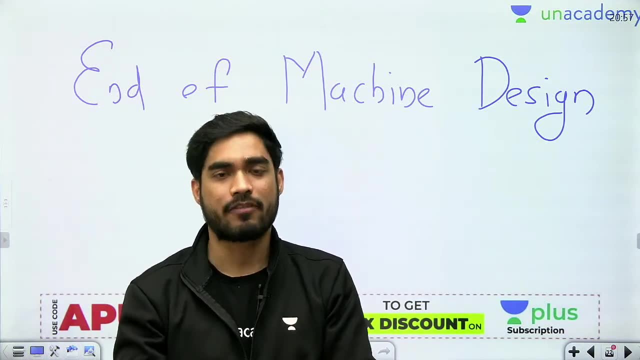 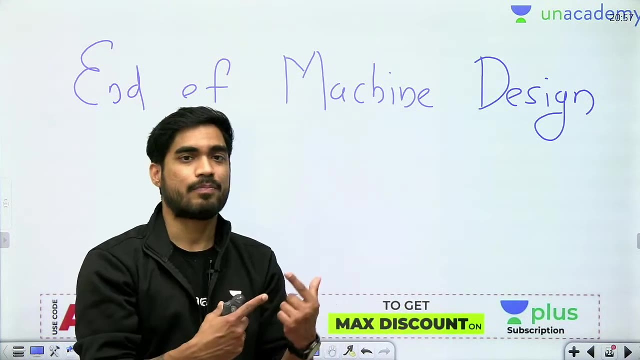 I am chasing. what I am chasing is what I am looking forward to is that these lectures should reach to each and every student. each and every student who is having lack of resources in order to prepare gate, okay, and if they want to prepare gate on their own, then these lectures will really help. 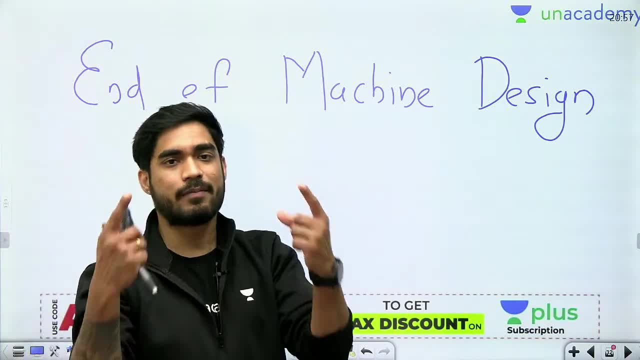 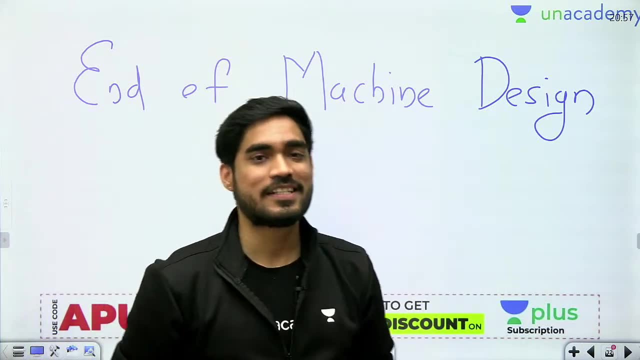 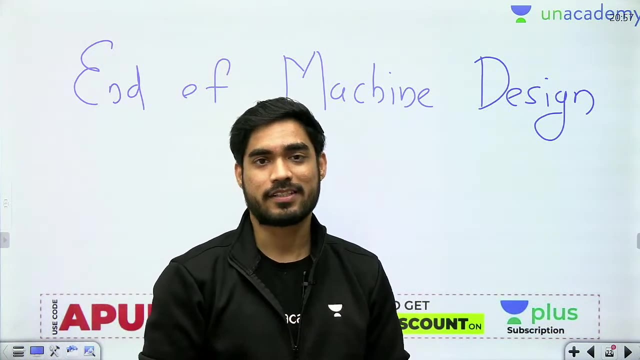 them, okay, so let's make these lectures available to everyone. thank you so much for listening to me. thank you so much for all the love and support you have shown. thank you so much for your likes. thank you so much for your shares. okay, now we have eight hours. 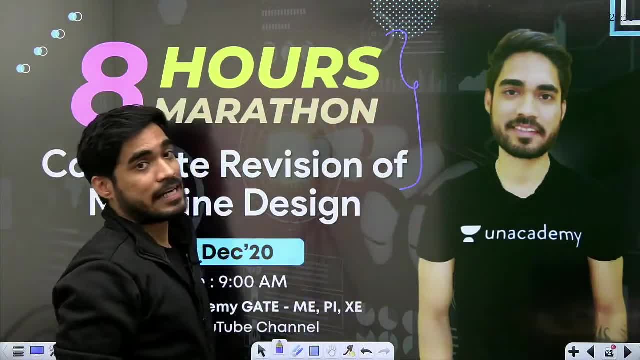 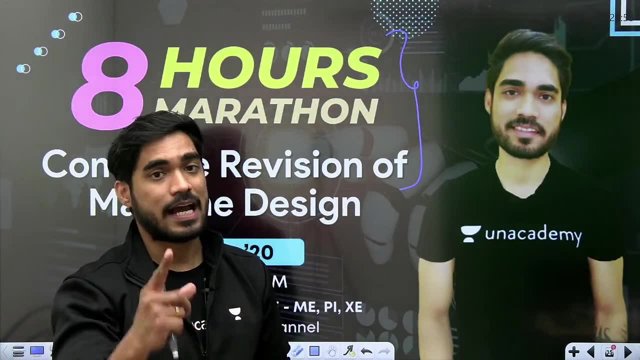 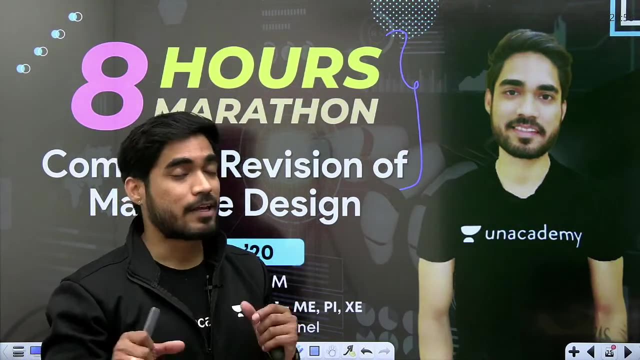 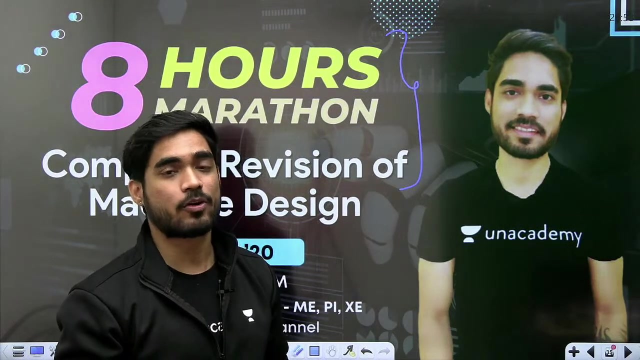 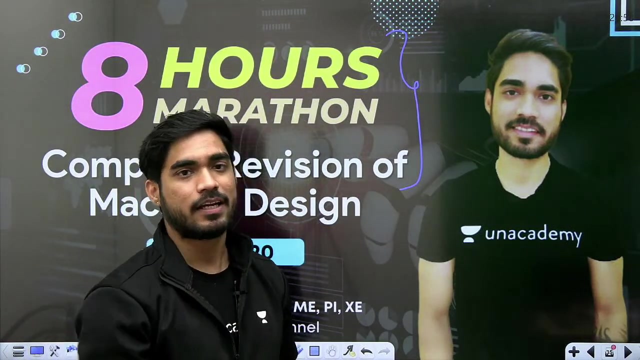 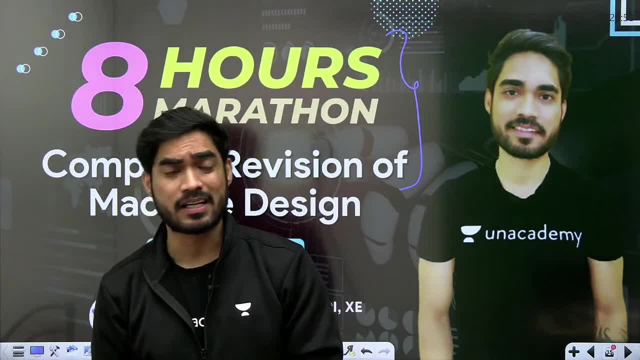 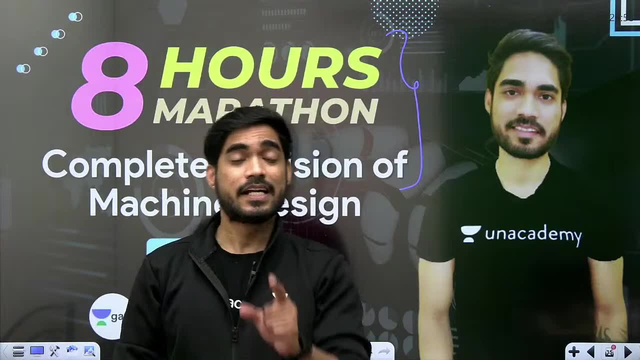 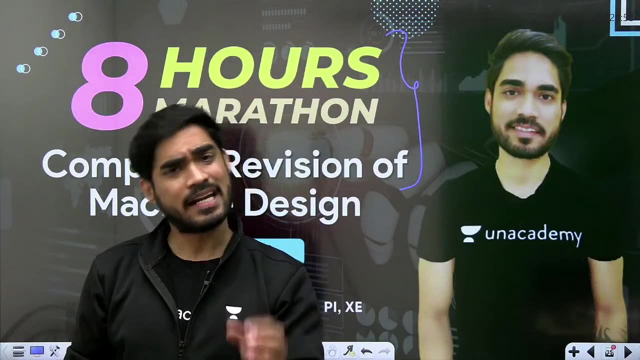 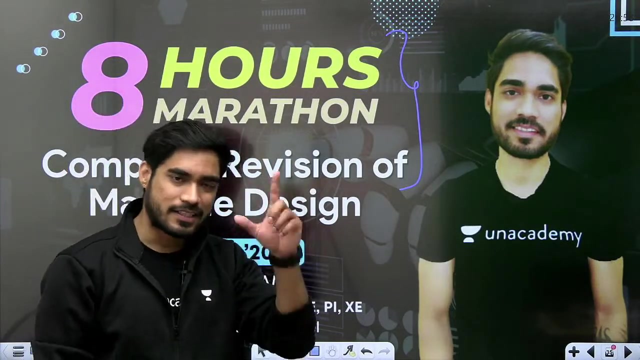 You have seen my last lecture, 5 hour marathon lecture, in which I took only 5 minute break. So, my brother, how did I complete 5 hour lecture with 5 minute break? It is all because of you people. I only took 5 minutes of break in 5 hours lecture last time and every marathon lecture. you see my all marathon lectures. you see I will have taken only 5-10 minutes break and this is only possible because of you. 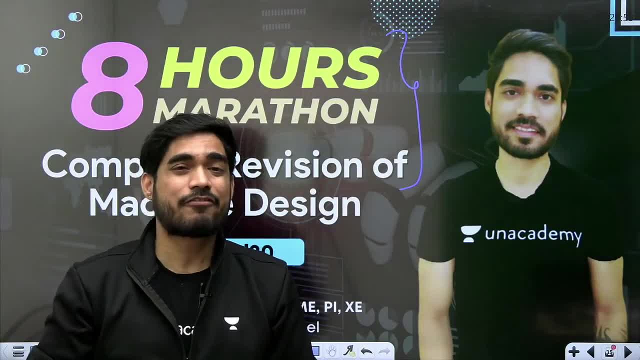 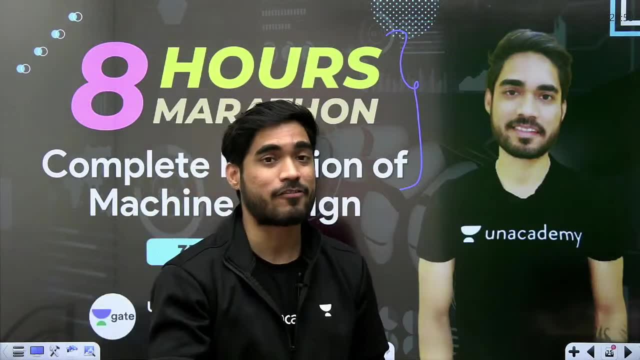 Because whenever I feel like giving up, whenever I feel like giving up, I will take 5-10 minutes break. Whenever I feel like taking breaks, whenever I feel like sitting down, then I look at the number of people watching these videos, I look at the number of likes and it really inspires me, really motivates me, it really fills me with energy. 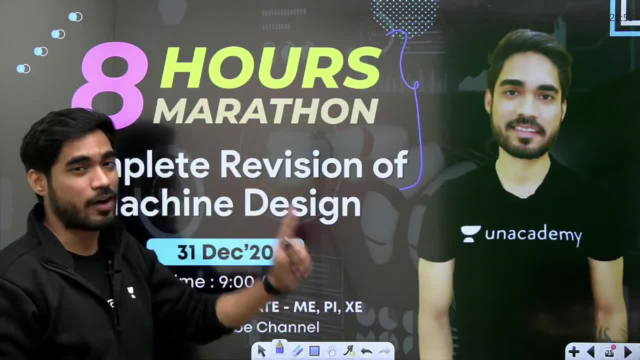 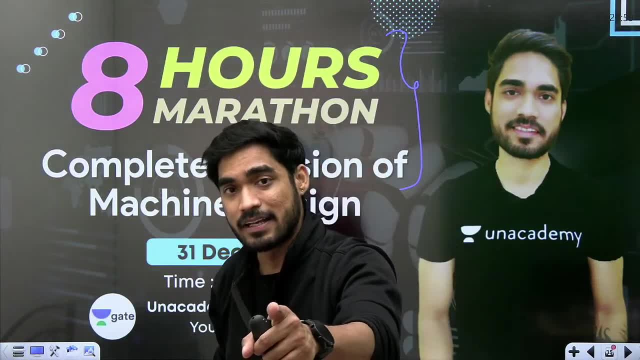 So my brother, tomorrow also I have 8 hours of class only for you people, only for my students, and I really need you, I really need your support. So please share the link of this. I will share the link in telegram channel. So please copy and share that link to all your groups and call all your friends online. 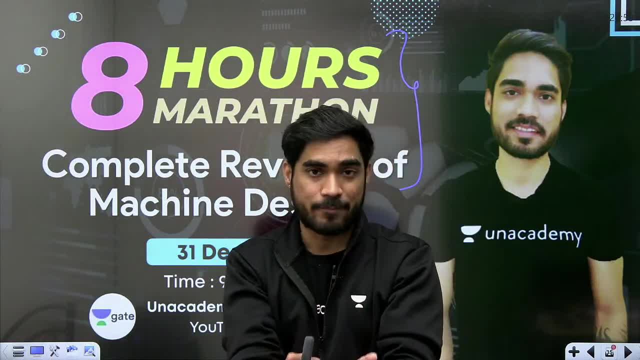 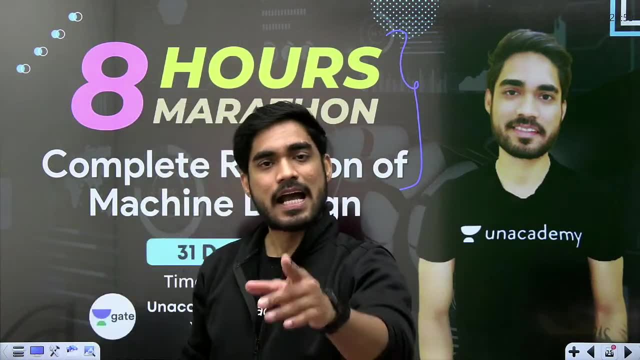 And please be live tomorrow. okay, Give me half of your day, 8 hours of sleep. you leave that, So you have only 16 active hours Out of those 16 active hours. I am only asking you for giving me 8 active hours. 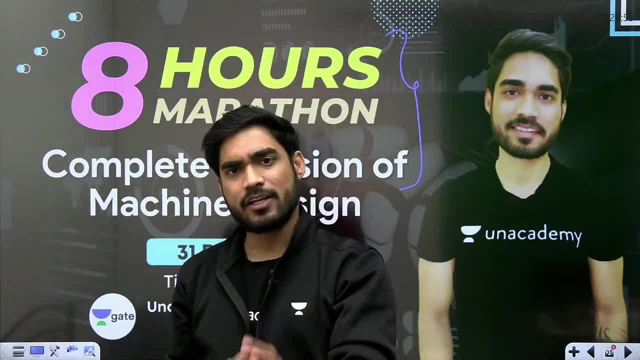 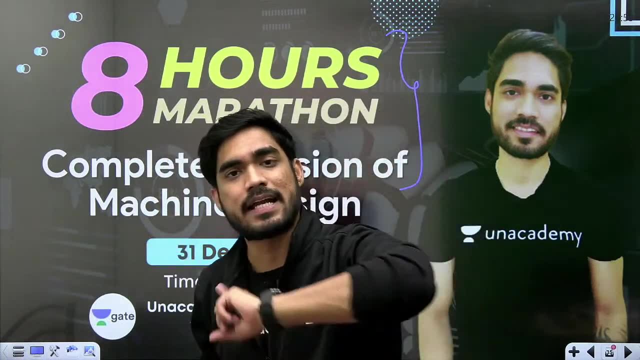 Give me 8 hours and I can guarantee you that you will not regret it. I can guarantee you that, after watching these 8 hour lecture series, you will not open machine design until the last day of gate. This is my guarantee, my brother. 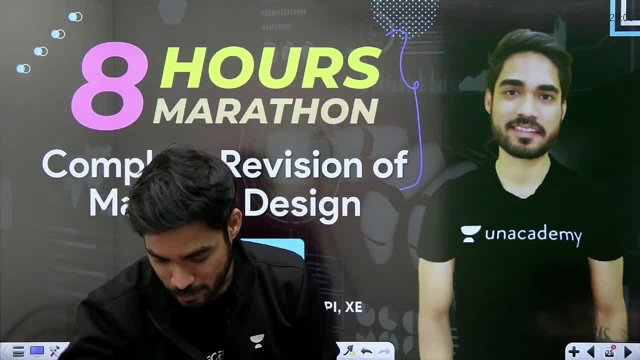 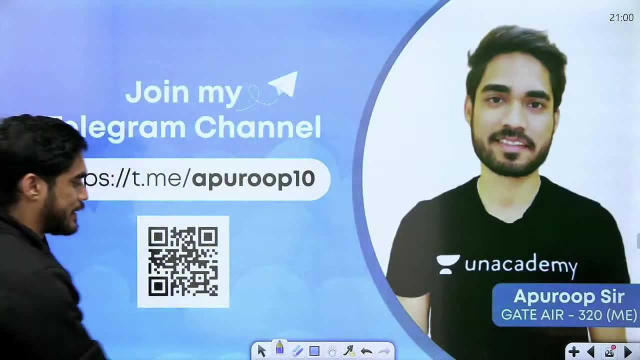 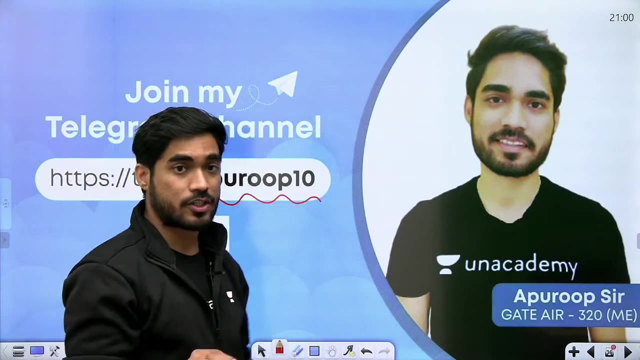 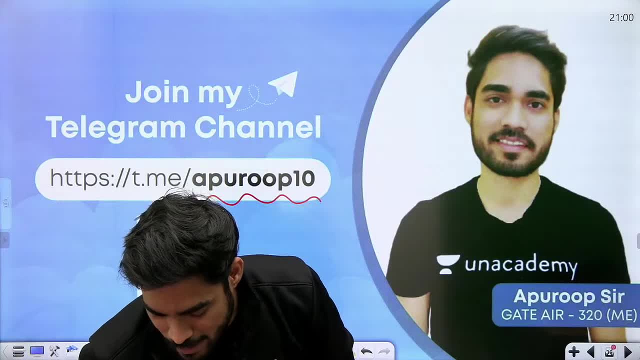 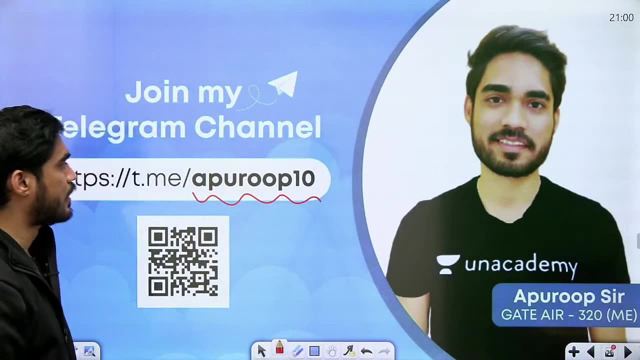 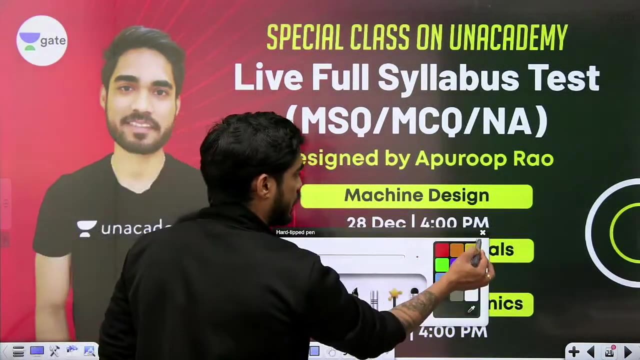 So don't forget to follow this telegram channel. Hey, my brother, I will do all the mistakes. I will do all the mistakes. I will fix them, Don't worry. Okay, And beta, don't forget that I have taken live tests of these subjects, Okay. 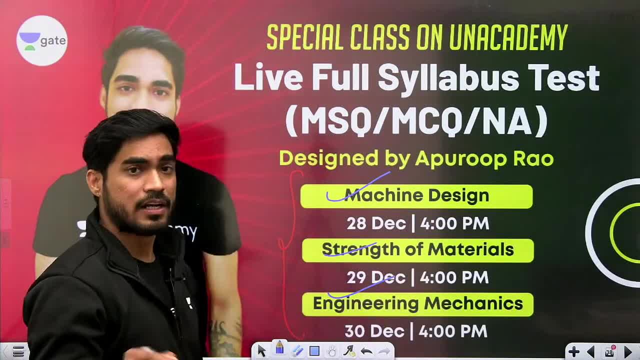 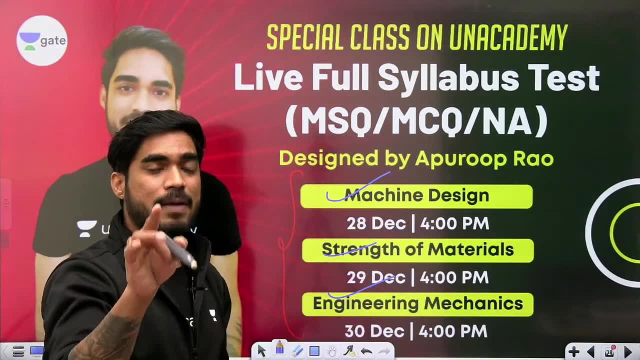 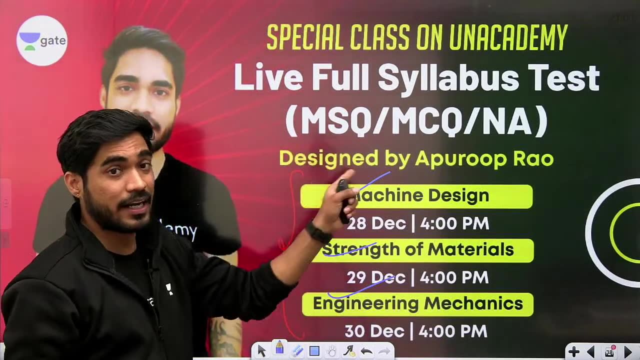 Live test of machine design, strength of material engineering- mechanics is over, But you can watch them by going to my special classes. Okay, You can watch these links. You can watch these classes by going to my unacademy profile. So go to my unacademy profile and give this test. If you have missed this test, there are some really interesting questions, Okay. 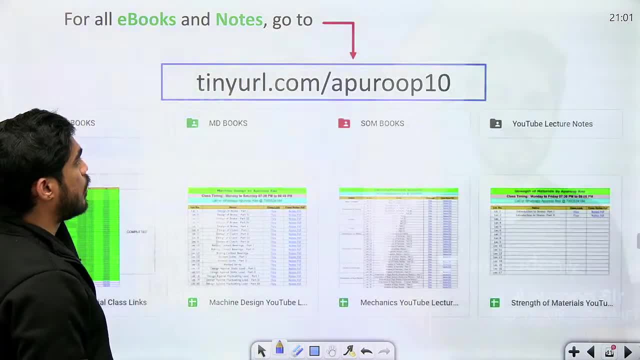 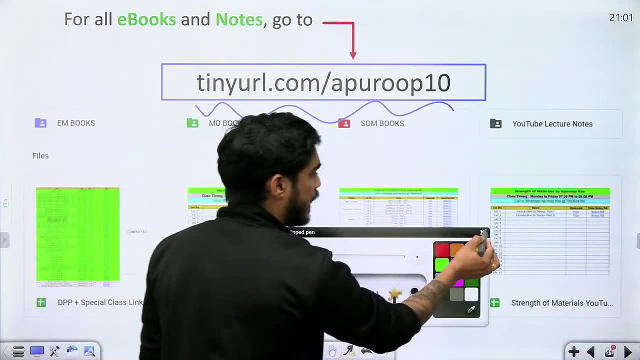 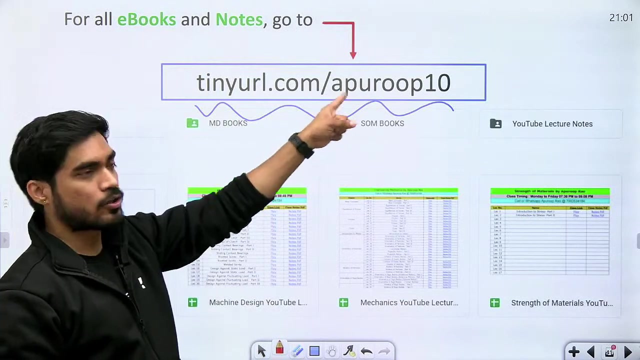 And don't forget about this. Tinyurlcom slash, approved 10.. Don't forget about this, my brother. Whatever lecture series is available here, whatever lectures I have taken, all of that is available here. Tinyurlcom slash, approved 10.. 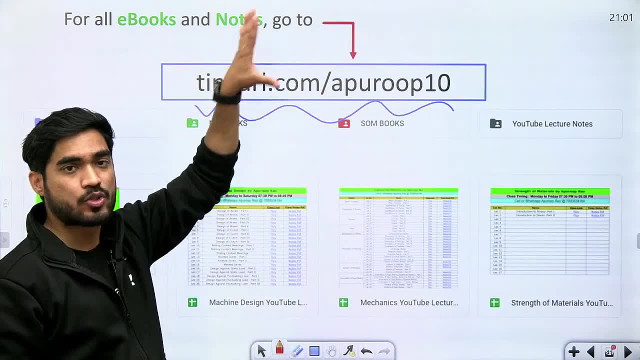 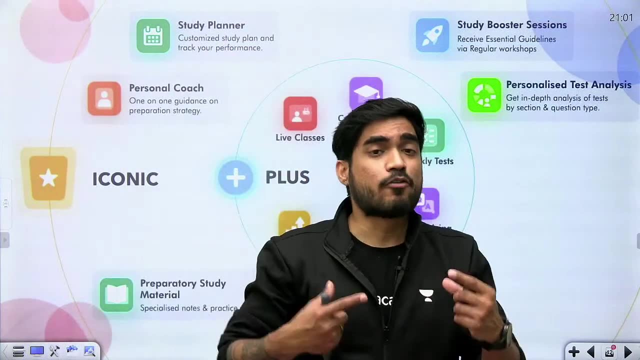 Just open this link, copy this link, paste it in your browser and beta open. tinyurlcom slash approved 10.. Okay, And if you want to prepare with me, if you want to prepare with the best of the faculties on unacademy, then beta, come to unacademy. 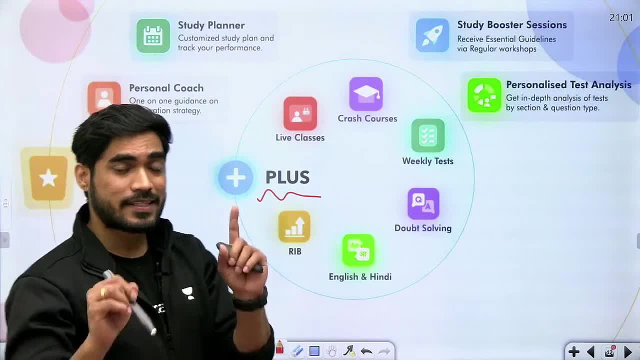 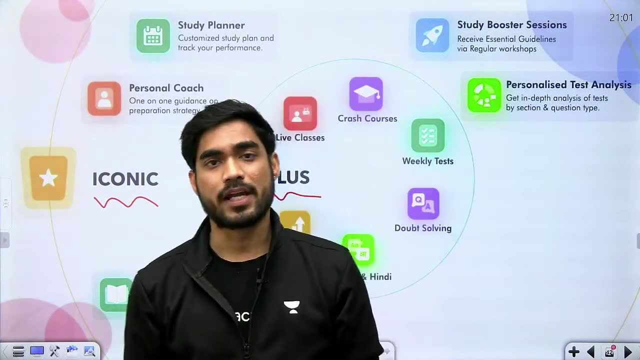 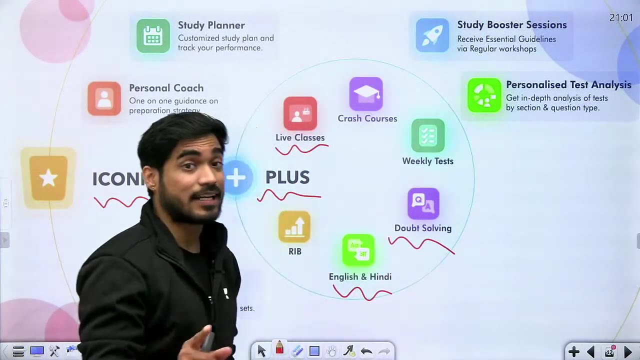 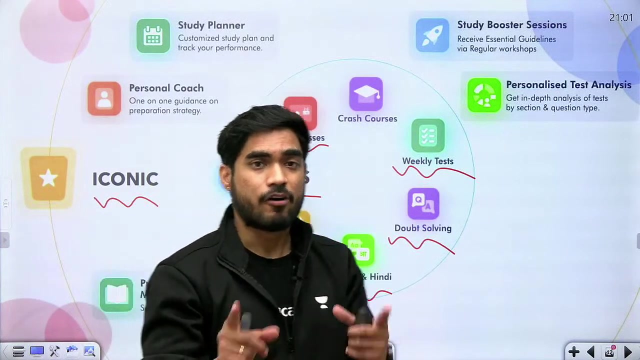 Plus and unacademy iconic. Unacademy plus is India's number one learning platform. Unacademy plus pe apko, wo sab kuch milega jo online learning ke liye zaruri hai. Jaise ki live classes in English as well as in Hindi. You will get doubt solving sessions, dedicated doubt solving sessions from the best of the educators. You will get weekly tests. So everything you need to prepare for GATE, everything you need to prepare for ESC, everything you need to prepare for PSU- All of that will be available here. 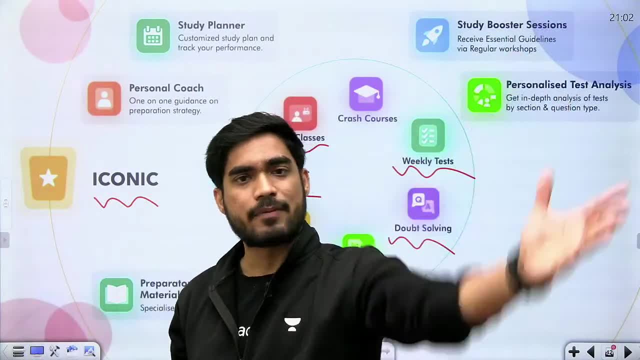 Ab aap ye soch rahe hoge, ki sir, sab kuch toh yahi mil raha hai, unacademy ki kya zorrath hai. So, beta, I am sure I know that if you want to prepare on your own, everything is available here. 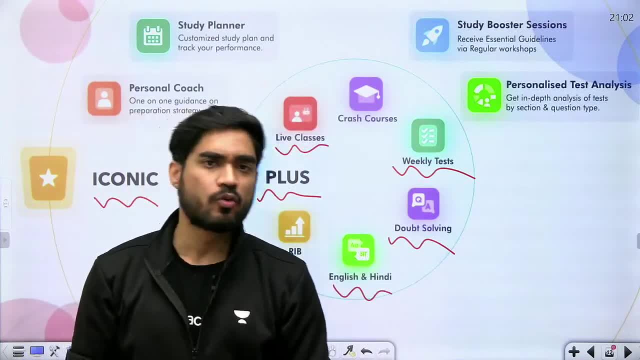 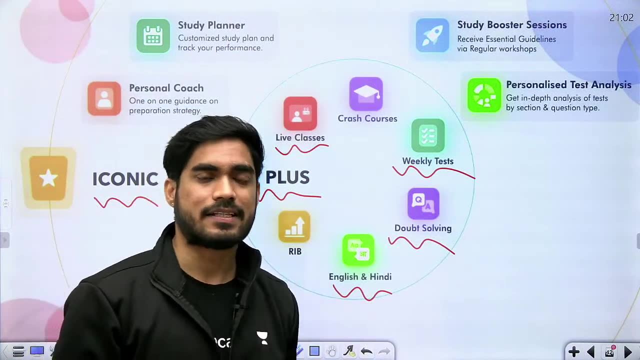 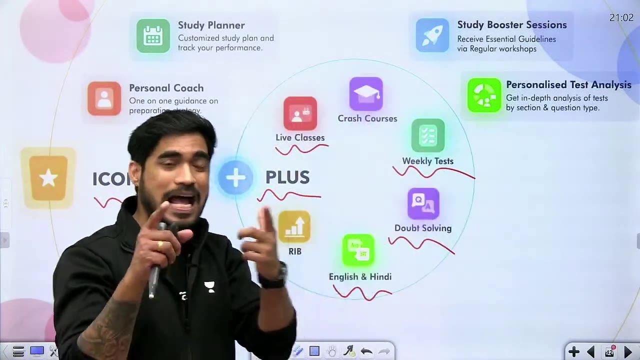 But, beta, trust me that at some point you will get doubts, at some points you will need practice problems, at some points you will need personal guidance. So all of that will be available on unacademy. So, beta, agar aap ek step aage jaake unacademy plus pe aajate ho toh aap chances of getting a good rank. 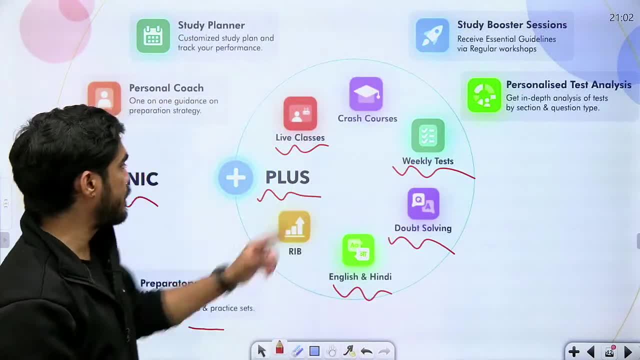 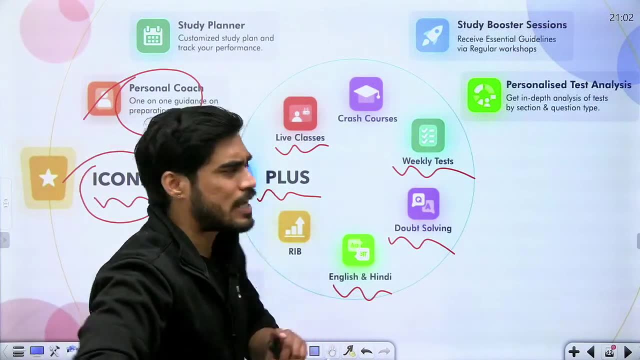 Bahut zyada exponentially increase kar dete ho. Aur isse bhi ek kadam aage hai. unacademy iconic subscription, where you will get a personal coach. Personal coach, kya karne wala hai, mere bhai? Personal coach, aapka poora schedule banane wala hai. 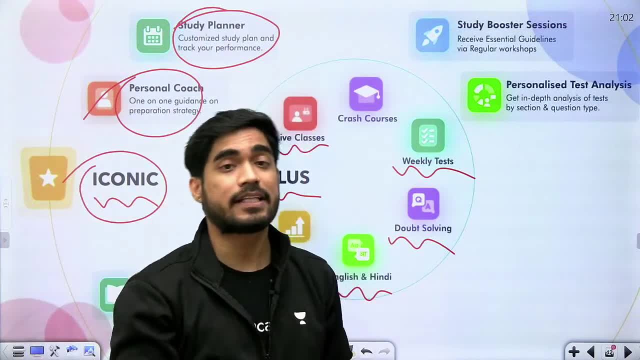 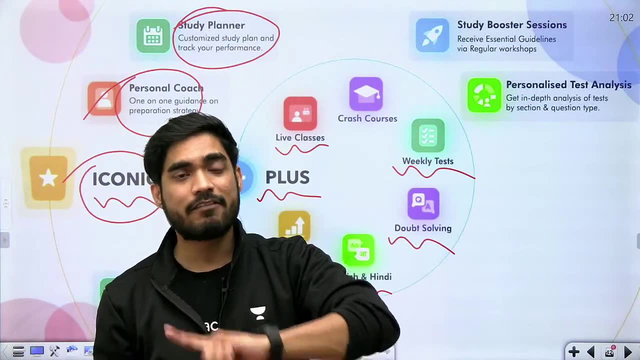 He will prepare the entire schedule. He will make sure that you are following that schedule Every day. you will get push notification, you will get calls, you will get one on one direct interviews where they will be asking you about your progress, Whether you are following your schedule or not, and all that. 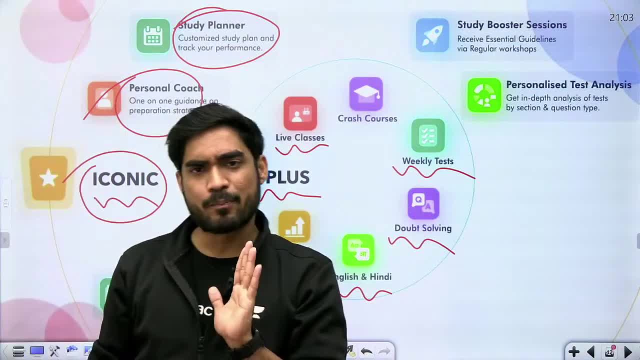 Okay, So personal coach will give you that Personal push, Wo ek push aapko milega daily basis pe jo chahiye aapko padhne ke liye, aapko acha prepare karne ke liye. Okay, 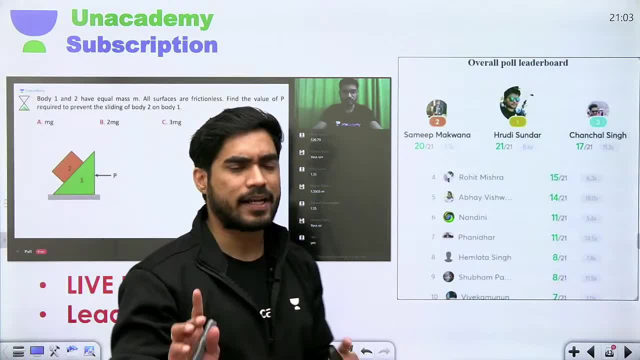 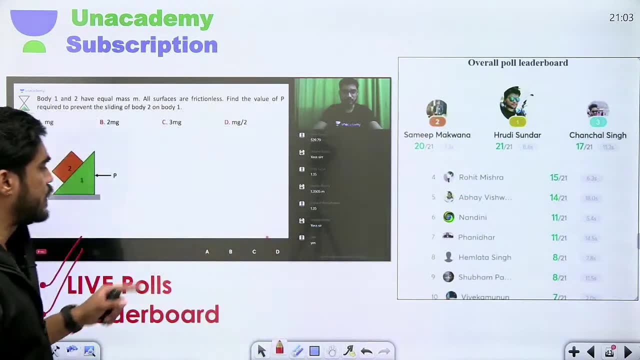 And beta. there are lots and lots of features on unacademy which will really help you in online learning. Okay, Jaisa, live polling or leaderboard. jahan aap har objective questions me quiz competition ki tarah part le sakte ho? 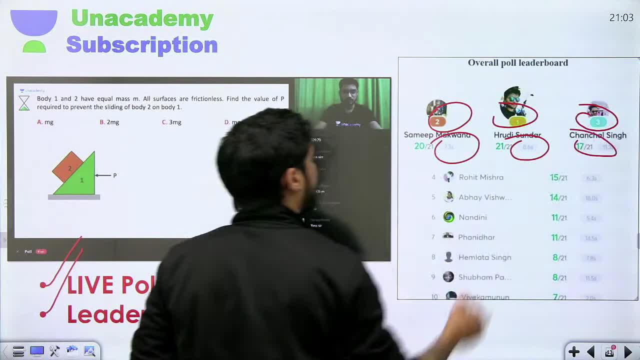 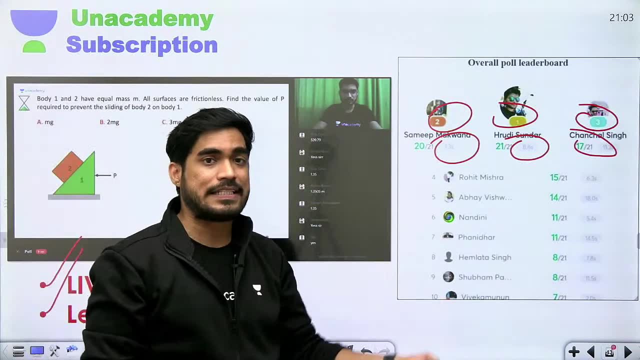 Leaderboard aapko batayega aapki rank kya hai, aapki timing kya hai. So ekdam quiz competition lagega ye. So it will be a fun learning for you. and time management, How you can manage your questions- all of that you can learn from here. 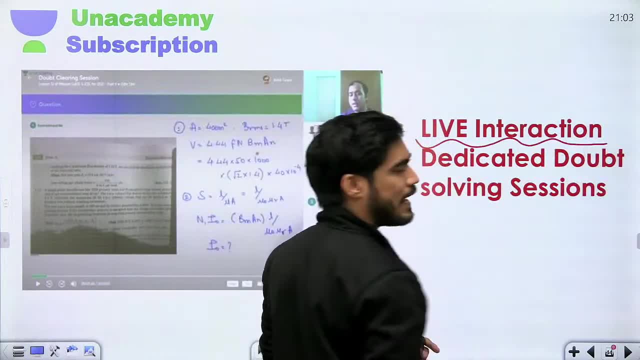 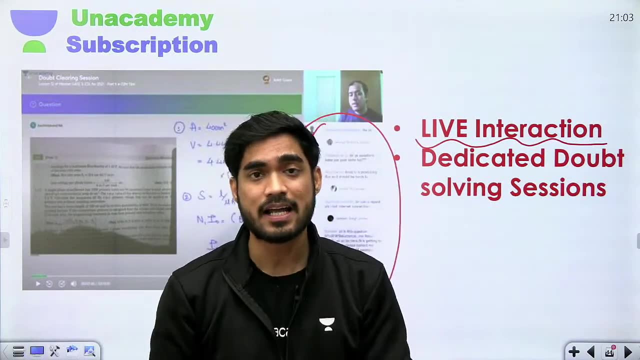 Okay, Live interaction. itna zyada live interaction hota hai, ki aapko aisa lagega, jase aap teacher ke saamne baith ho. Aap jo bhi ya comments me likhoge, usko teacher padh padh ke aapko aise jawab dega. aapko lagega, aap teacher se baat kar rahe ho. 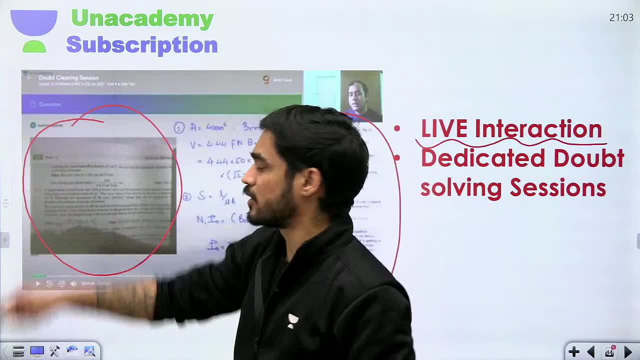 Okay, Aur koi bada question hai to aap, image kheech ke bhej sakte ho. You can take the image of a big question, you can send it to the teacher And there will be dedicated doubt solving session. 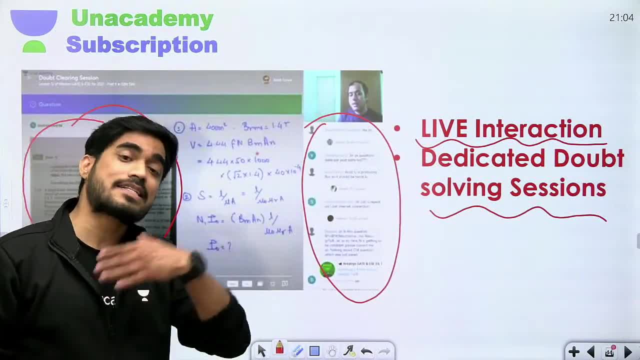 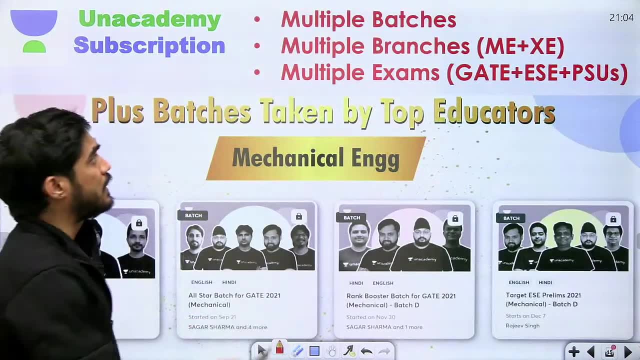 Matlab ki doubt classes alak se hoti hai. There will be doubt. There will be doubt classes separately, So you don't have to worry that you will not get time to ask doubts. Okay, And beta yaha pe multiple batches hain. 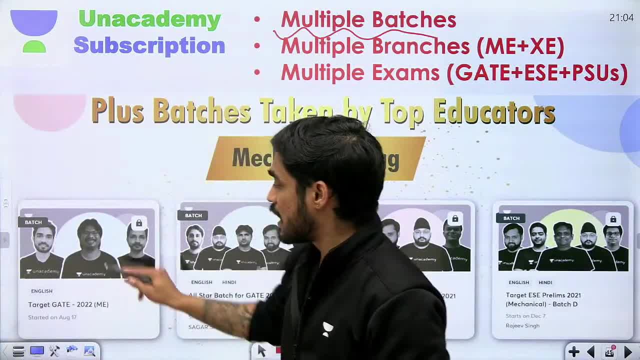 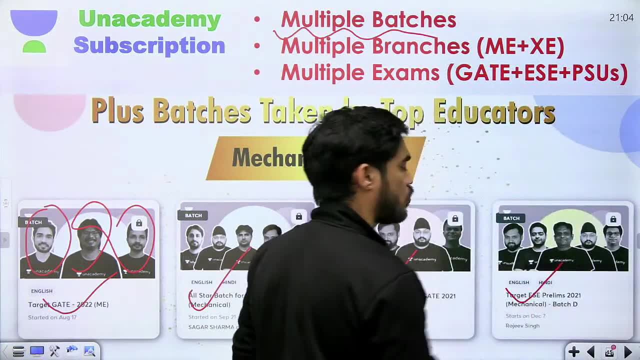 Har ek teacher ki apni alak. batches hain. Different different teachers come together to form new batches. Okay, So 22 ki batch, 21 ki batch, rank booster batch, ESC ki batch. Okay, You have so many batches and you can get into every batch. 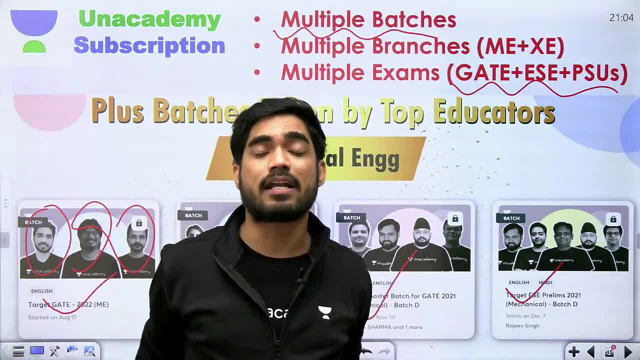 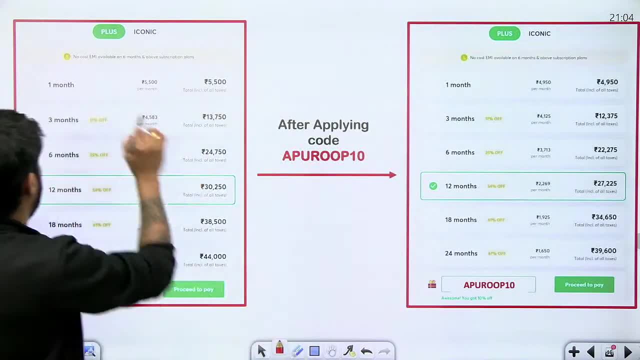 Har batch me ghus sakte ho, saari batch me ghus sakte ho. There is no limit on number of batches you can attend. Okay, All you need to do is take the Unacademy plus subscription One month se leke two year tak ka subscription available hai. 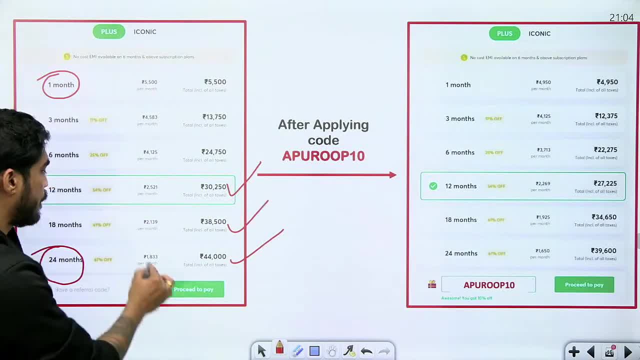 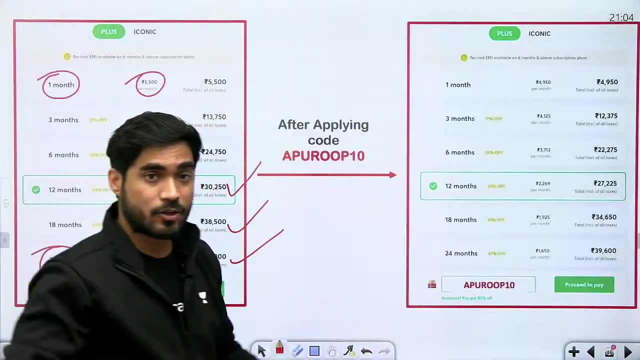 But I suggest you take one year, one and a half year or two year subscription, Because per month cost is very less And if you want to get advantage of all these awesome batches you need one year or one and a half year or two year. 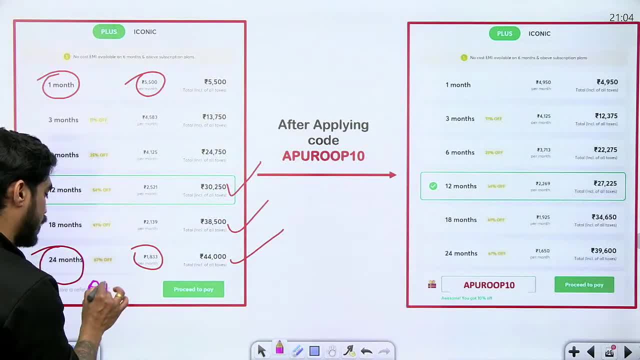 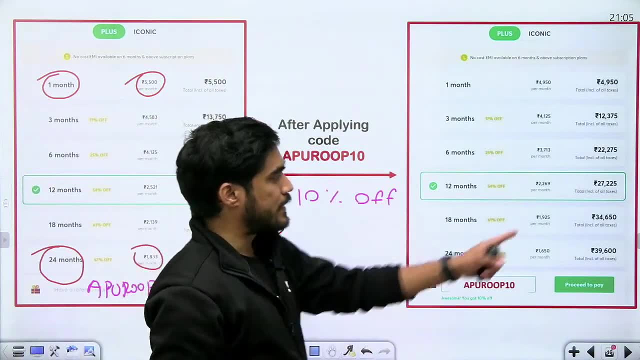 Okay, And you can use this referral code APPROVE10, in order to get 10% discount. Thik hai, Okay, 10% maximum off. Aapko mil jayega To aapke prices. ghatke itne ho jayenge. 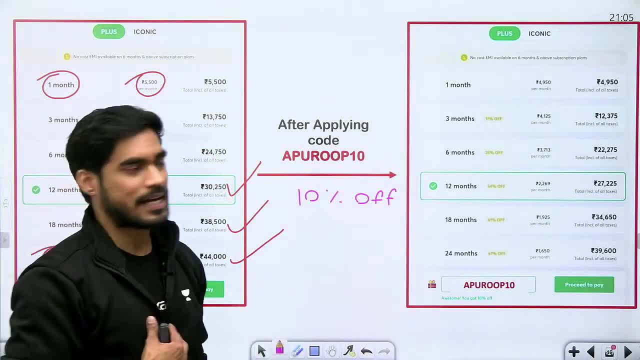 And beta, you will also get my personal guidance. Agar aap ye code use kar rahe ho, matlab aap bata rahe ho, ki aapko mujh pe bharosa hai, To aap mujh pe bharosa karke Unacademy agar join kar rahe ho. 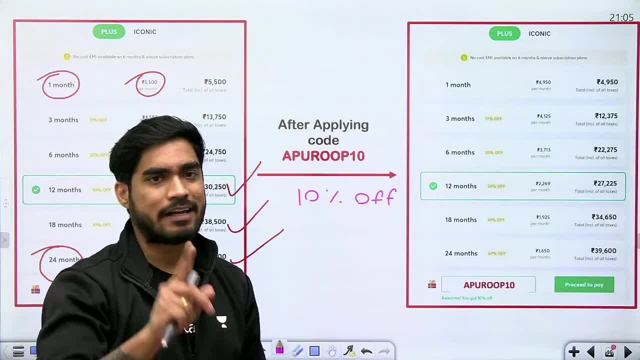 To beta main aapka bharosa to todunga nahi. I will always be with you. I will never leave you. I will be with you throughout your preparation. Aap 2 saal ka admission, lo 1 saal ka lo 6 mahine ka lo. 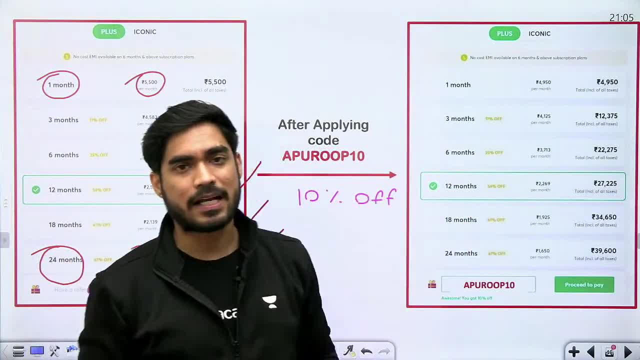 Main puri preparation ke dauraan aapke saath rahaunga, Aapke saath kadam se kadam mila ke chalunga. Koi tension nahi hai. Aap mere bharosa bilkul join kar sakte ho. 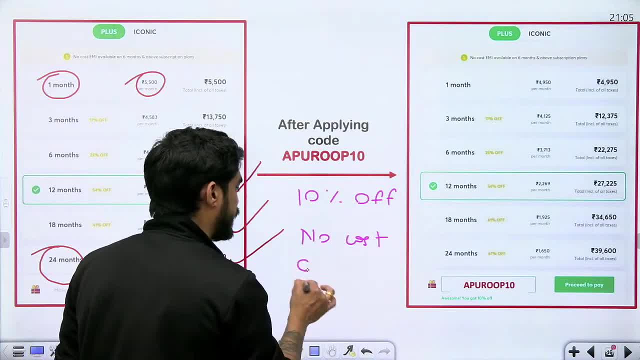 Aur aap ye fee jo hai no cost EMI pe bhar sakte ho, mere bhai, Monthly installment me bhar sakte ho Itna zyada affordable kar diya gaya hai, Education ko itna zyada affordable kar diya gaya hai. 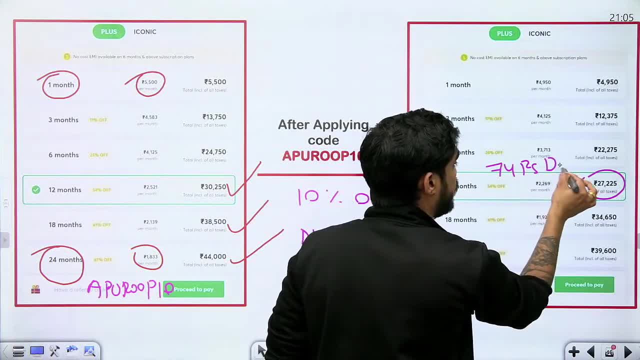 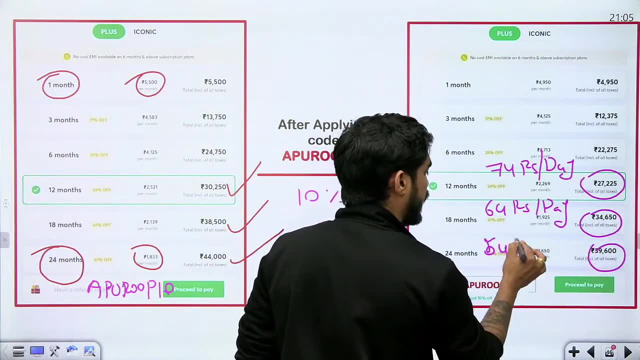 Isko dekho beta. This is lagbhag 74 rupees per day. This is lagbhag 64 rupees per day And this is almost 54 rupees per day. So you can imagine how affordable the education, online education, is. 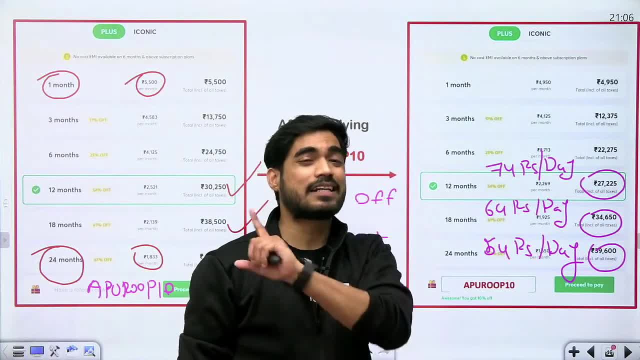 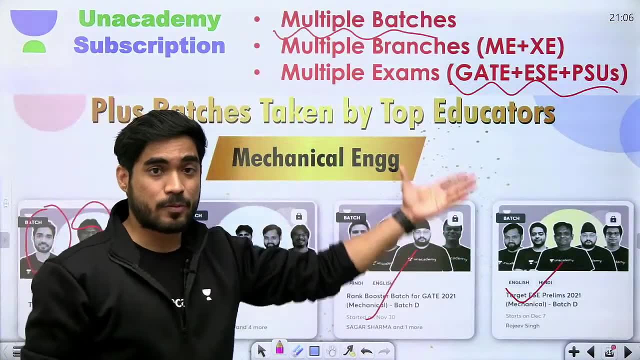 Due to Unacademy. Okay, 54 rupees per day. It is like nothing, Compared to what people used to pay for these education, For education from these lecturers. people used to pay in lakhs, And now only 54 rupees per day. 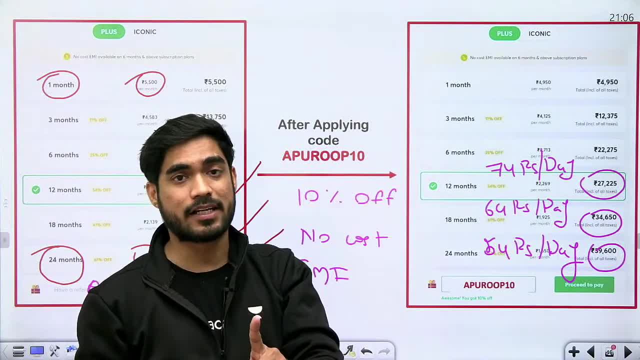 Sif 54 rupees. prati din me aap in awesome batches me admission le sakte ho Ek se zyada saari batch me saare educator, se pad sakte ho. Okay, So that is the beauty of Unacademy. 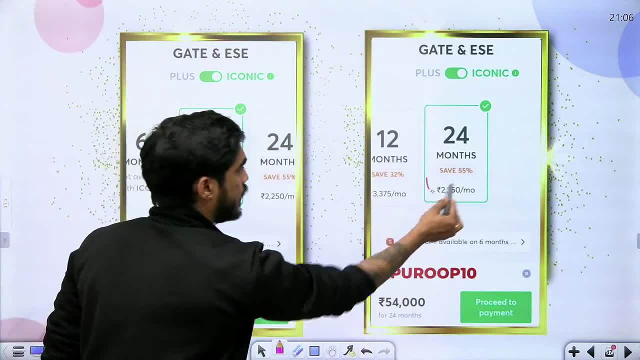 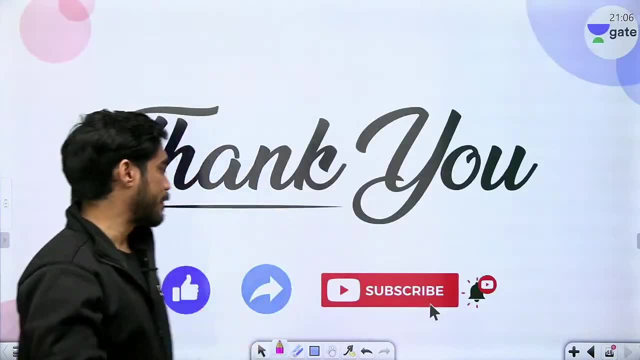 And you can also take 1 year and 2 year subscription of Unacademy Iconic. So I will be there soon on Unacademy platform. Okay, But before te travel like this, hit the like button, share this link and subscribe to this channel. 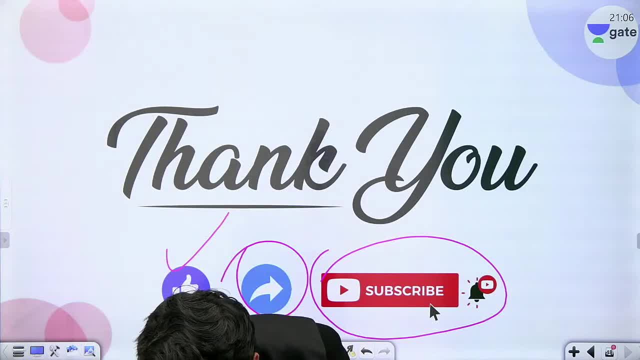 Okay, Thank you so much for watching. Thank you so much, Dibianshu Kalpesh Ayush. Thank you so much, Jino. Thank you so much. Thank you so much Aliy aircraft, All of you. 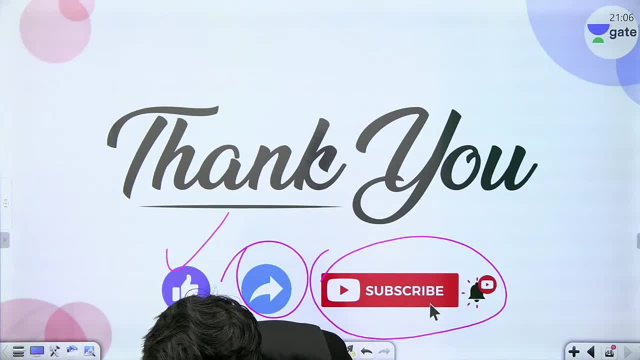 Thank you so much, Priyanka. Thank you so much. Thank you so much, Brijesh. Thank you so much, Ashwina. Thank you so much. Thank you so much for lovely messages. Thank you so much. Thank you so much, Carla. 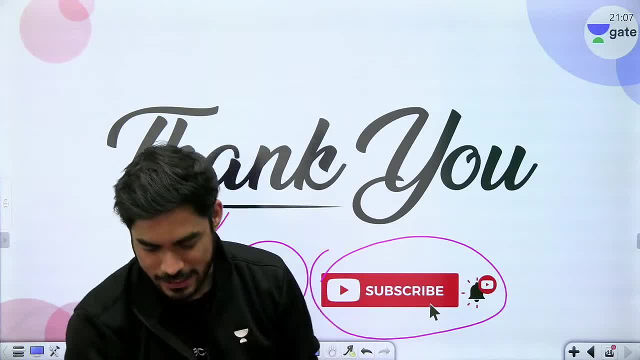 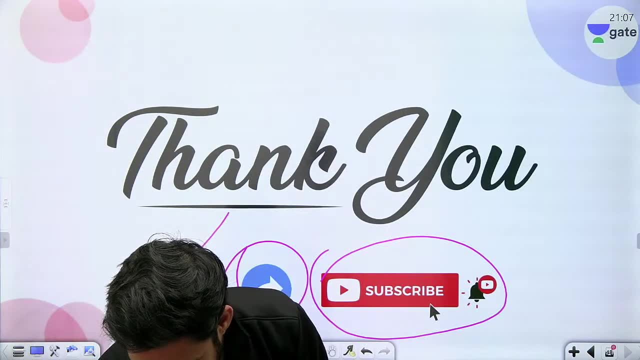 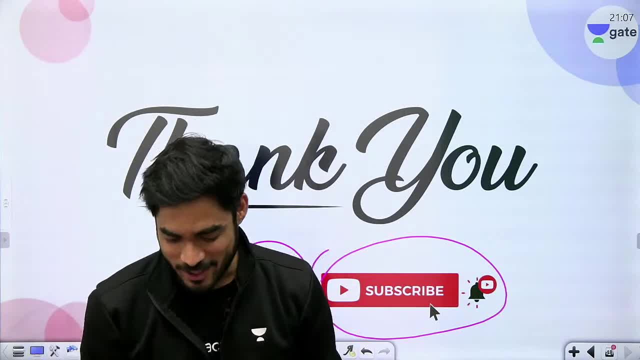 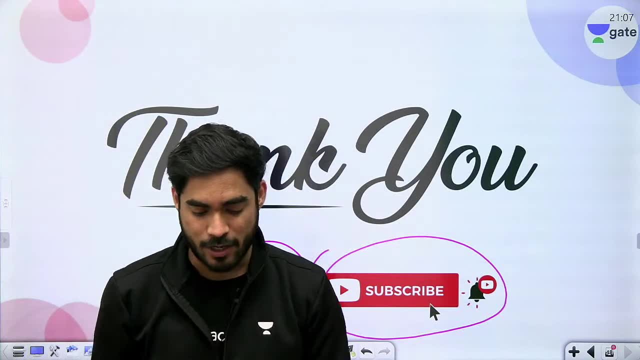 Lal fool, Peela fool. Thank you so much. Thank you so much, my brother. Thank you so much, Uday, Thank you so much, Nitish. Yes, yes, Everyone has to come tomorrow, my brother, And make it happen. 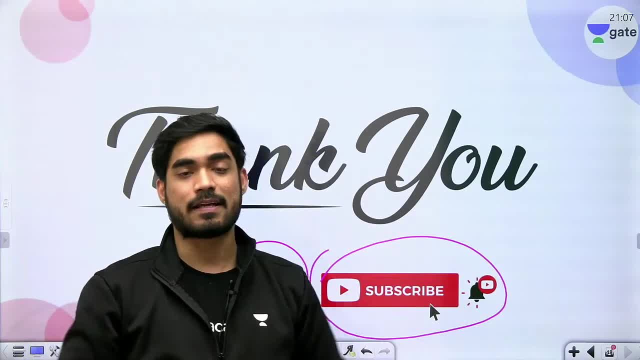 Together. Okay, We will sit for 8 hours and show everyone that we can do it. If we can do it, then we will do it. If we can do it, then we will do it. my friend, If we can do it, then we will do it. 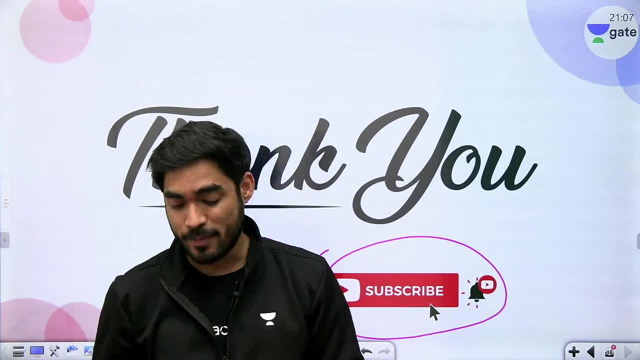 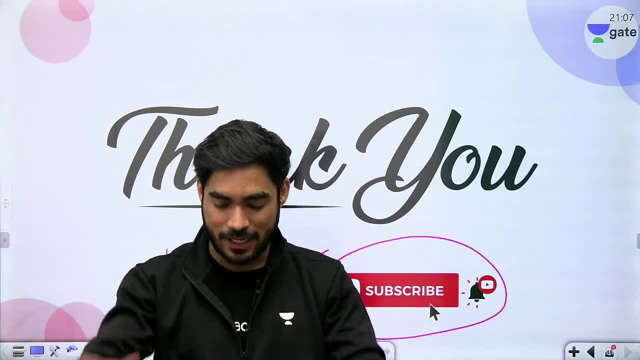 Yes. So reach tomorrow to make it happen. Tomorrow, everyone, at 9 in the morning, wash your hands and feet. No, not wash your hands and feet. No, wash your hands and feet and reach. After doing puja, go to the temple mosque, take the blessings of your parents and sit. 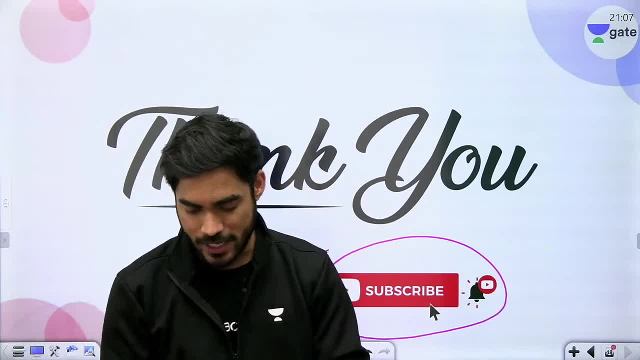 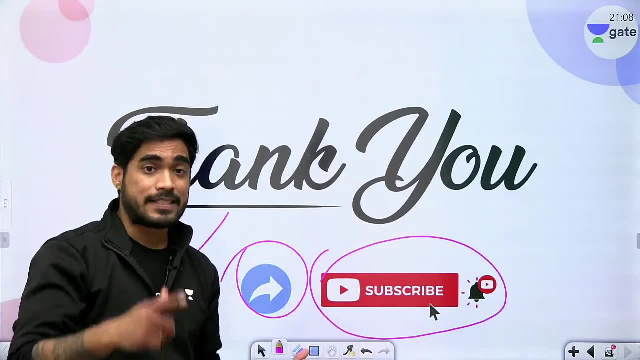 And 8 hours continuously, we will make it happen. The whole machine design. Okay, Okay, Okay. Thank you so much, guys, for all the love and support. I will keep on coming. This is not the end, my friend.